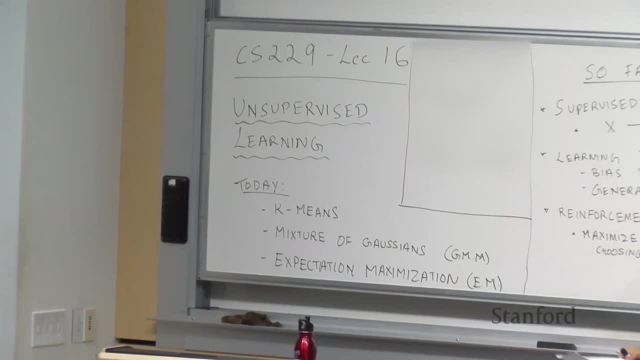 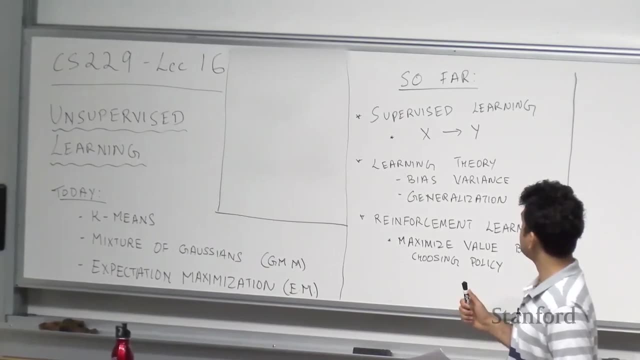 And um to- jumping into today's topics. uh, so what we've seen so far is, um, the first few weeks. first, uh, three, four weeks or so. we covered supervised learning, where we were trying to learn a function that maps x to y. 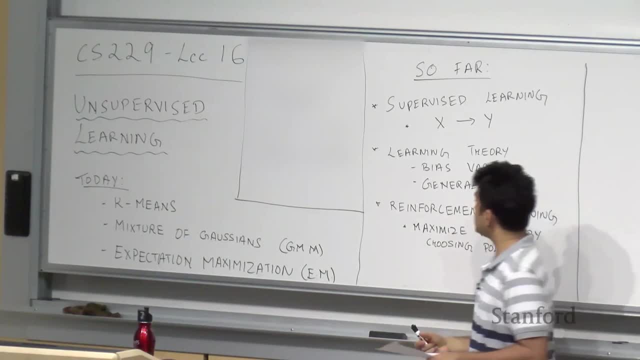 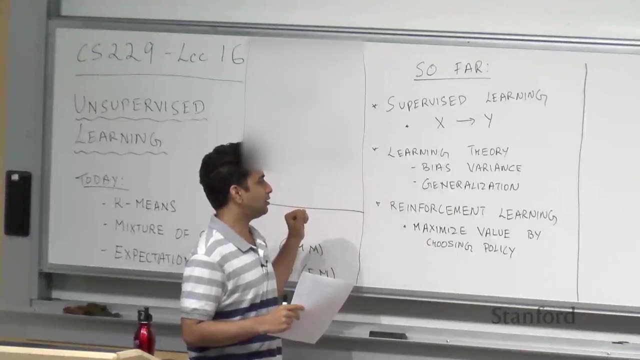 and we are given pairs of x- y as our training set or examples. And then after supervised learning, we went into some learning theory. We studied bias variants, uh, trade off in the bias variants analysis and saw a little bit into generalization. 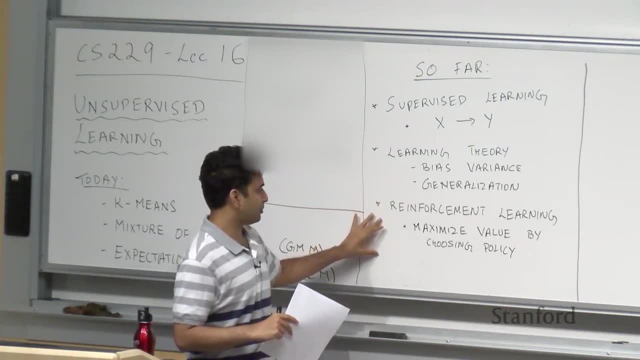 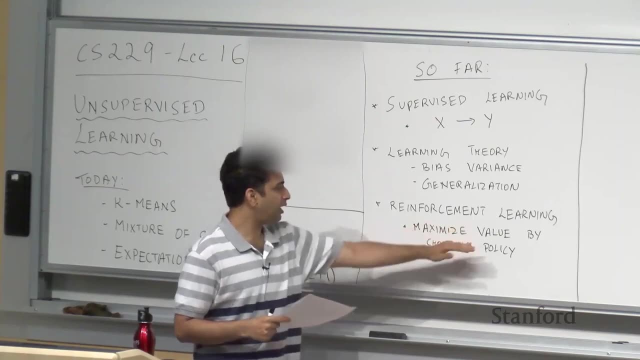 And then we um. last week we saw reinforcement learning, where the goal in reinforcement learning is, rather than minimizing some kind of a loss function, we wanna maximize the value by choosing a suitable policy right, And here value is the long-term. 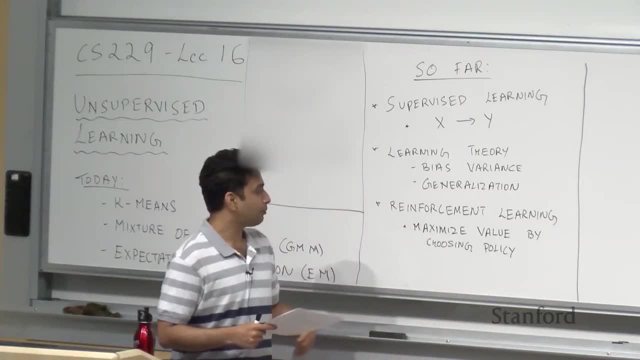 uh, cumulative sum of discounted rewards, and we want to maximize the long-term reward by choosing a policy. Now, the new chapter we're gonna start today- starting today is unsupervised learning And in the unsupervised learning case, um, we are given a dataset generally. 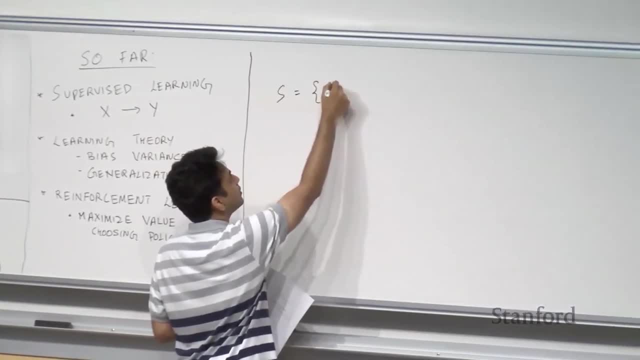 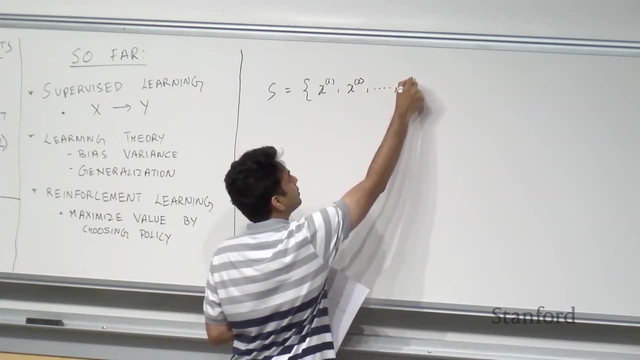 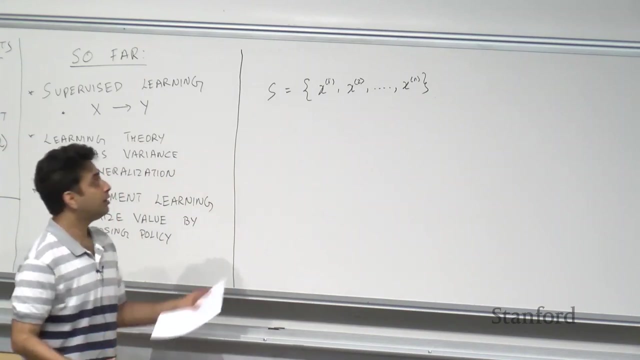 um a collection of x1, x2, etc. xn right, And we do not have a corresponding y variable associated with each x variable. We're just given a- a set of collec- um um examples um. 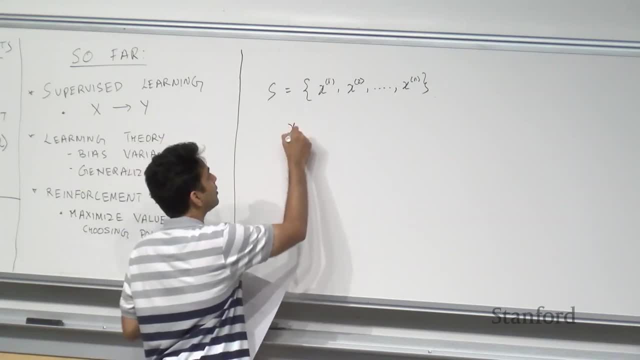 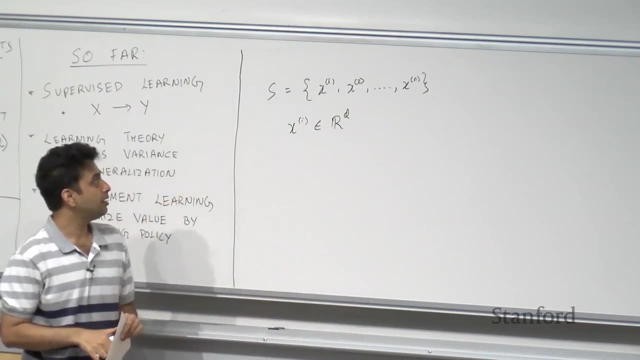 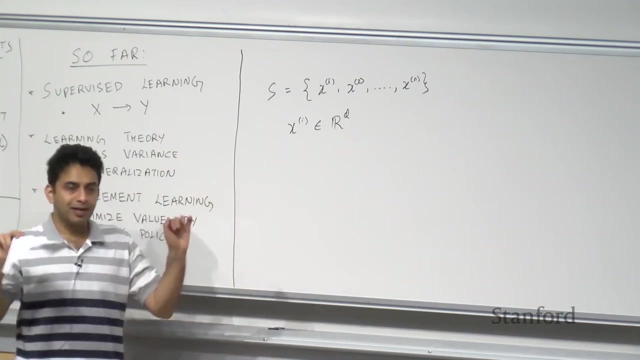 x- a- a set of x's where each x i is in Rd in a d-dimensional real space, for example, And our goal is to learn some kind of a structure in these x's right. We don't have a corresponding correct answer. 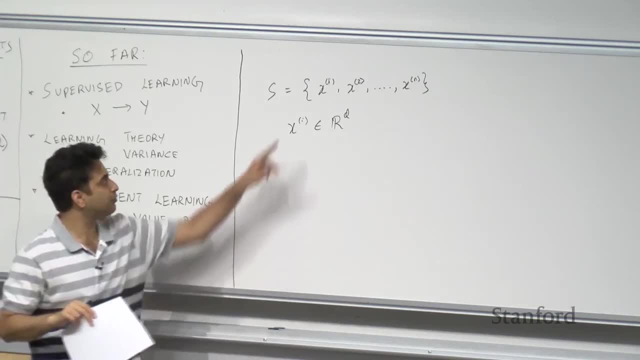 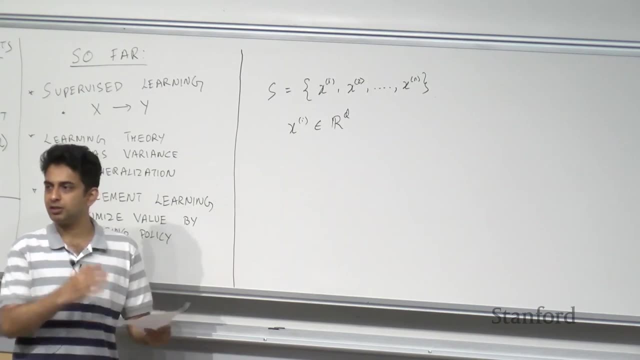 We don't have what's otherwise called supervision of what the correct answer is for each x, But in general, we are just given some- some- a collection of x's and our- and we are- the goal is to find some kind of an interesting structure in. 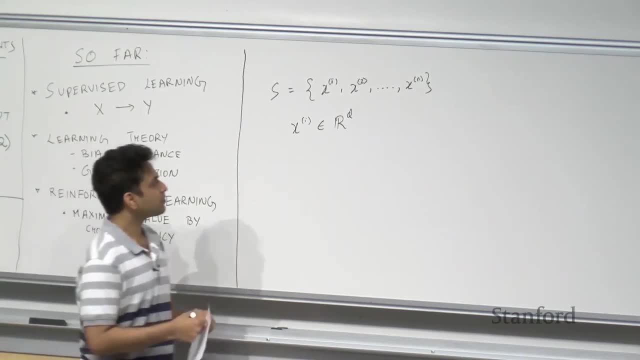 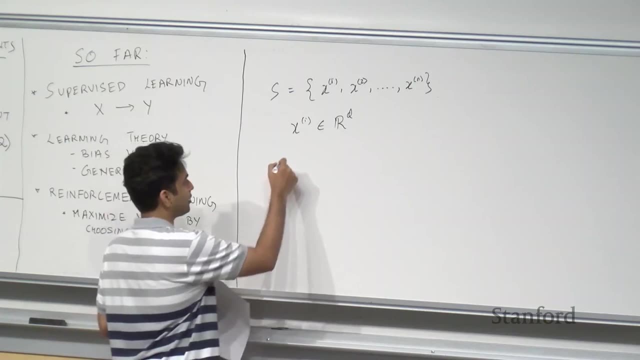 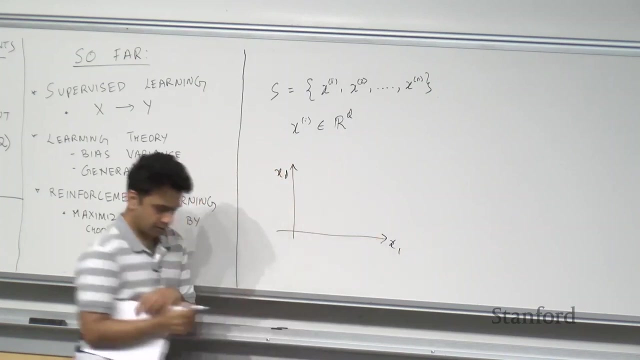 these x's. that hopefully gives us some new insight, right? So um, we've seen logistic regression before And in the case of logics- logistic regression, you know. um x1, xd- Let me use a few colors here. 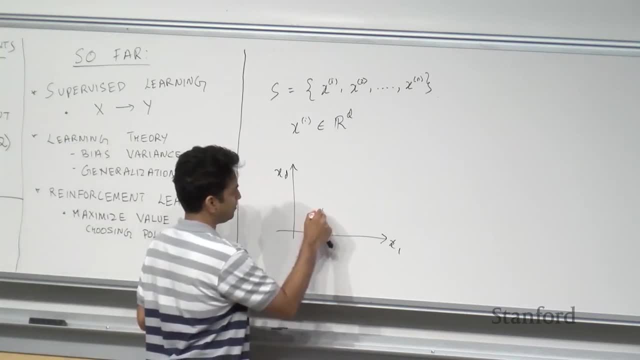 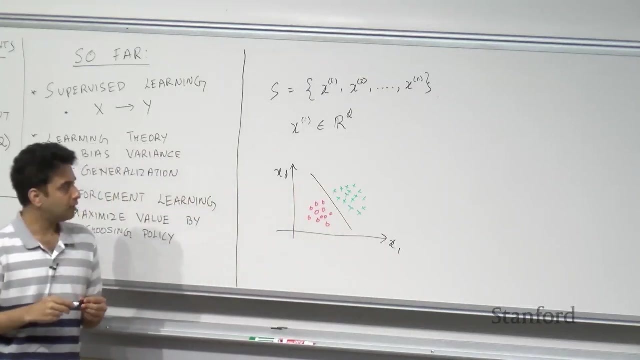 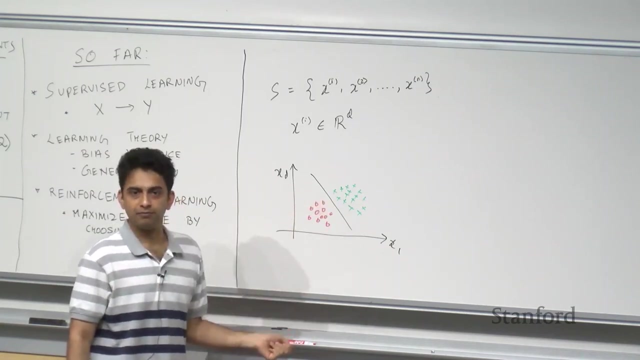 We had some- we were given a dataset like this and our goal was to find a separating hyperplane. right, That was-. this is- is supervised learning, because we are given the correct answer. that is the color of each point along with the point itself, right? 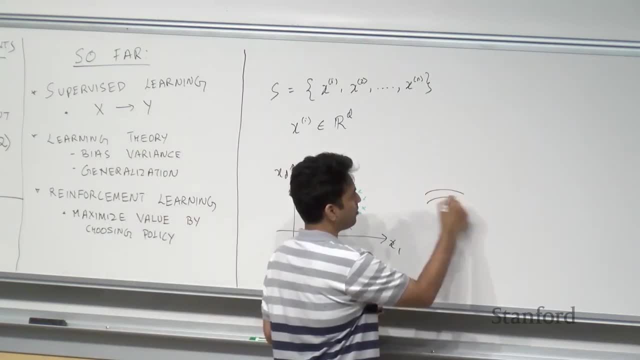 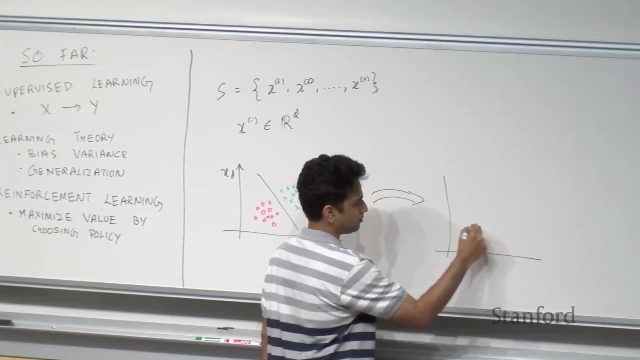 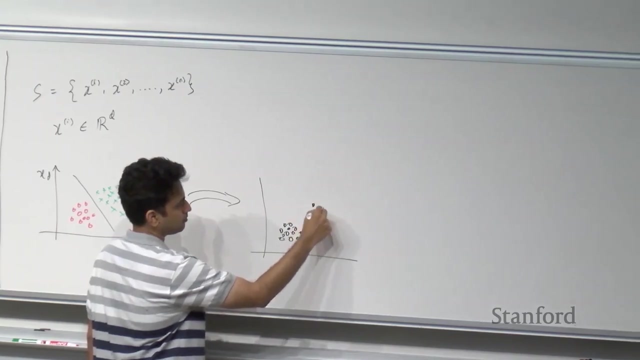 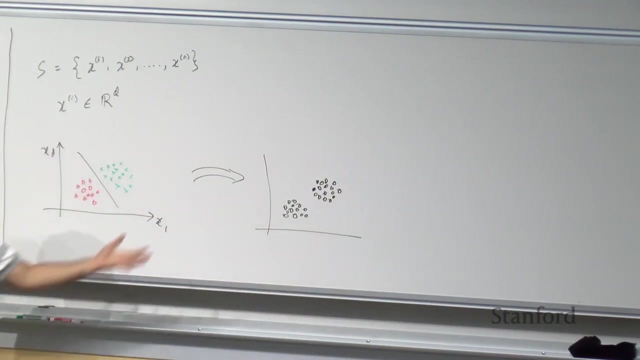 Whereas in the unsupervised learning, a sim-, the-, the- the problem would translate to something like this: right, We are given some points, just the x's, okay, And our goal now is to learn some kind of an interesting structure here, right? 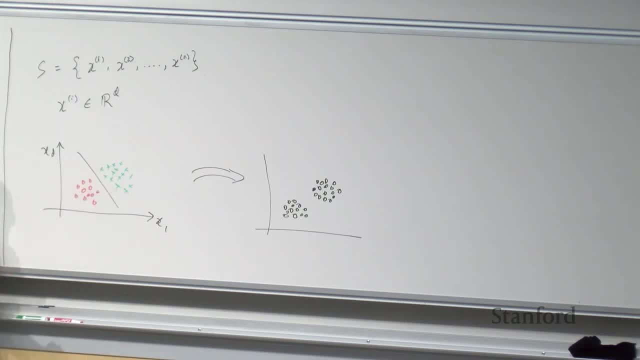 Previously we had- we had- the correct answer for each uh, for each input. Now we are just given a collection of x's and a reasonable uh structure to find in this. are these two clusters, So, loosely speaking, uh? 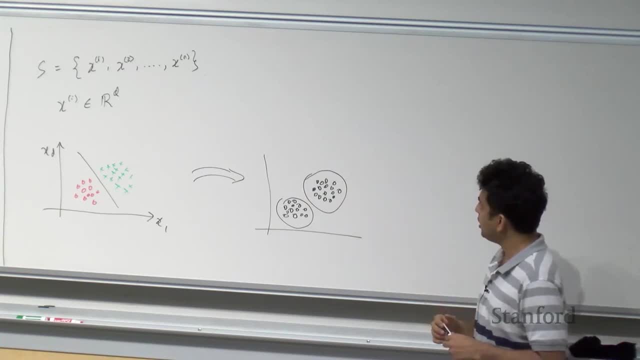 we want to look for- for uh, such structures with- when we are given just x's. However, this problem is generally not very well defined, right? In the first case, for each point, we- we were told what the correct answer is. 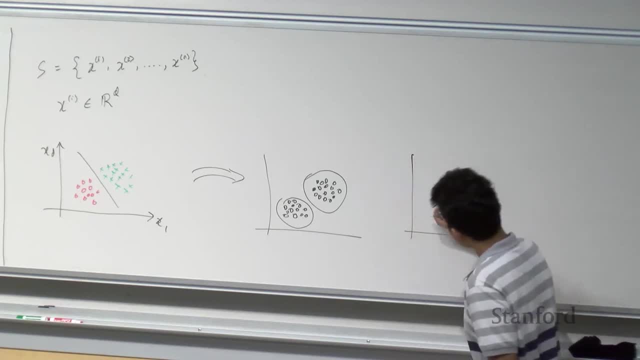 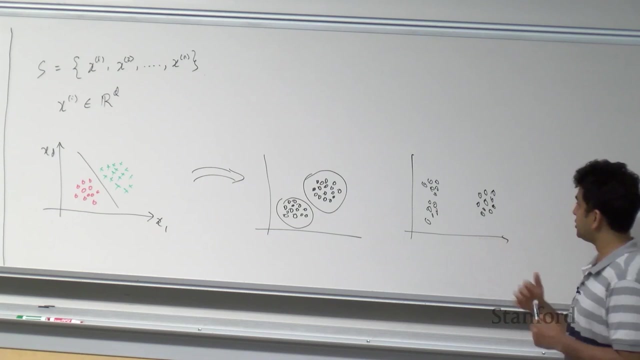 But consider a problem like this right And if- if you are asked to find an interesting struct-, substru- structure in this kind of a data, it would be totally reasonable to say: this is one cluster, this is one cluster and this is another cluster, right. 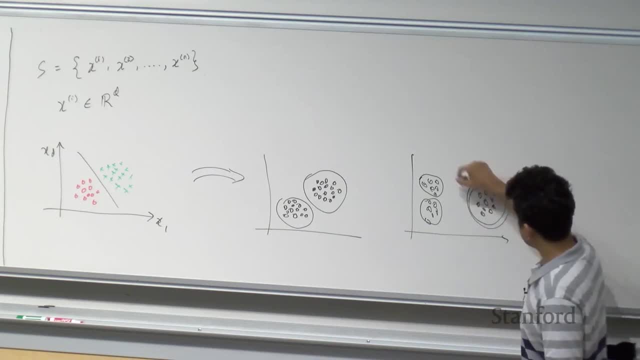 And another totally reasonable thing would be to say: this is one cluster and this is one cluster, right? So, in a way, there is no correct answer, so to speak, And our goal is to learn some kind of an interesting um um structure in the presence of such kind of ambiguities, right? 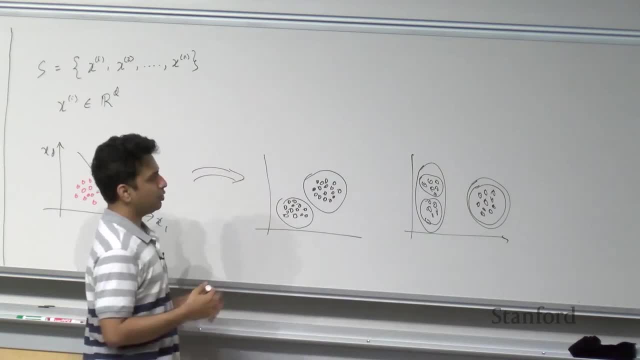 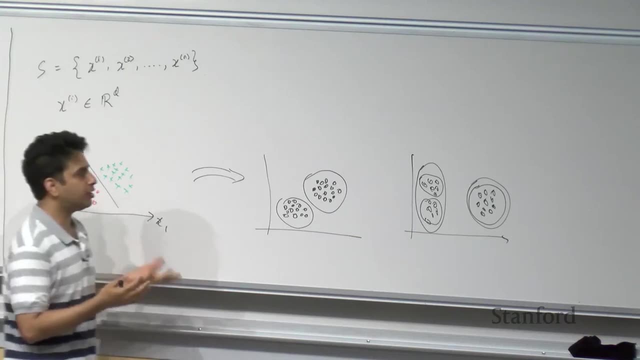 Uh, the um, the way to- you- you wanna think of this- is classification. problems in the supervised setting are somewhat related to clustering problems in the unsupervised setting Right, Where the cluster identity is like the class label and we want to looking at just the x's. 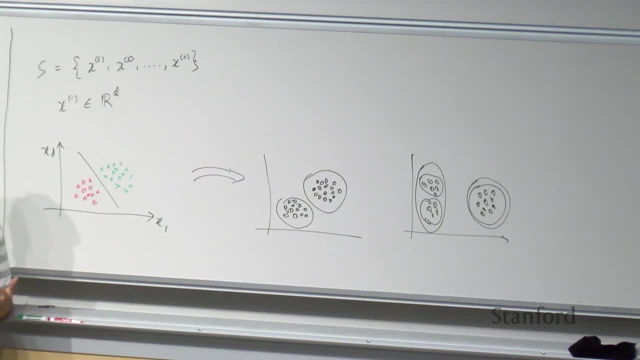 find out both how many number of classes there are and also to which class each example belongs to, right And um, why would this be interesting? So, for example, this would be interesting, for example, for uh, in examples where, supposing, you have, 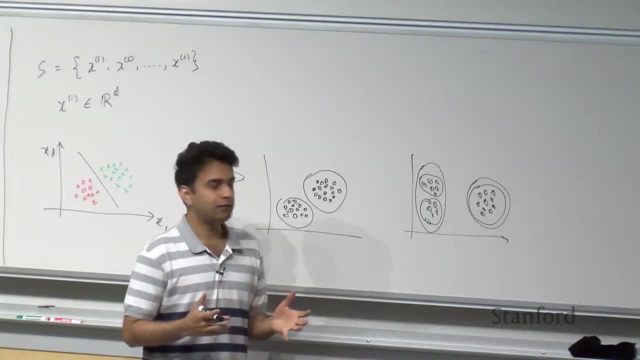 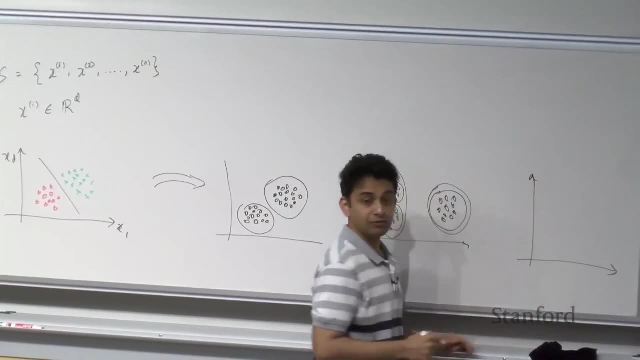 um, um, you're working at a marketing department and you have information about your customers, Right, And the information about your customers can be represented in in- uh, you know, in- in some kind of a vector space where you know you have the age of the customer here. 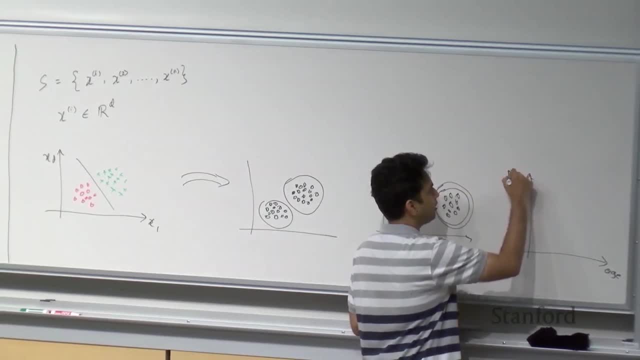 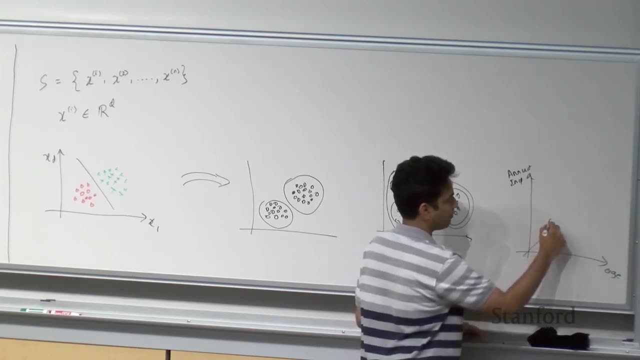 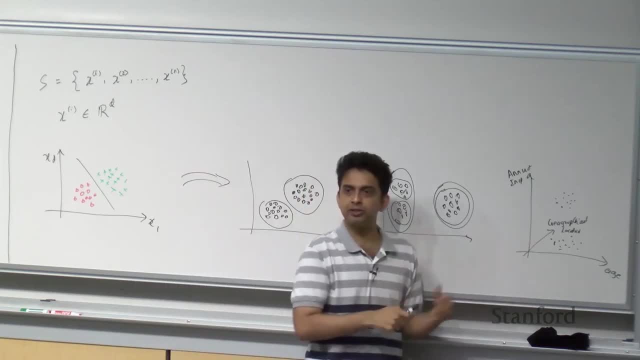 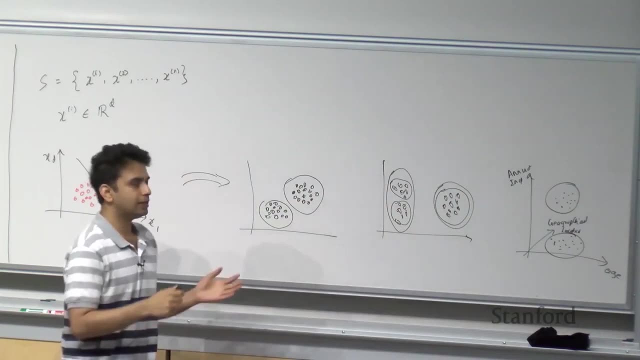 you might be interested to perform some kind of a market segmentation to identify you know groups of customers so that you can do some kind of a targeted, you know advertising or marketing campaign or some such thing right. So that- that's just one example of how- why unsupervised learning might be. 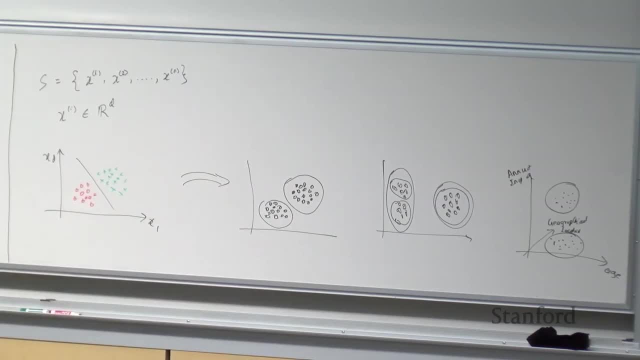 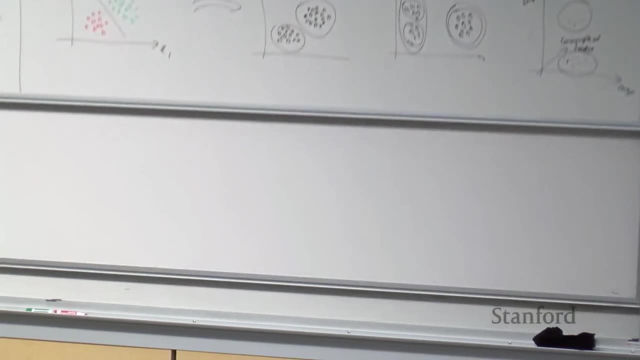 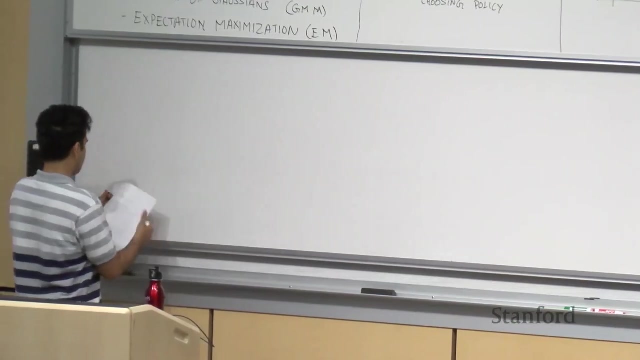 you know uh interesting. So the uh first unsupervised learning algorithm that we'll be seeing is something uh called as the um, the K-means clustering algorithm. The K-means clustering algorithm- um is- is uh pretty straightforward. 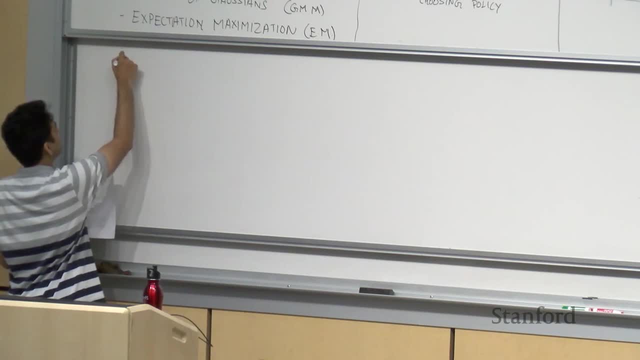 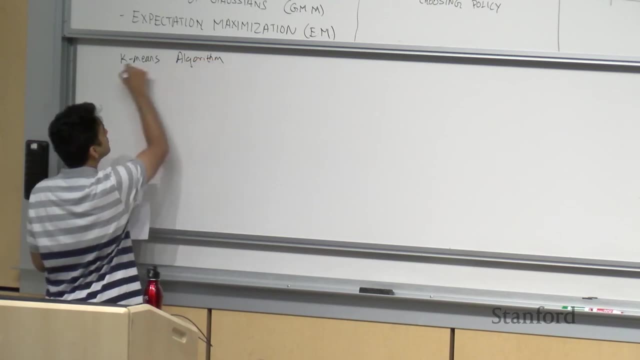 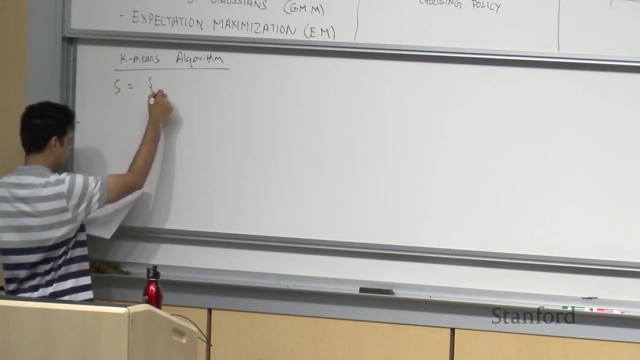 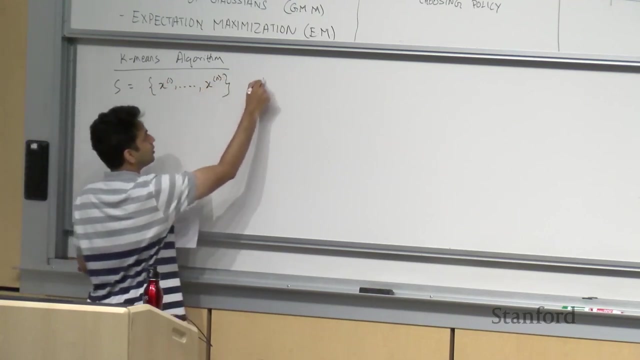 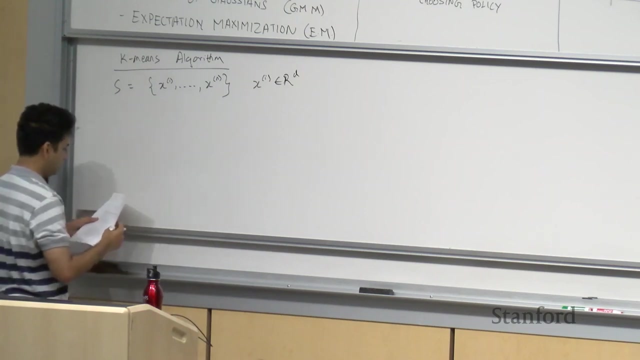 This is probably one of the simplest algorithms, uh for unsupervised learning, K-means algorithm. So you're given a dataset of n examples, X1 through Xn, where each Xi is in Rd right, And our goal is to group them into K clusters, right. 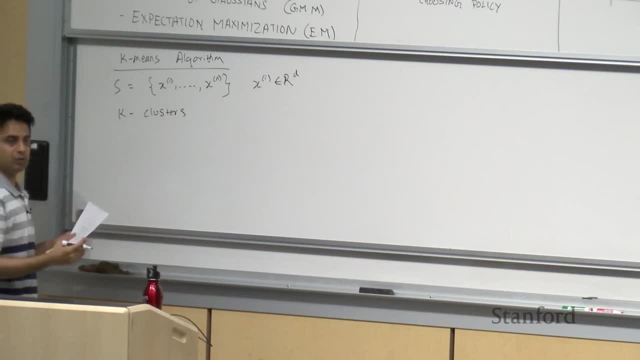 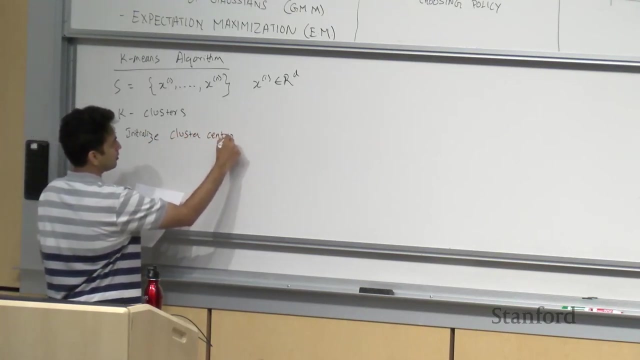 And for the purpose of the algorithm we are- we'll assume that Kn is given to us And the algorithm goes like this: Initialize Cluster centroids mu1, mu2, muk. So you have one um um centroid per cluster, where each of them are in Rd randomly, right? 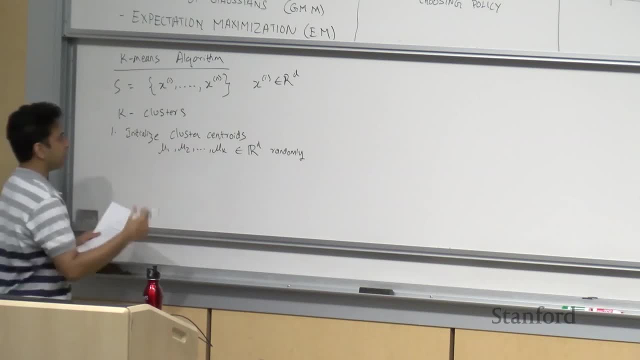 So each of these mu1,, mu2, muk, uh is a vector Previously in- in uh. our notations generally: uh, having a suffix to a variable generally meant it was a scalar right, But in- in this case. 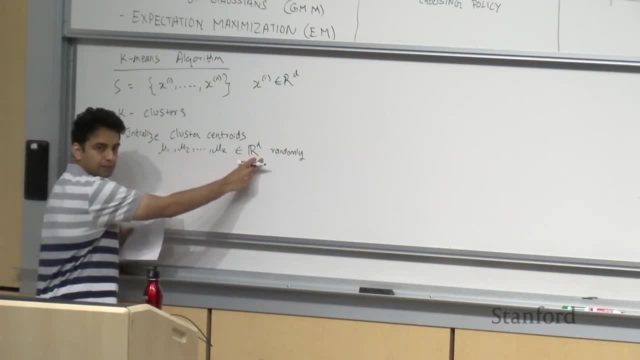 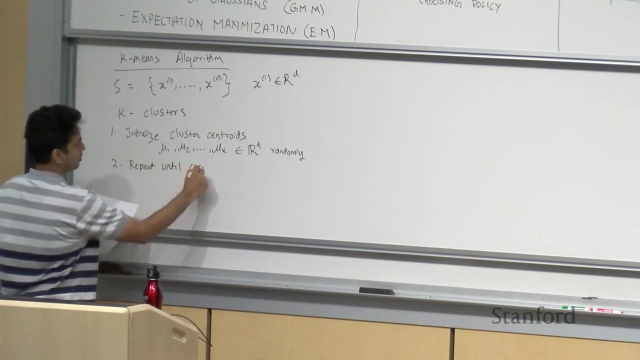 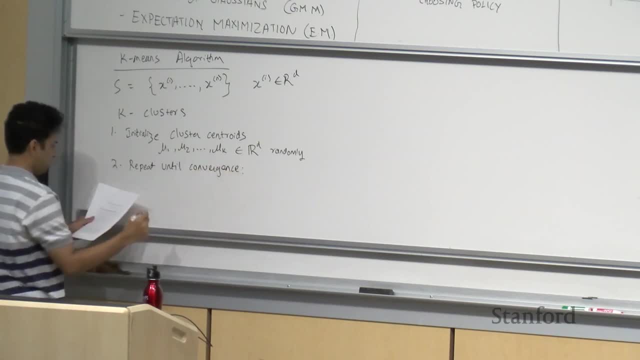 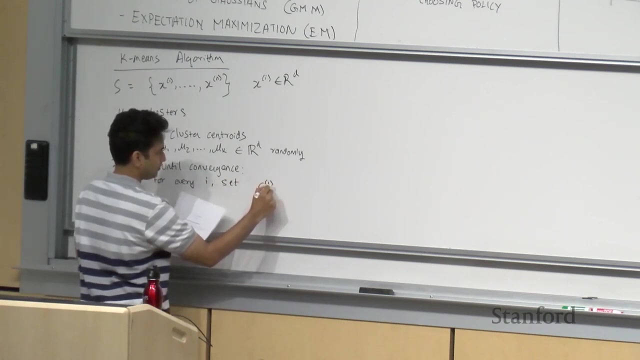 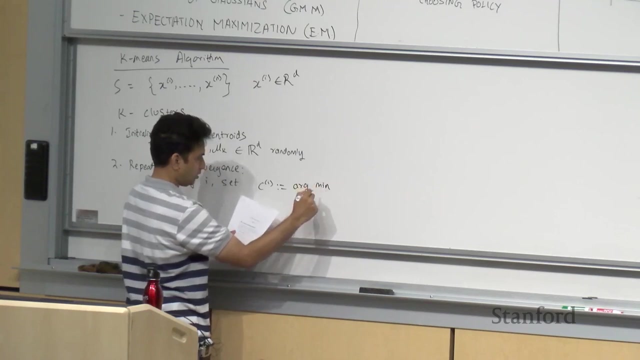 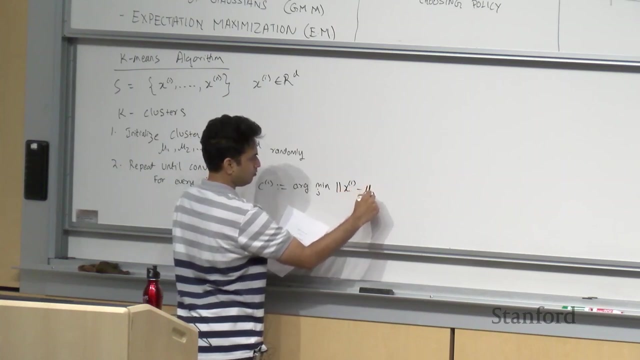 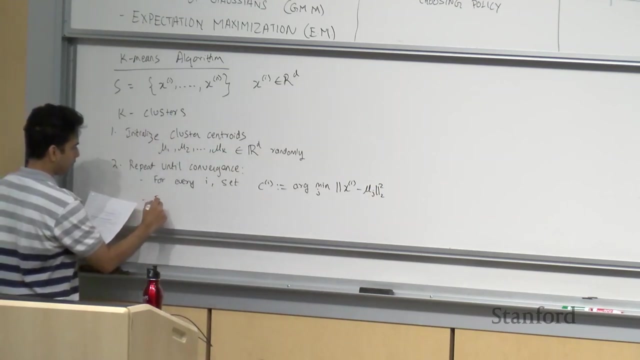 Repeat until convergence. For every i, where i denotes the uh example, number, set ci equal to arg, min j, xi minus j, And then that's step 1 and step 2 for every j where j is now uh, uh, where j indicates the cluster identity. 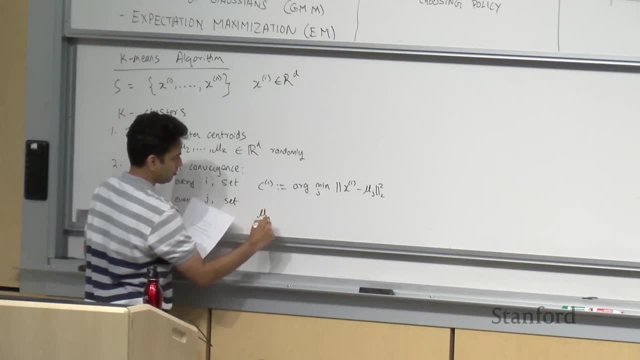 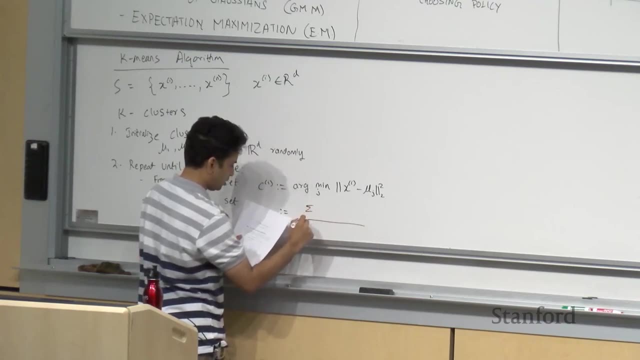 Then it lets us uh, uh, um, uh, sum over j. the set mu j equal to sum over i equals 1n indicator of ci and i equals 1n indicator of xi. Uh, but we can also uh. 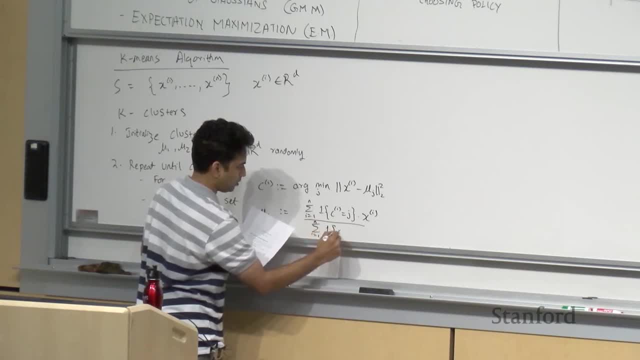 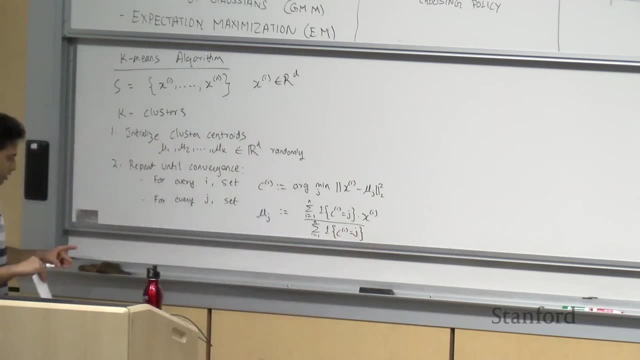 we can also do this. So we can do this. We can do this. c i equals j. So what are we doing here? K-means is an iterative algorithm where we are given a set of n examples which we index by i. 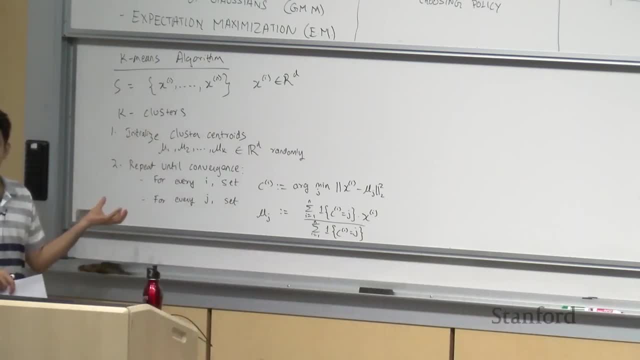 and we want to identify k clusters. where the k clusters are indexed by j, We initialize the cluster centroids randomly. where mu 1 through mu k are- are each a vector in Rd and we repeat until convergence: where for every- for every i. 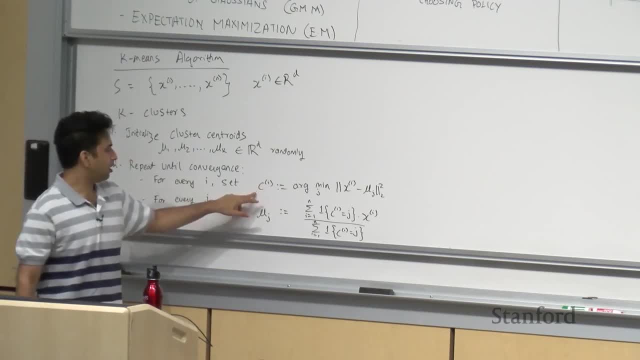 we set c? i Here, c uh c. you can think of c as an array of length n, where for each example there's a corresponding c? i, for every x? i there's a corresponding c? i, and we set c? i to be the identity. 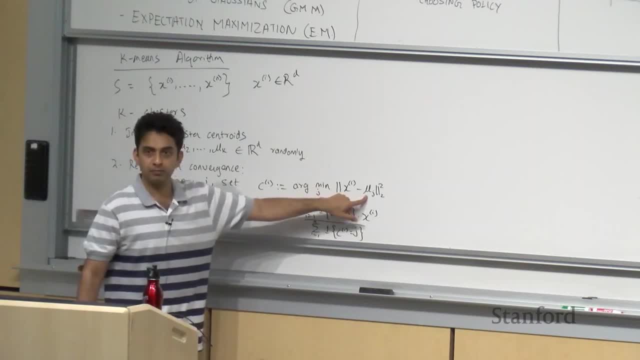 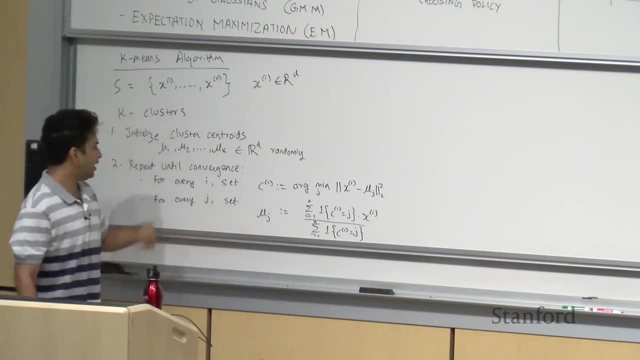 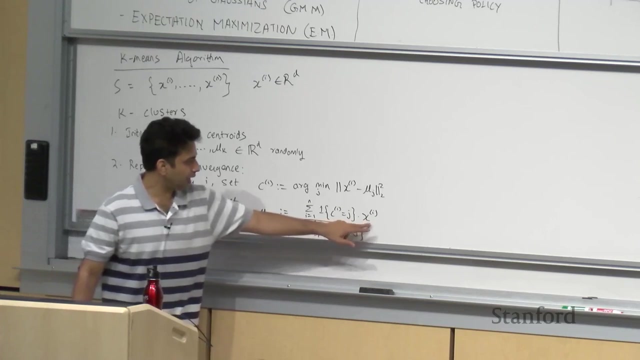 that's the R-min of j identity of the nearest mean right And based on the set c i vector or c i array. we then recalculate mu j, where mu j is calculated as the mean of all x i's for which c i equals j. 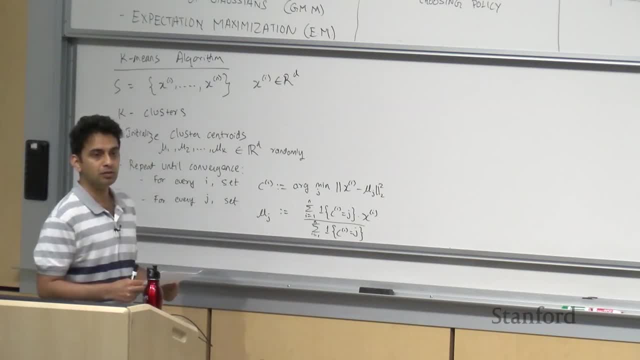 Yes question. So, uh, as I said already, for now, let's assume k is told to us. you know, we- we are given what k is and this is the algorithm, right And the way. um, it's- it- it's a pretty straightforward algorithm where we 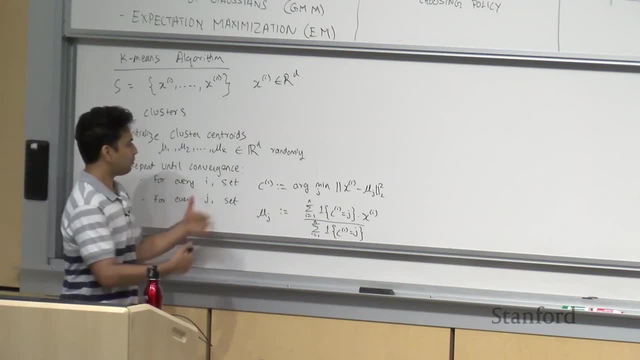 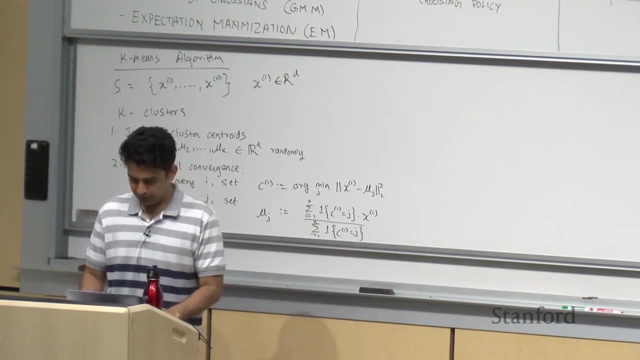 uh, where we alternate between one step where we are id- where we are calculating the cluster identities for each example, and in the other step where we are recalculating the cluster centroids, And this is probably seen through a simple uh visualization. 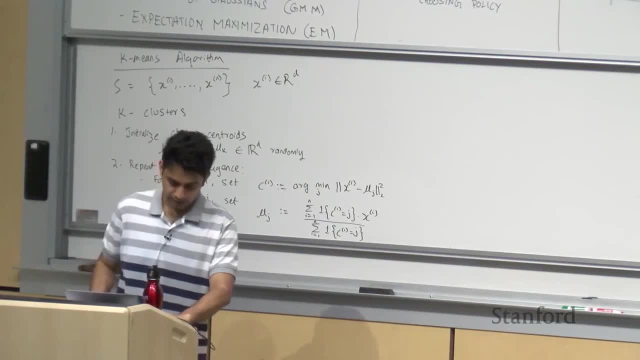 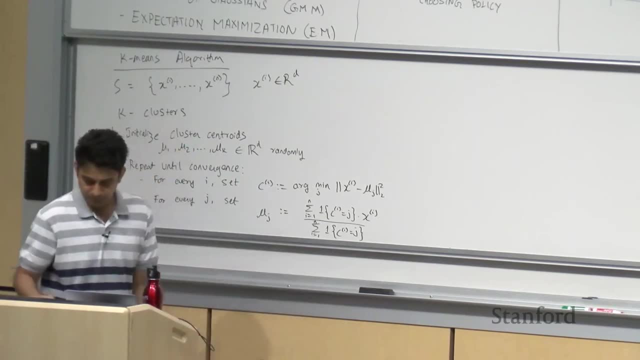 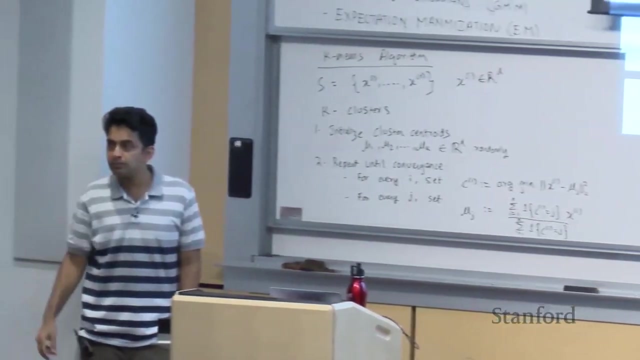 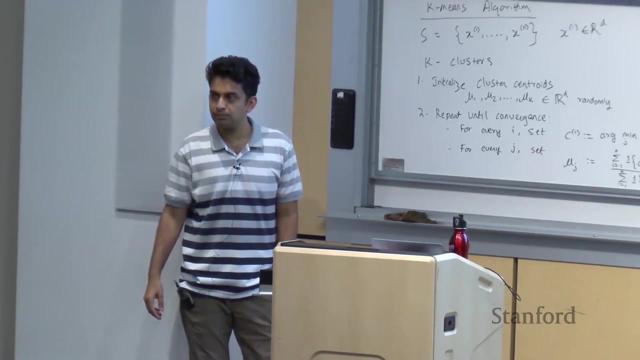 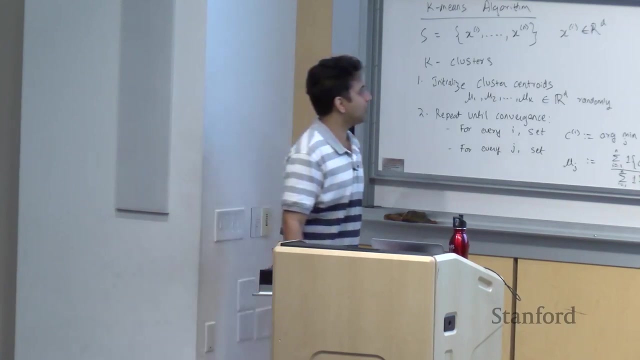 which we'll have a quick look at. Any questions on this. so far, Yes, question So-. so, uh, the question is: uh, what happens? uh? can we use, um, uh, an answer? supervised learning setting to learn. 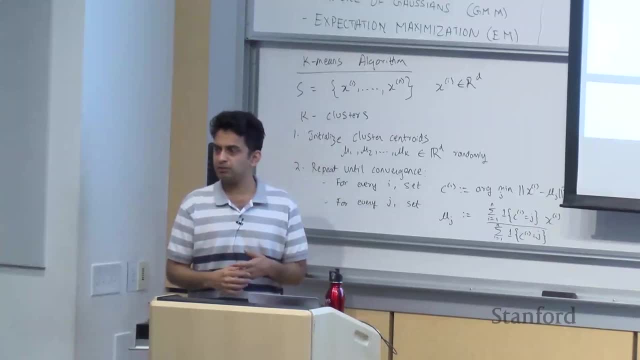 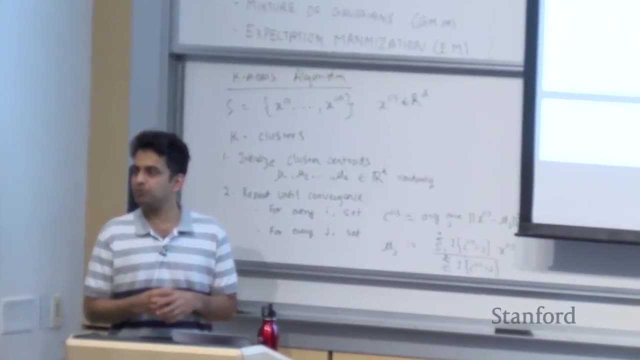 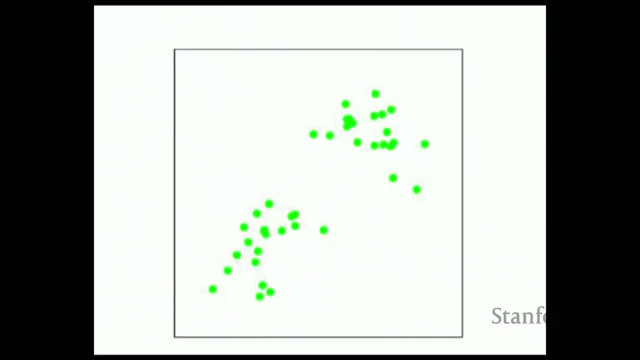 the different cluster centers and use that as a classification algorithm. Yeah, it might, or it might not behave the same way as a supervised learning algorithm. Yeah, So supposing this is, you know, uh, think of this as a collection of points that are given to us. 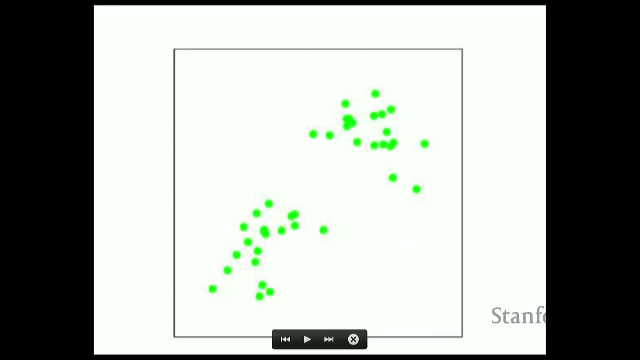 where each green point is, um, you know, is-. is- is uh a data point in um x, i and r, d. And the way uh, the algorithm uh works like this: We st- here. we assume k equals 2,. 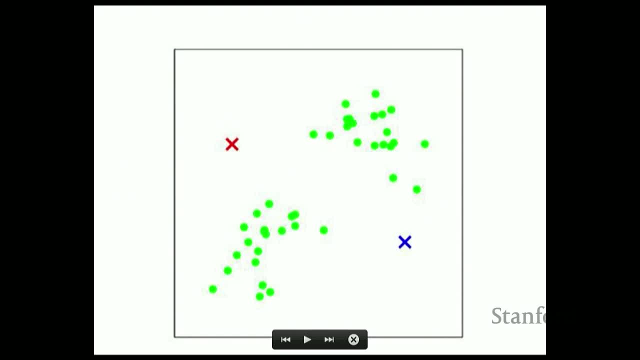 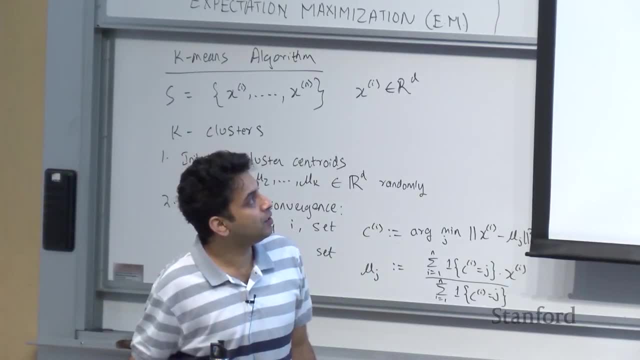 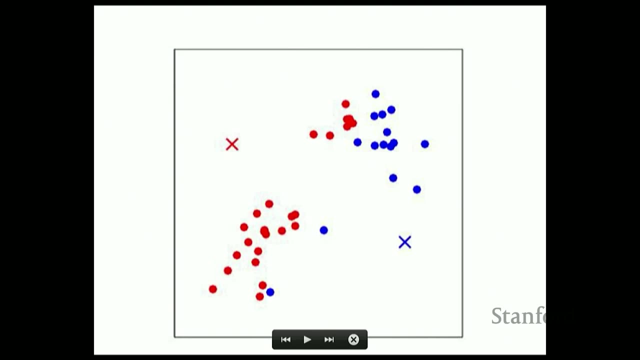 and the red x and the blue x- you can think of them as mu 1 and mu 2,, which are randomly initialized. And in the first step, what we do is, for each point, for each point x, we identify the nearest cluster right. 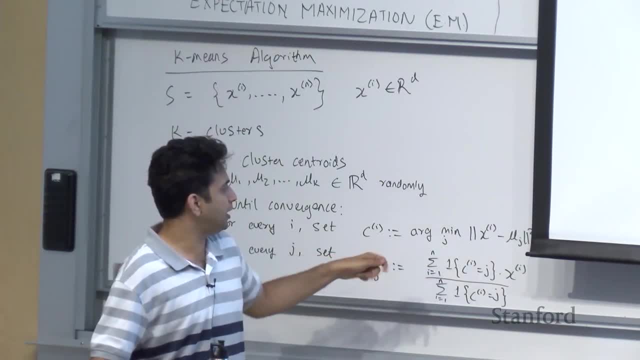 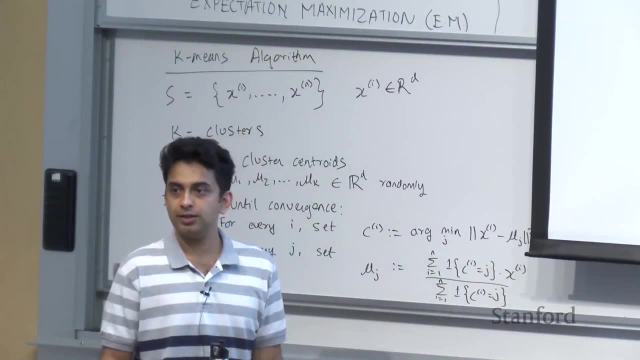 We- we- we set c i to be uh, the nearest cluster right. We set c i to be the identity of that cluster which has the smallest L2 distance between that point and the uh cluster centroid. So over here the red dots are those for which the red x is closer. 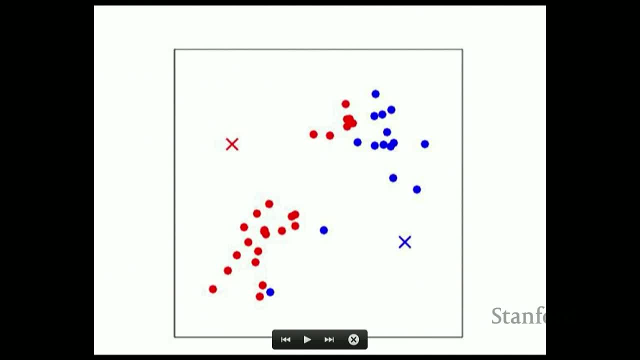 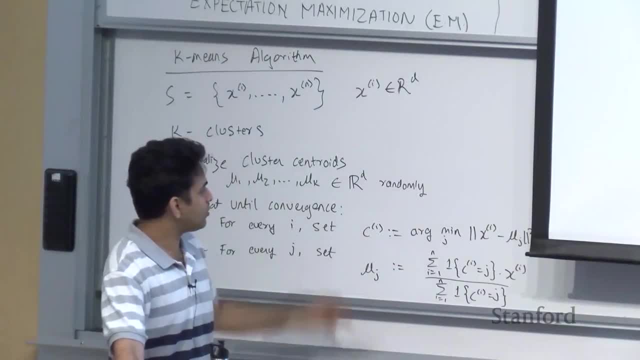 and the blue dots are those uh uh x's for which the blue x is closer right. So this is like setting the- the c? i's in the first iteration And once we set the c? i's in the next step. 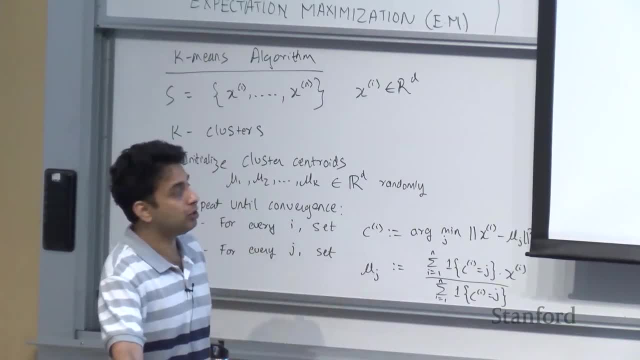 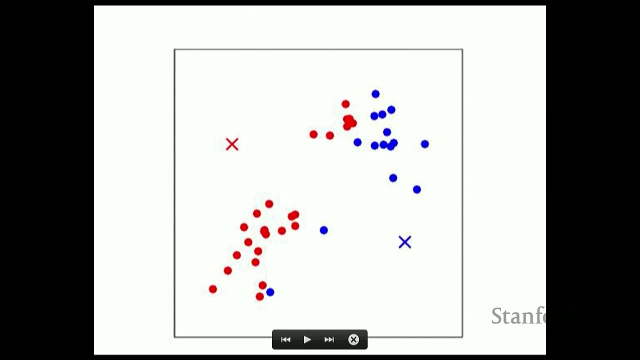 what we do is recalculate the mu-, uh, the mu j's. So what happened here? I'm gonna go back one slide. So, uh, at this stage we set all the cluster identities And in the next stage what we wanna do is recalculate the red x. 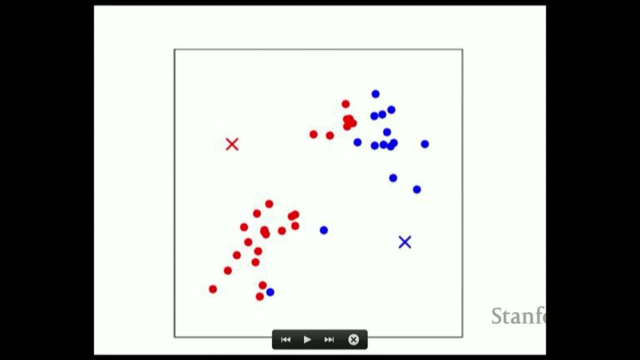 that is, uh, the mu to be at the middle of the red points, at the red circles, And similarly recalculate the- the blue mu to be the center of all the blue circles. And that's what happens in the next slide over here, right? 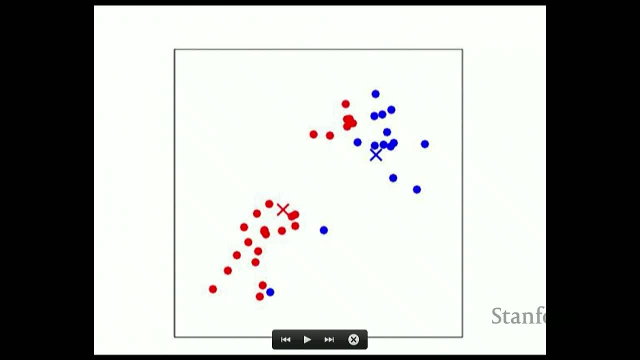 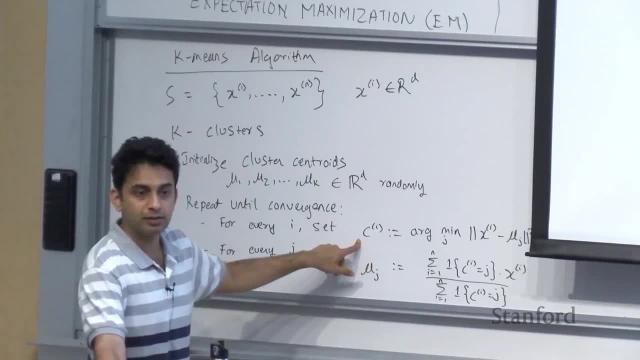 So this is- this is just taking the mean of all the points of uh, the corresponding color. And then what we do? we repeat and assign new cluster identities, reevaluate all the points to see which new cluster centroid they are closer to. 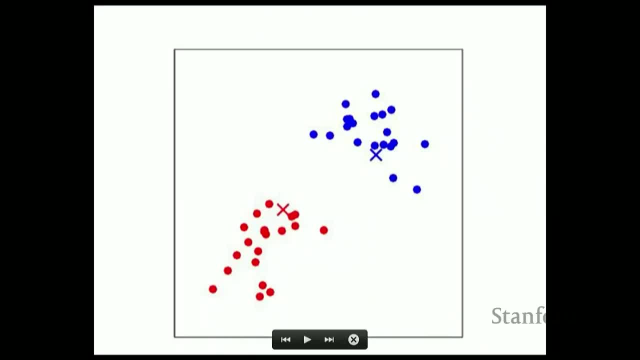 So what happened? Uh, let me go back one slide just to see the difference. So these two points, which previously belonged to the- the old blue centroid, now got mapped to the new, uh, uh, to the red one. And then we reevaluate the centroids again. 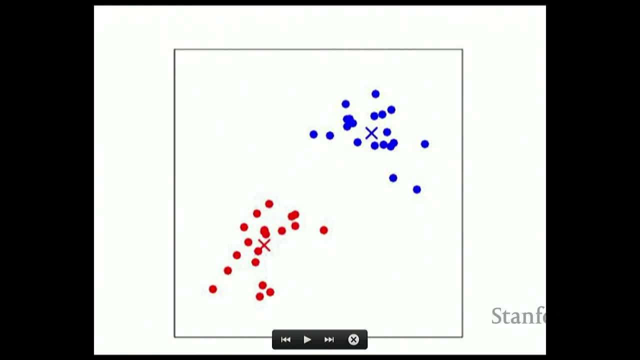 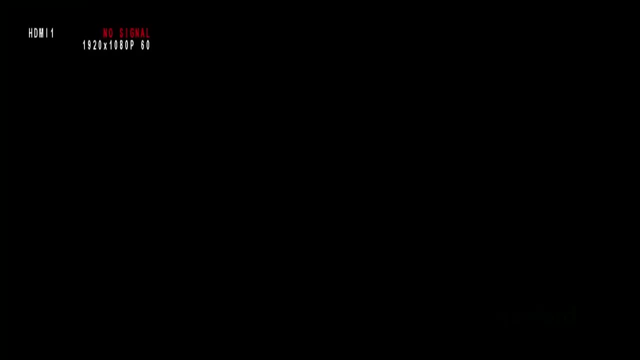 and the centroids will now move to the center right, And once we reach here in the next iteration, I actually moved a slide. you know, nothing changes and we declare that the algorithm has converged. right, It's a- it's a pretty- pretty simple and straightforward algorithm. 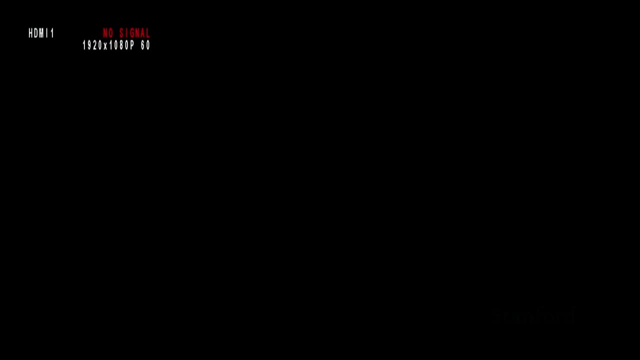 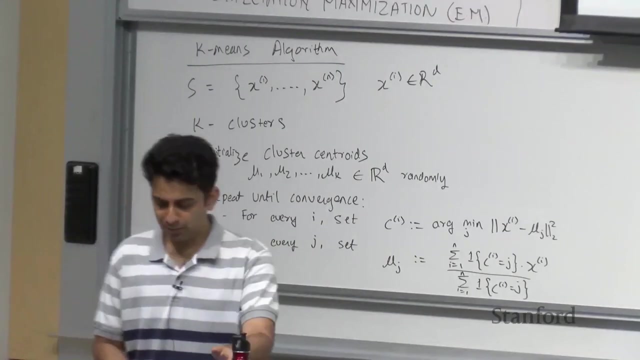 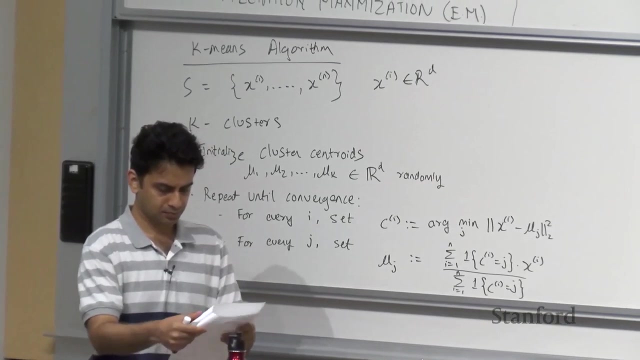 And now the- the uh, a few natural questions to ask. is you know, will this algorithm always converge and will it always give us- uh, give us- the same- same answers all the time? Yeah, So it can be shown that the algorithm does always converge. 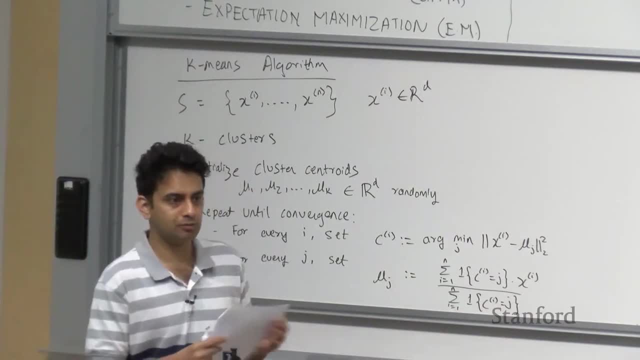 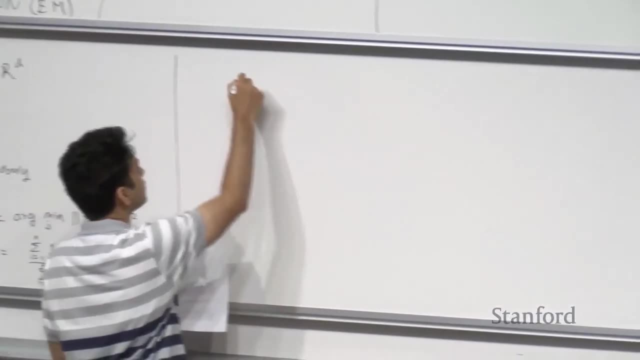 And what we mean by convergence in this algorithm has a special meaning. So if we considered this loss function called J of C comma, mu to be equal to k, Yeah, Yeah, Okay, Okay, Yeah, Okay, Yeah, So amazing. 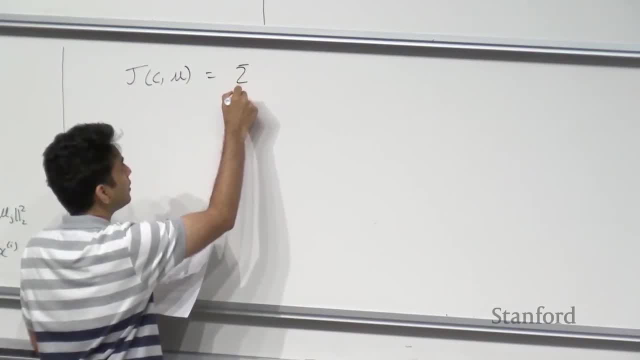 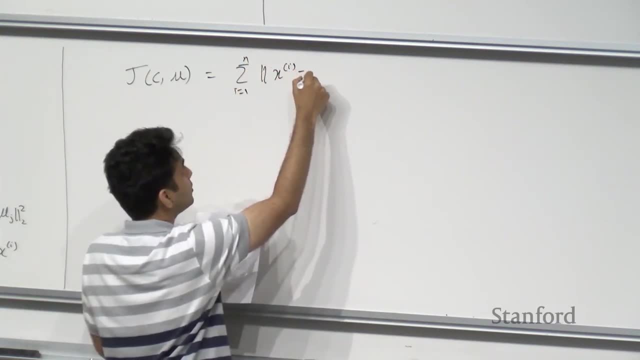 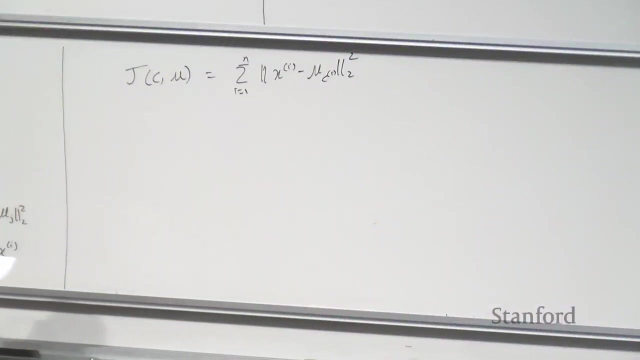 Okay, Okay, Right, Yeah, i equals 1 through n xi minus mu ci squared, And this is also called the distortion function, And the k-means algorithm is basically an algorithm to minimizing this particular loss of the distortion function in the form of coordinate descent. 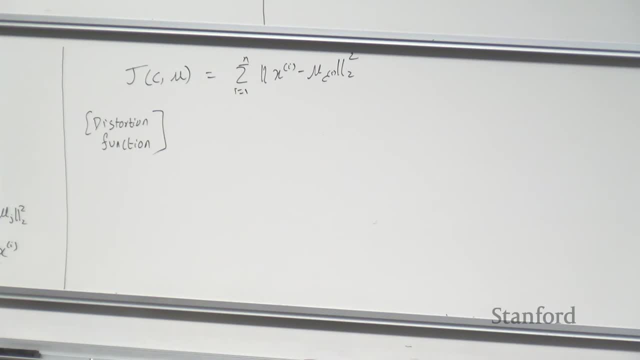 So what's coordinate descent? Coordinate descent? you can think of coordinate descent as a variant of gradient descent, where what we are doing is, at each step, instead of minimizing the loss with respect to all the input variables, we only minimize the loss with respect to a few variables by holding the others fixed right. 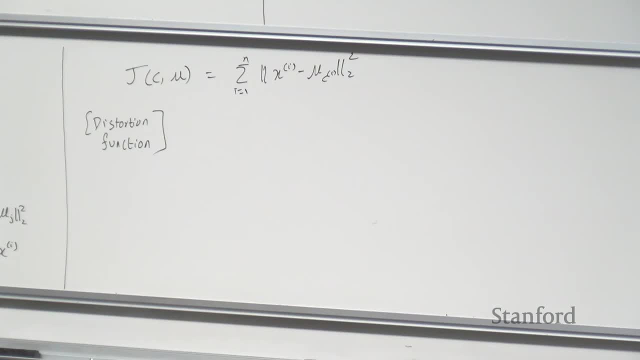 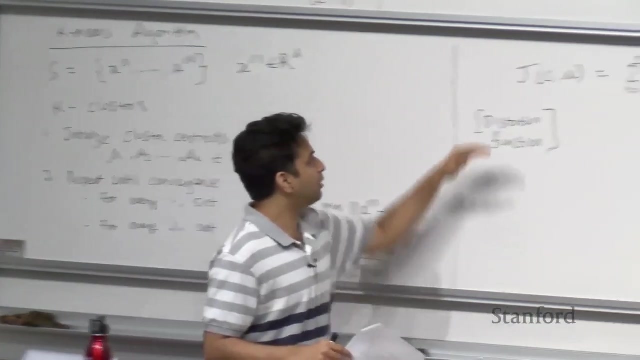 So the- the uh. step number 1 corresponds to minimizing the distortion function by holding mu fixed and optimizing c where- where we calculate mu c's. And step number 2 corresponds to then minimizing j, again by holding the c's fixed. 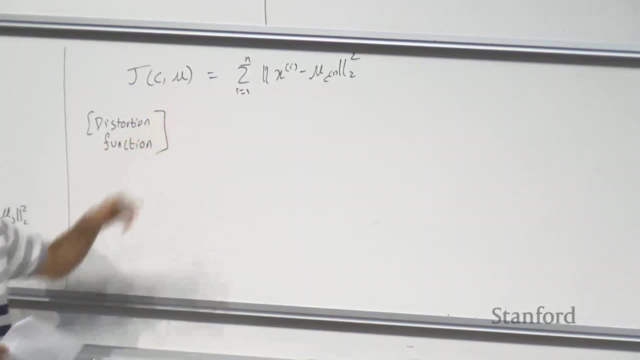 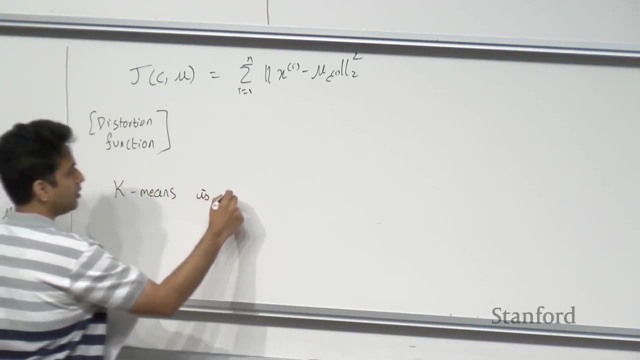 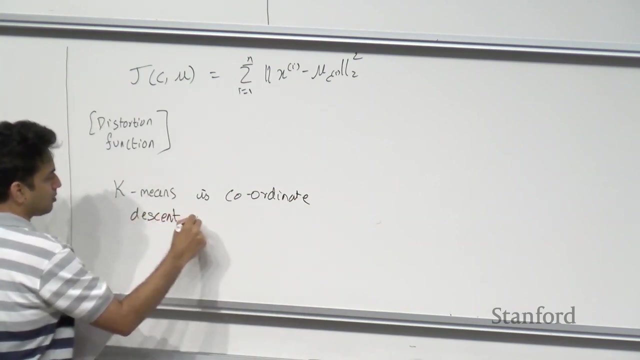 and optimizing it with respect to mu right. So k-means is coordinate descent of the distortion function j, where in- in one step we optimize it with respect to c and the other step, with the- we optimize it with respect to mu. 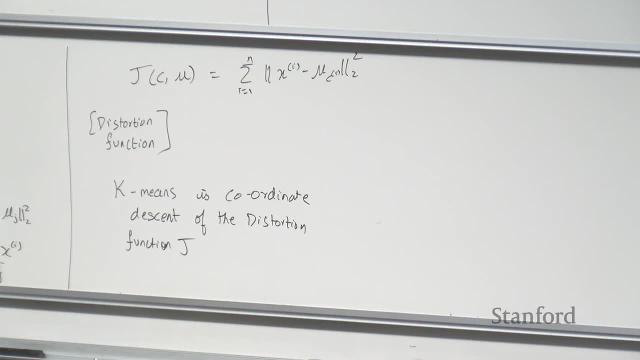 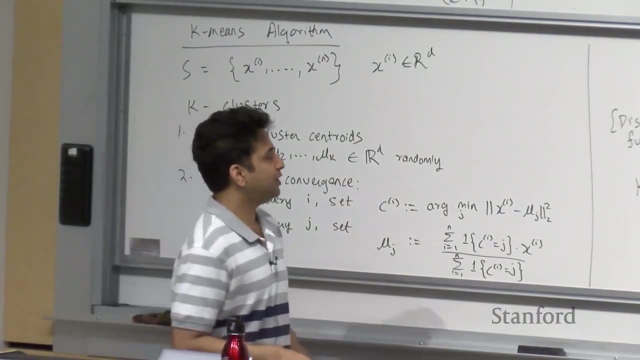 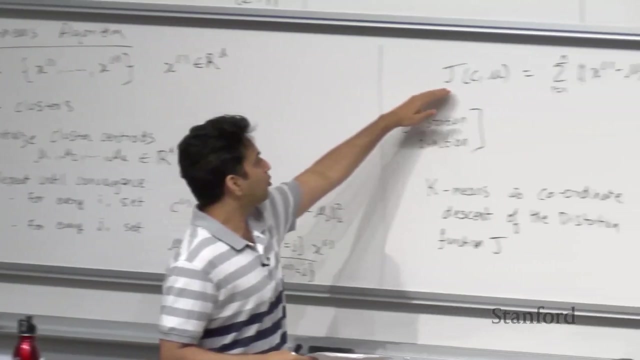 and the result of the optimization results in these- in these uh- closed form rules for recalculating the c's, and- and mu's. And we say that k-means algorithm converges in the sense that eventually we are going to reach some kind of a local minima of this. j function right. 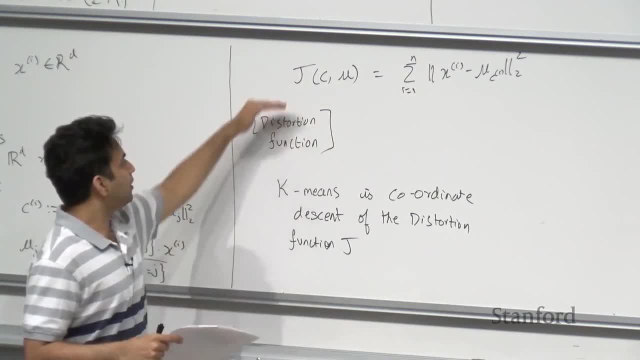 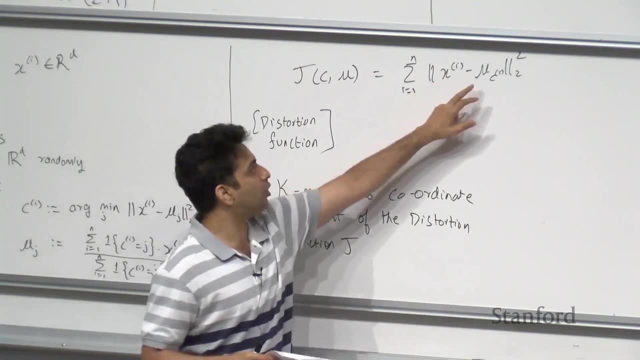 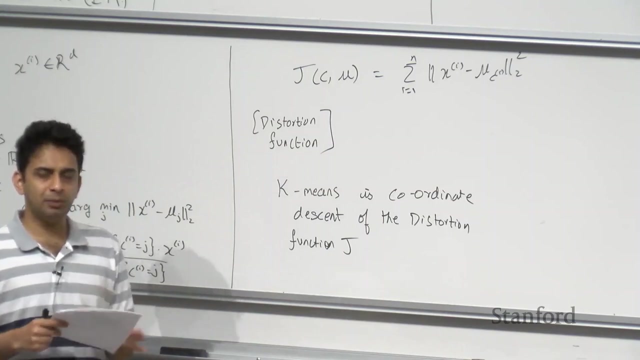 It may so happen that, uh, we may have minimized j, but we may end up toggling between two sets of mu- two sets of mu's and c's alternating, uh, uh, once we reach a local minima, though that happens extremely rarely in practice. 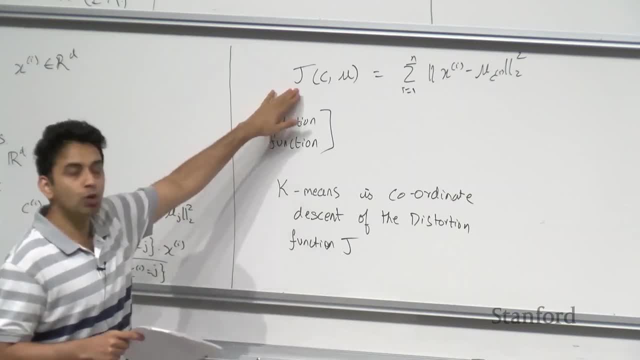 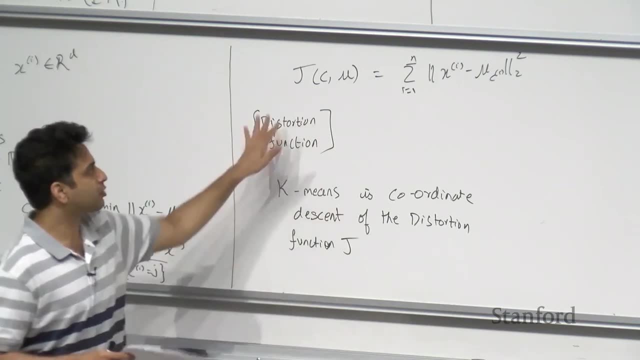 But we will eventually reach a state where j is no longer minimized further. We're gonna flatten out in j and most of the times, pretty much all the time- in practice that's gonna result in some kind of uh, mu and c that does not change anymore. 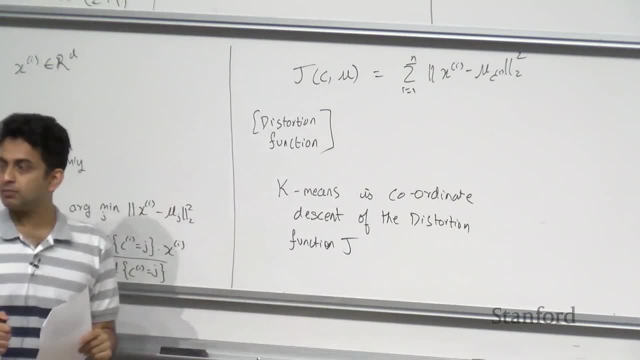 This j is non-convex, which means the- the mu's and the c's that we end up in can change from run to run. If you start with a different initialization, you may end up with a different set of mu's and c's right. 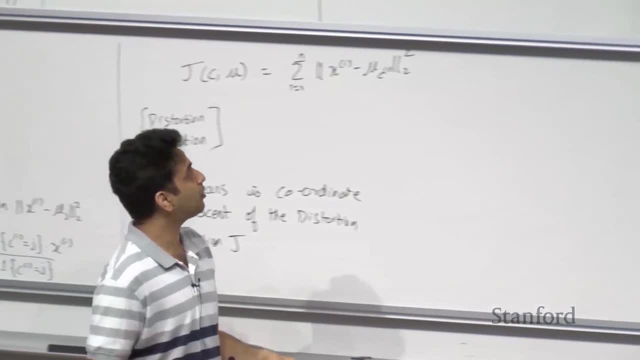 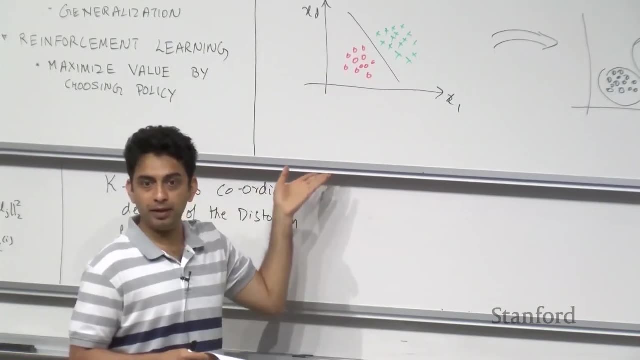 Which- which kind of uh ties back to a question that was asked before You know? uh, why do we, you know, ever need to use the label identities- um and- and not just perform, uh, perform clustering. 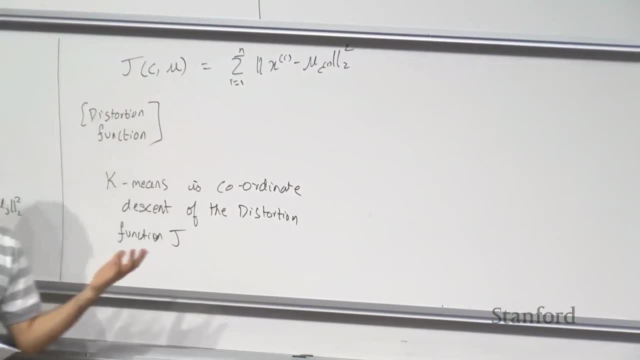 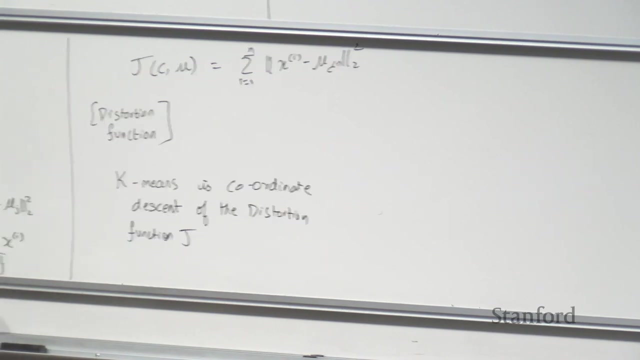 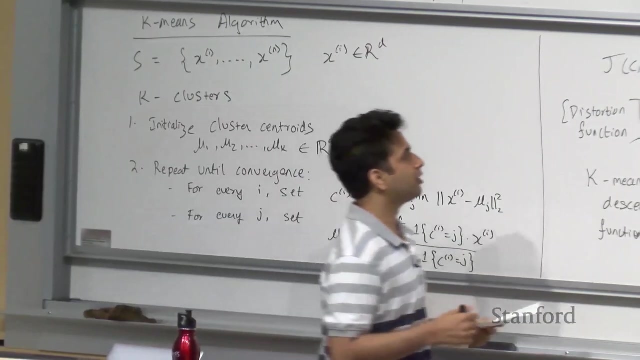 And the answer is- is that this is basically a non-convex pro- problem and we can end up with different- uh, different cluster identities depending on the initialization. Any questions on this? Yes question. So the question is by looking at a function. 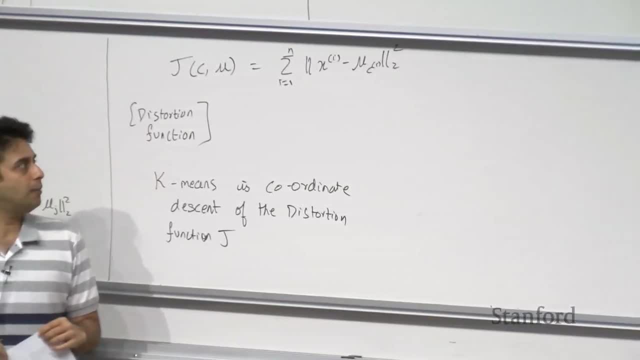 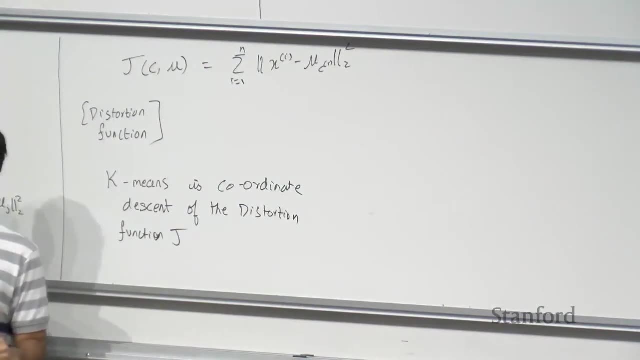 how do we determine whether it is uh convex or not? Uh, in general, it is um. the answer is not always straightforward, So it is easy to show that something is convex by showing it, as you know, a composition of convex sub-functions, right? 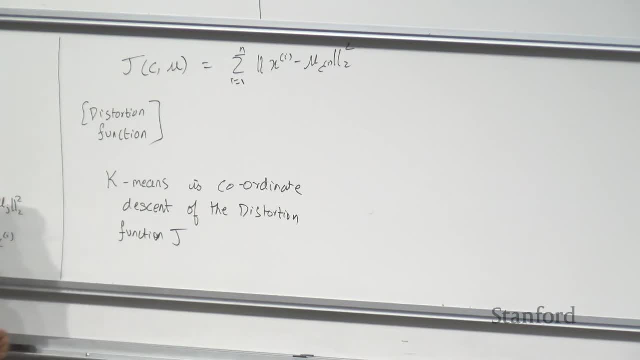 Uh, however, showing something is not convex. uh, is not always that straightforward. Uh, something could uh, which may not appear to be convex at first, can sometimes, with some kind of re-parameterization, may end up being convex, et cetera. 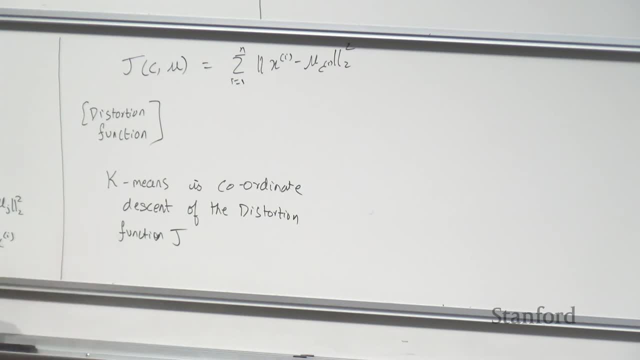 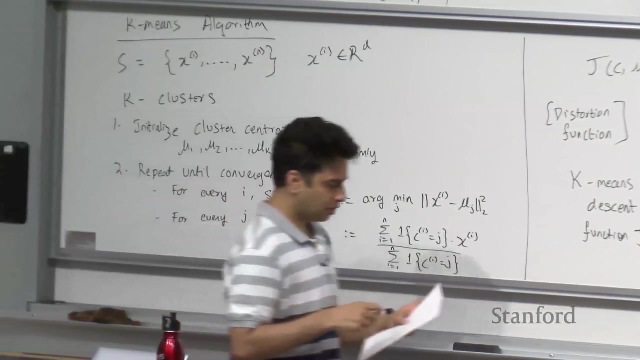 Um, in this case it happens to be non-convex. Any questions on this? Cool Uh. so, given this clustering pro- uh clustering approach that we've seen, let's move on to something that is slightly different and also somewhat related. 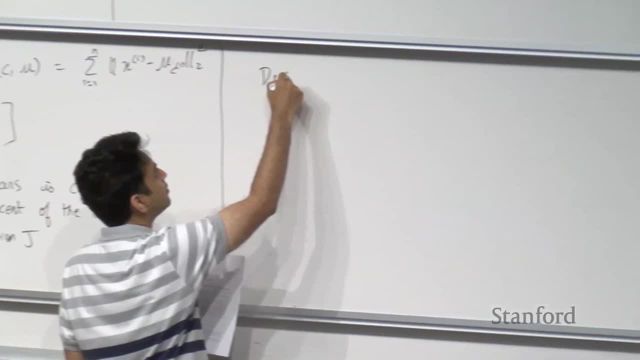 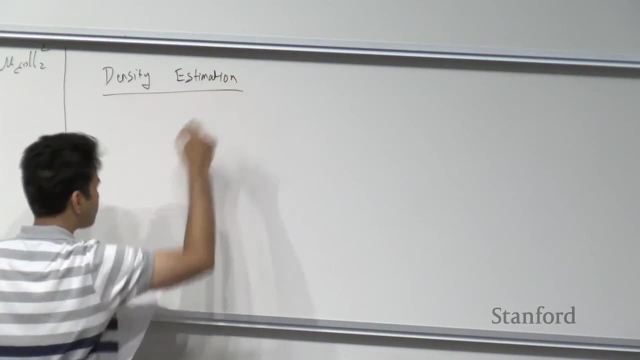 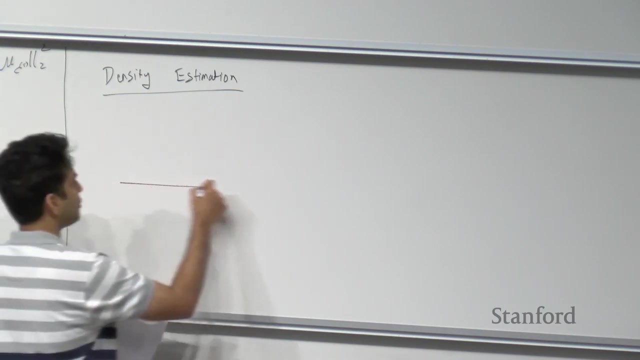 It is the problem of density estimation. So density estimation generally refers to the problem where we are given some number of data points. We're given some number of data points, and this is in R, you know. think of it as the x-axis. 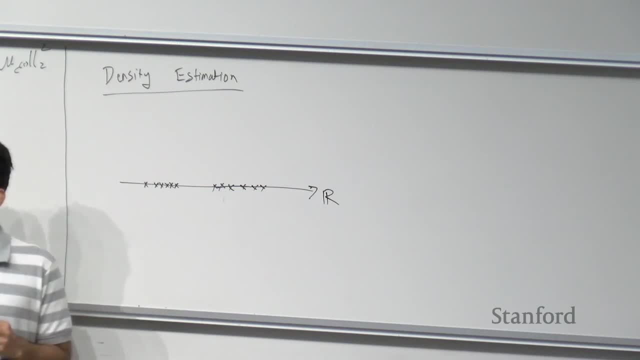 And these points are residing in the continuous space, right, And the goal is to now, uh, we assume that these points are sampled from some kind of a probability distribution And because this, uh, this- these points are- are- are coming on a- on a- on a continuous distribution, 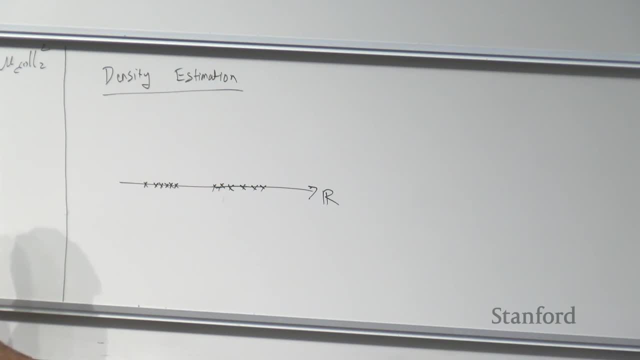 the corresponding probability distribution has some kind of a density right. It's not a probability mass function, but it's a probability density function, right. And given these points- points that look like this, the question is: you know what is the density function from which these points were sampled? 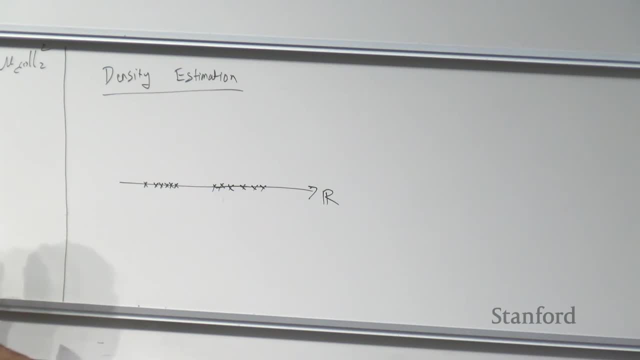 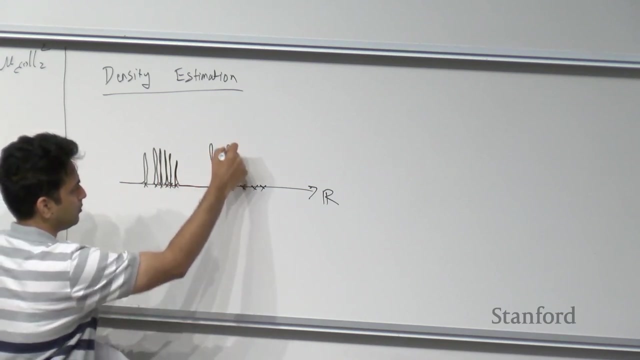 And in general, it's a very hard problem because, uh, if you want to fit this data really, really well, then the best possible fit would be a density that looks like this, where it has, you know, like a Dirac delta function over every data point. you know- you know. 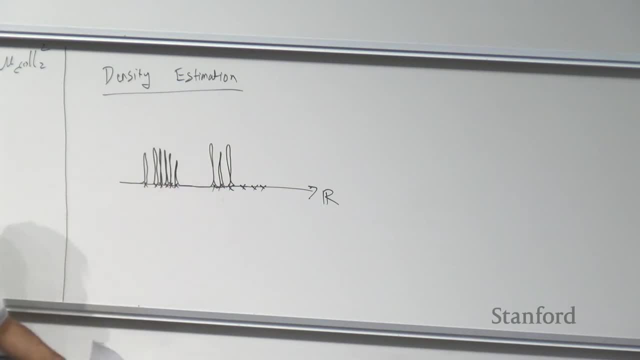 a peak that you know, that- that's really really peaked over each data point And you can, you know, uh, this- this- this, uh, this is a valid- valid density, but at the same time, 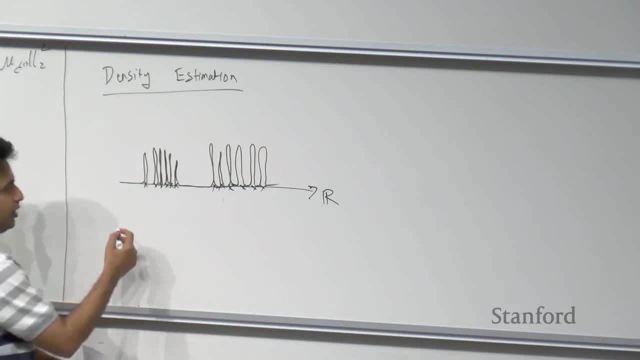 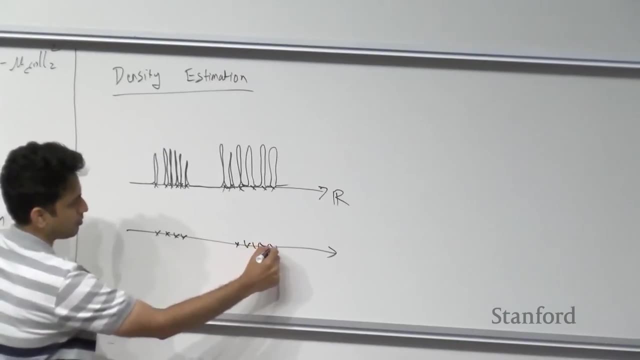 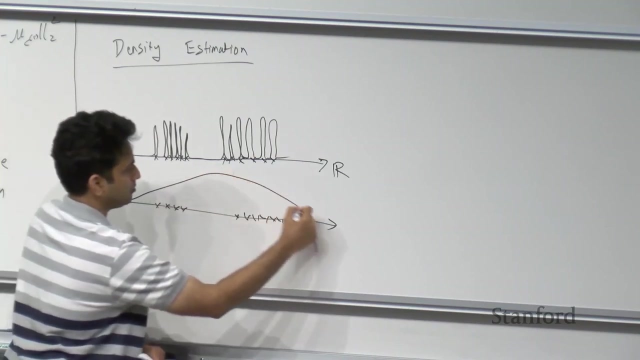 it doesn't feel natural. right Another- another, equally valid density would be: you know, something that looks like this right, And now this is also a valid density, right From which it could have been sampled, because there's nothing to the left. 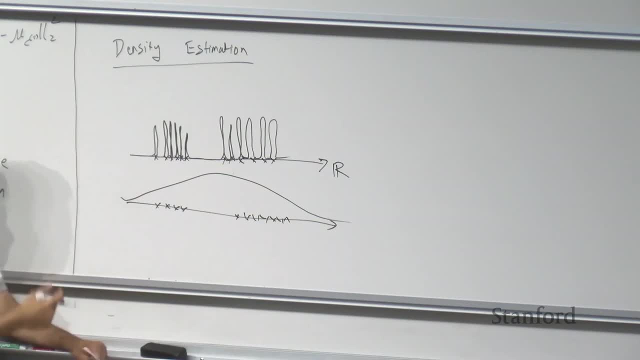 nothing to the right and there's some values over here. you know that- there's something uh that- where- where there's some data. so you might- you might have some kind of a density And also this is also a valid- right. 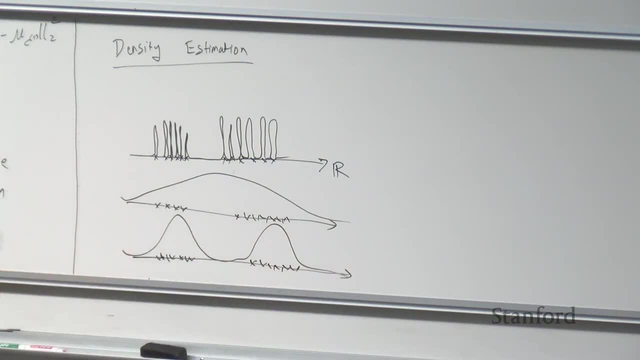 So all these are different possible answers for what the underlying density uh is, from which these points are- are calculated And kind of the- the fundamental problem of density estimation is that the density function has to be a continuous function In the case if- if these were you know. 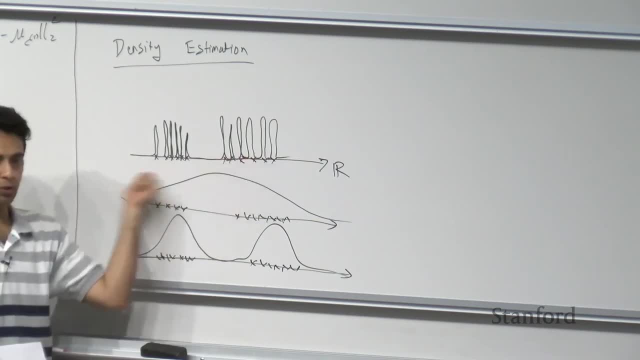 um, the outcomes of coin tosses- where the- the support was discrete, then maximum likelihood was- was pretty straightforward. You could, you know, treat them as a multinomial and just count them. But whereas in density estimation we need to come up with this smooth function over discrete observations, right? 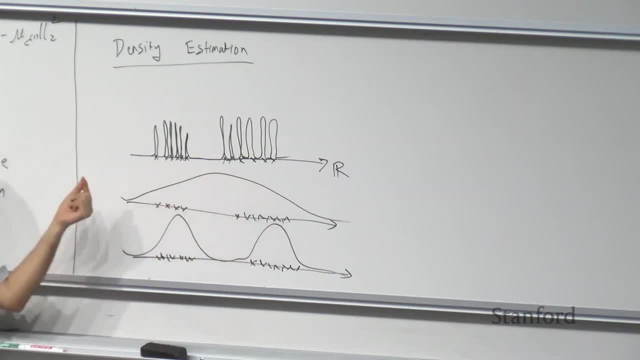 I- I say discrete observations because we have a fixed number of observations and we want to come up with a- with a- with a- a-, a smooth estimate. So a common approach in uh density estimation is to use this model called the Gaussian mixture model. 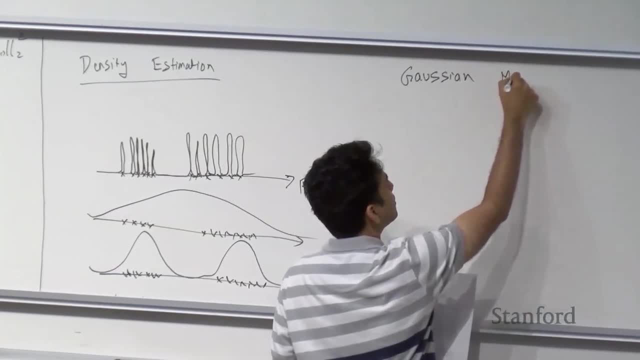 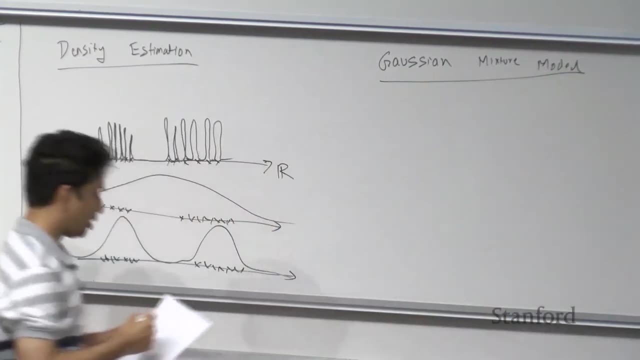 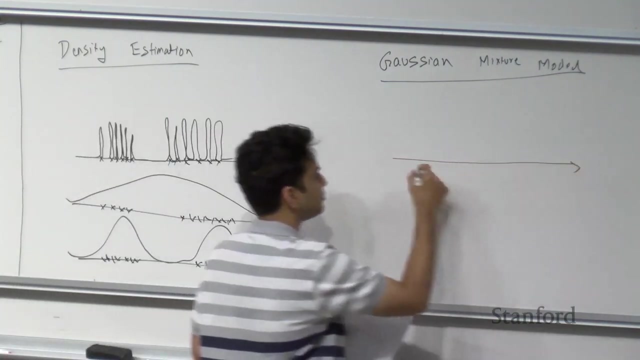 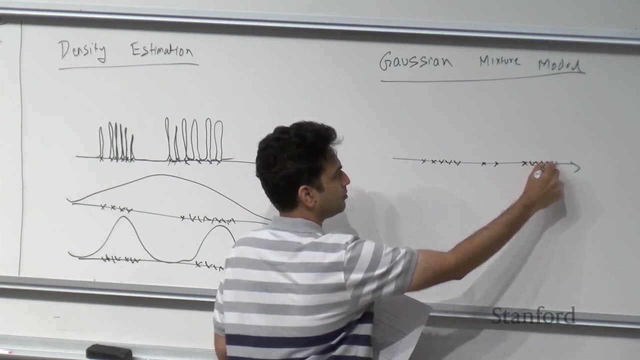 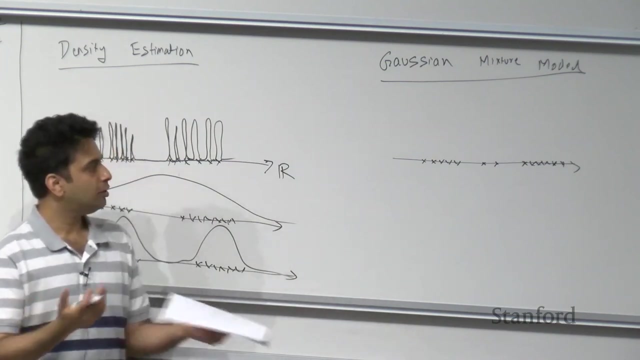 or it's also called the mixture of Gaussians right, The Gaussian mixture model, where, given some- given some um uh- data points that look like this right, We wanna- we make this hypothesis that there are these two underlying different- 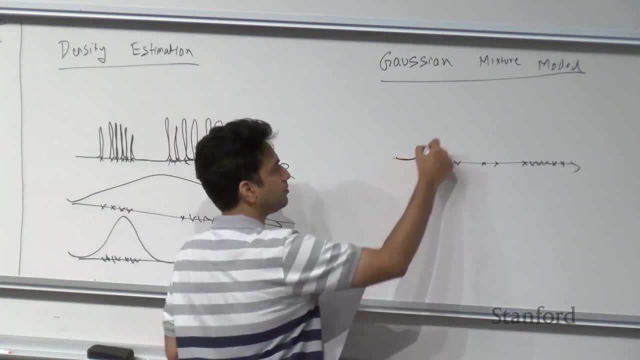 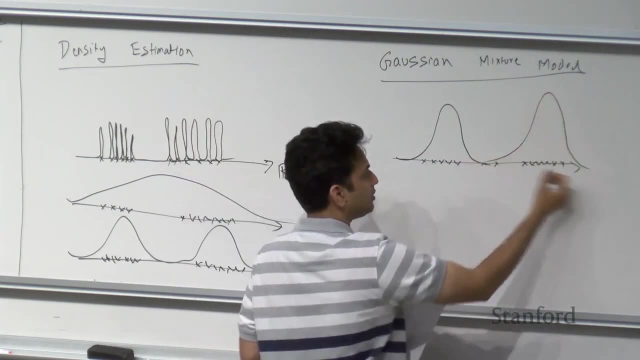 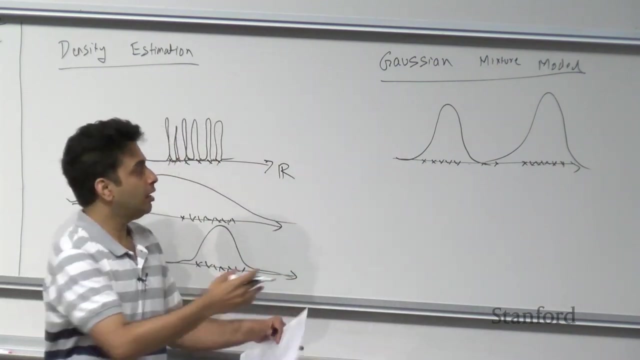 two different, distinct Gaussian distributions, And there is one Gaussian distribution from which these were sampled, another Gaussian distribution from which these were sampled, and together you can take the sum of these two Gaussians- uh uh- Gaussian probability distributions and say 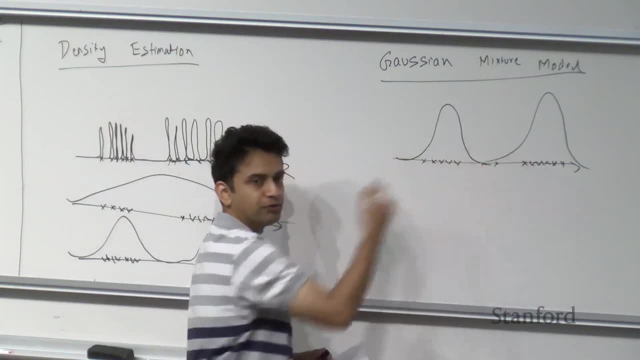 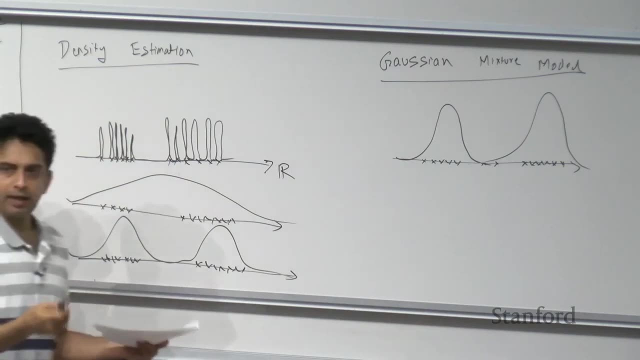 this entire dataset is sampled from these two different Gaussian, um, uh, these two mixture of these two Gaussians, right, And the choice of k is something again uh is- is uh, uh, similar to, you know, in k-means it- it is something that we choose by- by. 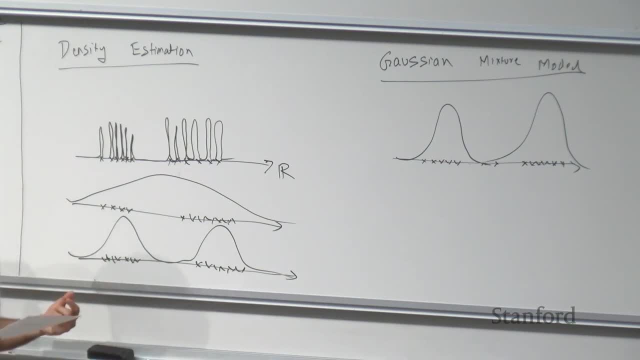 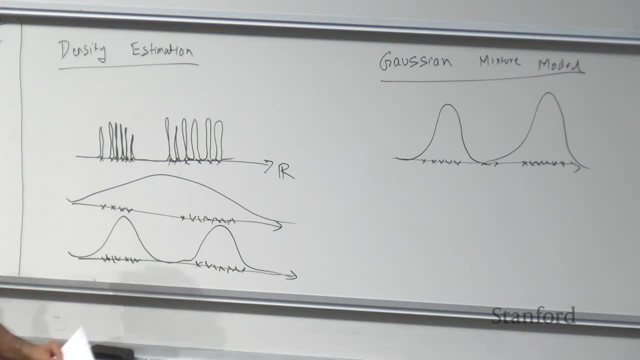 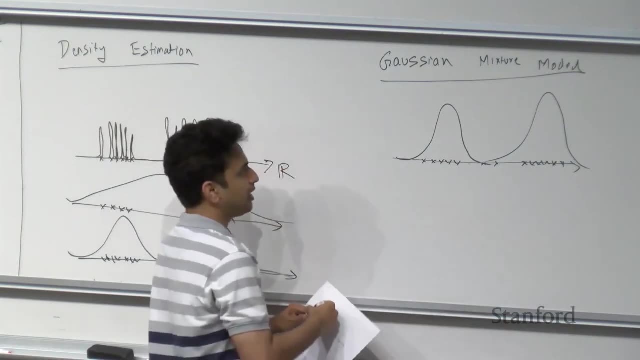 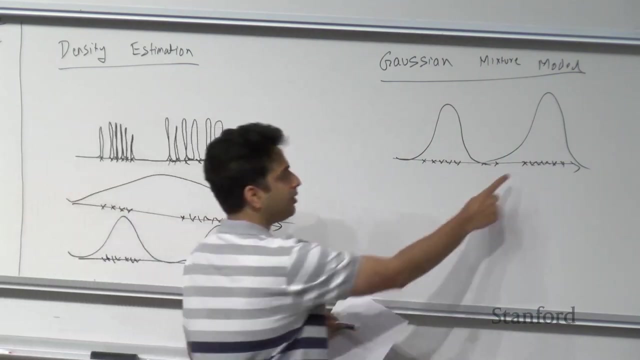 fit the number of k And the uh. the problem we have now is to- is to uh. given this dataset estimate the two Gaussians from which the dataset might have come right, We are not told what the um identity of the two uh Gaussians are. 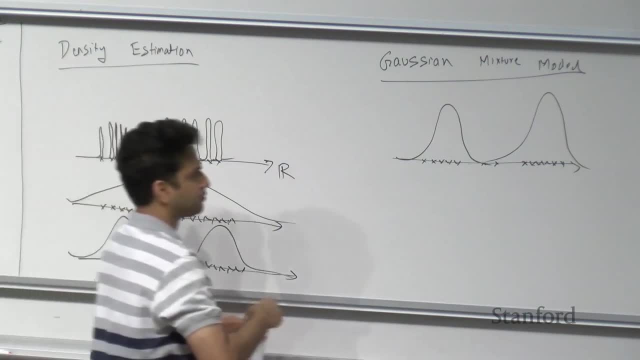 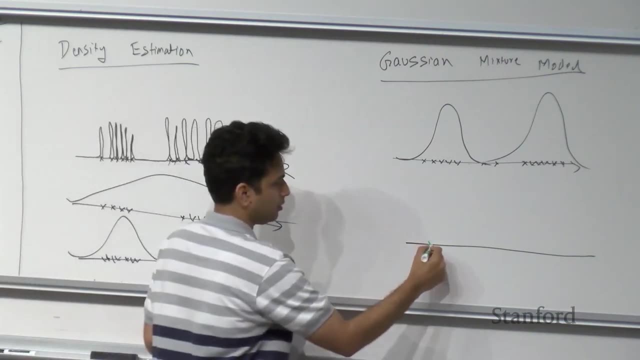 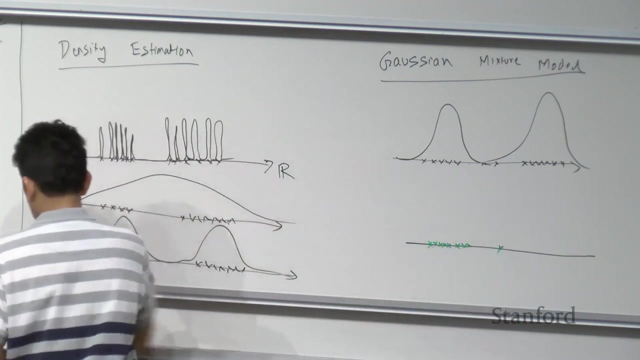 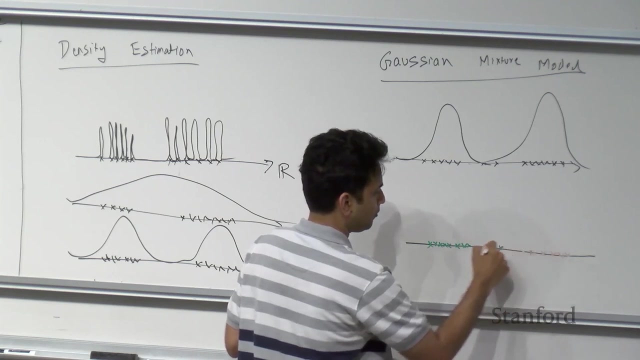 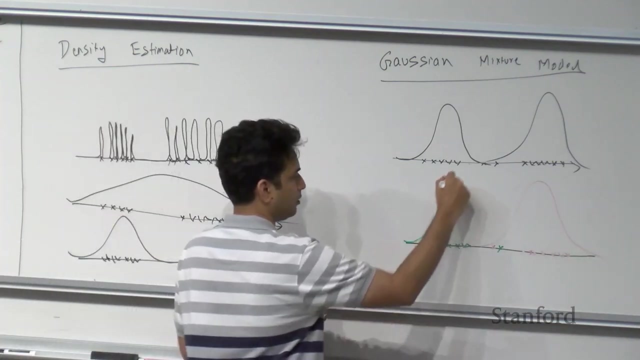 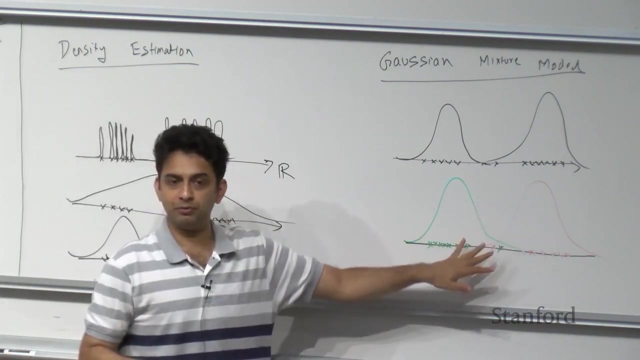 If this were to be a supervised setting, then we would have, you know, they would come with some kind of an identity And we could have fit one Gaussian here and the other here, right. And this is exactly what we did in-. do any of you remember? 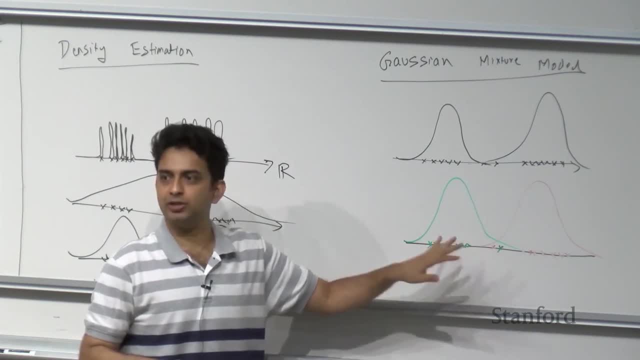 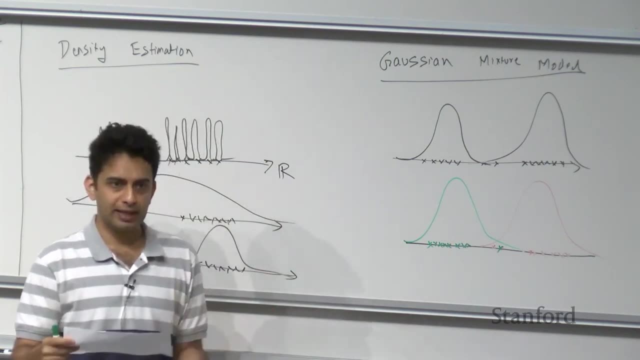 where we did something like this: GDA, GDA, exactly. So in GDA, we were- we were told that x's come from our- our sample from Gaussians. and there are these two different classes, class 1 and class 2, right. 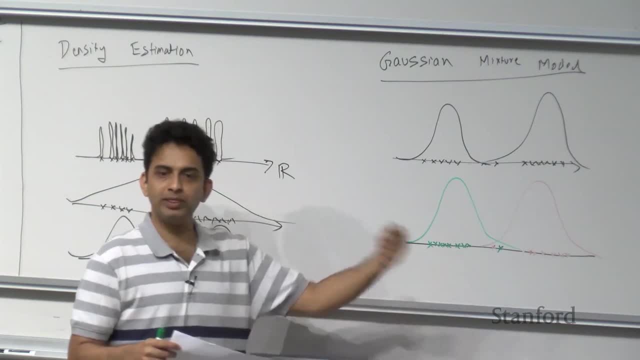 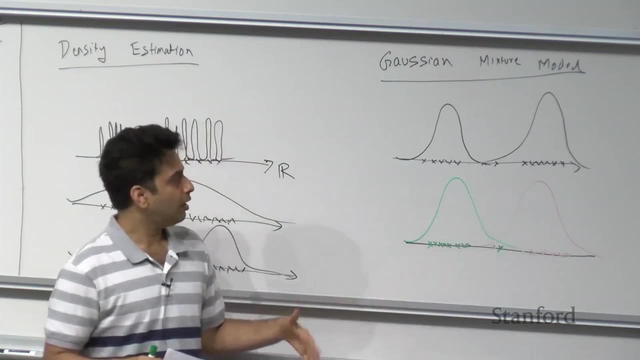 And our goal was to take these x's, along with their cluster identities, the corresponding y's, and estimate the mus and sigmas for the two classes. right Now, in Gaussian mixture model, we are essentially generalizing GDA in a way. 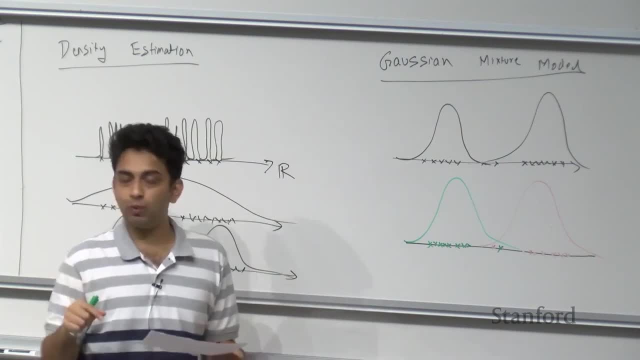 where we are not given what the y labels are, we are just given the x's and we also relax the constraint which we had in GDA that the covariance had to be the same. In this case, the covariance can be different. 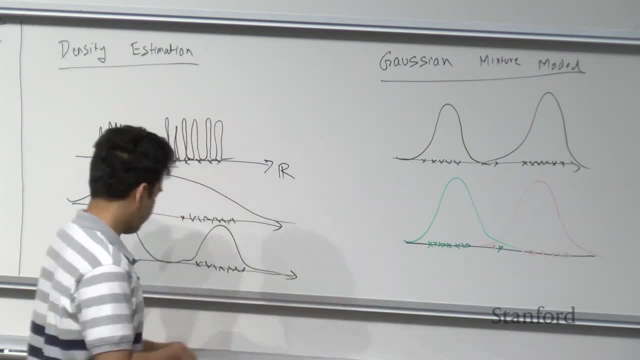 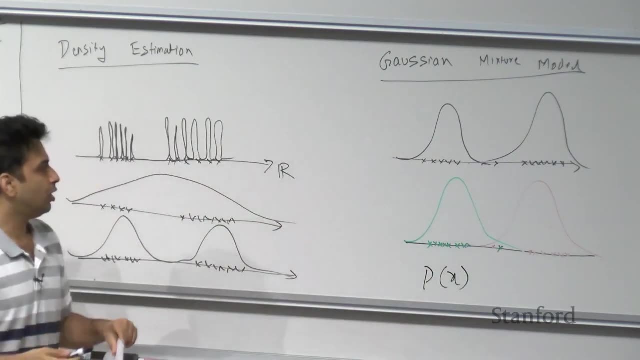 And our goal is to now come up with some kind of density p of x that allows us to uh assign probability density to the observed values. right? So that's- that's the uh, uh, uh, that's the setting in which 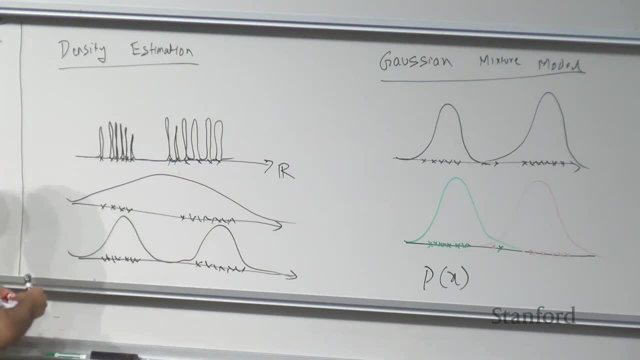 uh, the Gaussian mixture model comes into picture And the reason why, um, why we are interested to even calculate this p of x. there are many reasons why, uh, calculating p of x could be interesting, So here's one example. 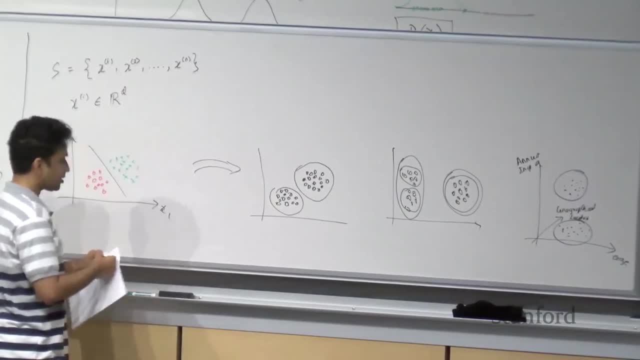 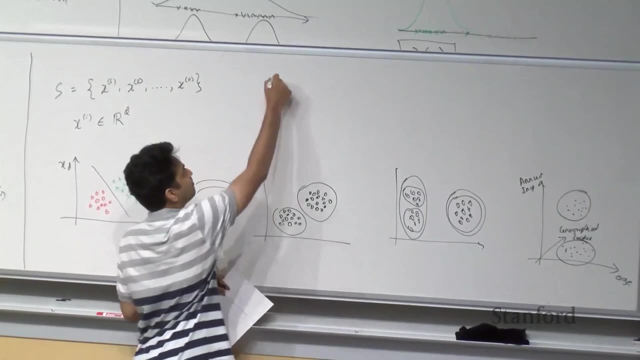 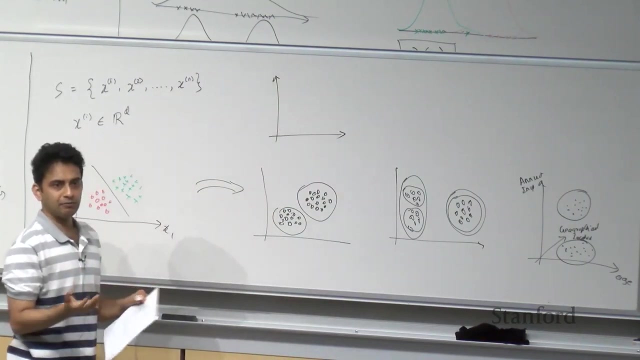 So here's a- a completely made up example. Supposing, uh, supposing you are, um an aircraft manufacturer, where, let's assume, the, the uh, the parts that we manufacture, have two kind of attributes. Um, let's say, you know, 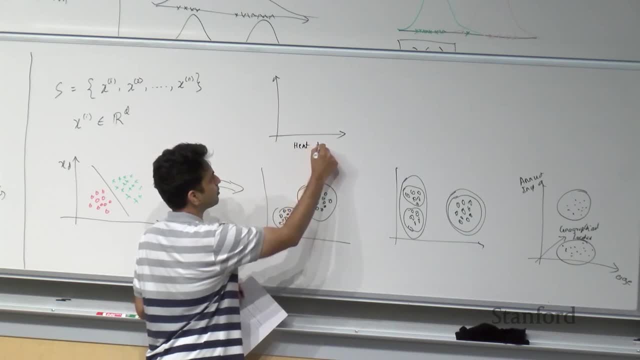 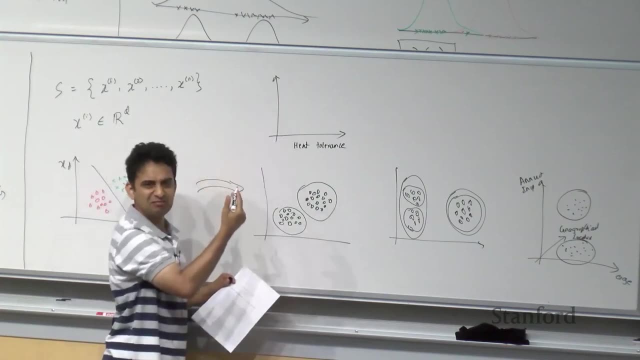 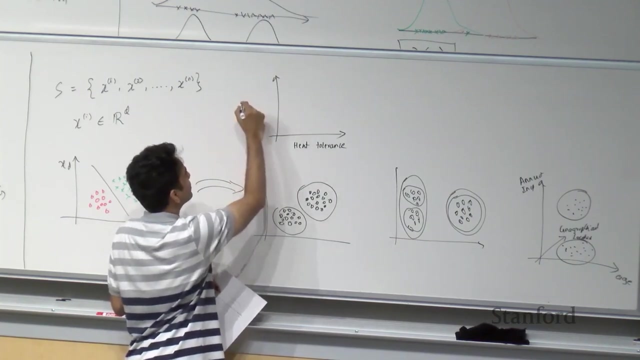 um heat tolerance, And if any of you are, you know, or in aeronautics, what- what might be another, You know? uh, let's say let's- let's call it um, um, um, um, um heat tolerance. and 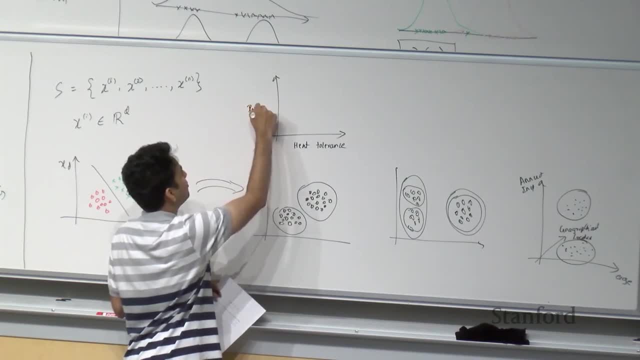 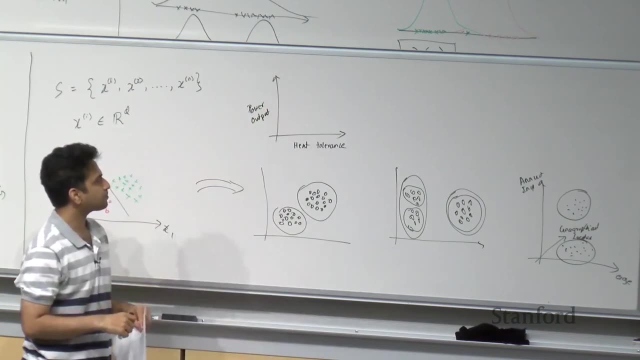 and um, whatever power output, whatever that means. So let's assume there are- there are- there are these two kind of um, um attributes that are- that are um there for, uh, some part that we manufacture. 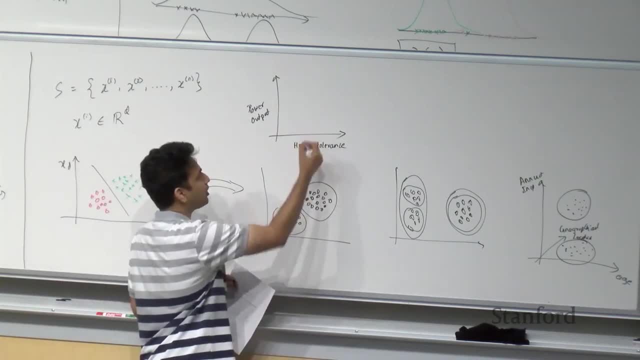 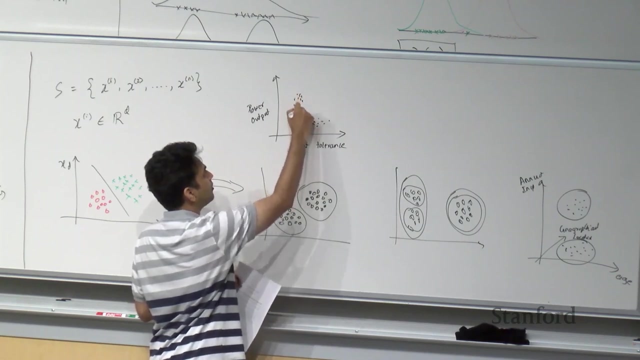 And in general what we observe that, uh, if you were to plot the, uh, the-, the every manufactured part as a point here, you might observe that most of the normal parts fall along some kind of uh uh a distribution like this: 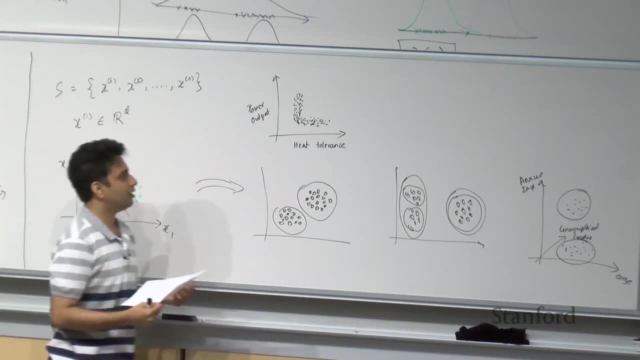 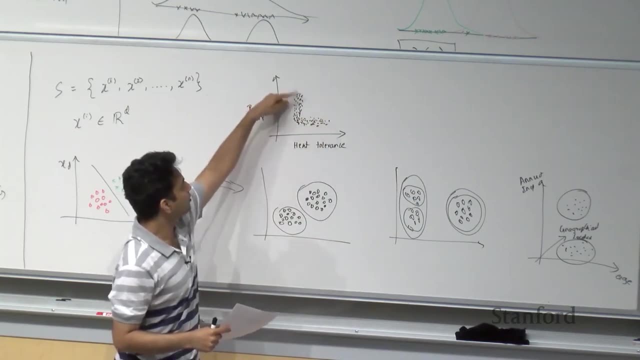 Maybe there are, you know, two different kinds of uh subtypes of parts, maybe based on the material or something, where some of them uh uh fall in distribution. some of them fall in this kind of a distribution, you know. 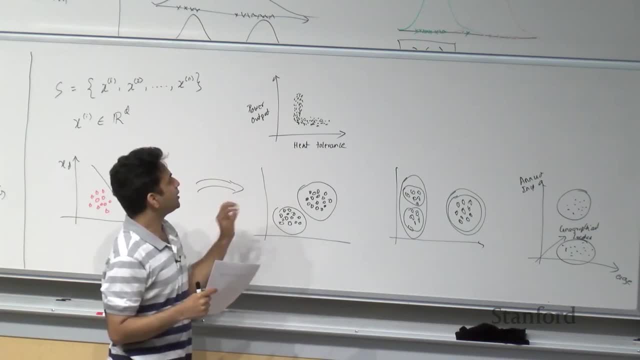 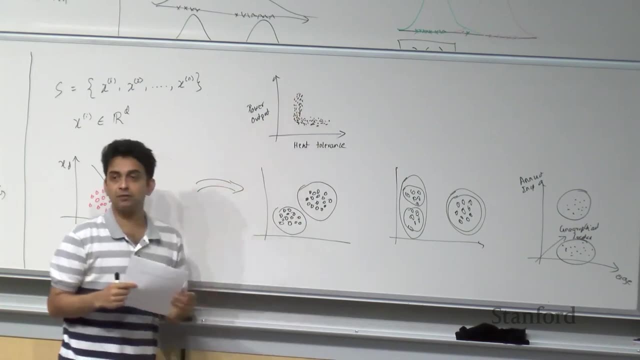 uh, uh, whatever be the reason, But you know, generally- let's assume that you know- normal looking parts fall in this kind of uh, um, belong to this kind of a probability distribution. Now suppose we want to- we want to. 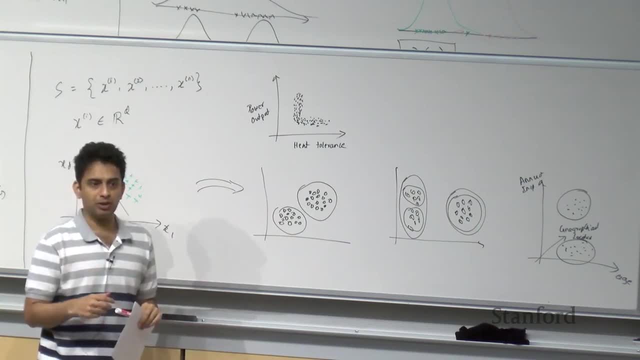 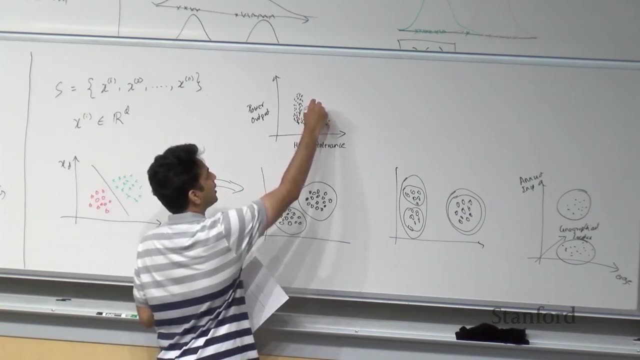 uh, uh. have some kind of an automated anomaly detection where we want to detect that you know, some part is- is- is faulty for some reason, right? For example, a part that may- that has this attribute, right? 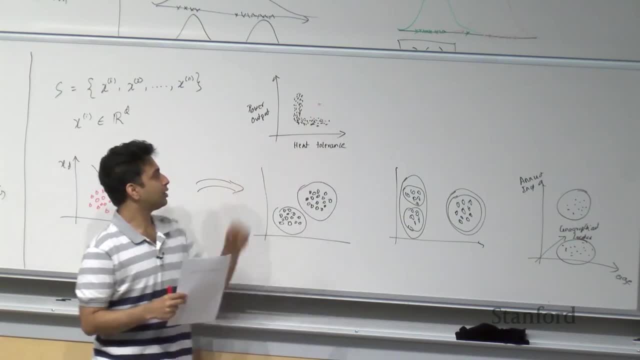 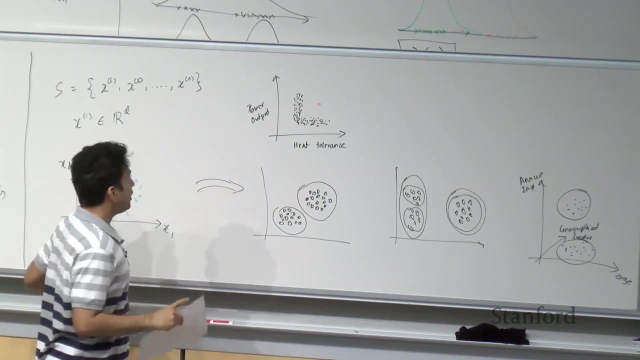 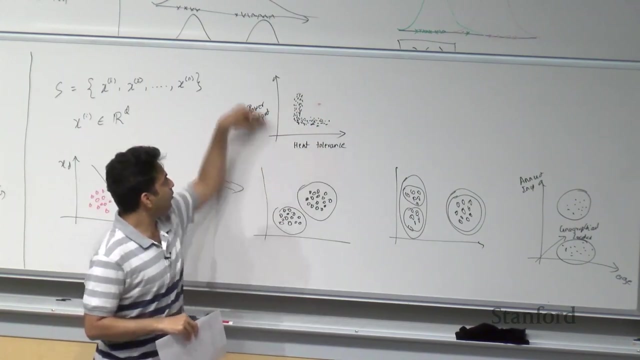 We want to identify that this point over here is- is uh is faulty, and at first it- it might appear, you know, uh, even though this looks visually away from this kind of a heat map, if you were to look at any one of 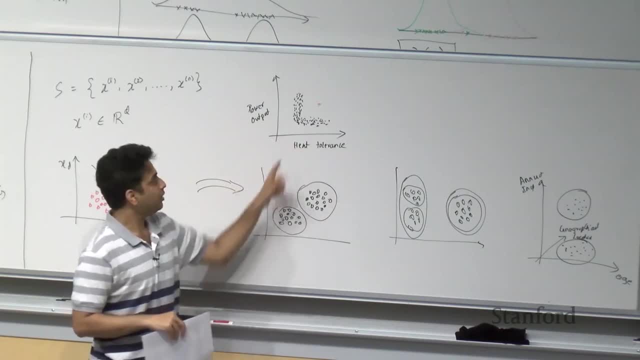 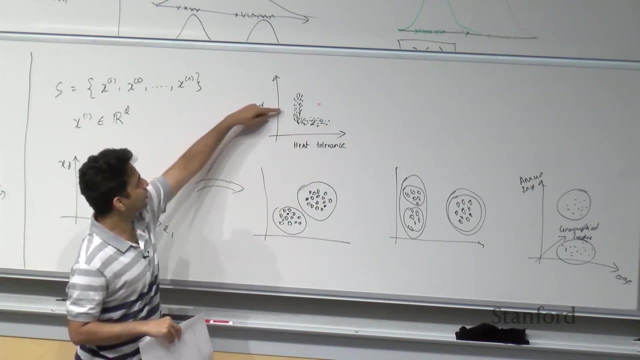 the axes alone, it looks pretty normal right. Just from the heat tolerance point of view it's kind of- you know, in the- uh uh, close to the mean, and if you just look at the power output it's also kind of near the mean. 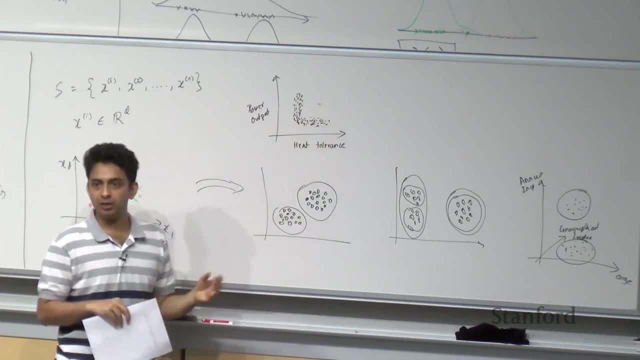 but it's this combination that makes it kind of, you know, an anomalous example, right And the- the way, uh, uh, this kind of an anomaly detection is, um- can be carried out in practice is to construct. 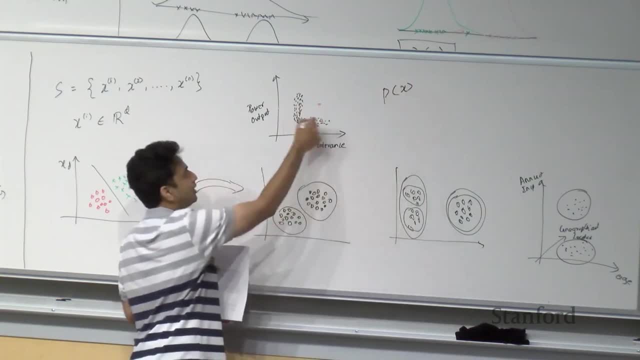 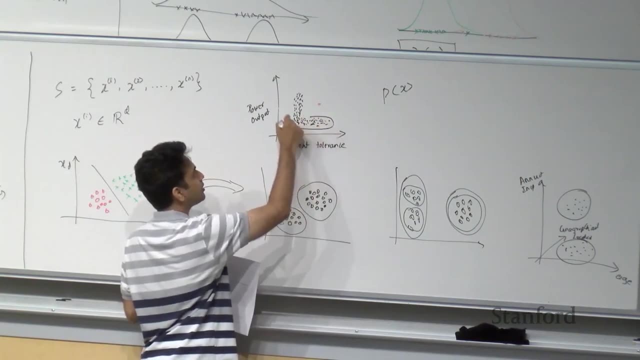 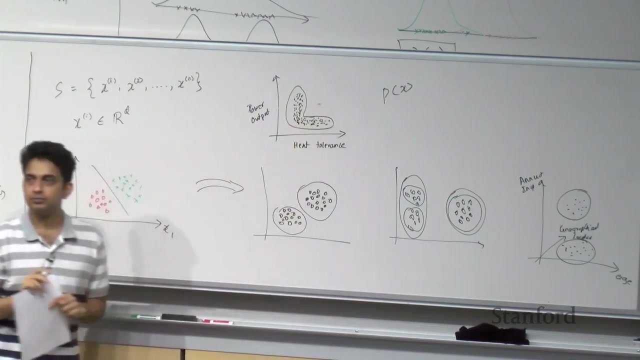 you know, a density estimate, P of x for these points, where the- where this P of x assigns high probability for anything that falls in this region and P of x assigns low probability for anything outside this region. right And a common approach to doing. 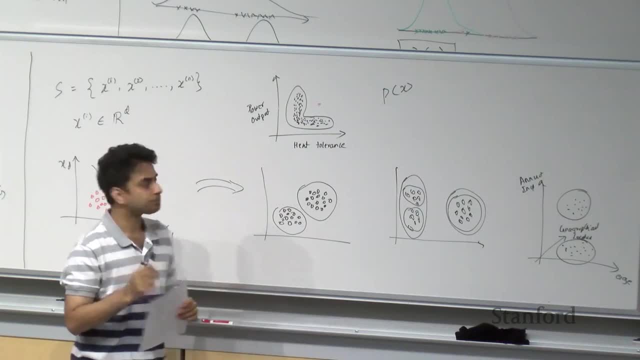 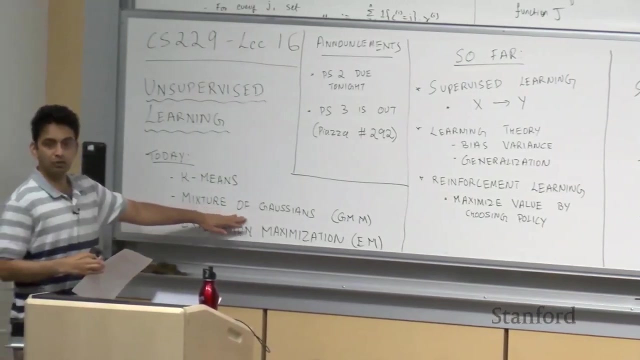 this kind of a density estimation is to use mixture of Gaussians. right, And the way we go about, uh uh, doing mixture of Gaussians is-. so, first, what we're gonna do is to provide you an algorithm to do mixture of Gaussians. 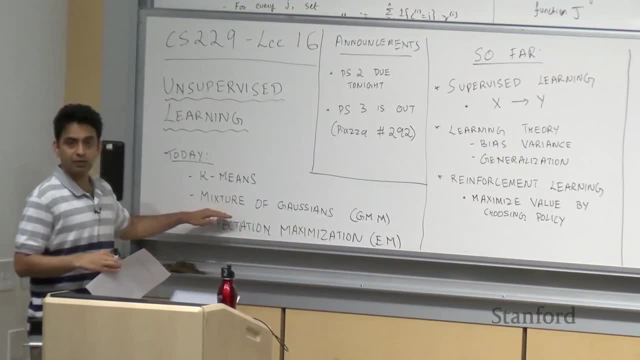 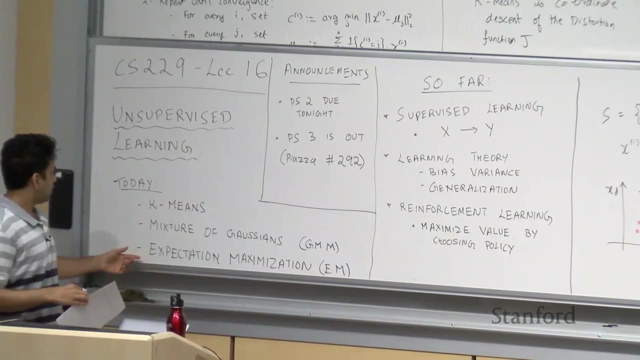 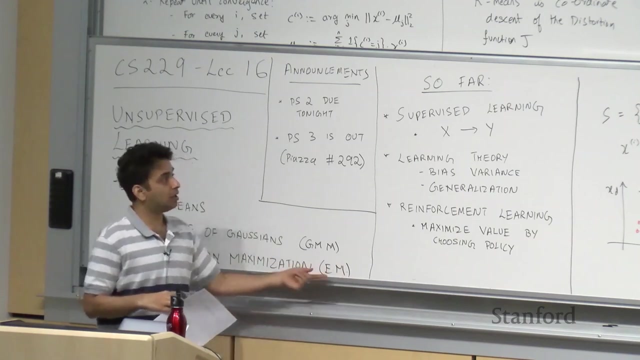 And we're gonna provide, uh, construct this first algorithm based purely on intuition, And then what we're gonna do is describe this general framework called expectation maximization and then re-derive Gaussian mi-, the uh Gaussian mixture model, using this framework. 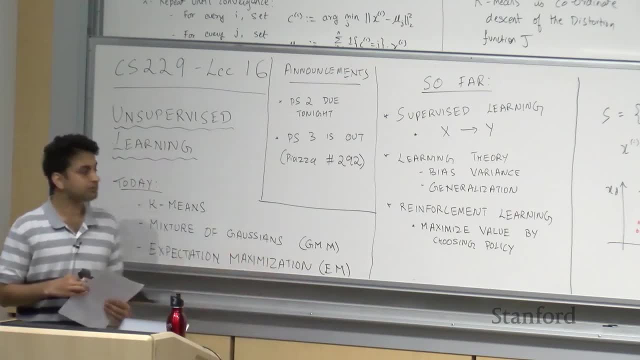 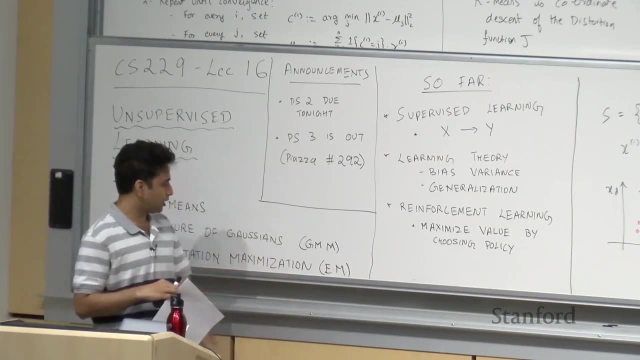 and see that we end up with the same algorithm that we got using intuition. The expectation, uh maximization, that we're gonna see next is a more general framework that works for a broad class of um, of- of of um generative models. 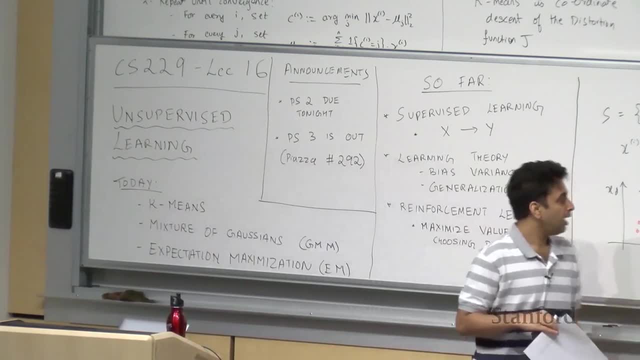 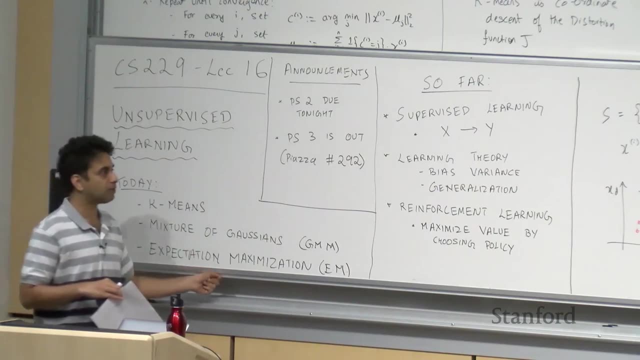 These are examples of generative models, And the uh Gaussian mixture model is just one such- one such model which can be solved through expectation maximization. This question, Uh. so, even given that you know, we know we have to pick Gaussians. 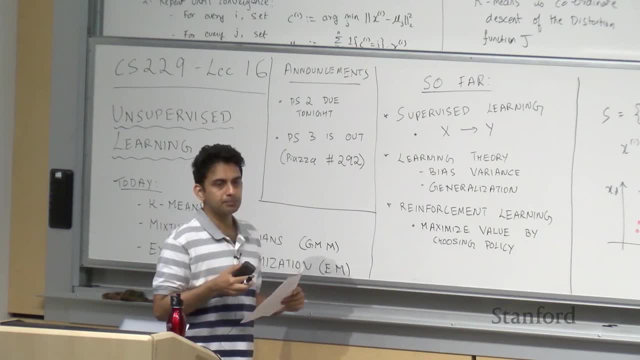 and you said we will typically choose K, like based on, you know, this triangle of the pre-K, and then you can do this, you know, But shouldn't we also like: doesn't someone need to tell us what is the highest? uh? 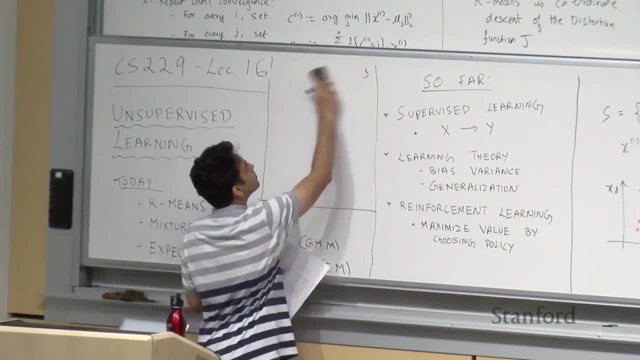 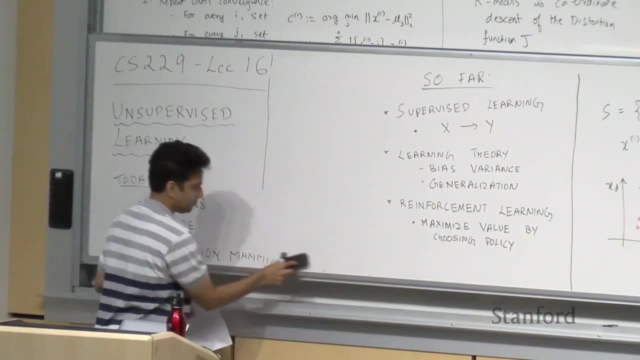 restrict- like what is the upper bound for the frequency that we will tolerate? on the previous figure, The K will fit best as the K- as K approaches the number of data points, right, Yeah, So- So don't we need to be told what the frequency of the previous is? 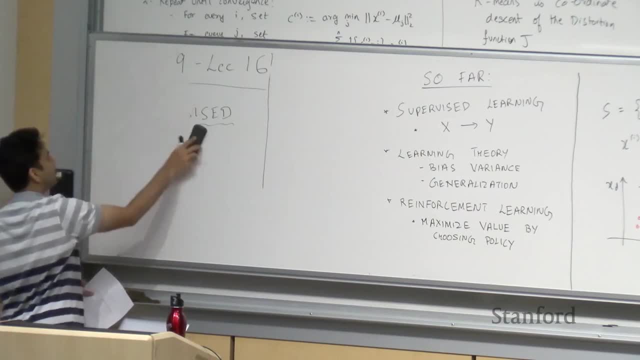 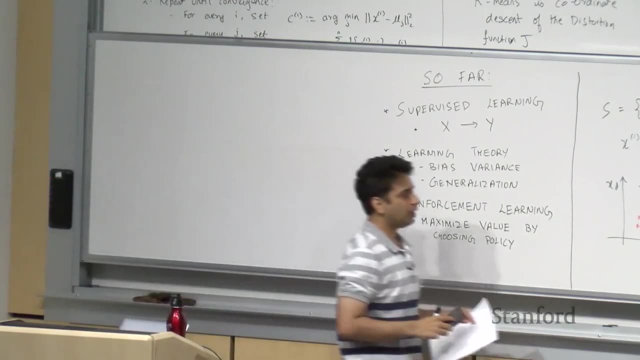 So the- the- the question is, uh, I guess, um, to- to kind of summarize this: how do we find out K And uh? it is true that as we increase the number K, um, we kind of fit the data better and better. 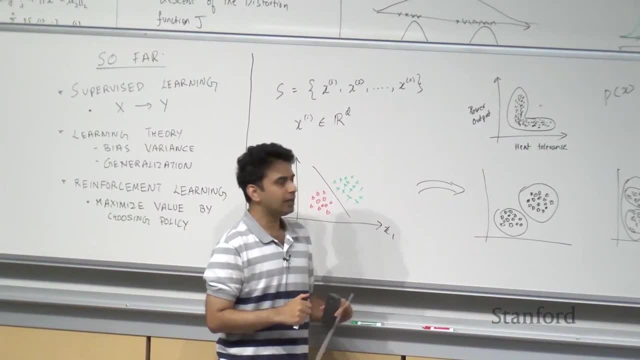 And? um, in order to kind of uh think of what's the best value of K? um, I will leave this as a thought exercise for now and we'll come back to this probably next week. Um, try to see how you. 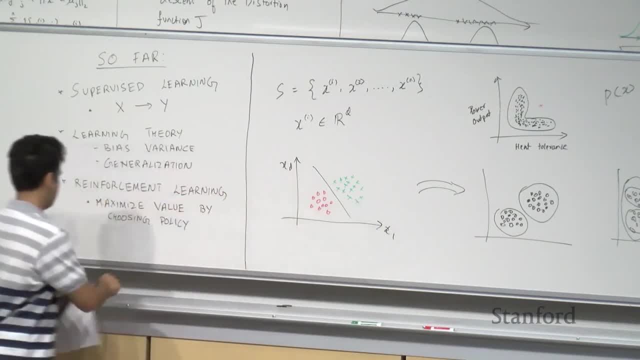 can apply, you know, uh, what we learned in um um in learning theory: bias and variance. you know How- how can you, you know uh, uh, give some thought on how you can apply bias-variance analysis on this kind of a problem, right? 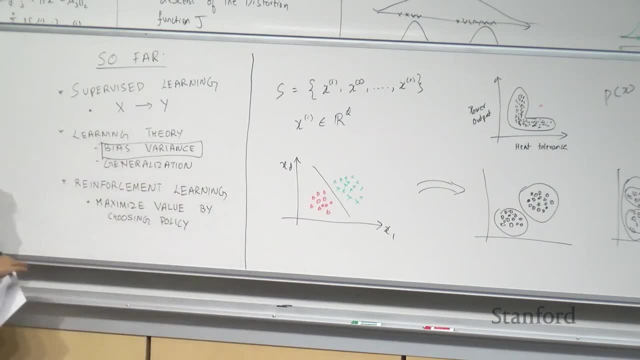 And we- we'll come back to this later. For now, we'll you know, for-, for- for today and for, uh, the rest of this week. we're gonna just cover more algorithms and we, you know, come back to- uh. 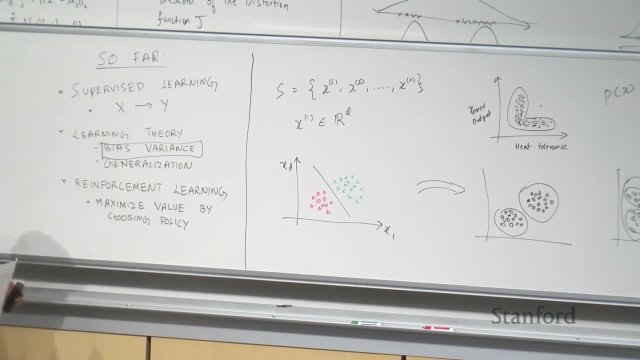 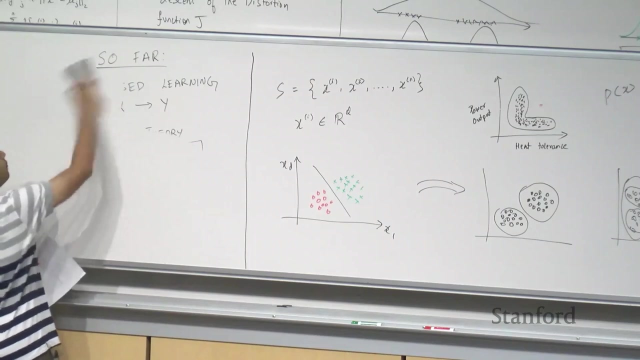 to it later with you know, and see how we can kind of approach it in a more principled way. You know, for now, you know as- as a mental exercise- see how you can apply bias-variance analysis in this kind of a setting, right? 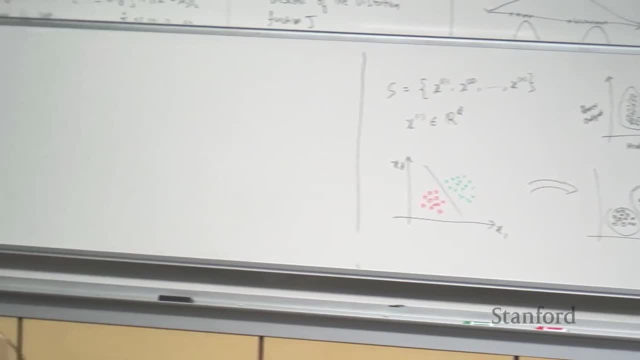 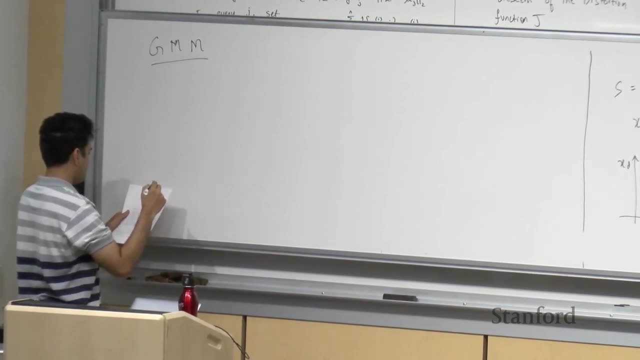 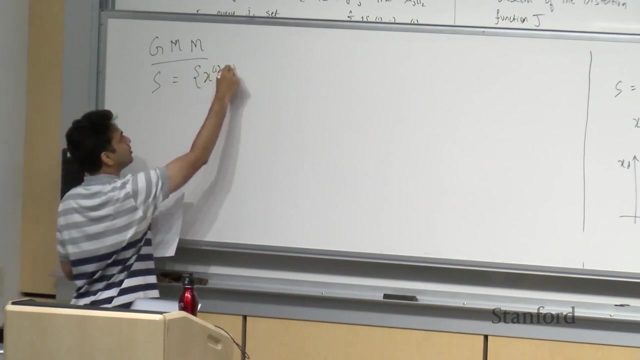 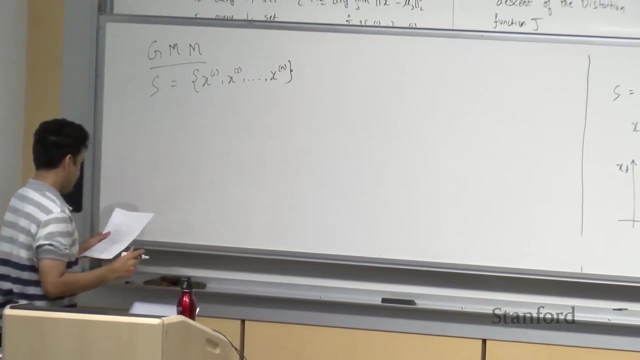 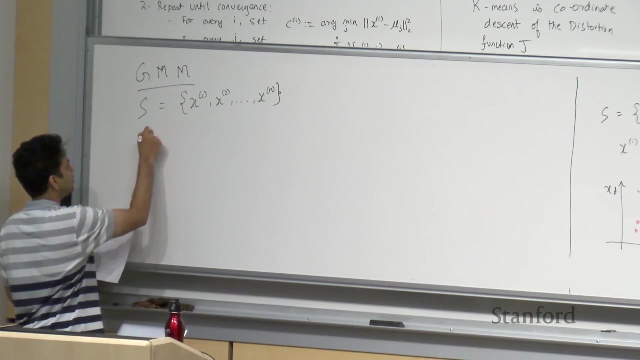 So in the uh mixture of Gaussians or Gaussian mixture model. So we are um, we are given a training set of just x's right, And then we're gonna assume there is this uh zi which belongs to a multinomial distribution. 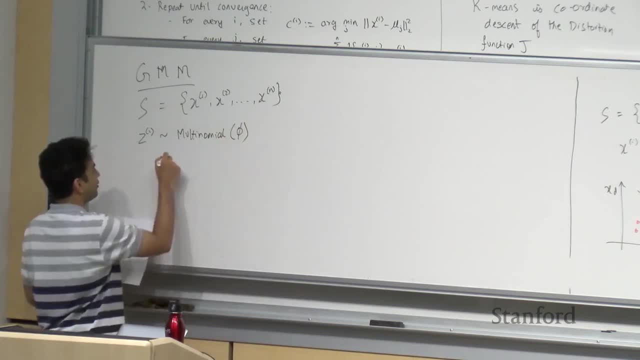 Parameter-. with parameter phi, where phi j is greater than or equal to 0, and the sum overall j equals 1 through k, phi j equals 1, right And phi j is basically um, um. phi j is the probability that zi equals j. 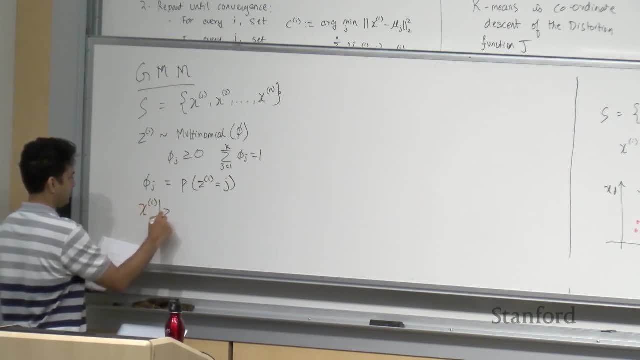 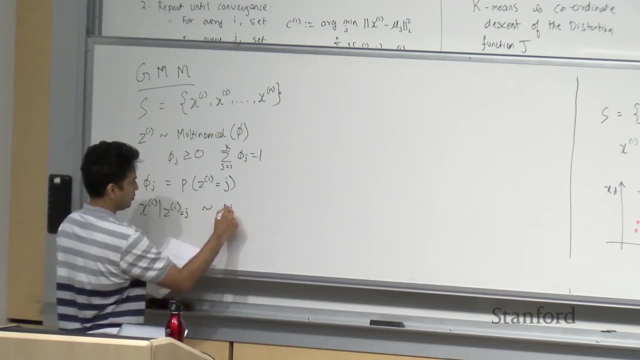 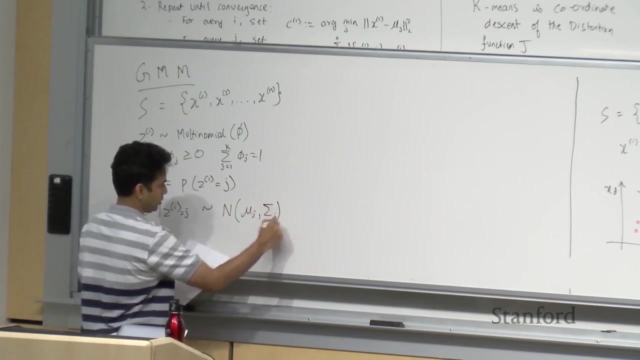 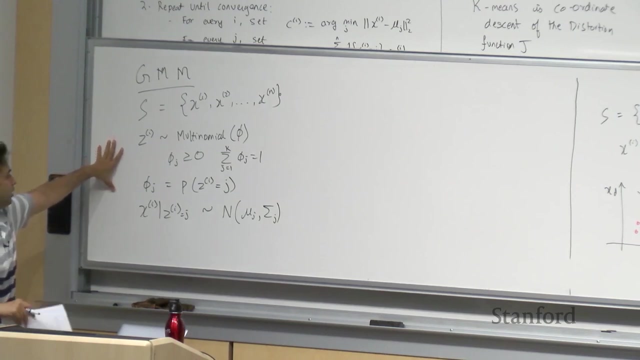 And then we have xi, given zi equals j to be distributed from a normal distribution of mean mu j and covariance sigma j right. So this is describing the model. So the- the way we uh assume the model works is that first we sample the 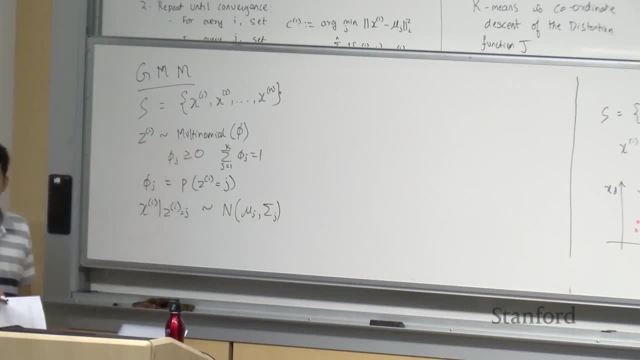 um, the class identity z from some kind of a multinomial distribution, right, And then you know, once we, once we have uh, sample the identity, we generate, you know an observation x, conditioned on the z value, that we 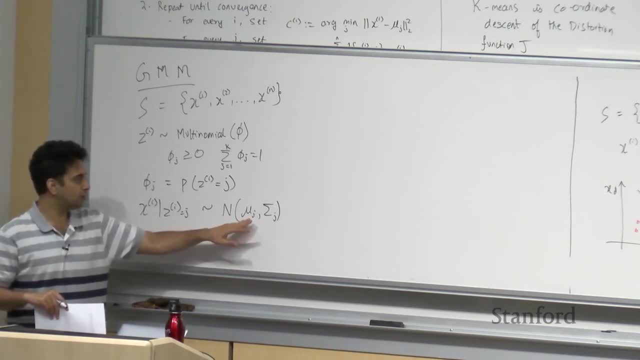 sample from some particular Gaussian distribution with mean mu j and covariance sigma j. This is very similar to GdA. right In GdA, um uh, the- the- the- the differences between this and GdA- uh. 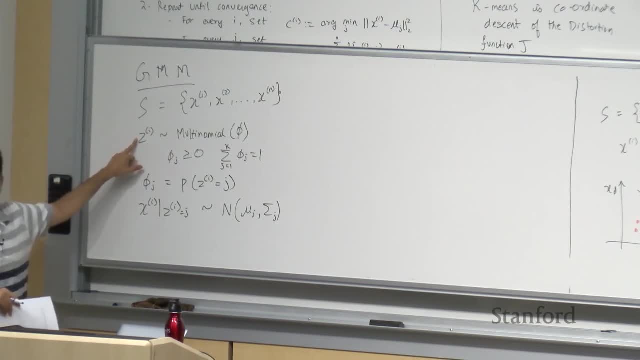 Ah, um. so what happens if um, uh, uh, dA is that in gdA we call z as y, Here we're just calling it z, And that is a common pattern that you will see when you know. 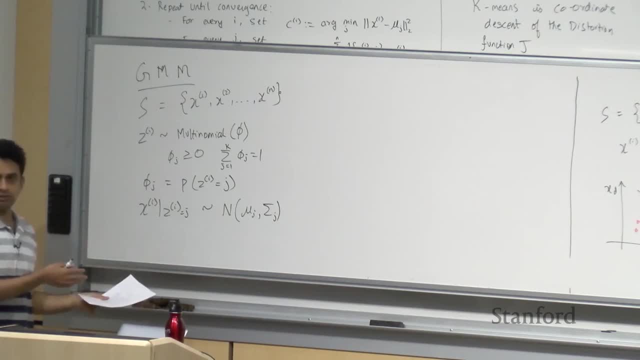 in-. in-. in the algorithms where we are doing full observation, which becomes a supervised setting, the variables that we call y, we end up calling them as z in unsupervised setting because they're not observed, right? In this case there is this underlying z that we do not observe. 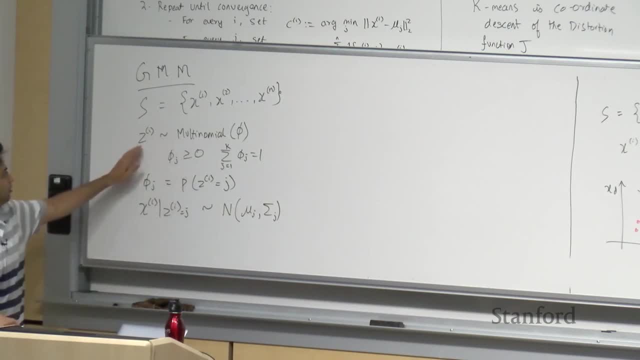 that is sampled from some multinomial distribution And, depending on the identity of the cluster that we- that we sampled, the observation is then sampled from a corresponding Gaussian distribution that has a mean and covariance specific to that cluster right, In these cases zi's. 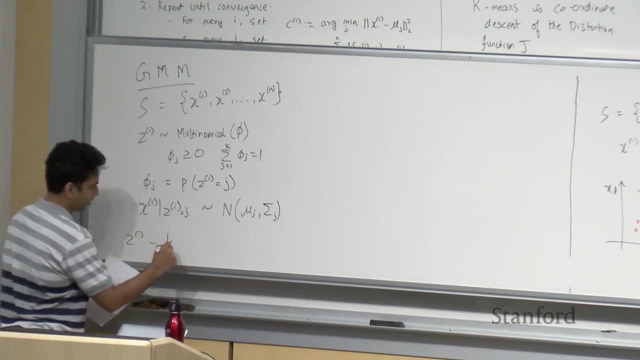 because they're not observed, are called latent variables. So latent variable is a fancy name for a random variable that we've not observed. You've just not seen what- what-, what its value is, and that's why we call it latent. Yes, question. 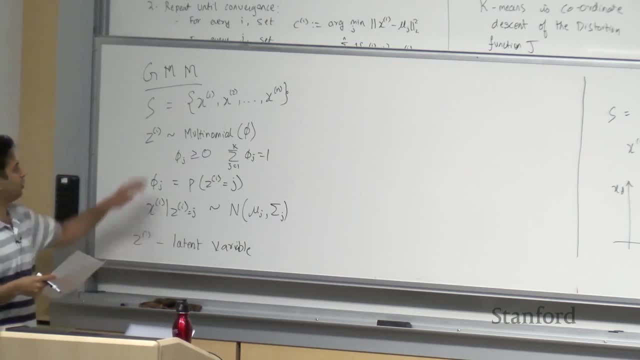 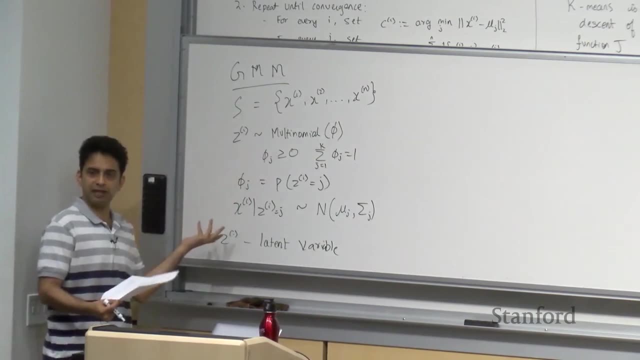 So is there a phi in the class probability? So phi over here is the- you- you can think of it as the class prior, The-, the- you know the- the- the class prior that we had in gdA. This just tells us of all the examples. 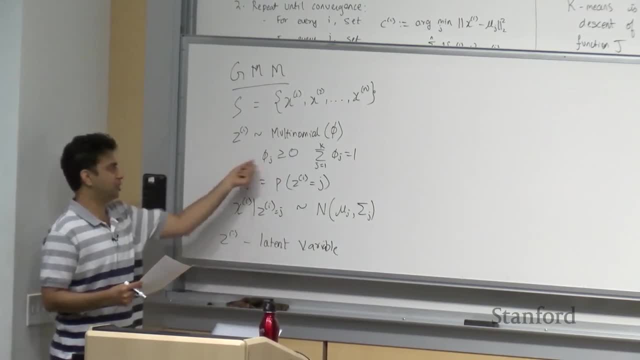 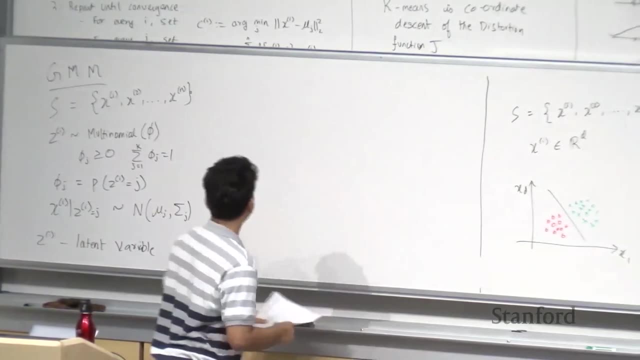 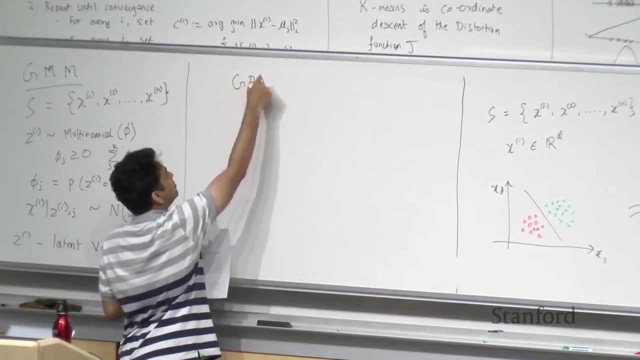 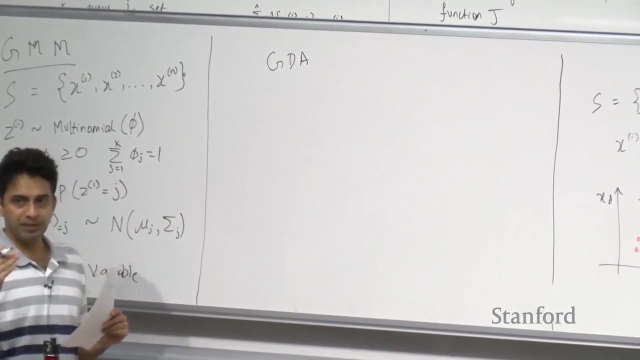 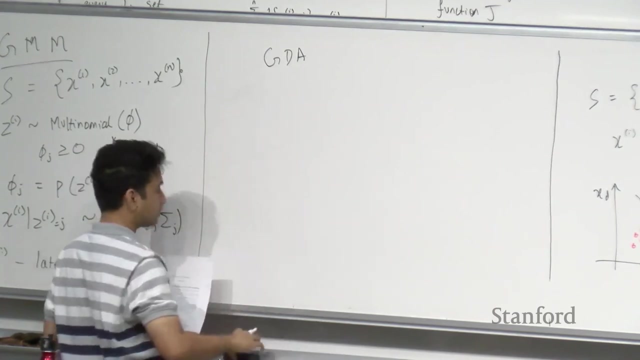 x's that we have. what fraction of them belong to cluster j? Good question. And now in gdA we perform maximum likelihood estimation in gdA and our maximum likelihood objective was- in gdA, it was log p of x. 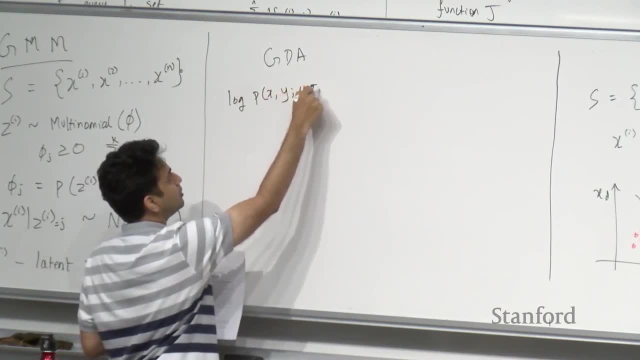 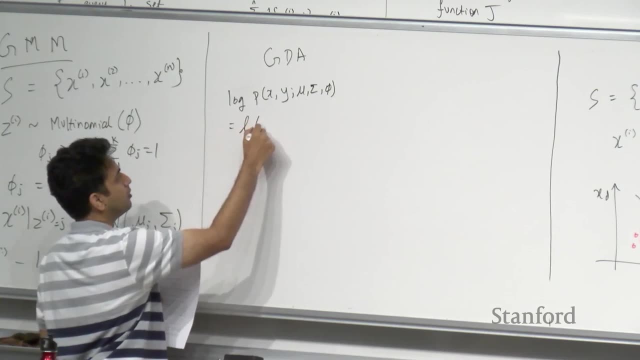 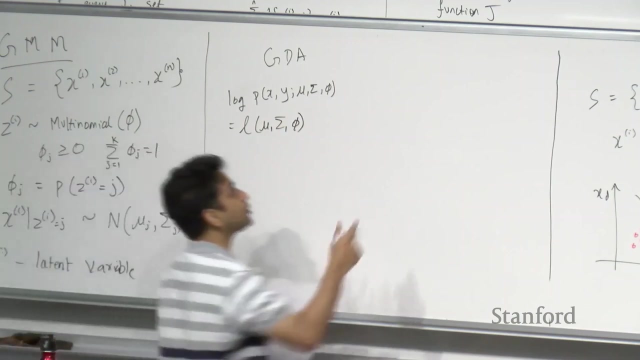 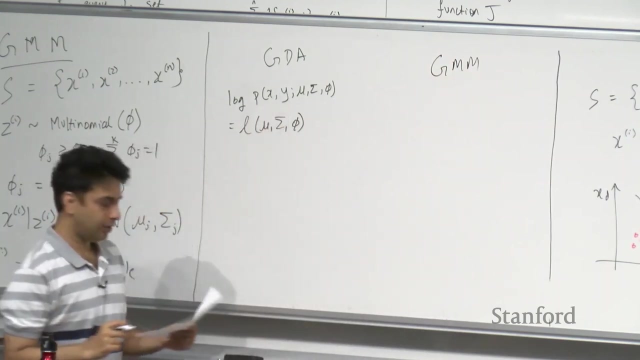 y, where mu, sigma and p were the parameters right. So this was the log likelihood objective in gdA right, Whereas in Gaussian mixture model we do not observe y right, And so in the- in- in the Gaussian mixture model. 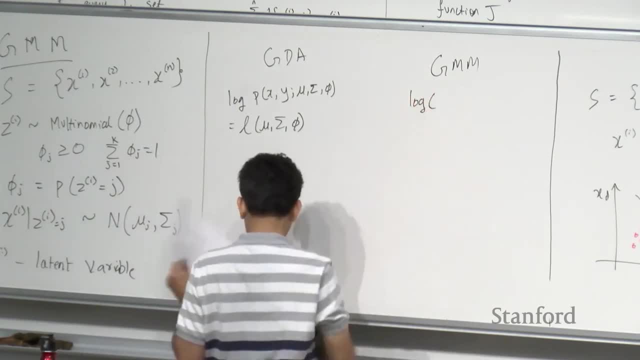 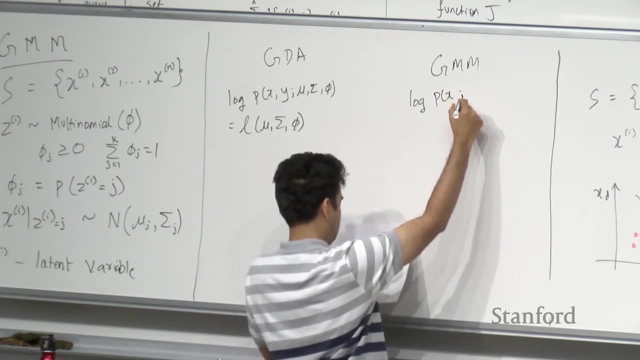 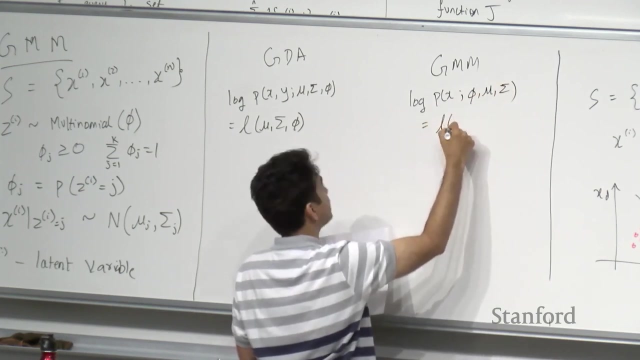 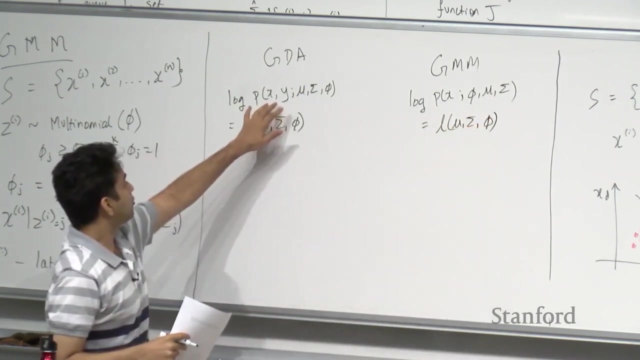 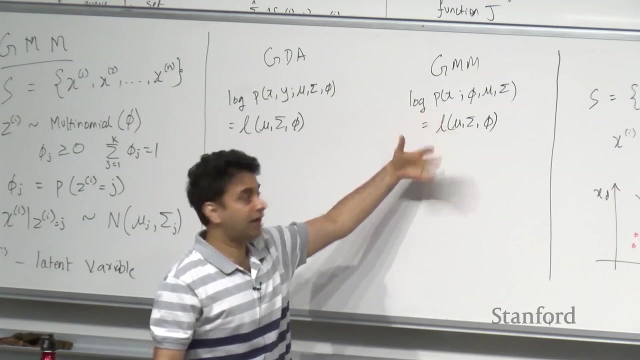 our objective will be to maximize log p of x given for phi mu sigma, And this will be our likelihood function right. That's the only difference Over here. your objective was the full joint distribution. Over here. we would have liked to do the same, but we haven't observed. 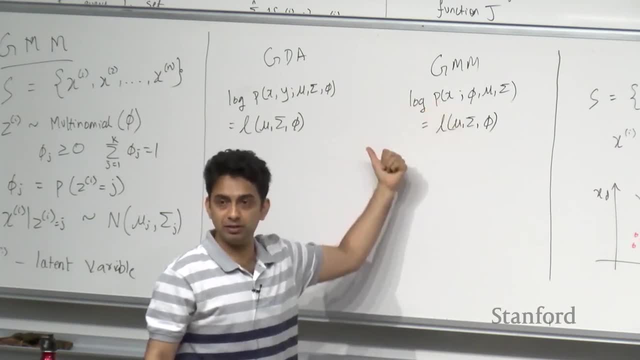 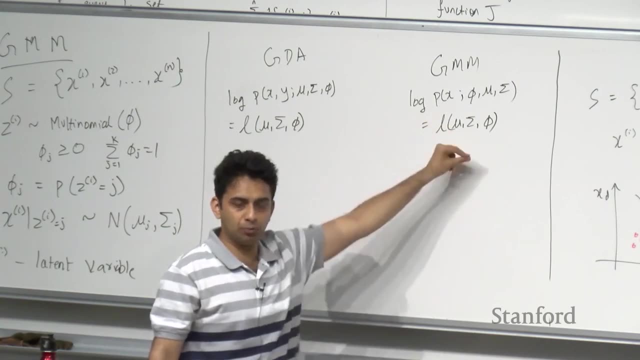 The wa- the corresponding y's, which we call as z's here, right, they're- they're- they're not observed. So we cannot construct a likelihood function because we won't know what value of z to plug in in this expression, right? 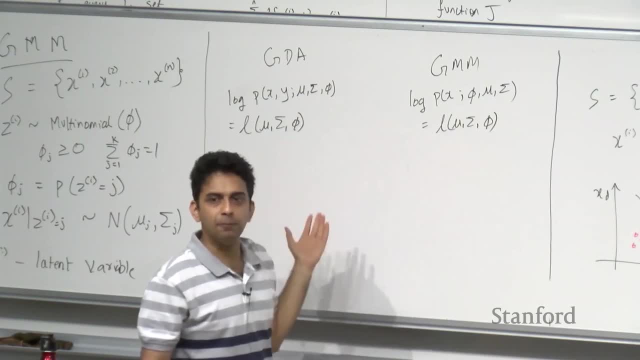 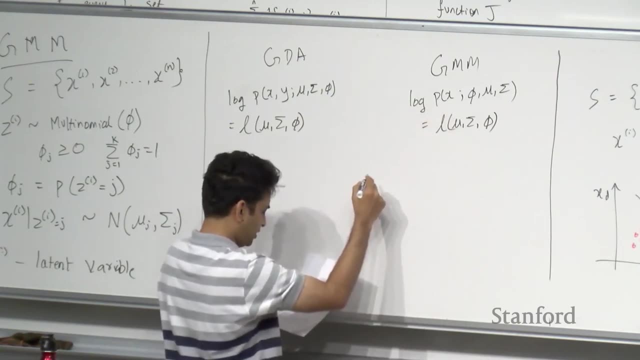 If you had observed them, it- it was pretty straightforward. we would have been just doing gdA, And so instead, what we do is maximize log p of x- right And log p of x can- can also be written as log sum over z. 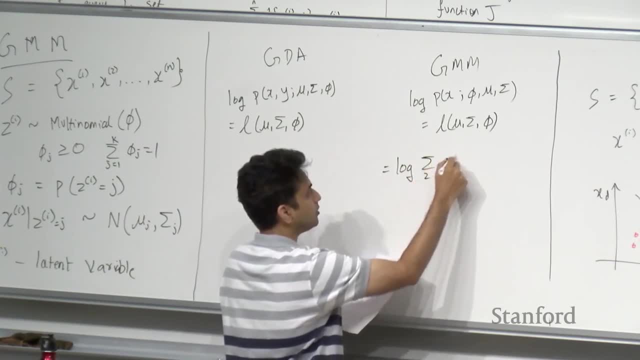 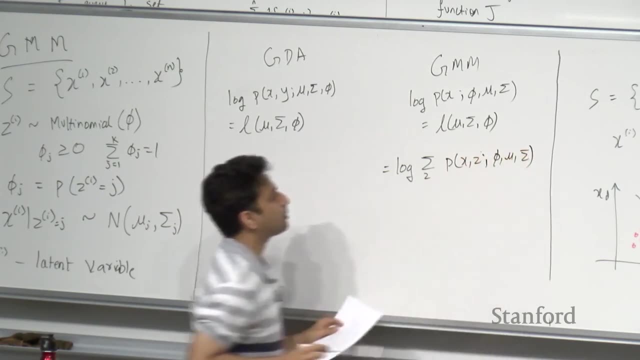 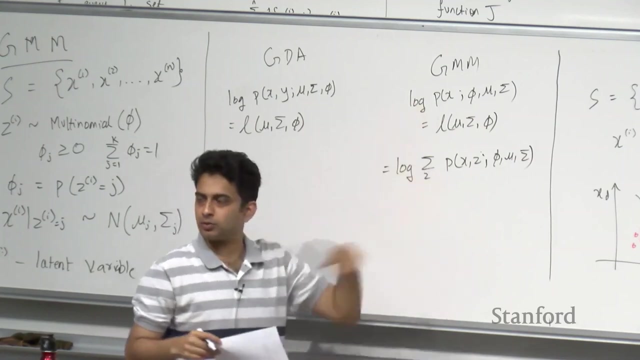 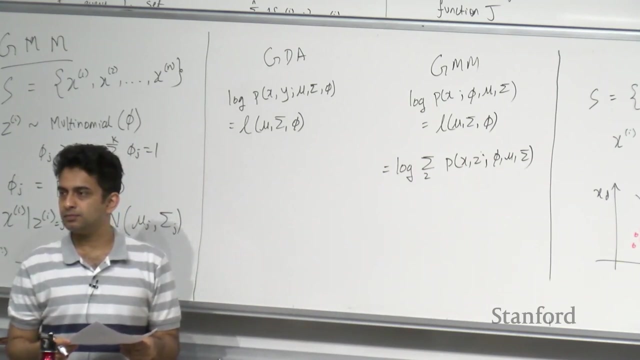 p of x comma z phi mu right. So we write out the full joint distribution and marginalize out the latent variable. Any- any questions how we went from this to this? This question? So the question is: uh, uh. 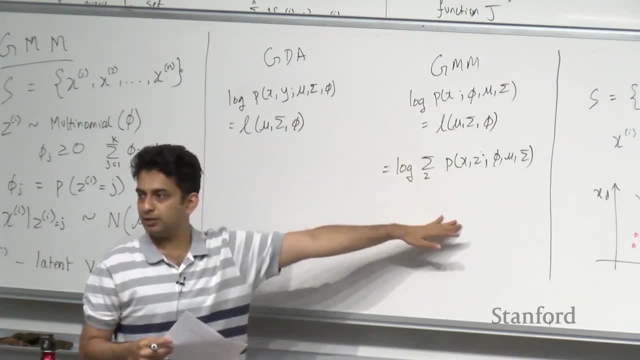 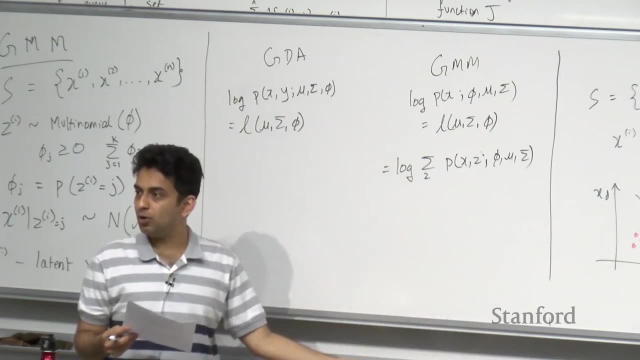 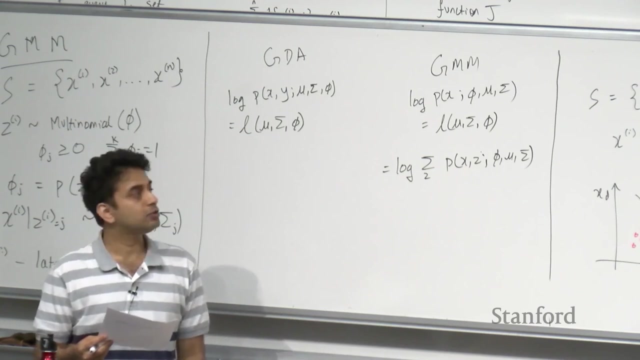 shouldn't z also contribute to our, uh, likelihood objective? And the answer is: if we had observed z, then yes, it should have. but we don't know what z is, So it- you know it cannot, So the- so the- so the question is: 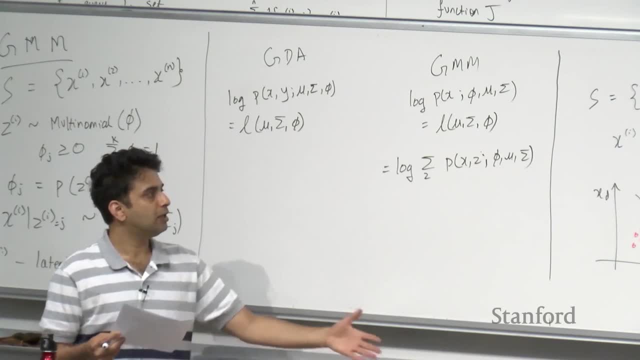 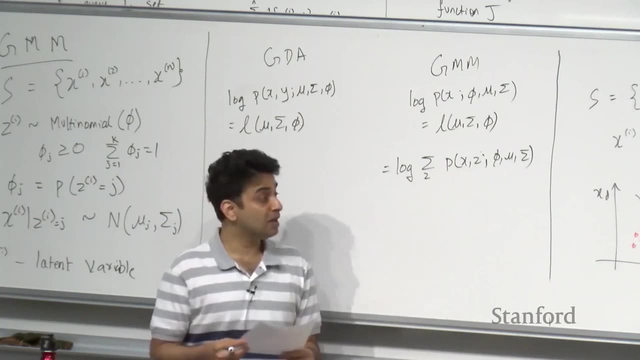 we are assuming there are k clusters and given a setting- uh, you know some value for k, shouldn't we therefore- uh, account for- for the cluster identity? Um, we are making an assumption about k, but we don't know which of those k clusters each point belongs to, right. 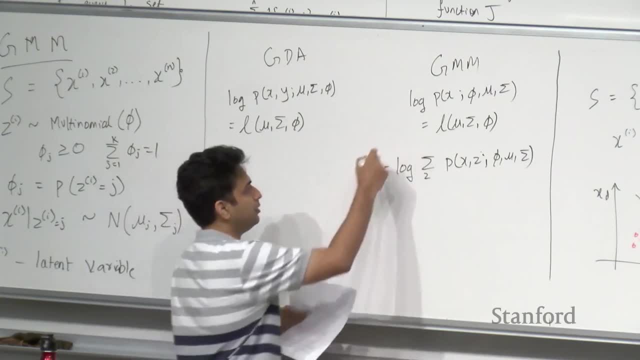 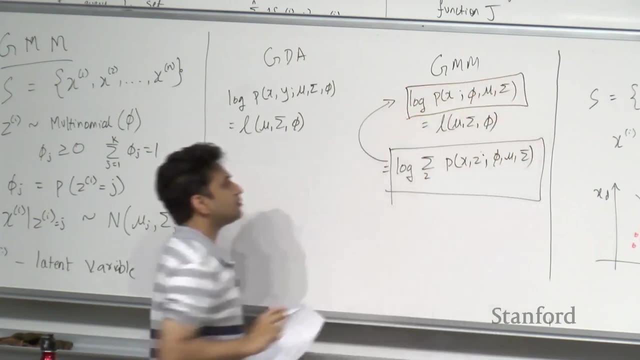 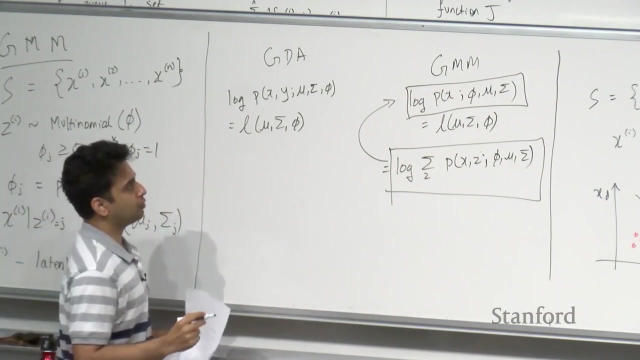 So our objective is to now maximize this expression, which is the same as this expression, right, And for the rest of- of uh- you know, today's lecture and- and throughout uh, it- it can be useful to set up. 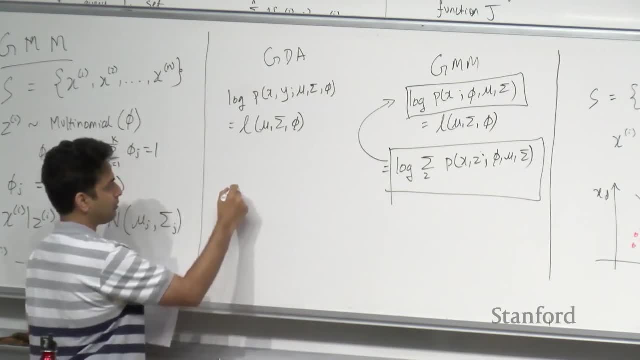 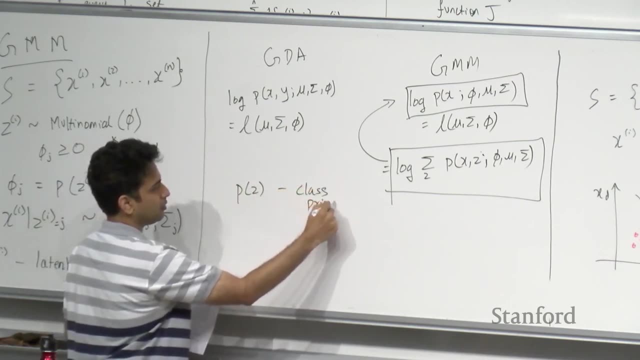 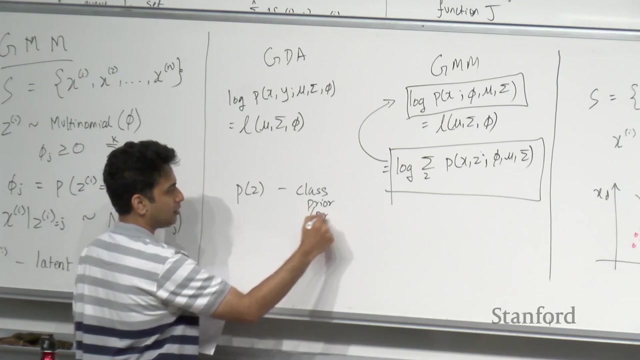 you know some kind of uh terminology. So, for example, p of z, we will call it class prior. or in cases where z is not discrete but it's continuous, we'll just call it prior right. P of x, z, we will call it the model. 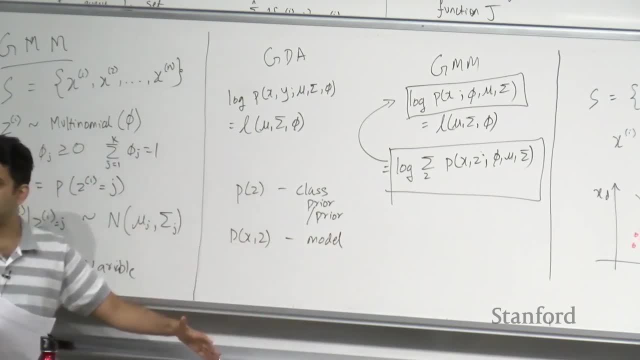 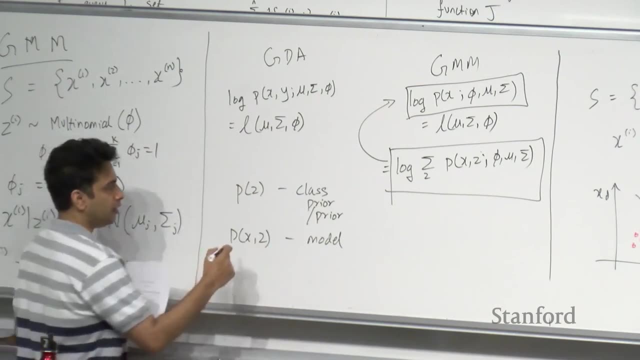 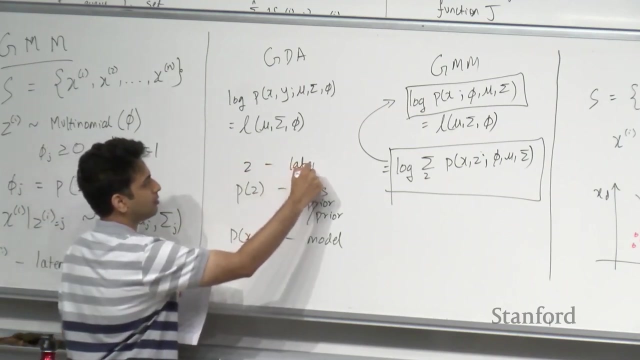 because it- it describes the full data generating process. The joint distribution- always gen- describes the full data generating process and that's always called the model. right And z in unsupervised settings is called latent because we don't observe it. 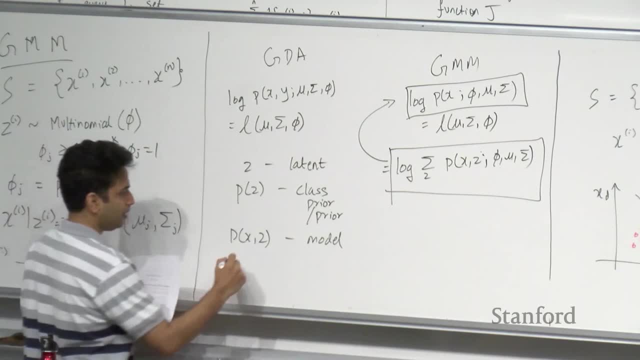 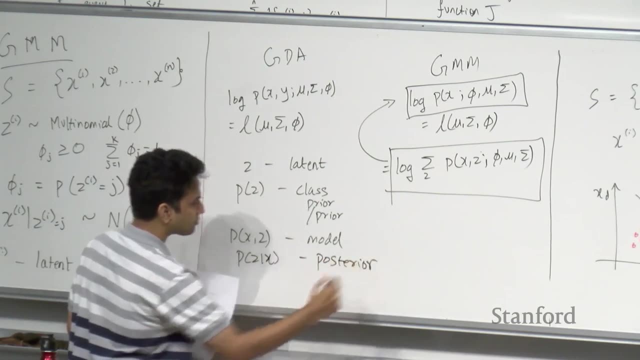 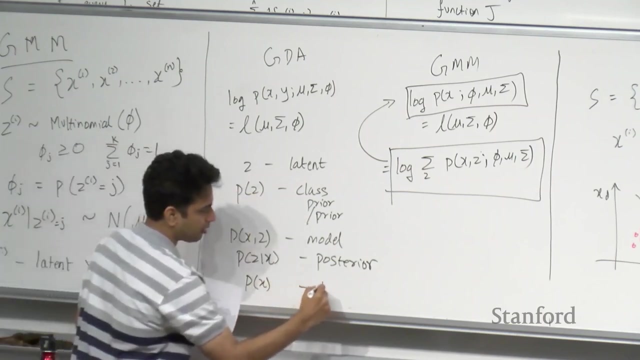 Latent is just a fancy word for unobserved, And p of z. given x, we will call it the posterior right And finally p of x. So p of z is called the prior and p of x will be called the evidence. 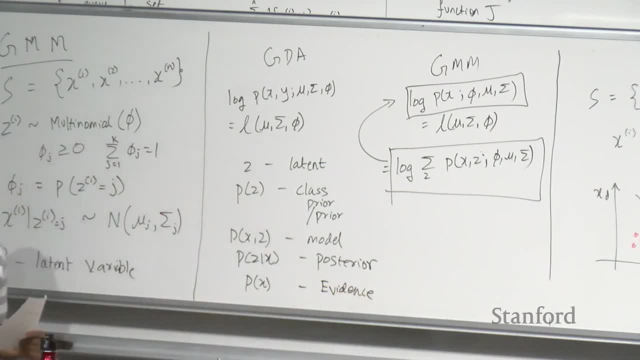 Evidence, because x is what we observe. that's the evidence based on which we are performing inference. right? This is just terminology And in this case we will call it evidence to the keyboard behavior. in this case, This is just terminology And in this case we will call it evidence To the keyboard behavior. in this case, it will be called the evidence as foresight. 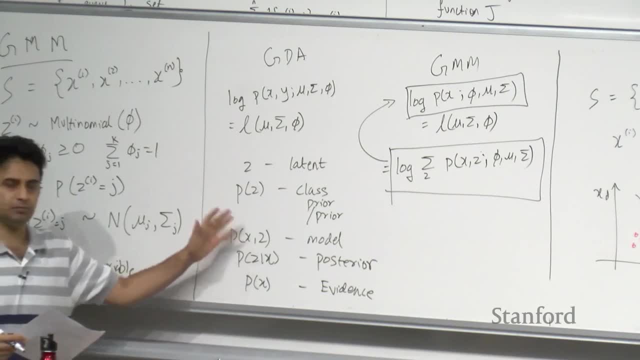 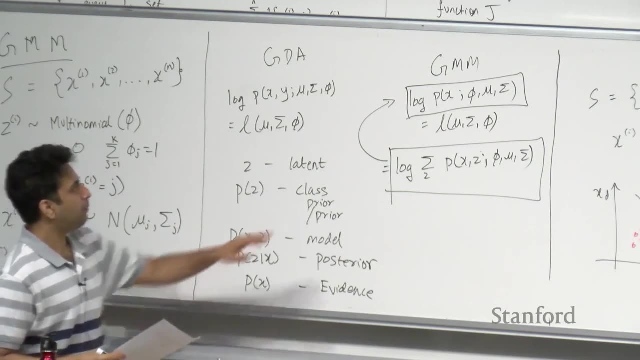 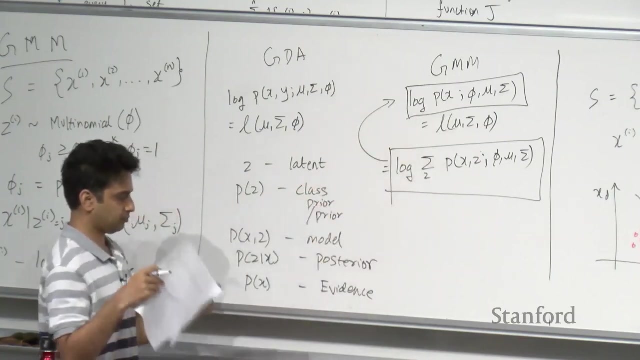 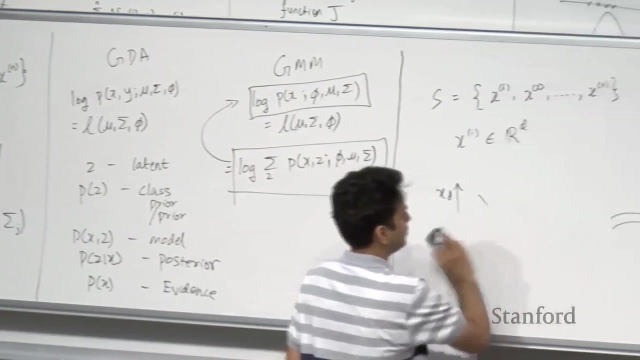 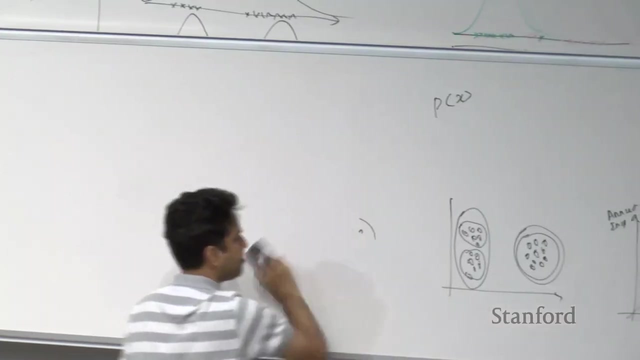 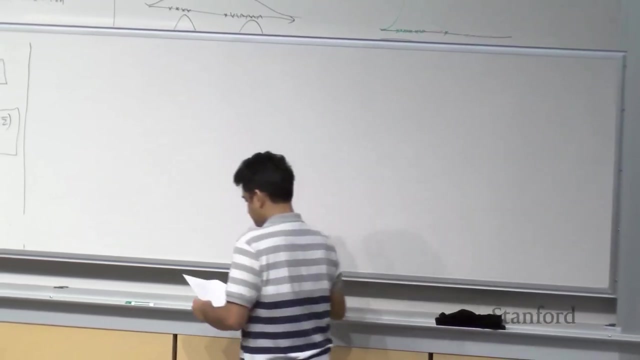 and this terminology is- is pretty standard and, you know, used in many papers, many, many books. So our goal is to maximize the likelihood, using the evidence right And this- the way we go about doing that- is right. 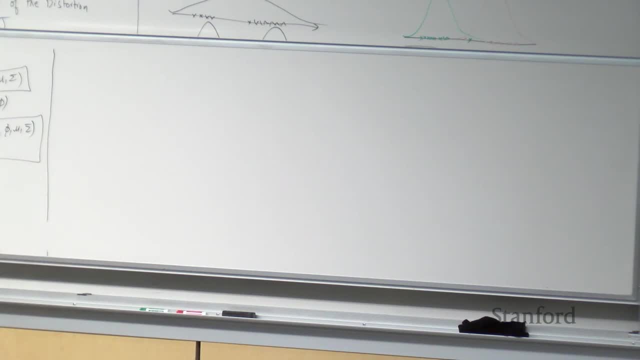 So to directly maximize this evidence, uh, uh, directly, ma- uh, maximizing- maximizing this likelihood, if we were to attempt it the way we did it with GDA, of taking derivatives, setting it equal to 0 and solving for the parameters. 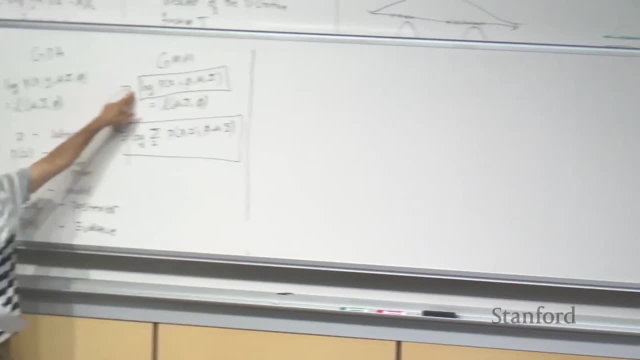 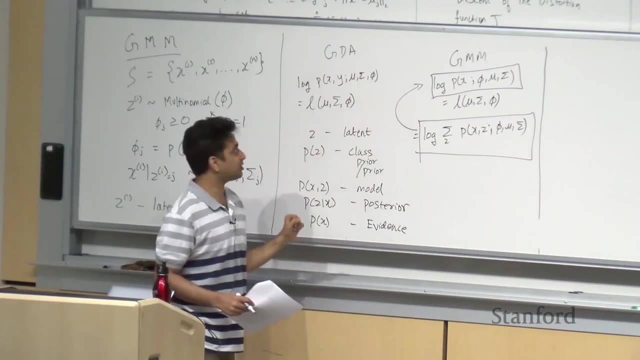 you will observe that you won't get a closed-form expression for this. You can try it out. you know you won't get a closed-form expression for the way we got it with GDA. In GDA we got a closed-form expression because we had observed both x's and z's. 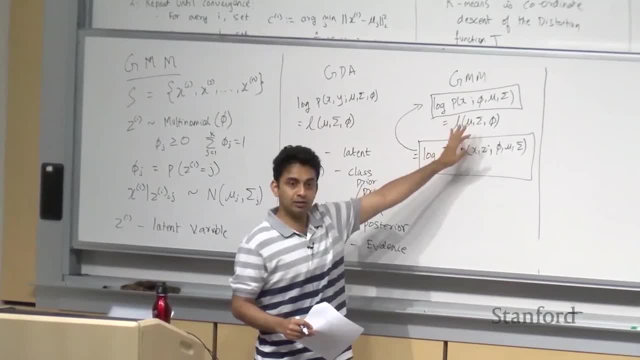 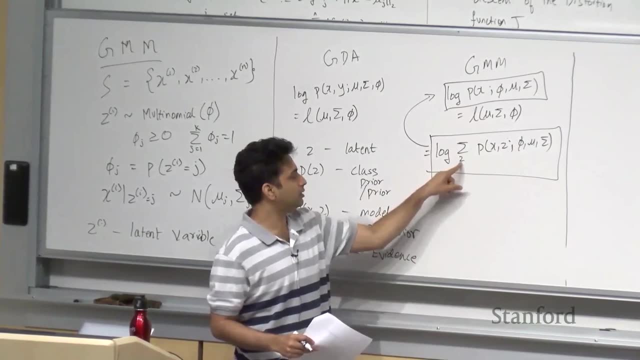 we called it y's, and if we had observed both x's and y's here, we would have gotten a closed-form expression. But because, uh, the z's are not observed and we are taking this uh uh, marginalizing them. 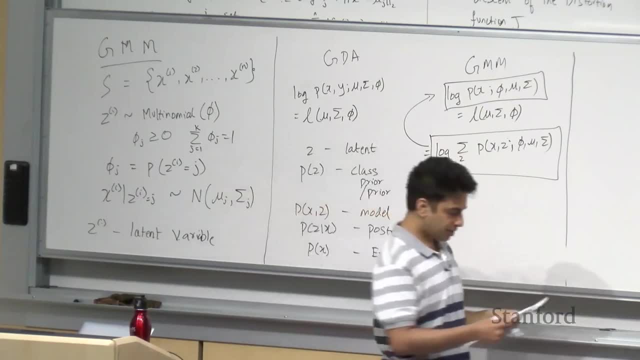 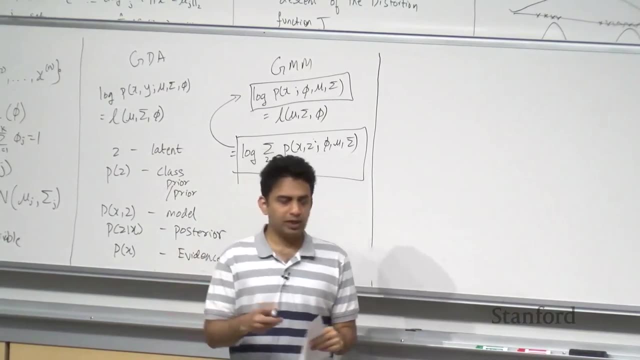 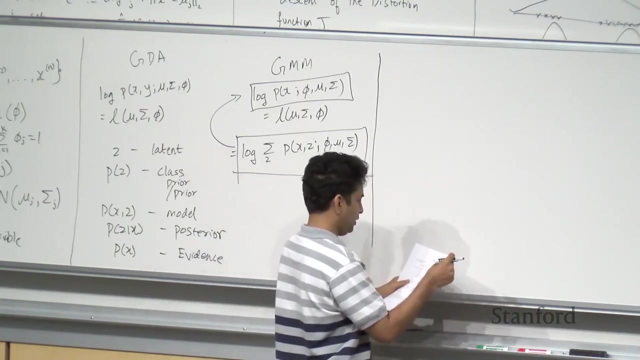 if you- if you work it up- we will not get closed-form expressions. So instead, what we will do is just like: uh, you know, uh, taking inspiration from k-means, we are going to first, uh, imagine or- or- or- or come up with some kind of an estimate for z i's first. 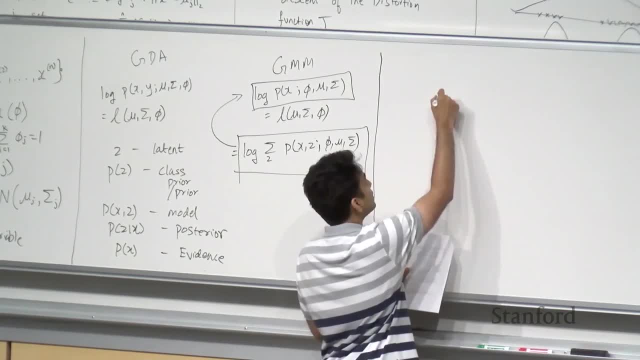 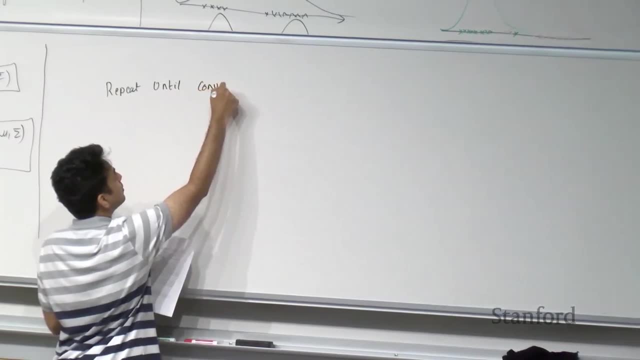 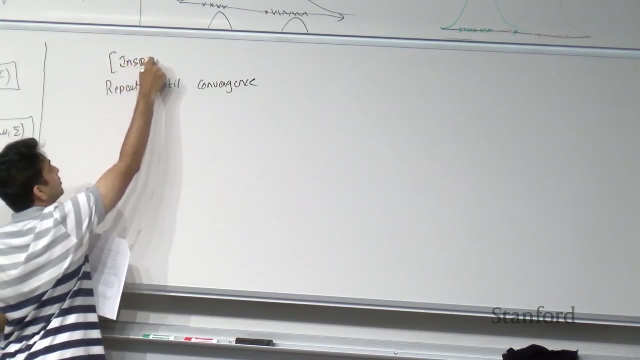 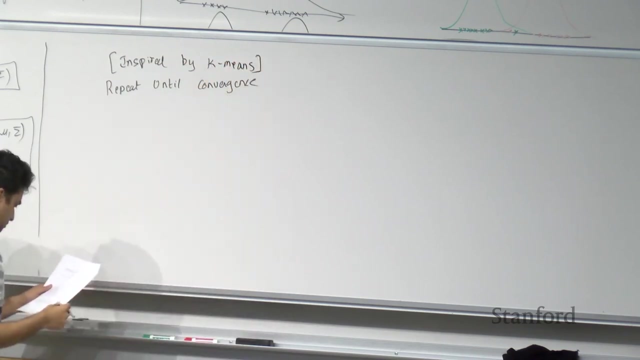 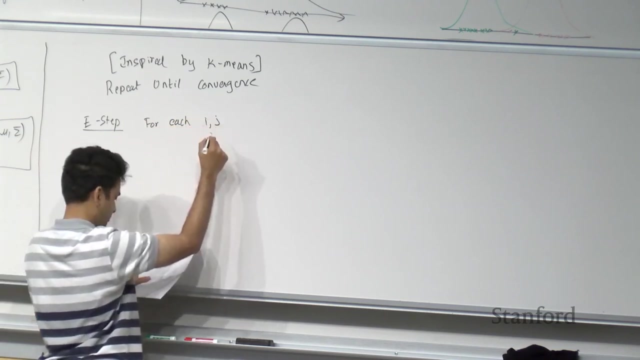 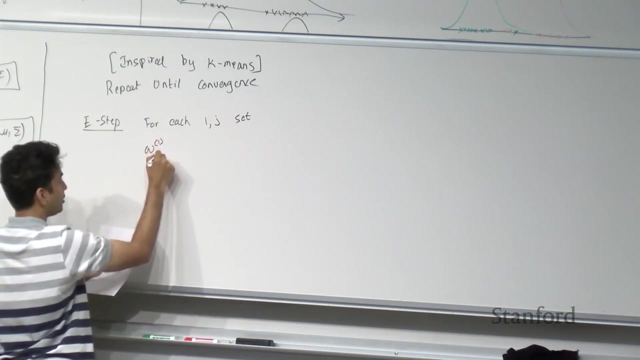 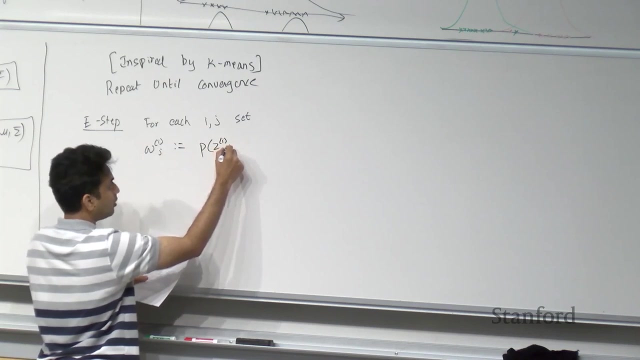 So the algorithm that we are gonna do is, uh, repeat until convergence. where this is, you know, just taken, inspired by k-means, We'll call it the E-step. For each i comma, j set Wij to be equal to P of z icals j given xi. 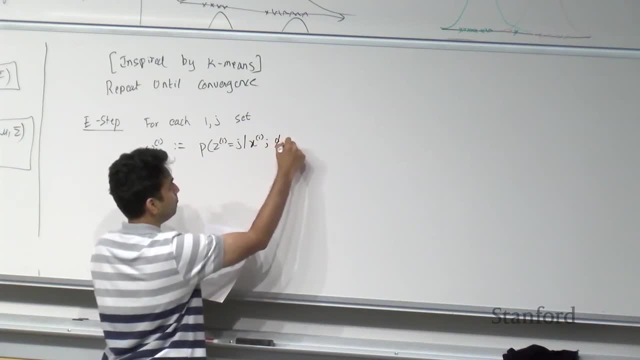 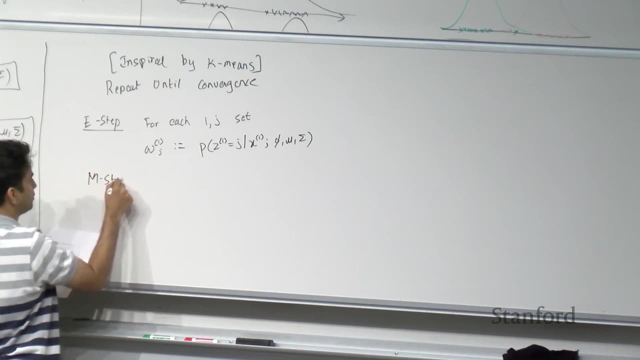 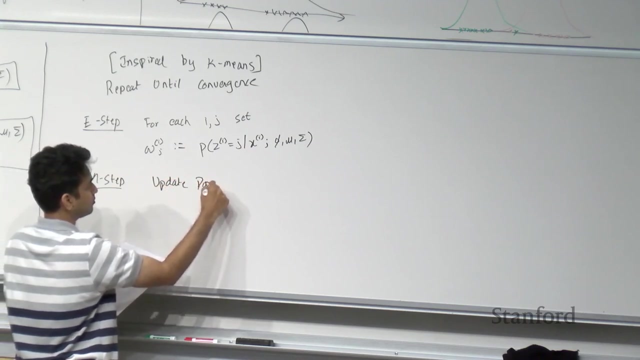 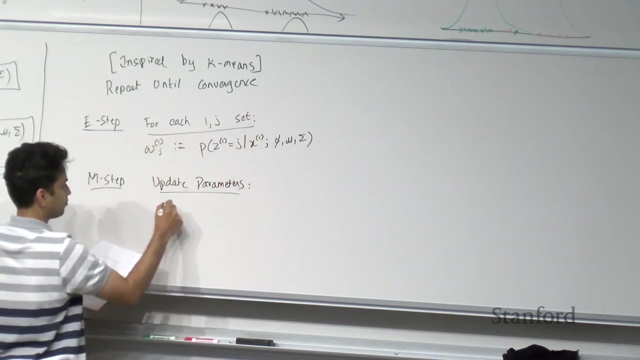 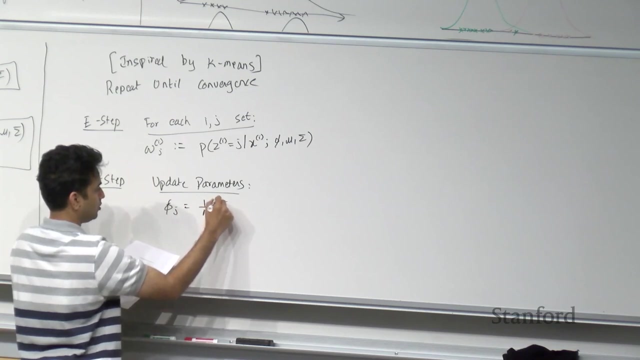 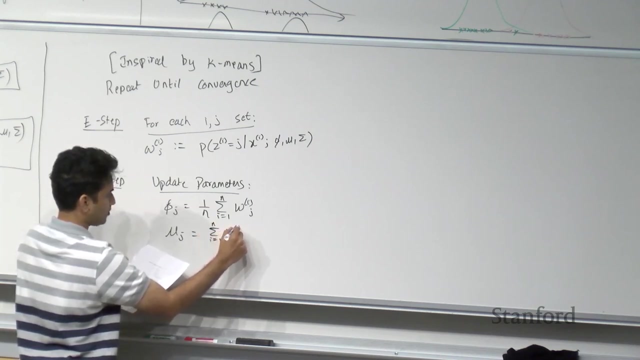 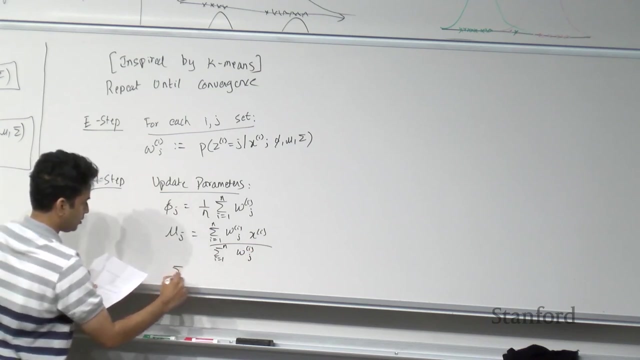 Parameters: phi, mu, sigma And the n-step update. the parameters: j equals 1 over n, 1 equals 1 to n, w and j 1 over mu. j is sum over i equals 1 to n, w, i, j, xi over i equals 1 to n w i, j. and sigma j is equal to. 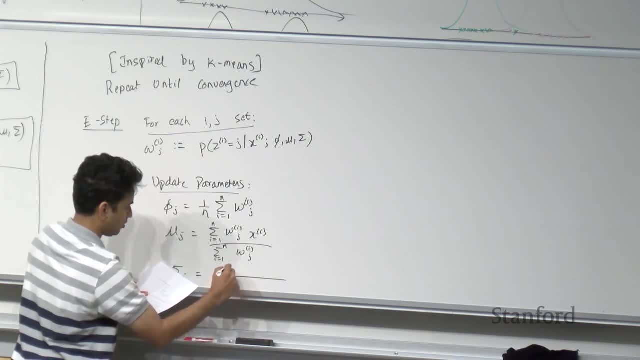 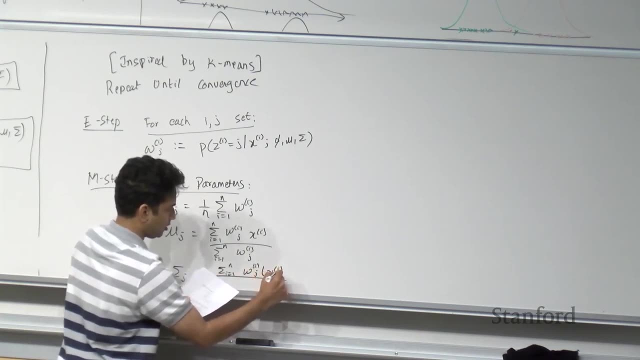 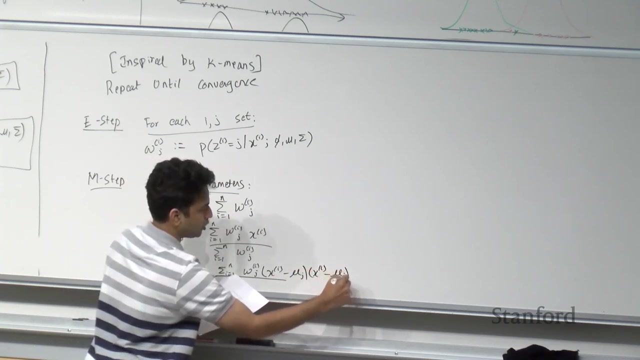 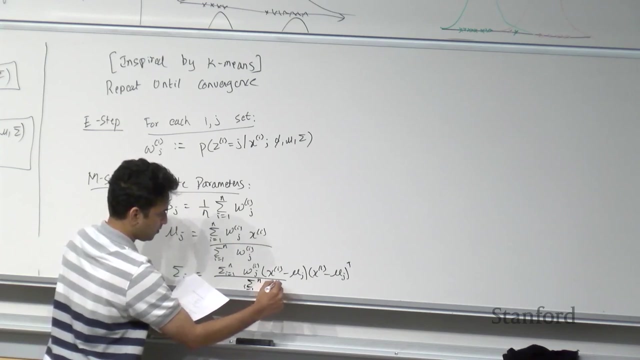 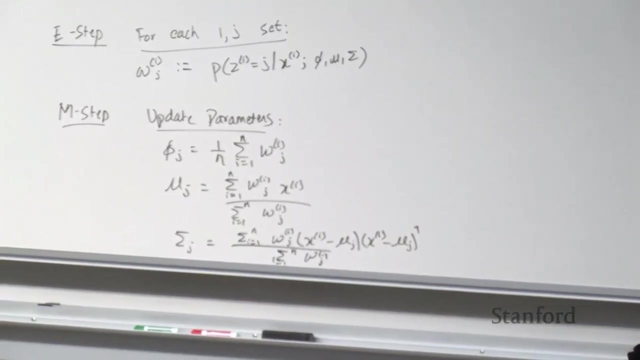 sum over i equals 1 to n w i j. xi minus mu j, xi minus mu j. transpose, divided by i equals 1 to n w i j. So what we did is we start with some random initialization. 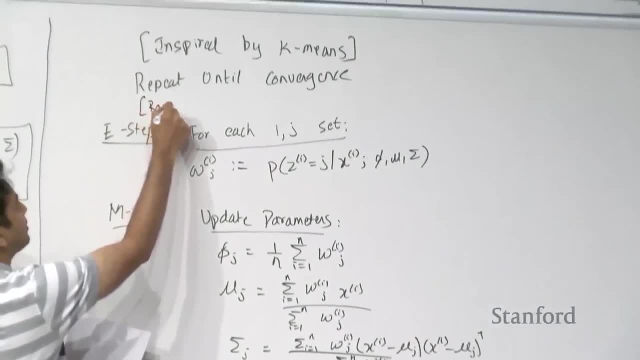 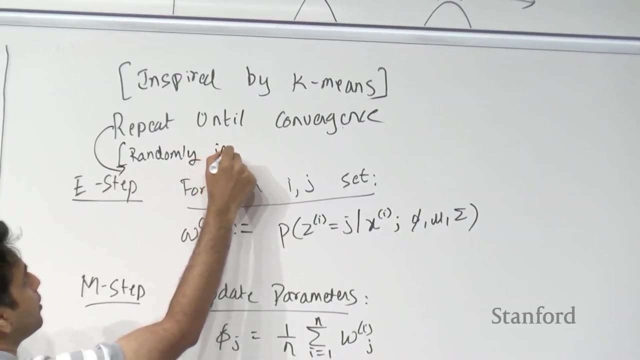 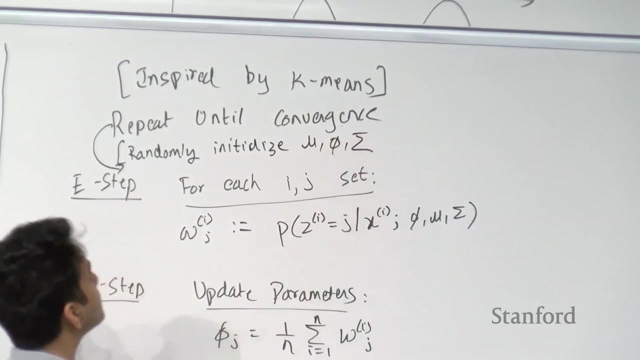 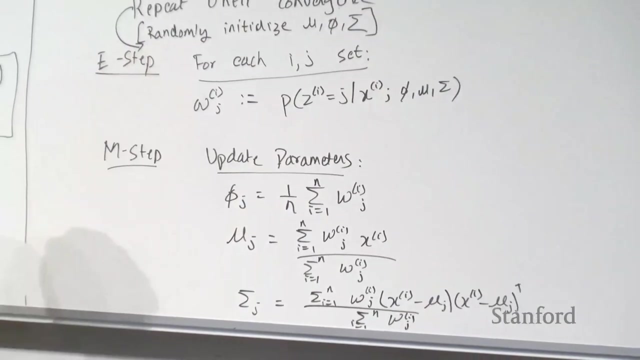 So uh, randomly initialized parameters, And so the repeat will start after we uh randomly initialize it. Randomly initialize mu, p and sigma. We start with some random initialization And think of this as the way we randomly initialize the cluster centroids and k-means. 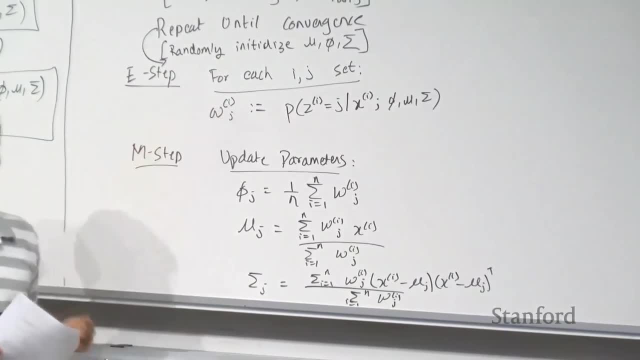 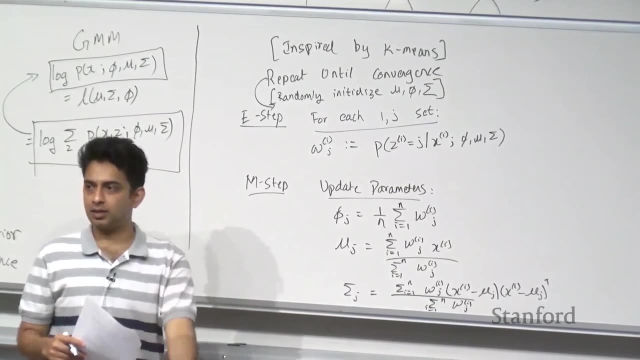 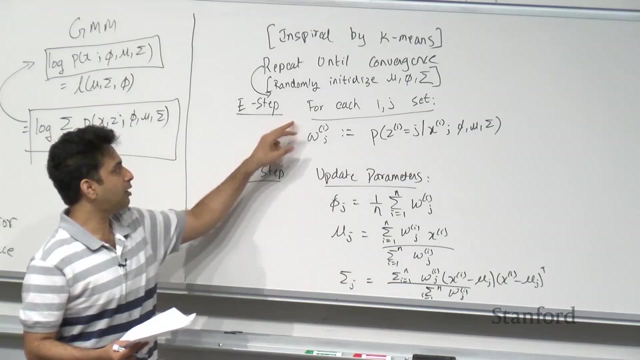 Right And based on the random initialization in K-means, for each point, we associated it to the nearest cluster centroid Right And the- the-. the kind of similar operation that you're gonna do here is, for each point, we're gonna assign a weight to each cluster centroid specific to that point. 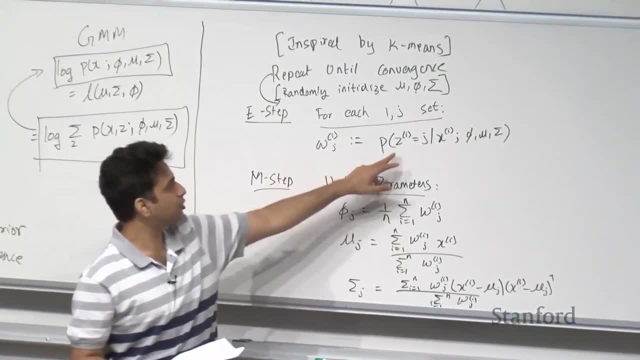 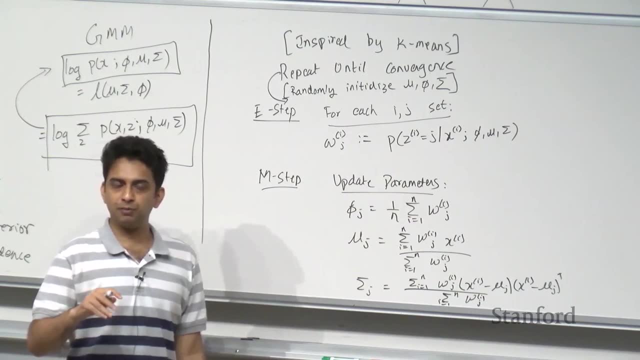 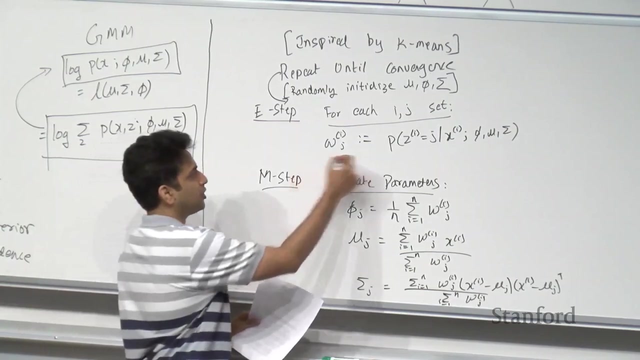 where the weight is the posterior distribution of p of z given x Right. So, given a point, we calculate a posterior distribution of the probability that this point belongs to a particular centroid. And this is just the posterior, uh um, the posterior distribution. 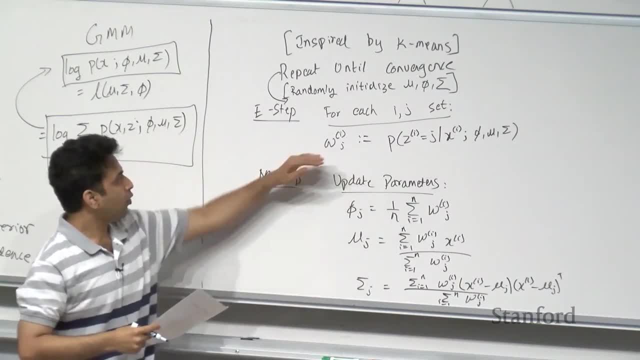 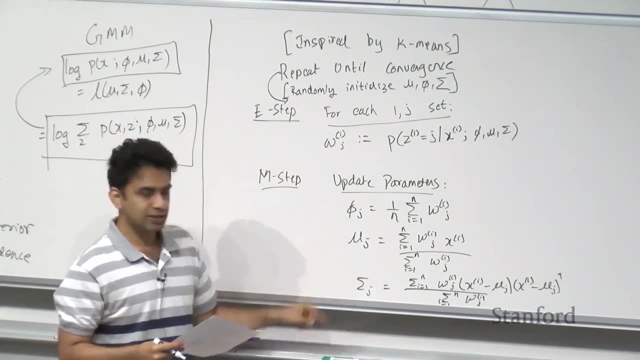 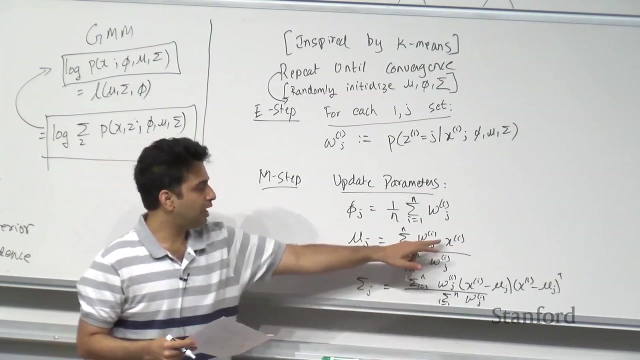 We're gonna call it a weight And once we calculate this weight, we're gonna re-weight all our data points to calculate the corresponding mus and sigmas Right. So, for example, x i will be-, um may belong to- will have a weight of. 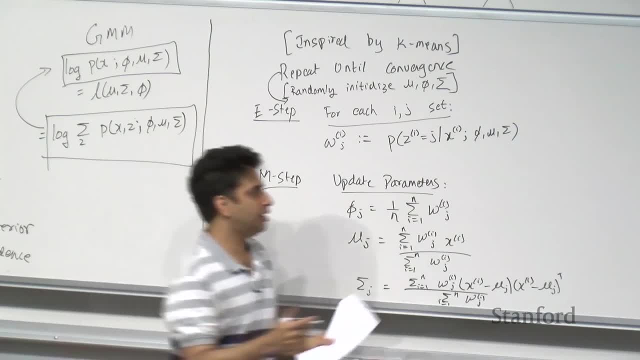 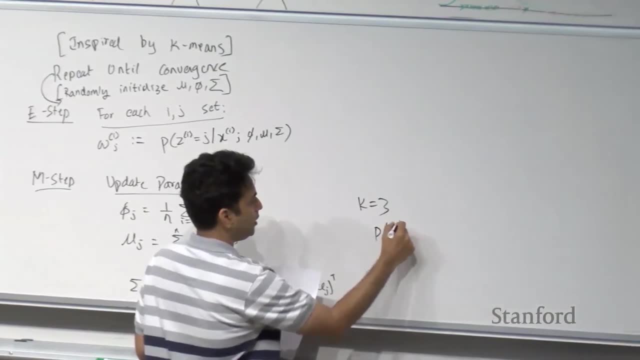 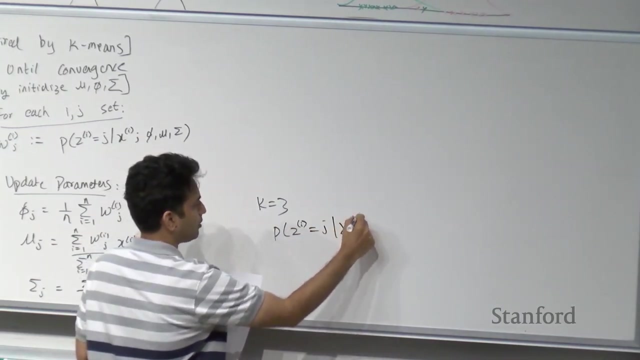 let's say um uh, if there are- if there are um, say three uh, centroids where k equals 3, then p of z i equals uh, um j, given x i right, This could be some kind of. 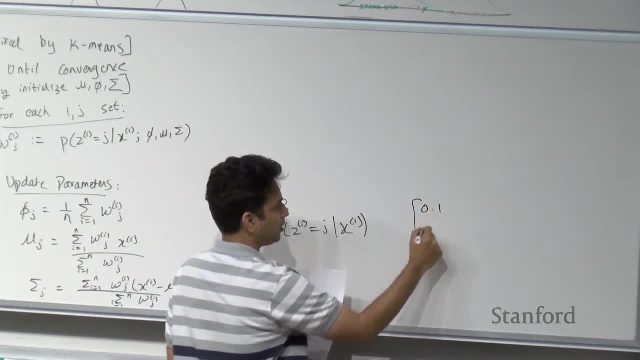 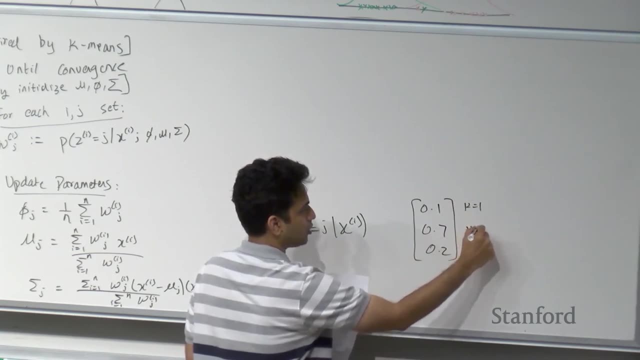 um multinomial distribution like 0.1, 0.7, 0.2, right, Where this belongs to: k equals 1, k equals uh, 2, k equals 3. Where, if the centroid mu was- was close to. 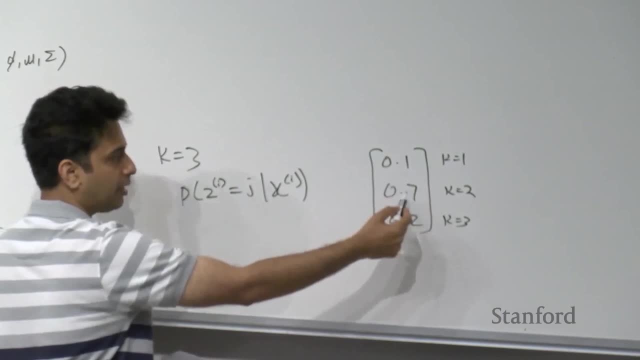 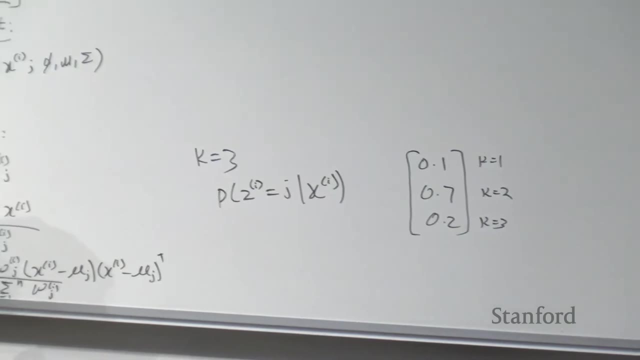 uh mu 2 was close to uh x i, then it would have a higher weight And you know these two are farther away so it has a lower weight. In- in case of k-means we would do a hard assignment of every point to one cluster only. 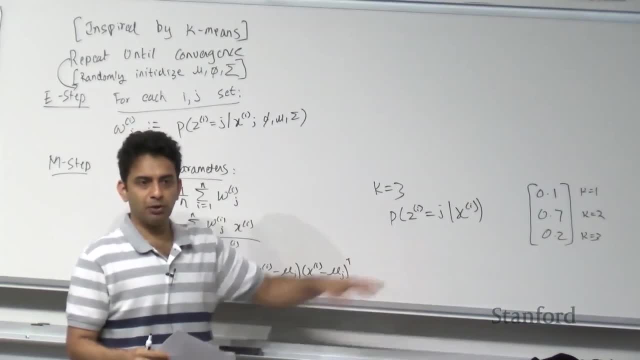 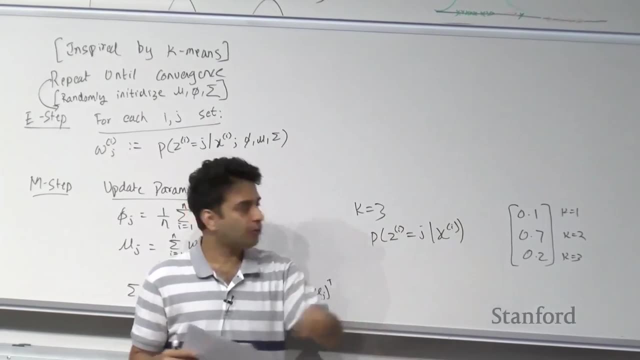 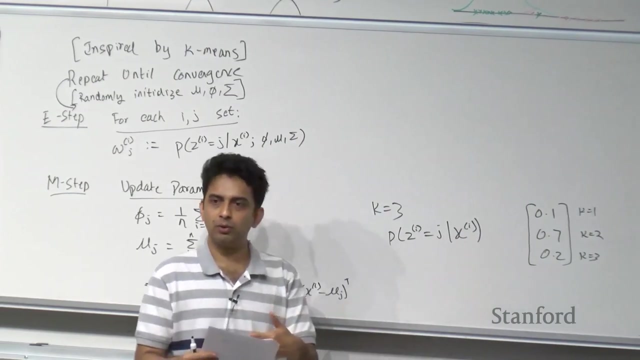 But over here you're doing a soft assignment, where every point has- has a soft assignment in the form of this probability distribution for all the cluster centroids And the- the probability assigned to the centroid that is closer to the point. By closer here we mean in a probabilistic sense, where it is 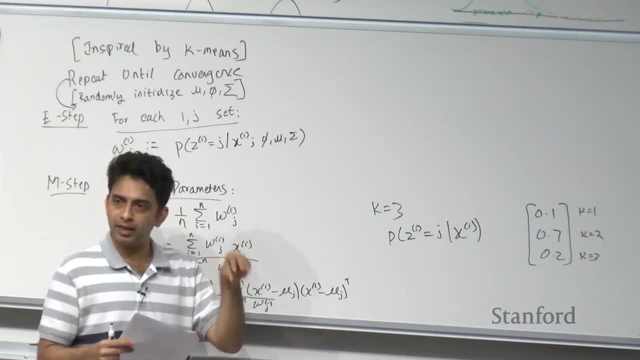 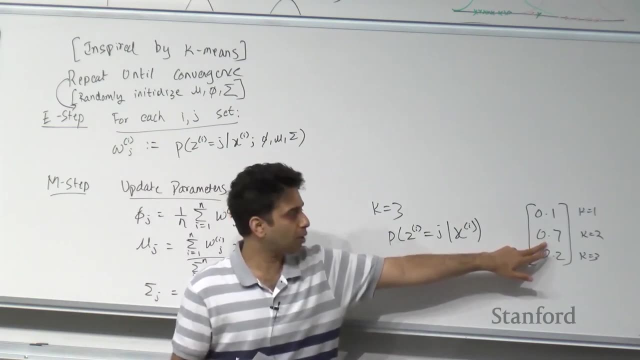 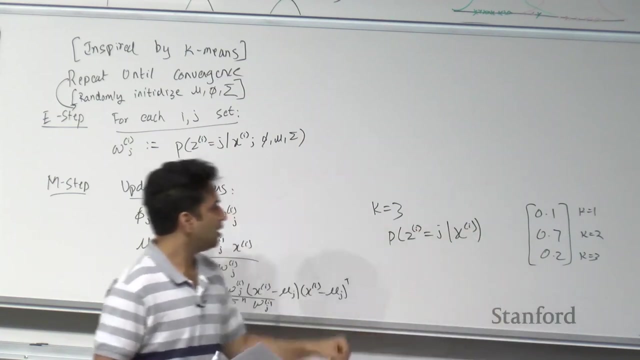 uh, it has a high likelihood in that- in- in- in that um clusters Gaussian distribution, then it will have a high posterior uh, uh probability. and we do this kind of a soft assignment of every point to- to the set of all clusters. 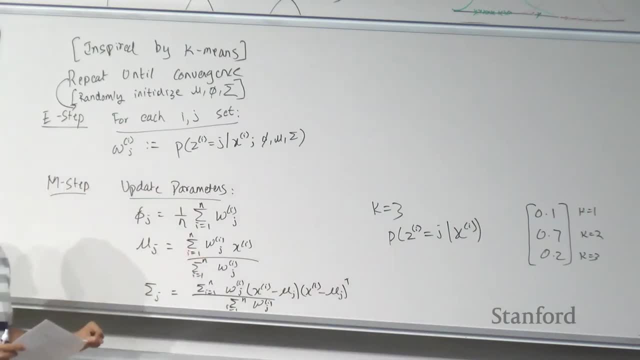 And using the- the cal- uh calculated weights. we recalculate the mus and sigmas using the weighted dataset. Here, every- every uh point i contributes to every centroid j and the contribution is weighted by the corresponding w i j Questions. 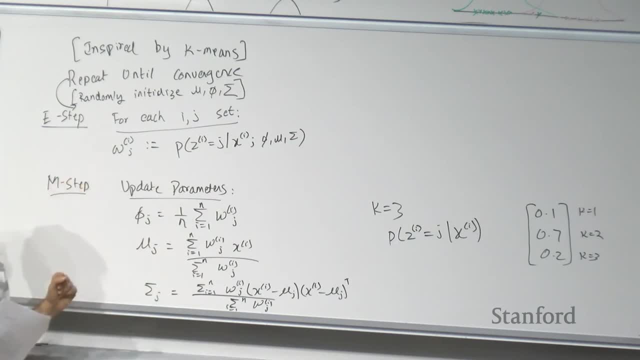 Yeah. So the question is, will this have a closed-form expression? Um, Yeah, Yeah, So-. so the question is- so for this, I would- I would uh remind you uh in- in case of GDA. 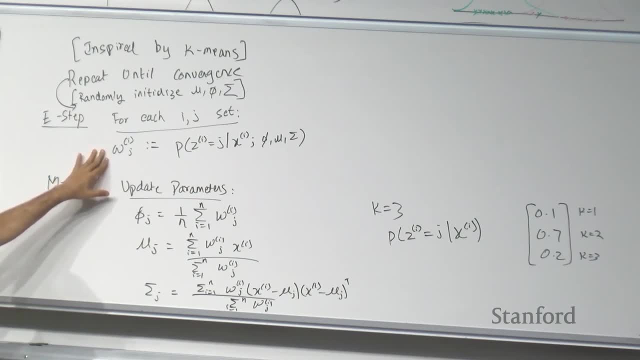 we had calculated a posterior that was very similar And, if you remember, the posterior had a form of Yeah. It had the form of a logistic uh, uh, uh regression. In that case, however, we limited ourselves to two uh. 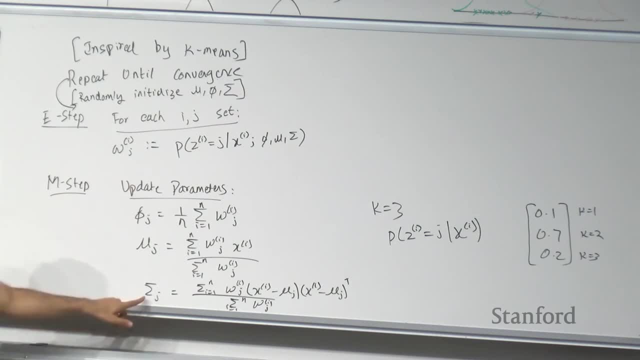 two points uh to two classes, and we also had a constraint that sigma was common to all of them. But in this case, when we relax that um uh constraint, what we will observe is that the posterior takes the form of a softmax right. 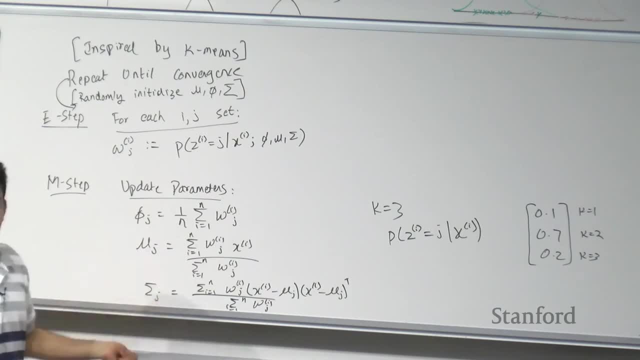 It-. it takes the form of a softmax that uses quadratic features, Quadratic features of x's, right, But uh, for- for a fixed value of you know, for- for small k's. you can, you know, come up with- with- with an expression for this. 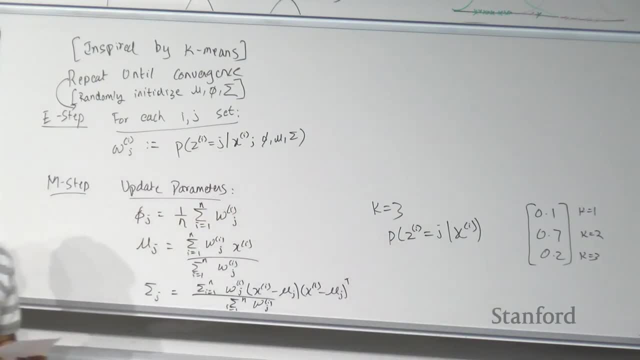 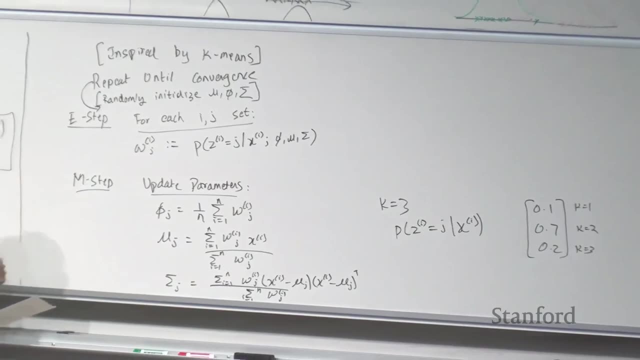 and in fact, you'll be doing this in your homework, So that will be clarified in your homework as well, right, So? um. so, inspired by k-means, here is a version of- you can think of the Gaussian mixture model as soft k-means. 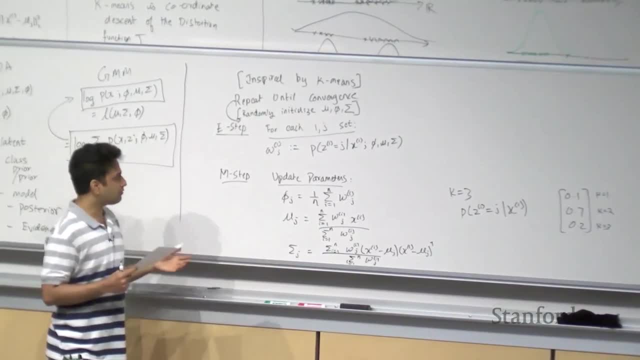 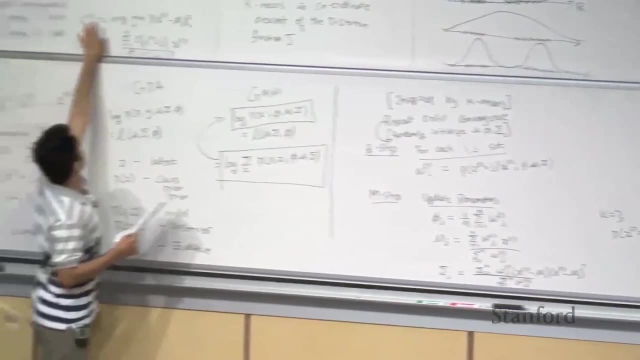 You know, people call it the soft k-means as well. Uh, we call it soft because, um, in the assignment phase in k-means, right In k-means, it was a hard assignment, right? This wa-. this corresponds to the E-step. 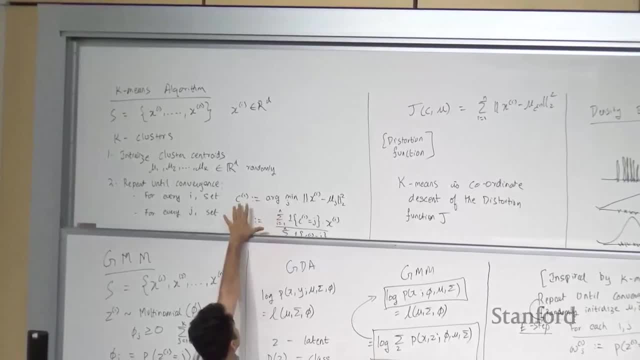 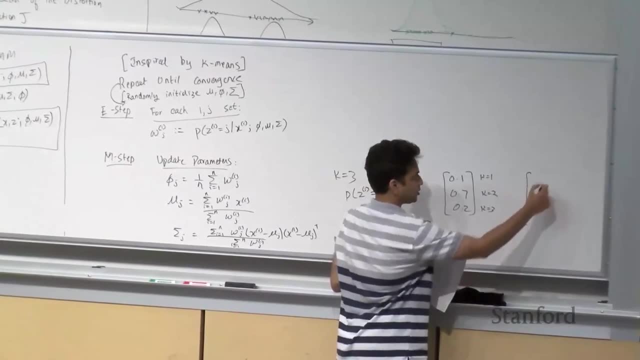 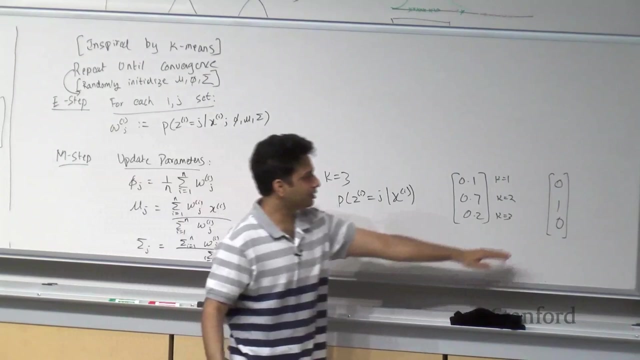 The uh in- in k-means. uh, the cluster identity was a hard assignment. You can think of uh- k-means as a way in which we calculate a posterior distribution which is always one-hot right. If- if uh, if you- if we calculate these kind of posterior distributions. 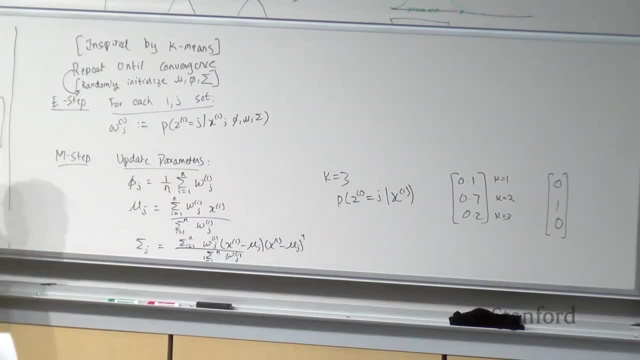 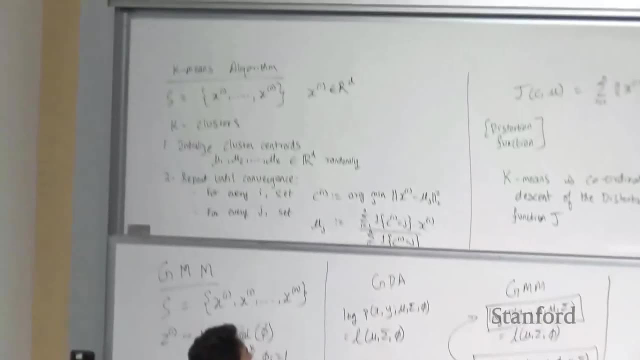 then we effectively get k-means out of, uh, GMMs, right And in the equivalent of the M-step, was the way in which we were recalculating mu's. Uh, the mu j's. we use only those- those. 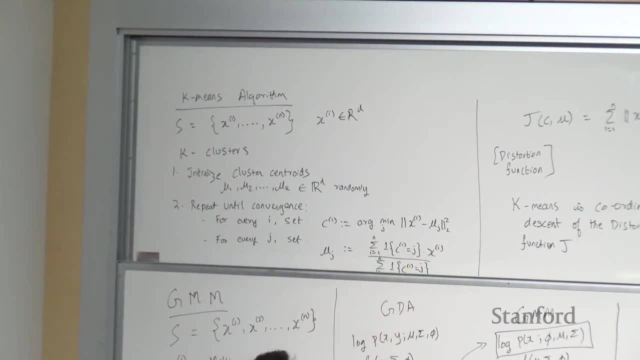 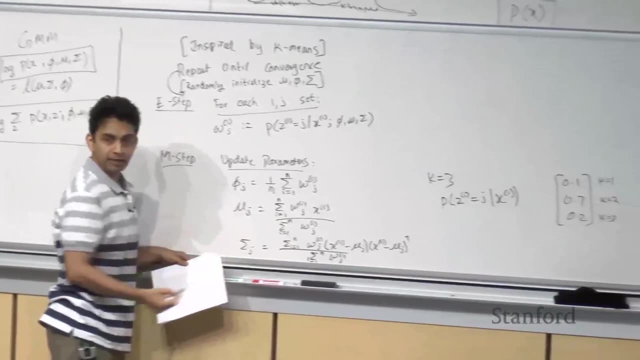 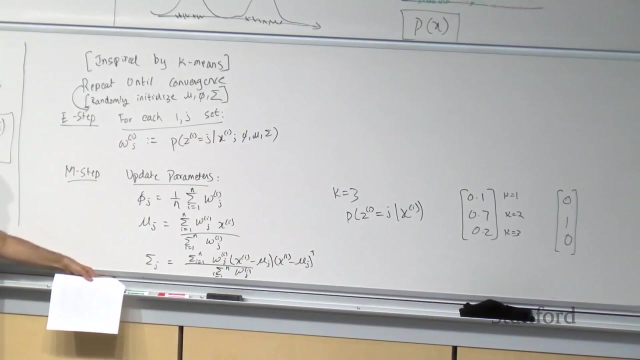 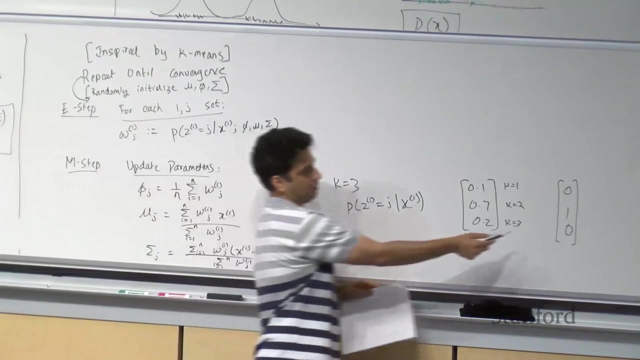 uh x's for which the cluster identity matched the uh uh, the corresponding cluster. And over here, instead of- instead of having uh, an indicator function, we're gonna use this soft assignment weight. Any questions? Yeah, So if- if w's are one-hot. 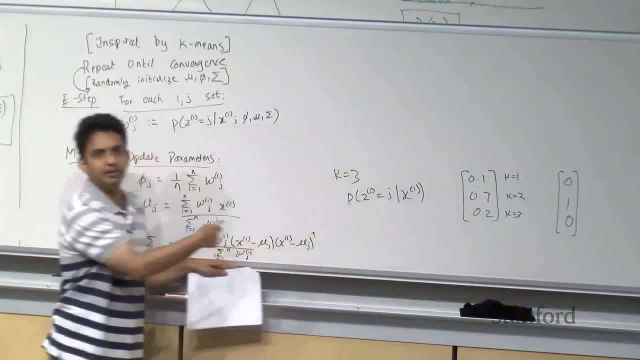 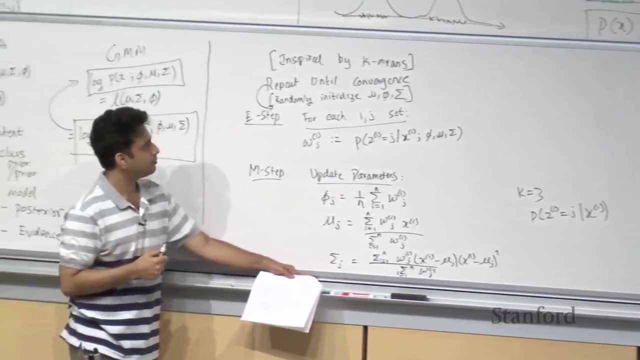 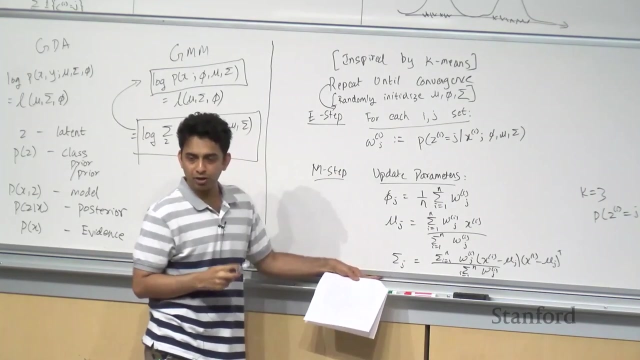 uh, then this- this will essentially be, you know, uh, uh, k-means Yes question. So the question is: how do we calculate w, i, j, f- if we- if we have not observed the i's? 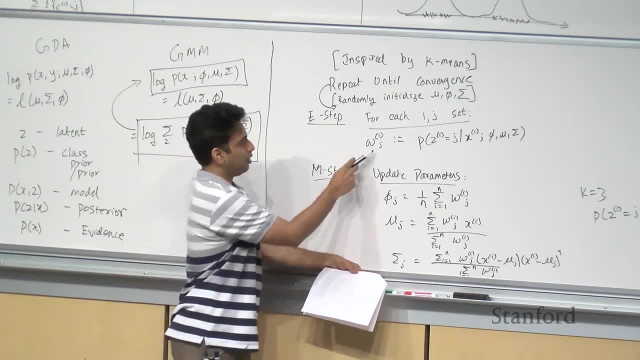 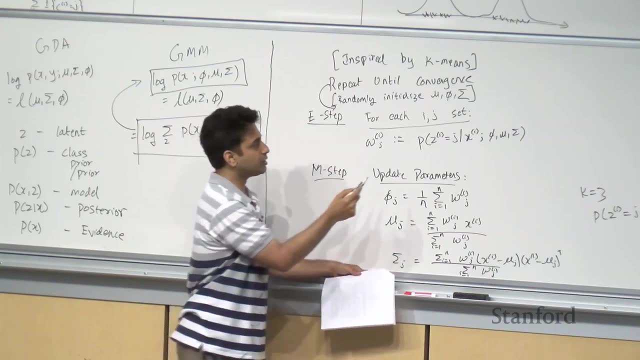 the z's. is that a question? Yeah, So here, uh, in order to calculate this, we don't need to know z i's right, So we don't need to- so we are just uh, cons-, uh, uh. 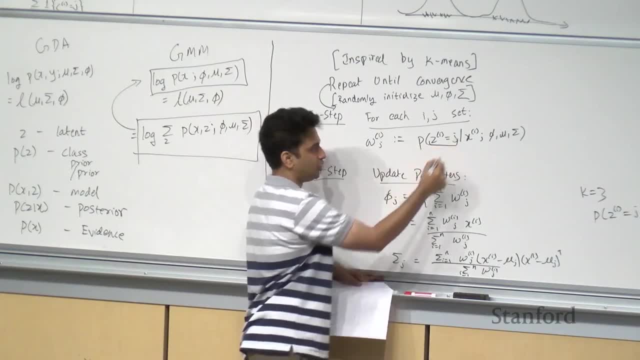 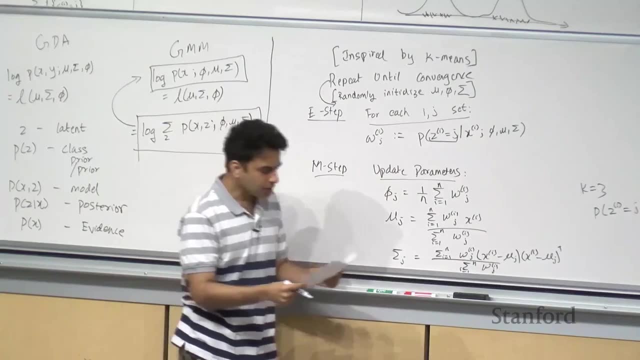 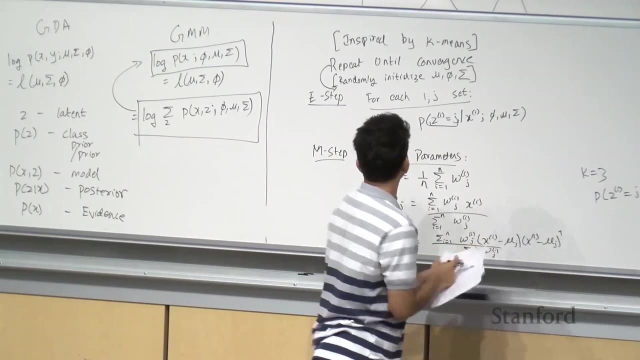 we're just constructing the probability that z i could be equal to j, right, And the way we go about doing this is to use the Bayes rule right, And the way you use the Bayes rule um right. So- and- and this can be calculated as p of you know. 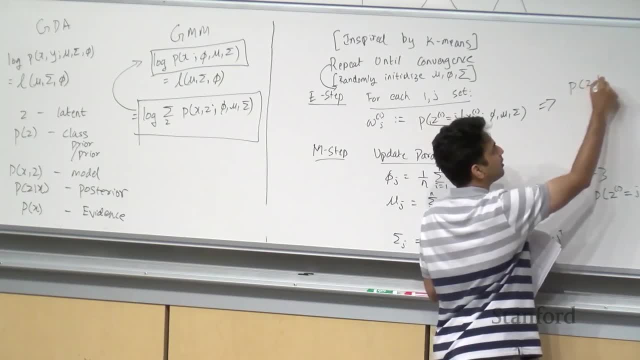 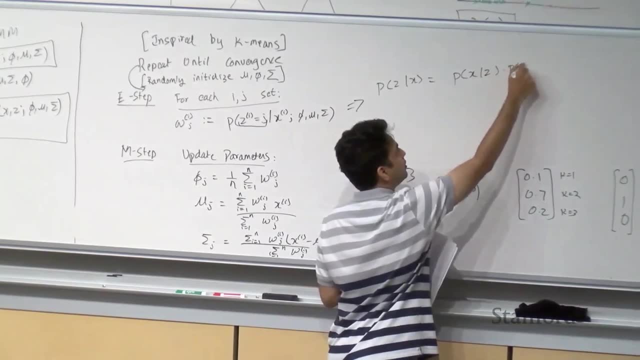 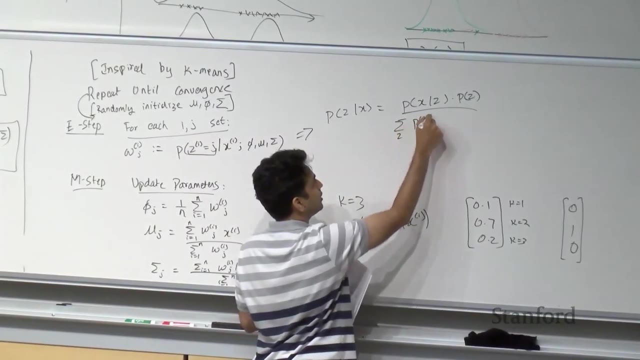 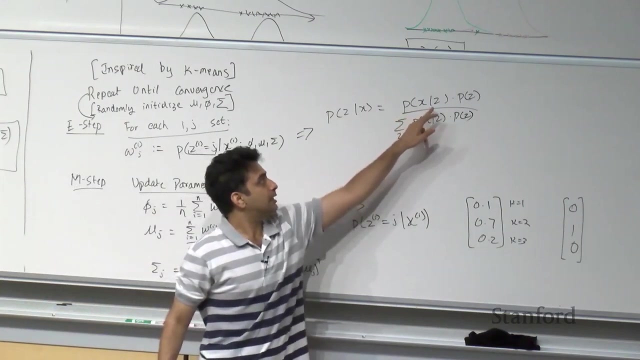 so p of z given x is equal to p of x, given z times p of z over sum over all uh, uh z. p of x given z times p of z. right Over here, p of x given z is: 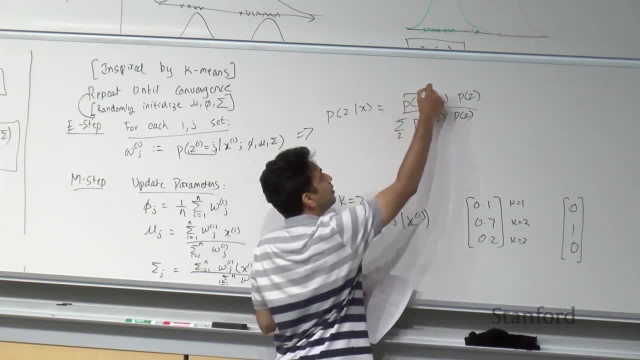 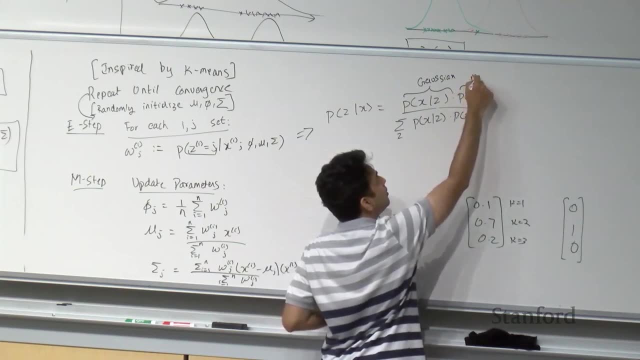 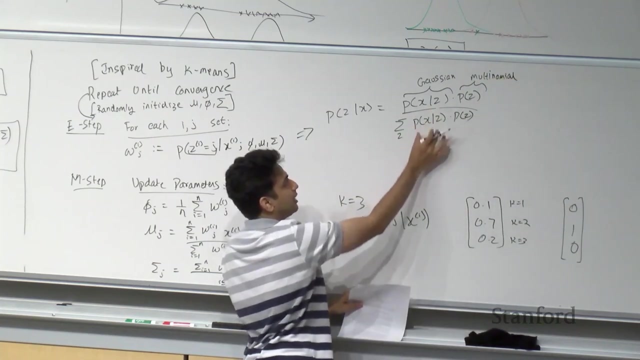 normal distribution. So this is Gaussian right And p of z is just multinomial right And in the denominator, uh, you know, it is same- the- the- the same terms: Gaussian and the multinomial, but you sum it over all the classes. 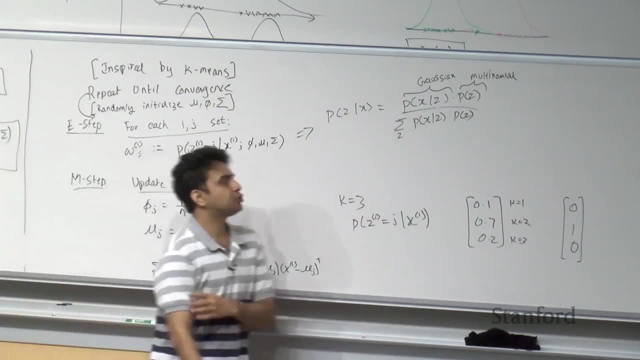 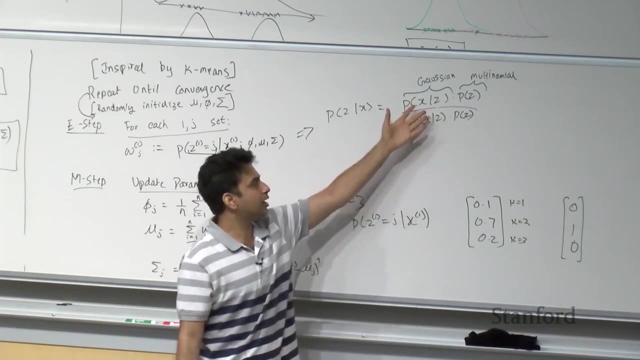 And you will see that. you know, uh, just the way you showed it in homework 1 for GDA, where in GDA this took the form of a logistic uh regression, Uh, here you can actually show that it takes the form of a softmax. 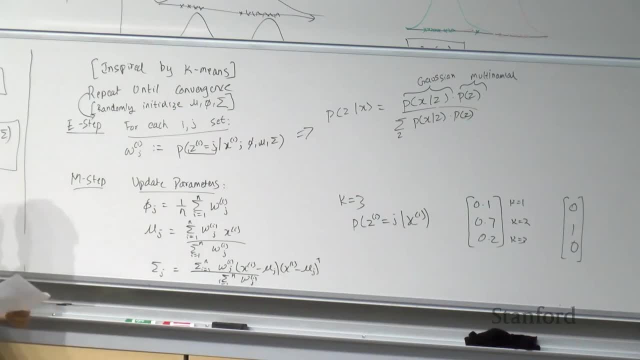 It's- it's very similar calculation. Any questions? Right? Yeah, So this is basically um the Gaussian mixture model, where we derive the steps to be uh, by taking inspiration from k-means right, And we are intentionally giving it the names the e-step and the n-step. 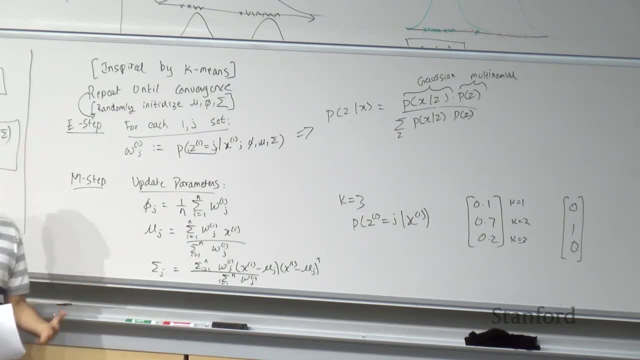 because next we're gonna um, um, talk about the EM algorithm and, uh, we're gonna derive it in a more principled way and we're gonna end up with the same update rules, right, And this is um you know. 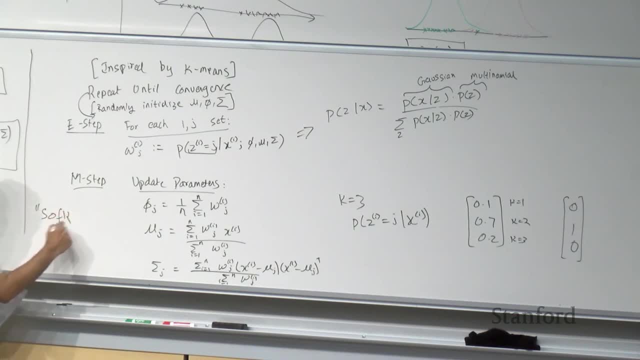 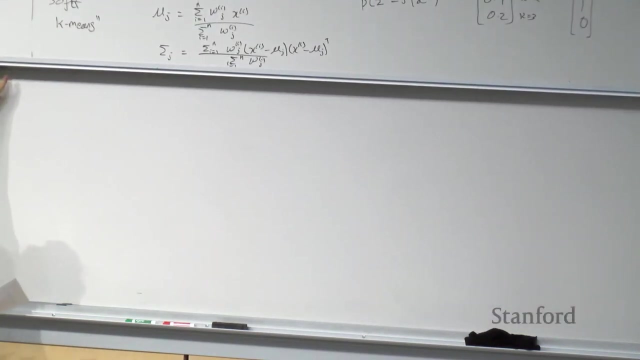 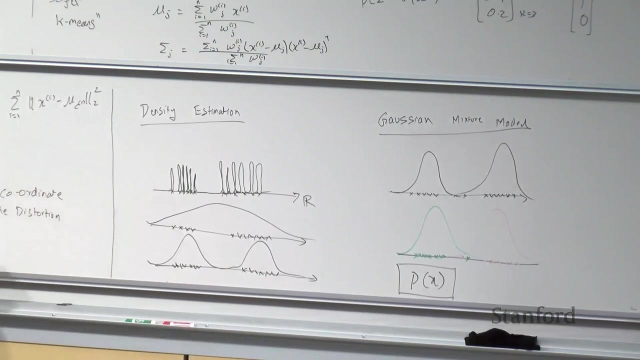 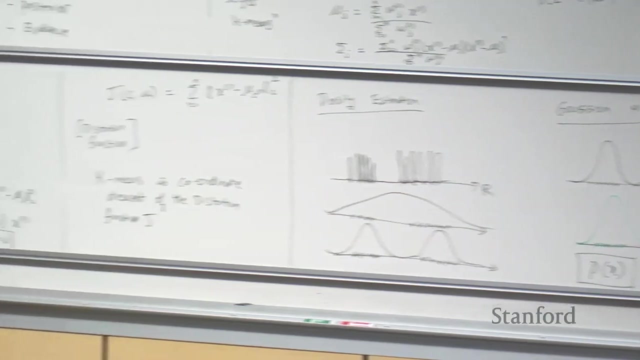 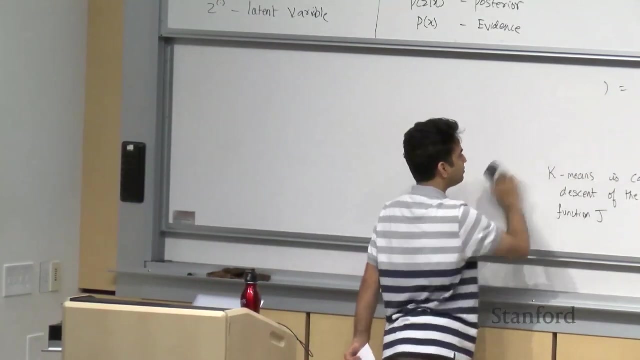 think of this as soft k-means. soft k-means Right. and now we're gonna switch gears and talk about the EM algorithm. So the EM algorithm is also called the Expectation Maximization Algorithm, That's an algorithm where it gives us. 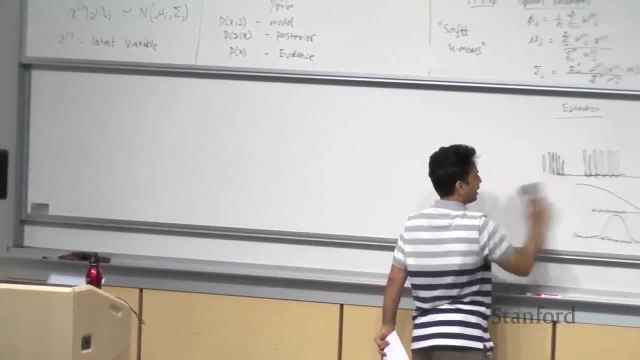 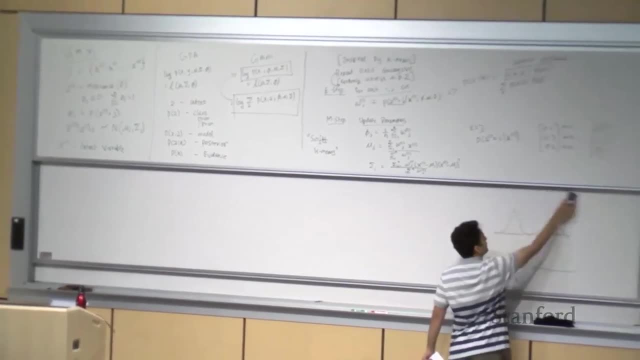 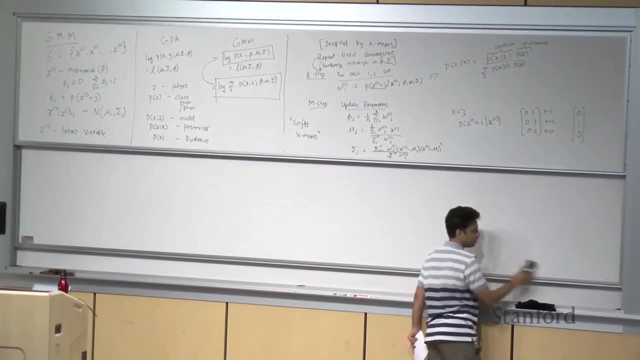 a framework of maxi- of- of performing maximum likelihood estimation when some variables are unobserved. right It is- it-, it-. it is used in cases where we have a functional form for the joint P of x comma z, and x and z could be anything. 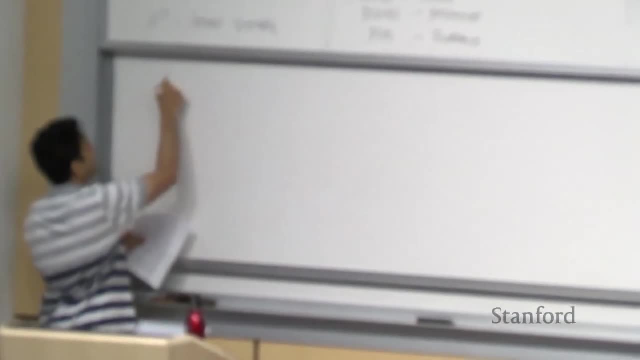 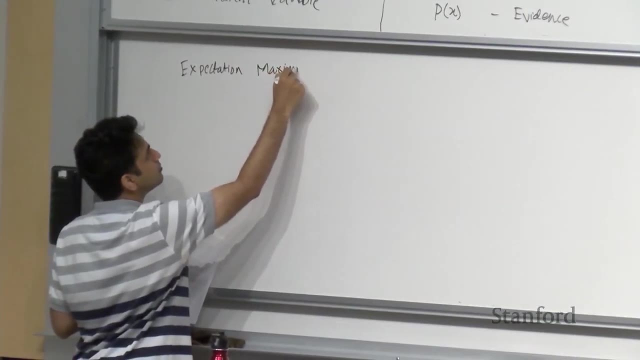 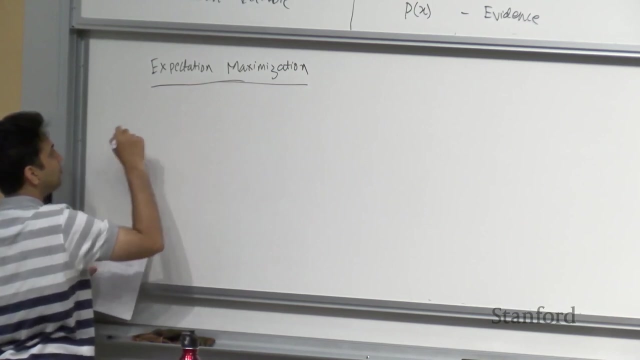 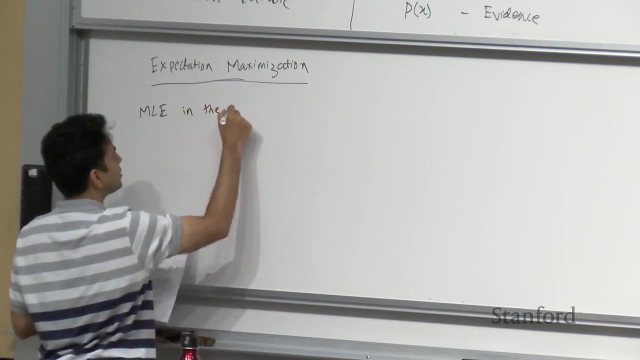 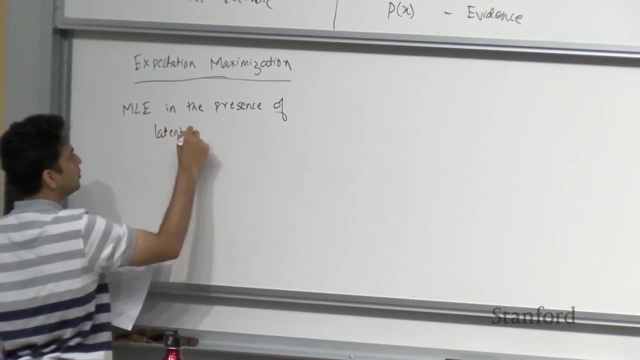 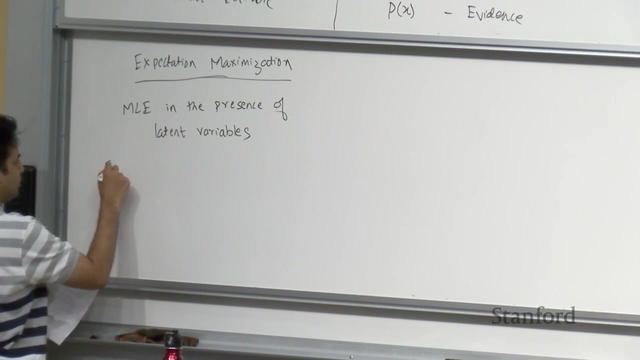 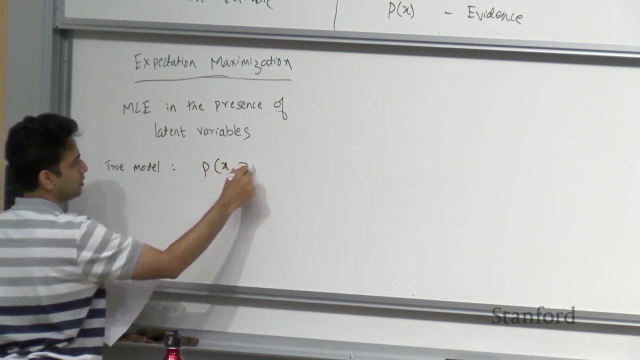 but z's are not observed. So expectation maximization Right, Expectation maximization is an algorithm where we perform MLE in the presence of latent variables right. So where the true model is P of z, of x, comma, z, with some parameters, theta. 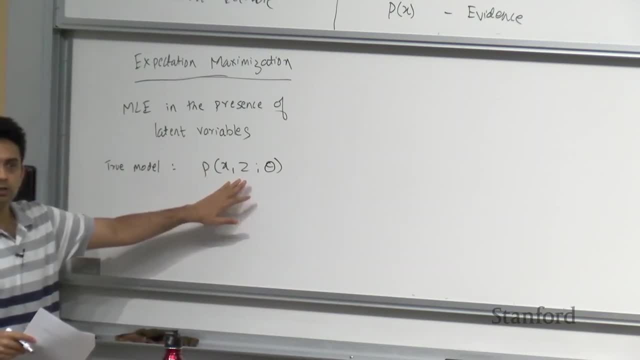 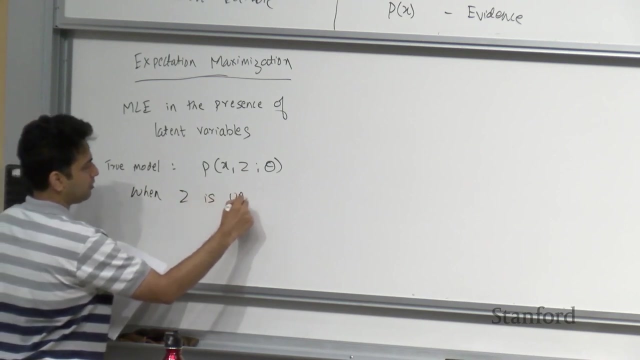 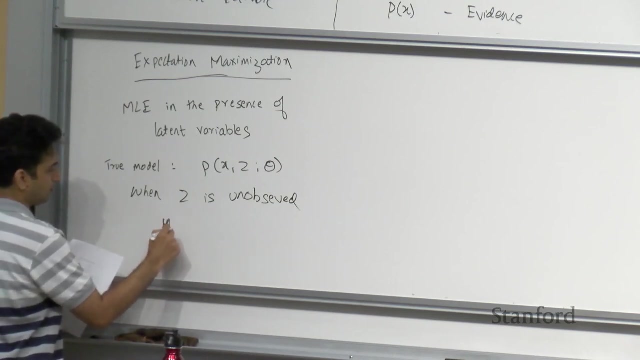 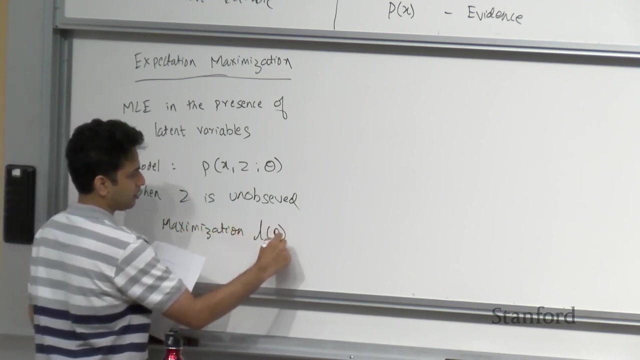 And if we observe x and z jointly? if everything is observed, then the problem is very simple. We perform simple maximum likelihood estimation, But when z is unobserved, we want to instead perform maximization of the objective. L theta equals log P of x. 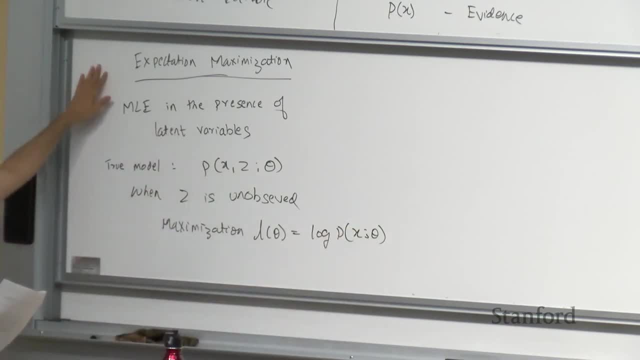 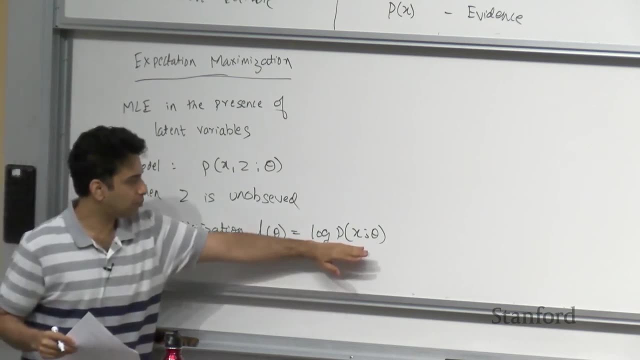 where z is marginalized And the EM algorithm or the EM framework gives us a framework for achieving this, where we maximize log P of x in an indirect way rather than directly, uh, taking the derivatives and setting them to 0, and so on. 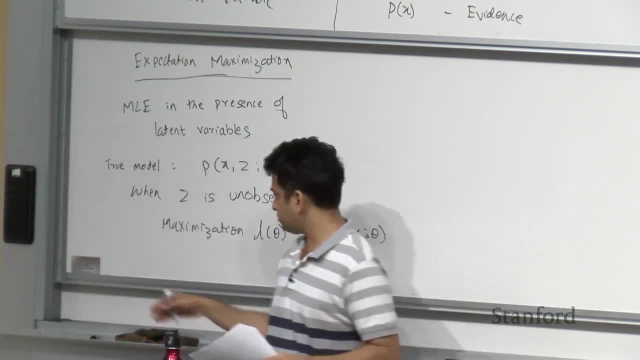 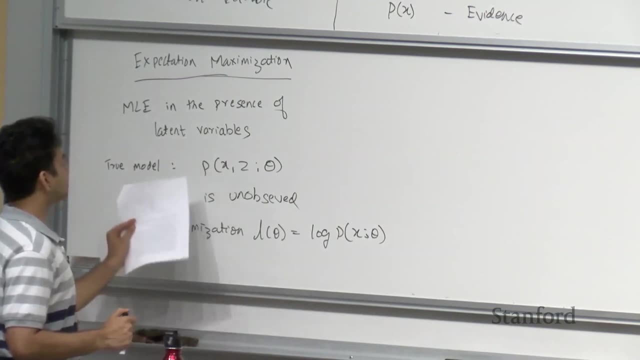 Now, before we go into uh, the EM algorithm, some kind of uh it- it can be useful to have some kind of a context here. So the EM algorithm was- was uh uh discovered some- sometime in the. 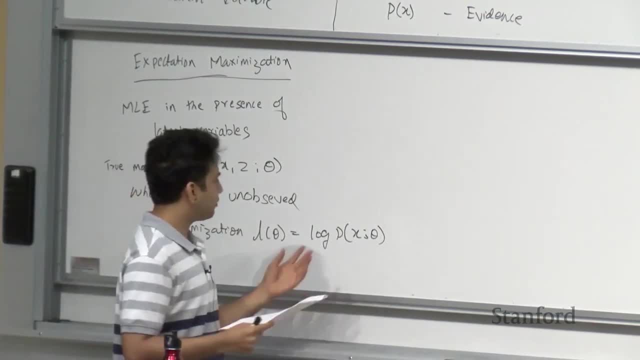 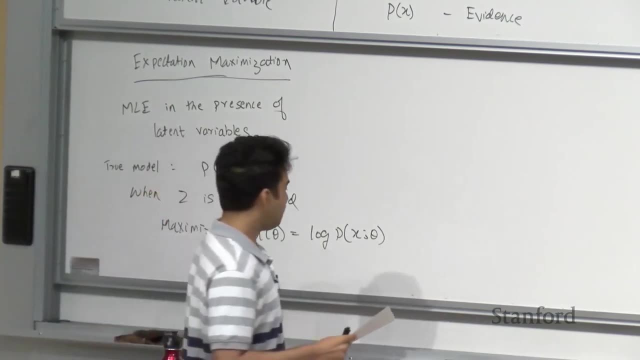 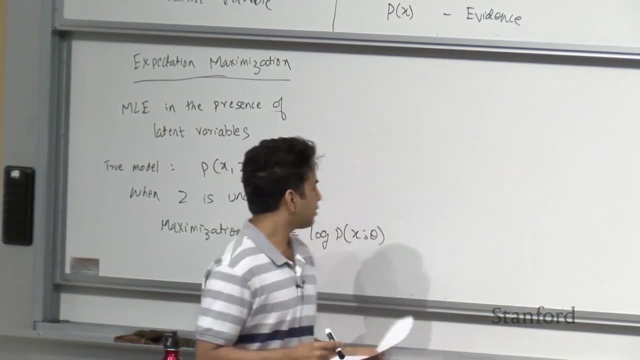 I think, early 1970s, where- uh, you know where- where people were trying to uh perform MLE in the presence of unobserved- uh, uh, unobserved- data. And it so happens that this- this framework, is so general and so powerful that there are- it has 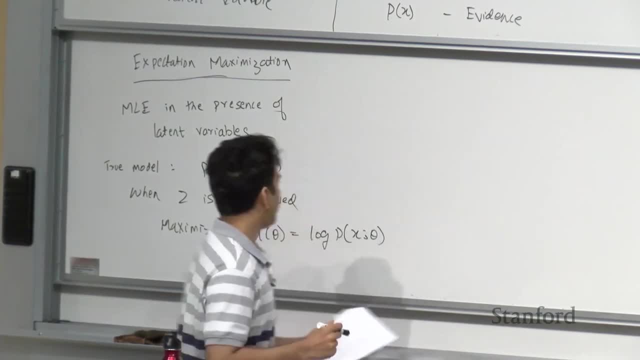 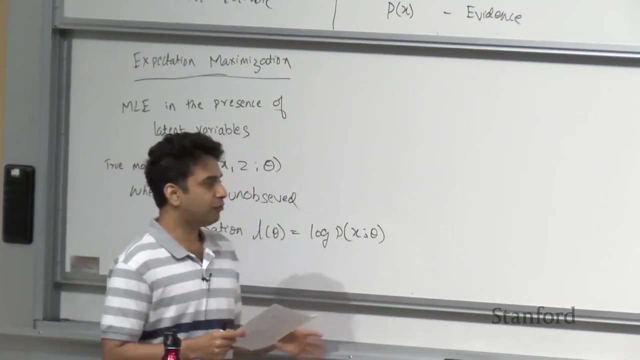 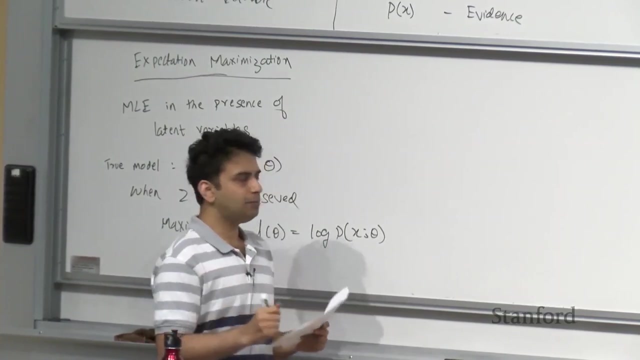 it has been adapted in so many different ways And it has been, uh, you know, minor extensions to the EM algorithms. uh, are there in so many different forms, But this framework is- is somewhat central, and understanding EM in a deep way will be extremely useful. 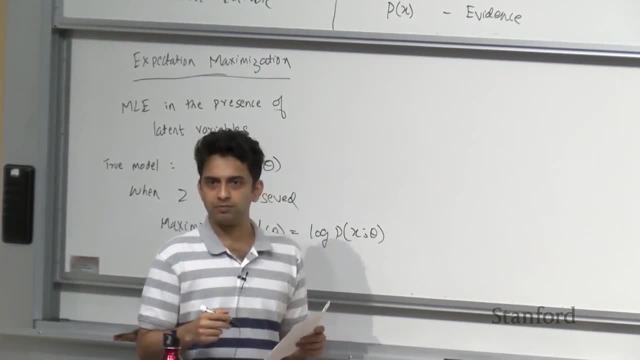 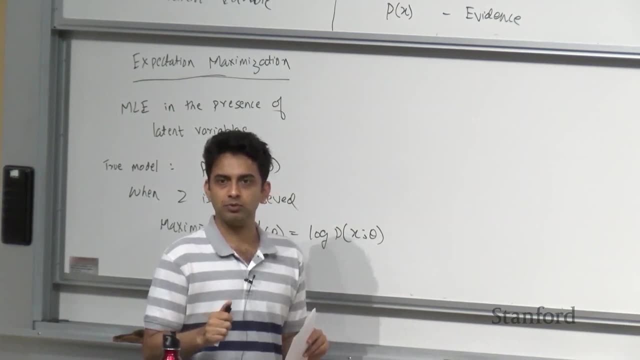 if you are interested in things like deep generative models, right, So in- in um. over the last few years, there has been, uh you know, tremendous growth in deep generative models. uh, where um you might have heard of? 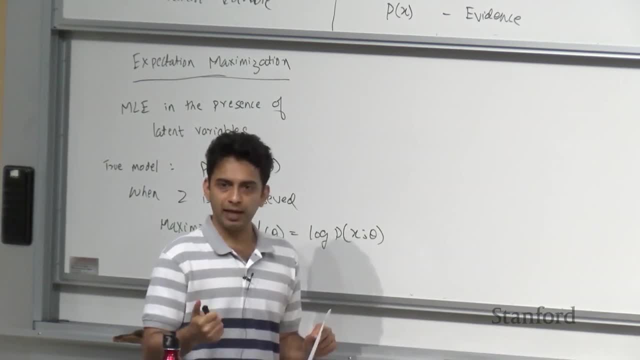 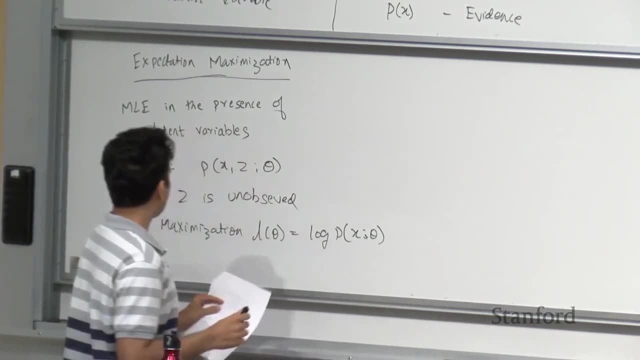 you know variational autoencoders, generative adversarial networks or GANs, or flow-based models, glow-based models, and all of them. understanding all of them would be a lot- much easier if you really understand the EM algorithm well. 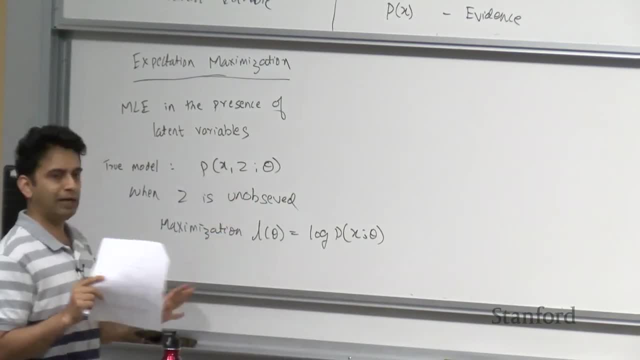 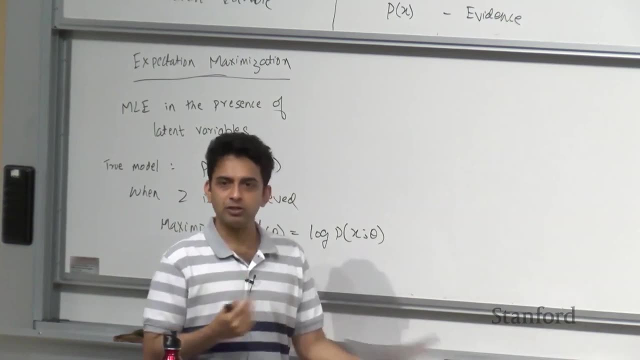 because the EM framework gives you a kind of a mind map where you can place all these different algorithms and kind of understand the strengths and weaknesses and- and you know what's common between them, what's different between them, and so on. 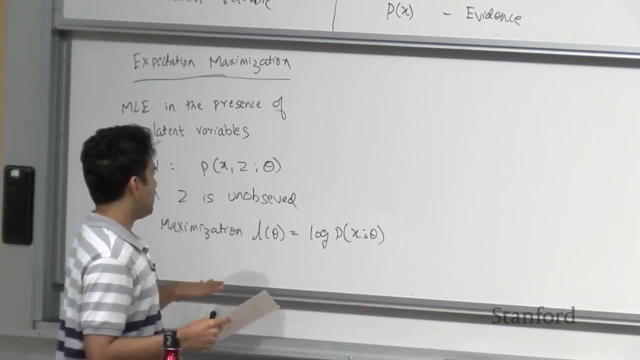 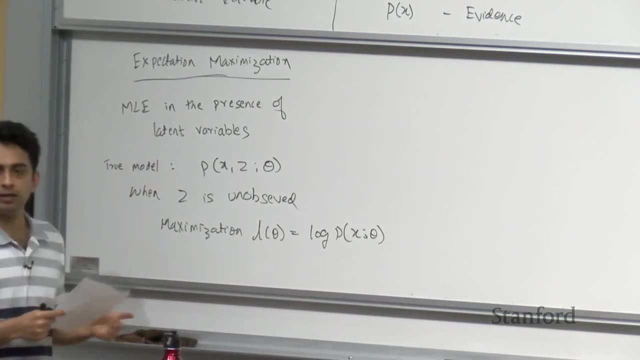 So EM algorithm is- is um one of the key algorithms to um for- for even modern, um um um deep learning or deep generative, um um um deep generative models, right. 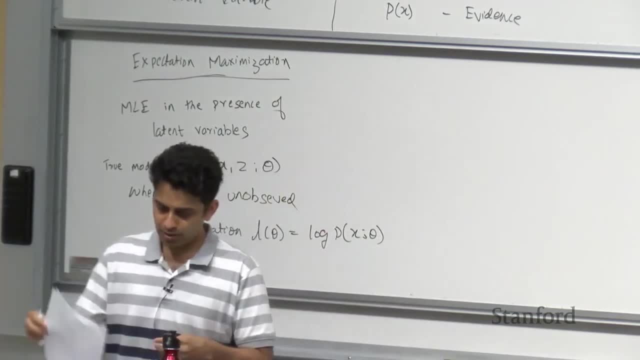 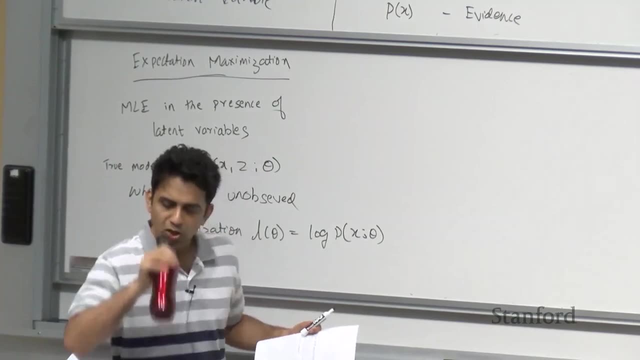 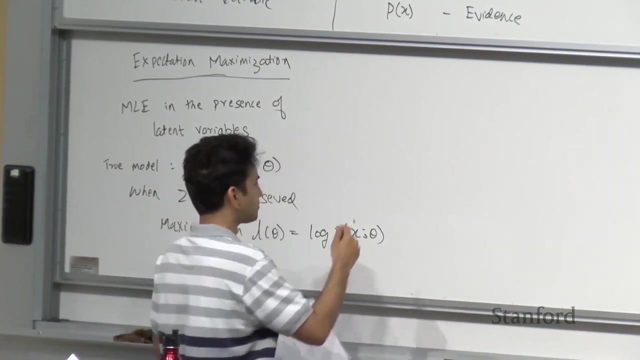 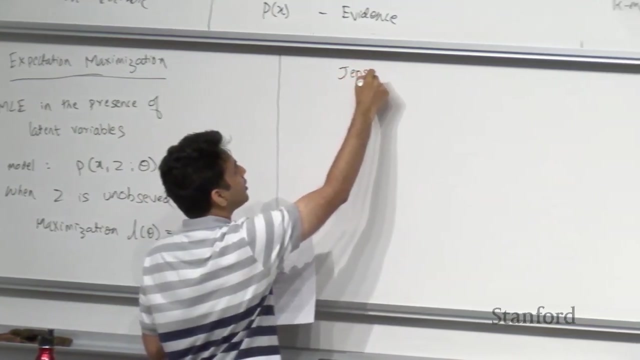 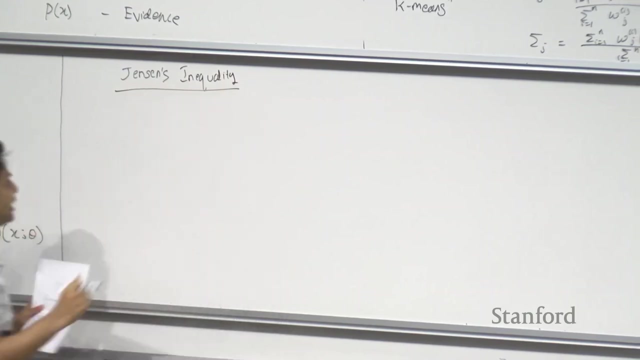 So before we jump into EM algorithm, we're gonna first look at something called as Jensen's inequality. So Jensen's inequality is a- is a very general probabilistic inequality that's used, you know, in- in very many places in probability theory and applied probability theory. 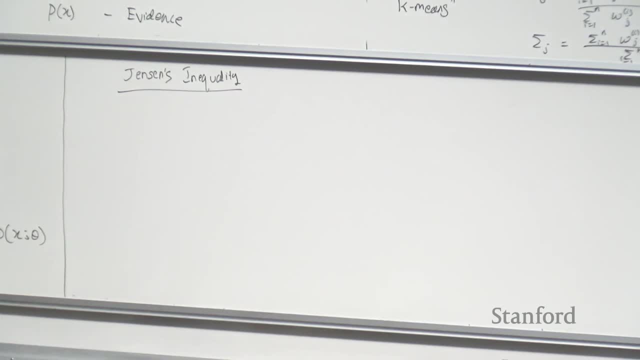 And it will show up in- in our derivation of EM algorithm as well. So you can think of Jensen's inequality as a um probabilistic tool that we will use in deriving uh EM. But Jensen's inequality by itself is-, is- is a very generic and 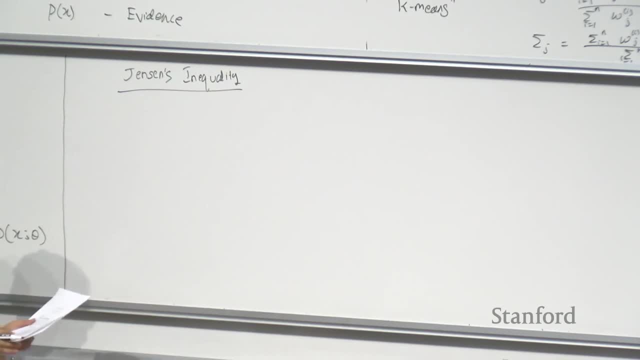 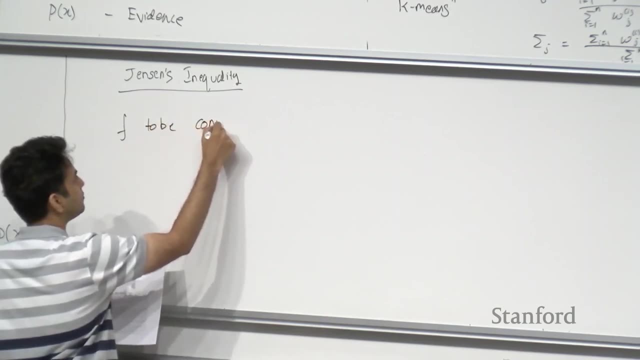 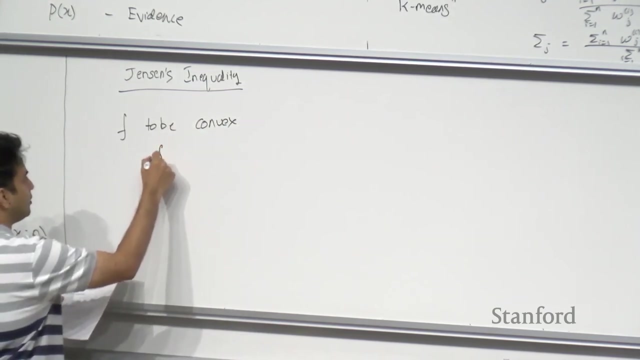 you know, commonly used inequality in- in uh probability theory. So let's- let's assume a function, f, to be convex right. Assume f to be a convex function, which means um f double prime of x is greater than equal to 0,. 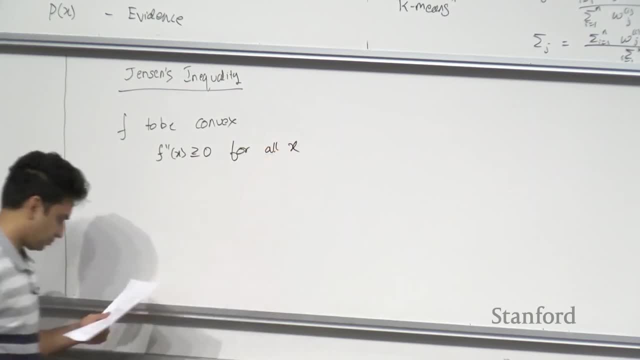 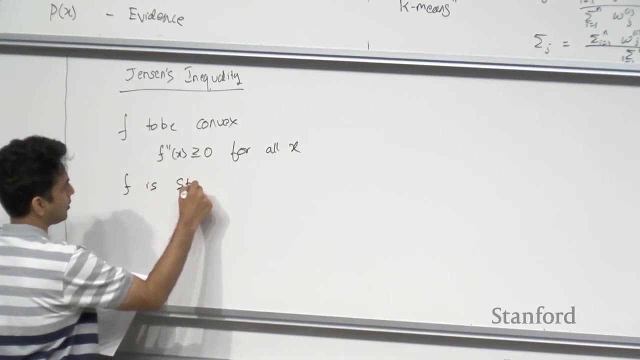 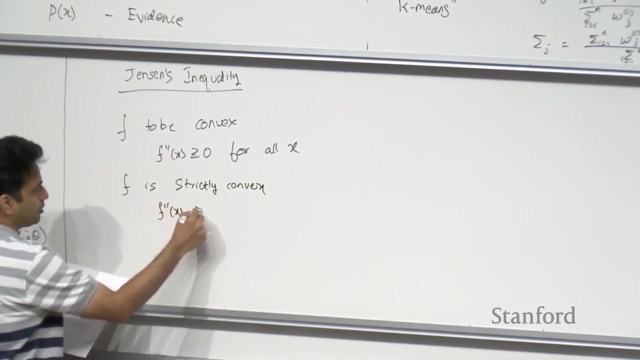 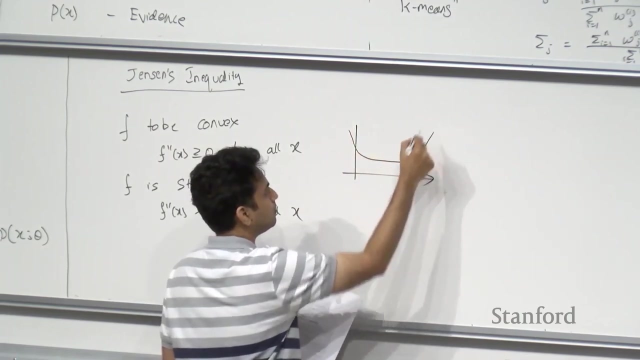 for all x, right. And we say that f is strictly convex if f double prime of x is greater than 0. for all x, right. So the, uh, the mental picture to have is f of x and this is x. 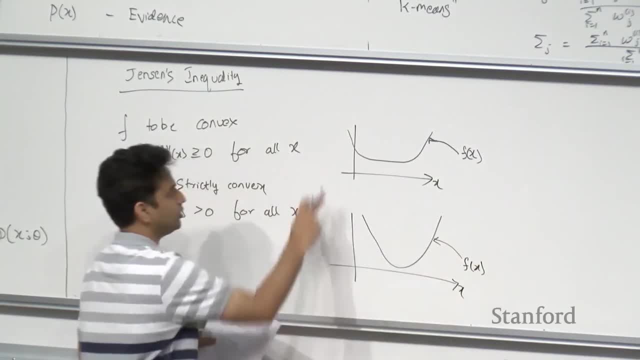 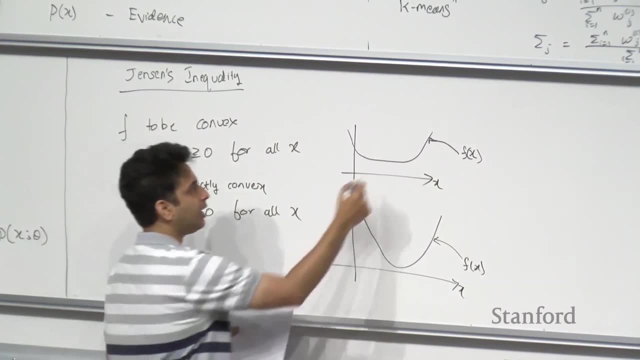 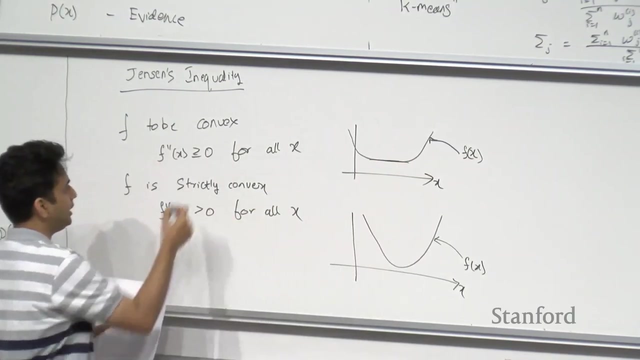 f of x and x. So this is an example of a convex function. Convex functions are bowl-shaped functions, right, And they can have a 0 second derivative in a few places where f, prime of x, uh is greater than or equal to 0.. 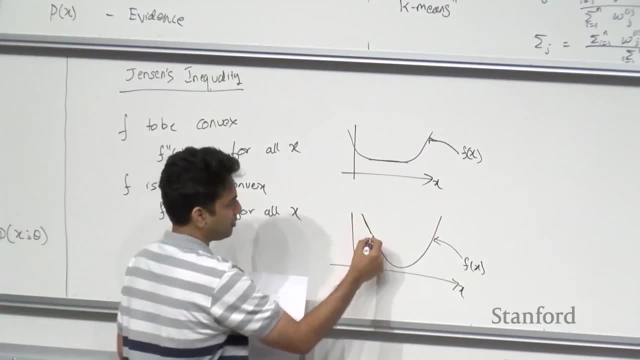 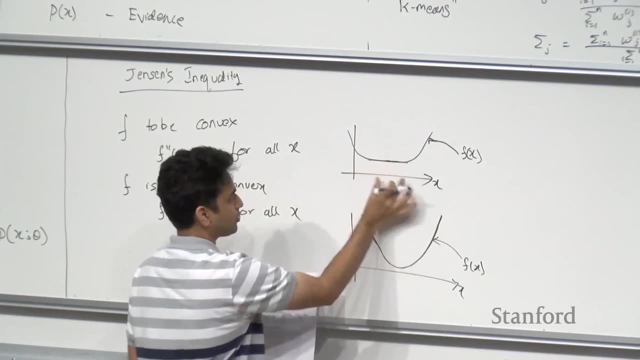 But in a strictly convex function the second derivative is never exactly equal to 0. It's always greater than 0. So if there are straight lines for- for certain input ranges in your functions, then it can still be convex. But uh, for a strictly convex function. 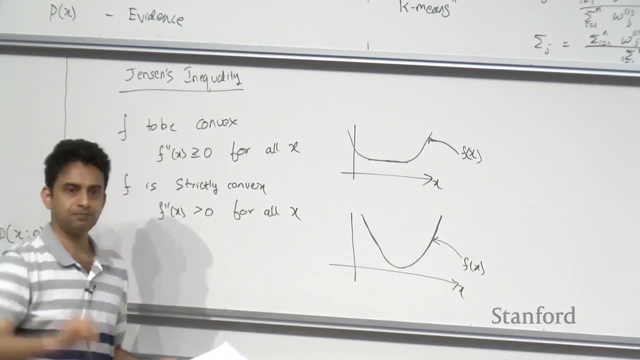 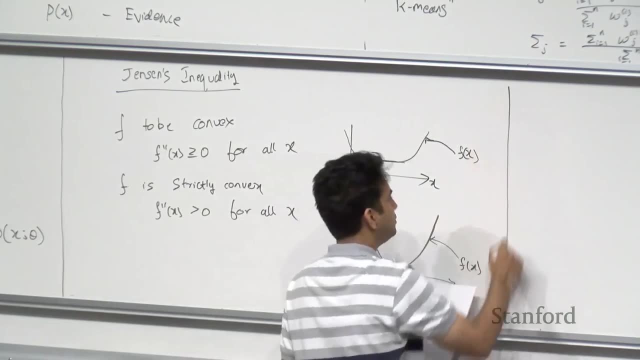 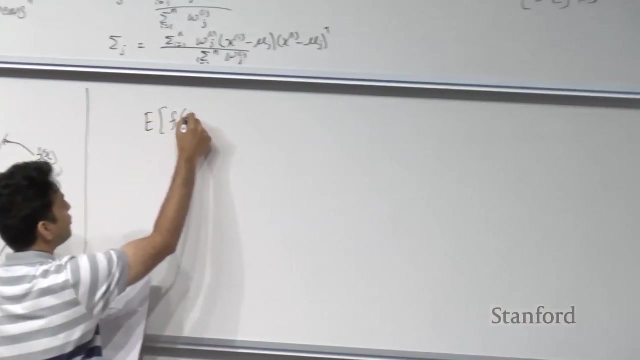 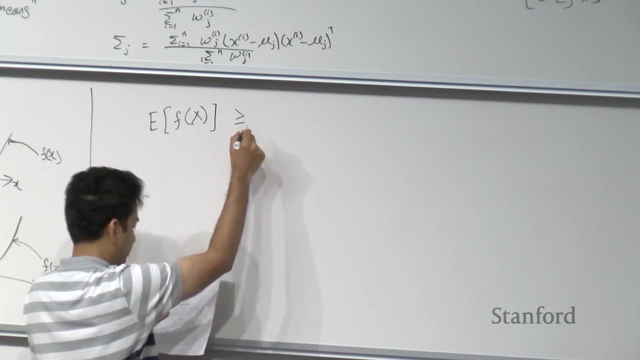 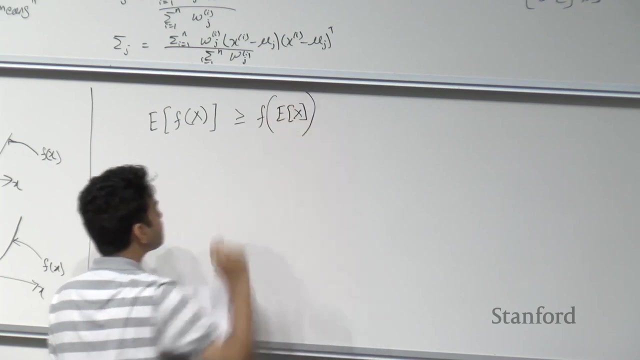 there cannot be straight lines, right, It should always be curving upwards, right Now? the Jensen's inequality tells us um that expectation of f of x, where x is some random variable, is always greater than or equal to f of expectation of x. 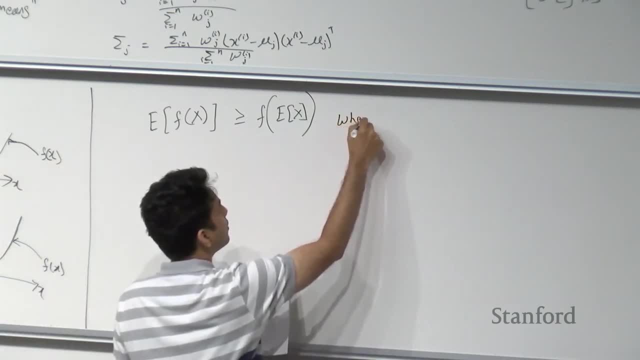 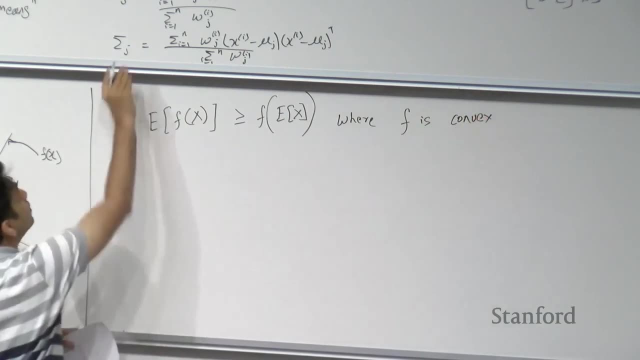 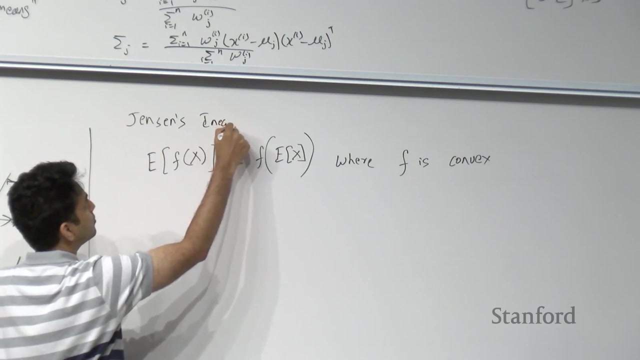 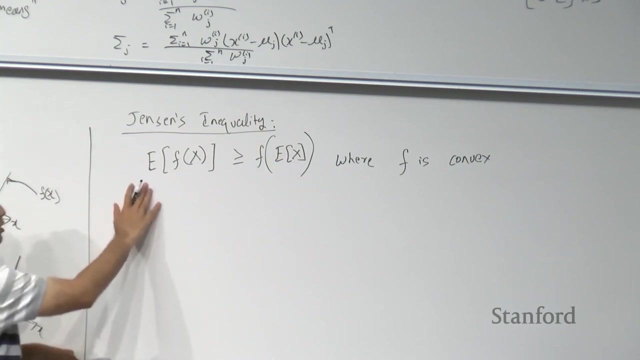 Where f of expectation of x, where x is a random variable, it is always greater than or equal to 0,. Okay, So is convex. So this is Jensen's Equal. So the Jensen's inequality tells that the expectation of f of x. 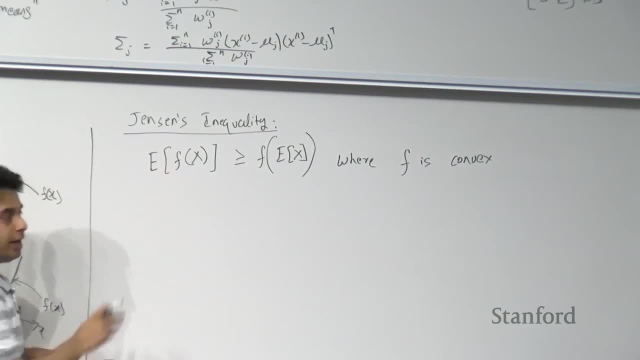 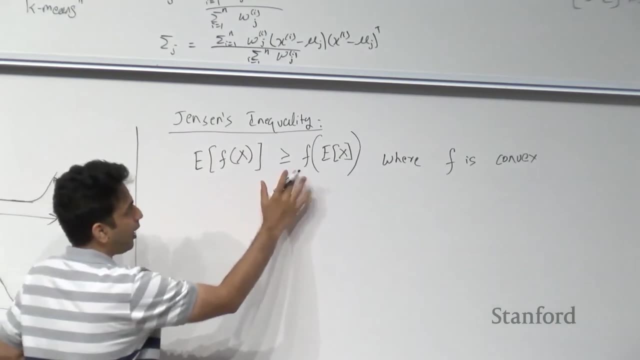 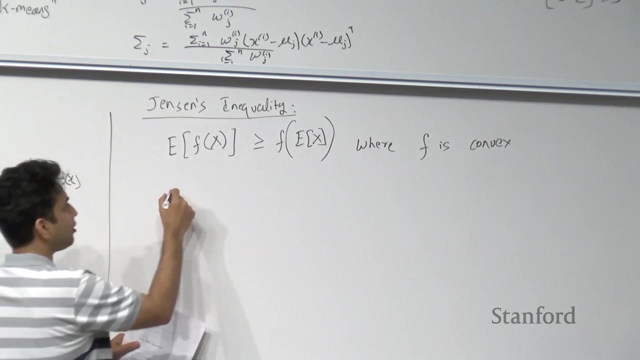 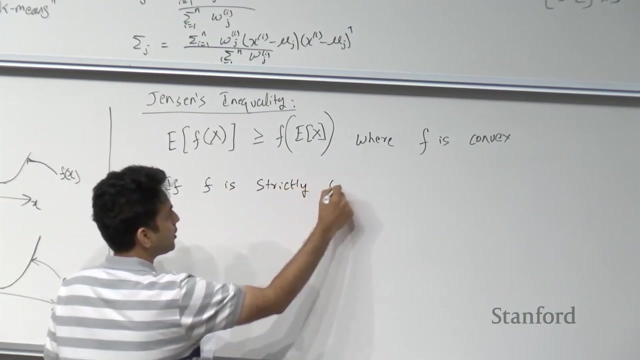 where f is a convex function and x is a random variable and the expectation is taken with respect to the randomness in x will always be greater than or equal to f of the expectation of x right And, moreover, if f is strictly convex- strictly convex. 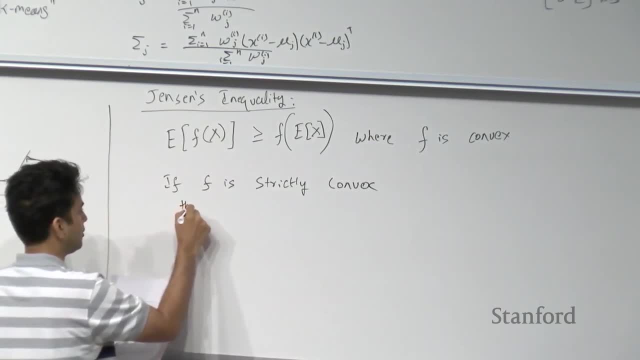 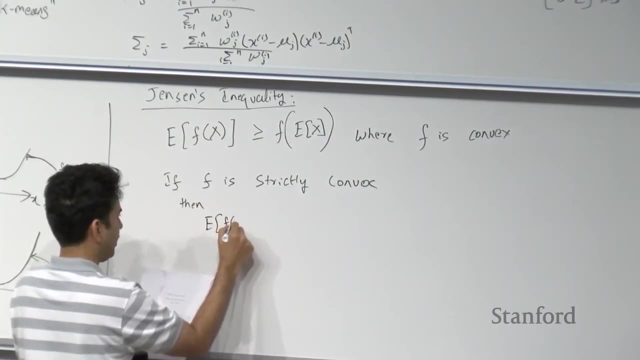 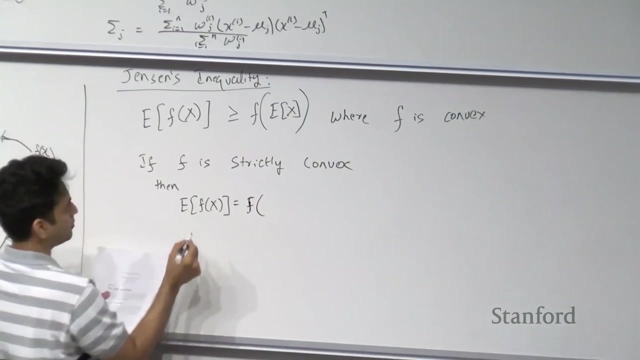 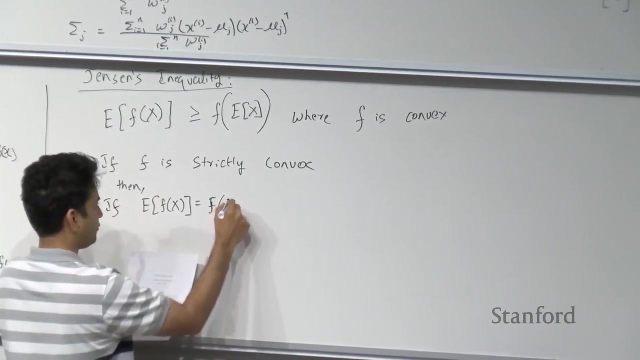 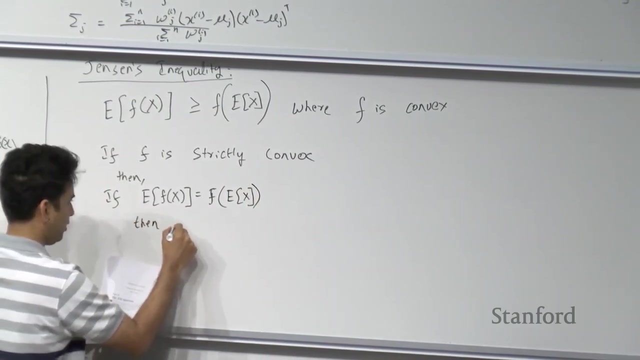 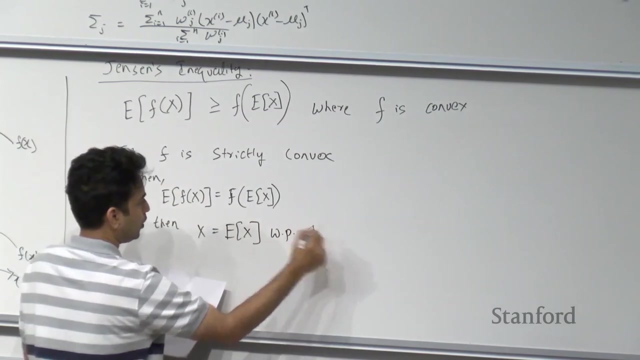 then expectation of f of x equals f- if then, then if expectation f of x equals f of e of x, then x equals expectation of x with probability 1.. There's a lot of jargon here. We'll- we'll uh, dissect it in a moment. 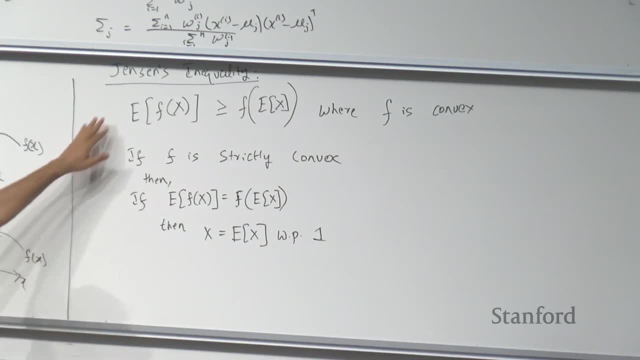 So to uh, just to restate it again, Jensen's inequality says: if f is a convex function and x is any random variable, um, then expectation of f of x is greater than equal to f of expectation of x. And, moreover, if f is strictly convex, 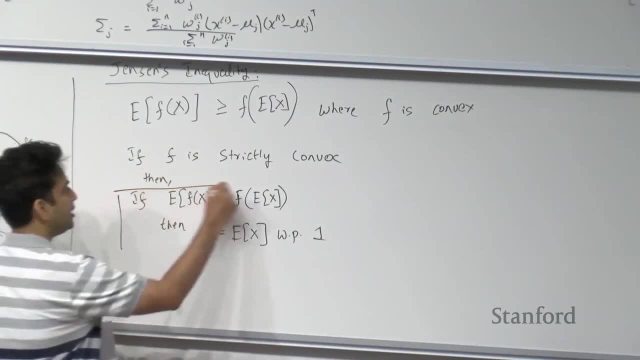 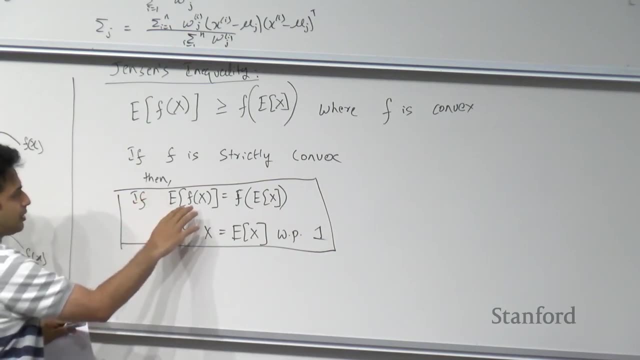 then this statement holds true. And this held statement holds true only if f is strictly convex. Now if expect- the- the statement is: if f of x equals- uh, expectation of f of x equals f of expectation of x, then it must be the case that x equals expectation of x with probability 1,. 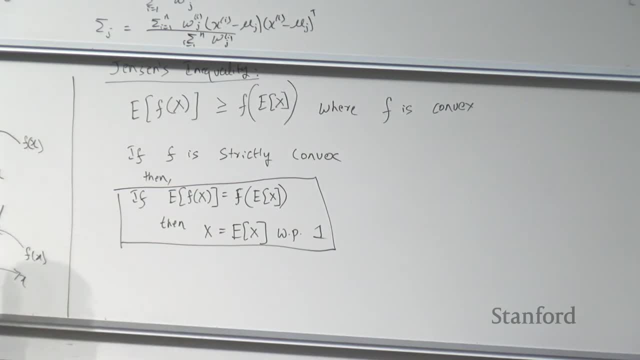 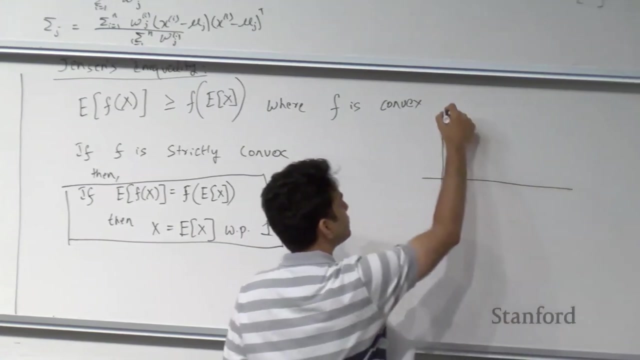 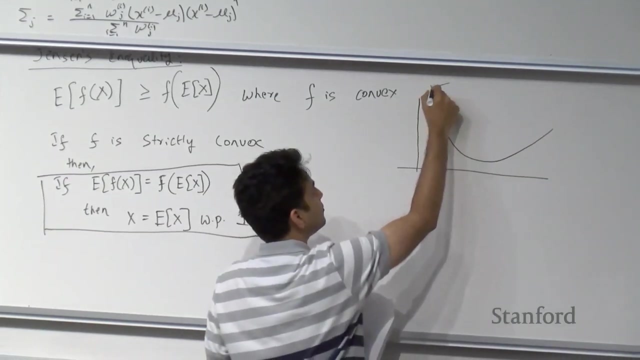 which means essentially x is a constant right. Now, what does this mean? Um to- to kind of understand this more intuitively, now this- this picture can help. right, Let this be some function: um f of x, right. 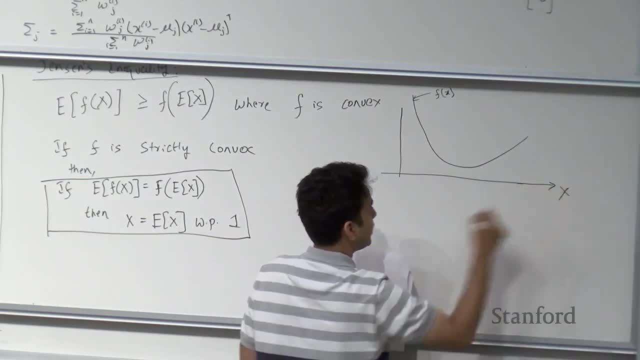 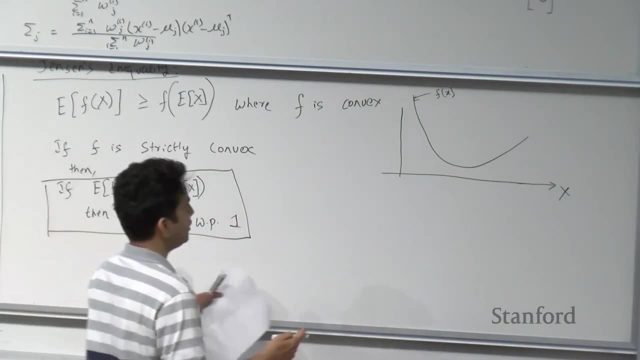 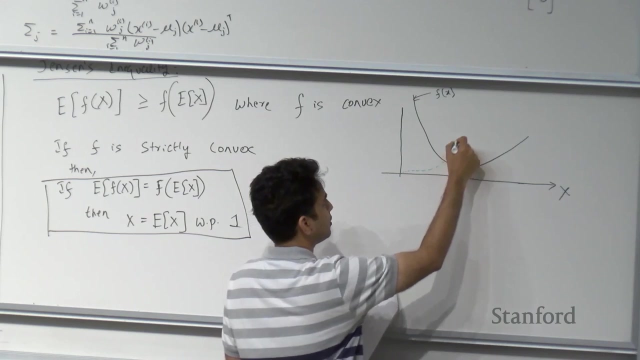 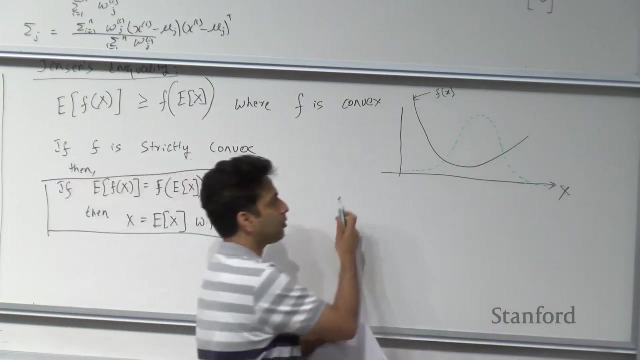 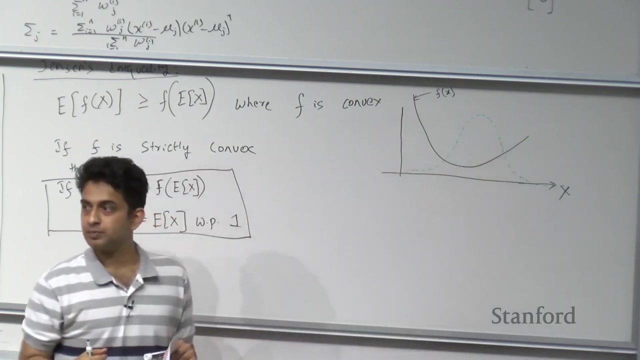 And this is basically x, right, And use a different color here. Let's also assume that x is- has a probability distribution associated with it, right? So the green dotted line represents the probability density of- of the random variable x, and f is some function of x, right? 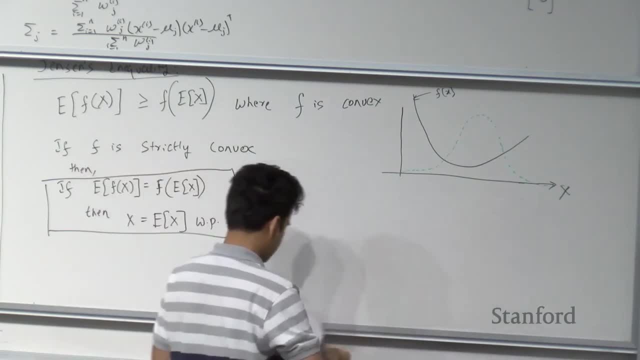 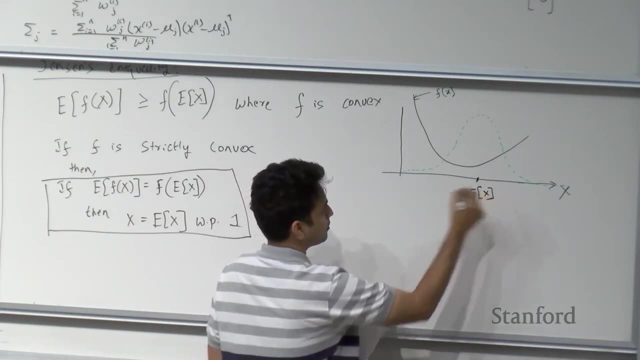 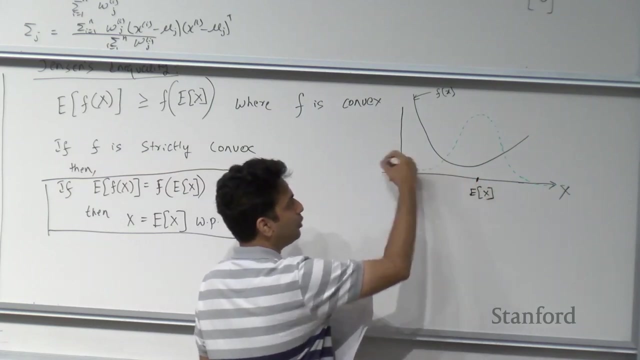 Now expectation of x or e-- uh would be somewhere here, So let's call this expectation of x, right. So expectation of x is- is um-. so think of it as like the mu if this is a Gaussian right. 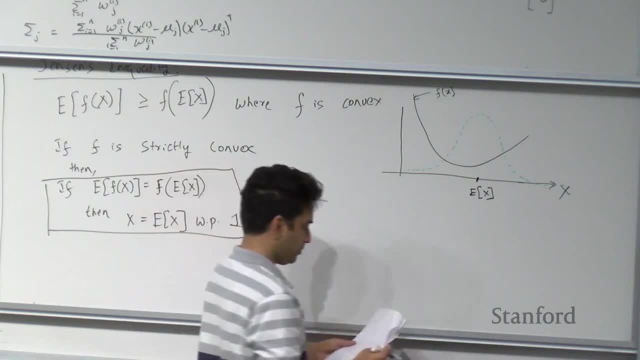 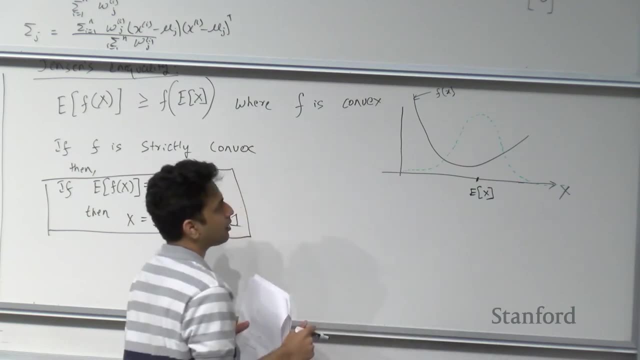 That's the expectation of the random variable right. And now um f of expectation of x, So um in- in- in the case where x- uh, let's assume x- takes only two possible values, So let's assume um-. let's draw another picture here. 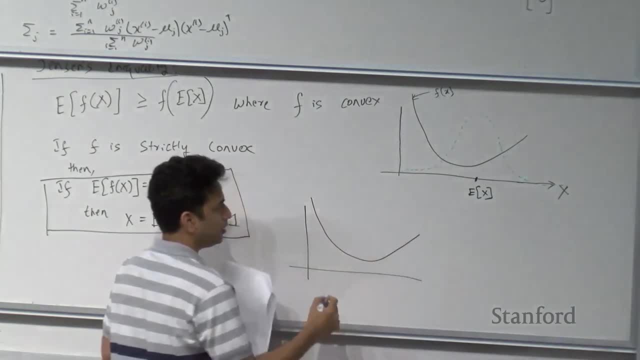 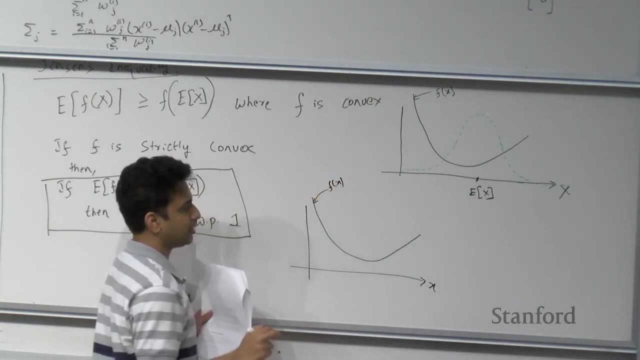 So this is x, this is f of x. Let's assume x takes only two possible values. Let's assume it's a discrete distribution. Here, we-, we-, we- we. uh, here x was continuous. but to understand Jensen's inequality, 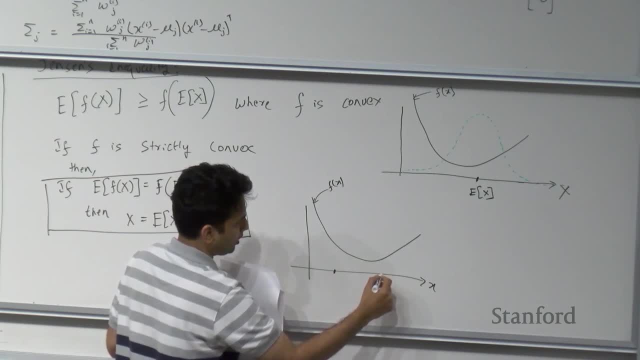 let's uh assume, uh, a discrete uh setting, where x takes only two possible values: this value and this value. Maybe they are, you know, 0,, 1,, 2,, 3,, 4,, 1, and 10.. 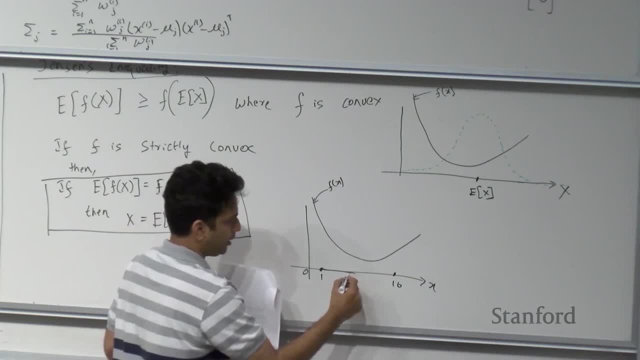 Let's assume te- x takes any one of these values And the mean of x. if it takes, uh uh, with probability half the value 1 and its probability half the value 10, then expectation of x will be 5.5, right. 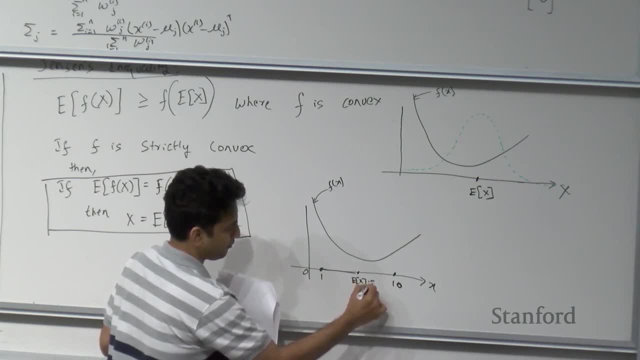 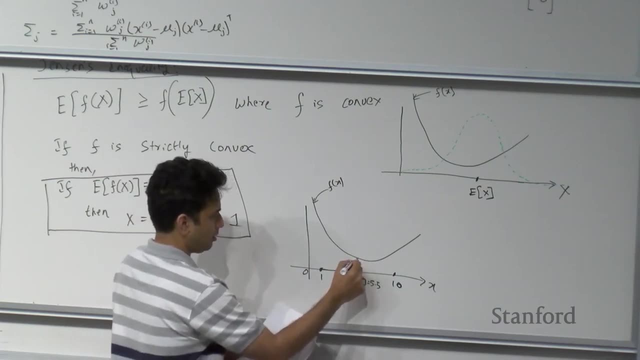 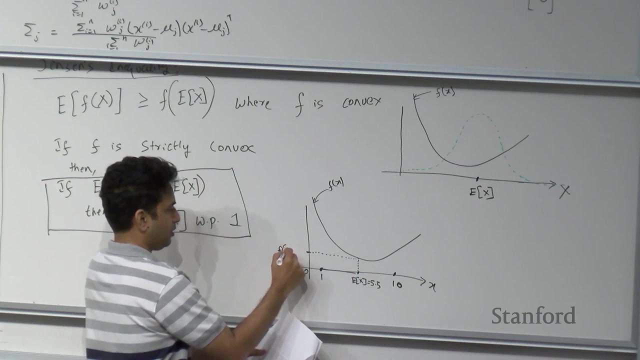 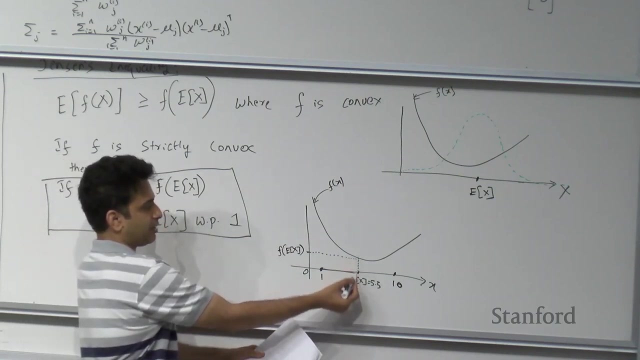 So expectation of x equals 5.5.. Is 5.5?? Yeah, 5.5.. And this over here is f of expectation of x. Okay, Does that make sense? This is the expectation of x. You evaluate f at expectation of x and you get f of expectation of x. 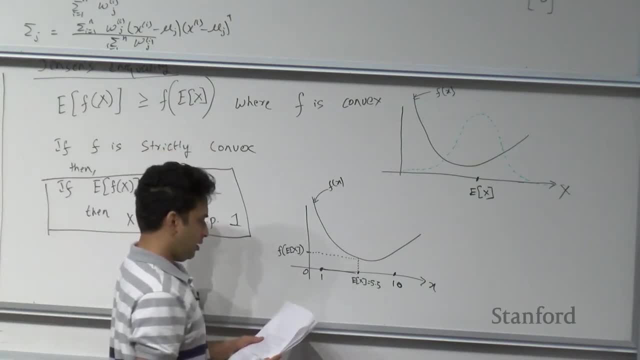 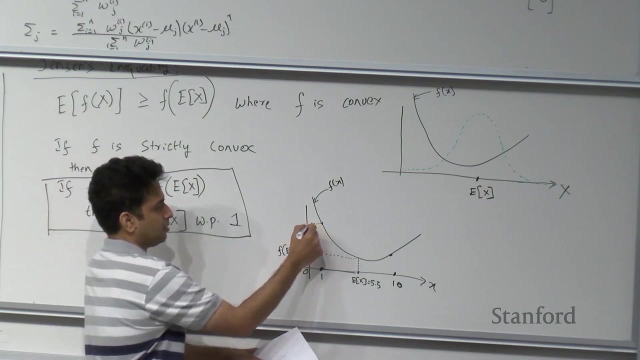 That's the uh, right-hand side right Now. similarly, um, with probability half f of x- can- takes this value, and with probability half another half f of x takes this value right. So this is- let's call this a and b. 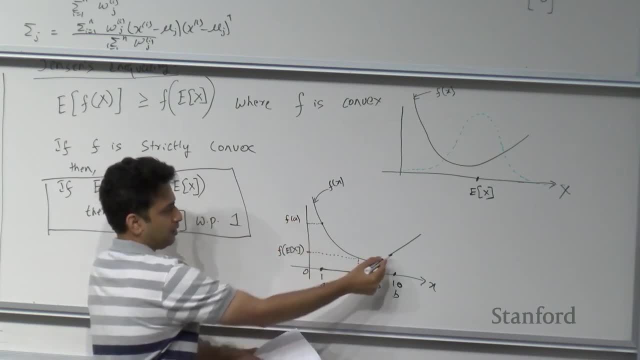 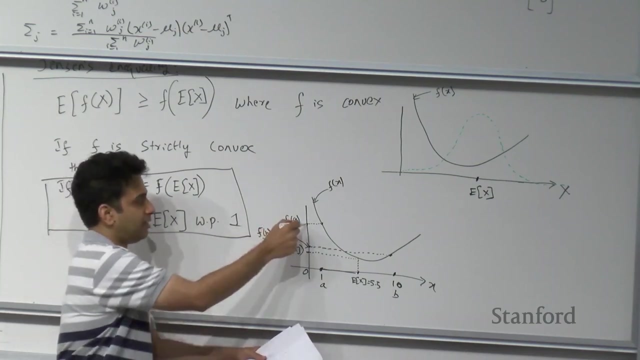 So this is f of a and this is f of b. Right, And expectation of f of a and f of b is basically the midpoint between f of a and f of b. right Because with probability, half it takes this value. with probability half it takes this value. 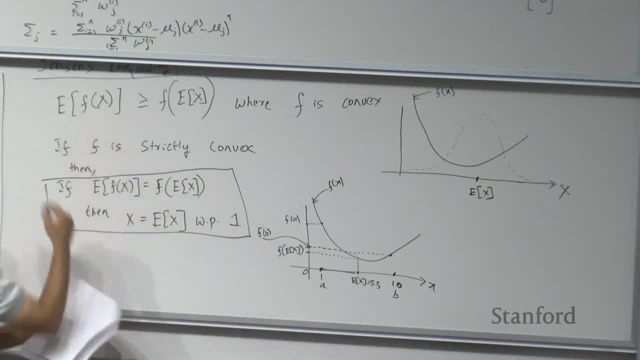 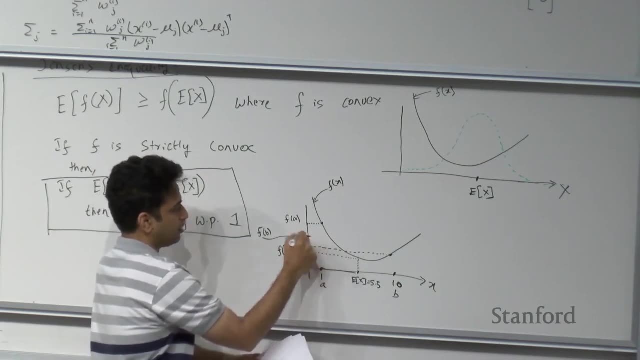 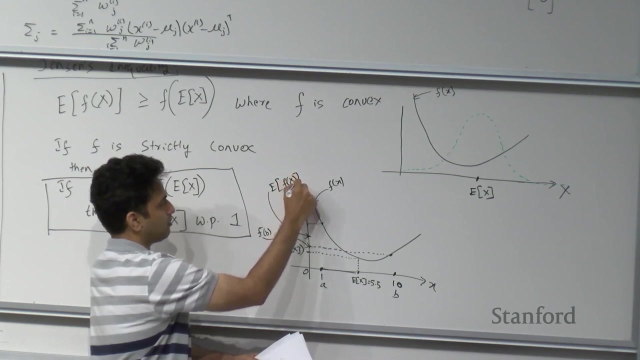 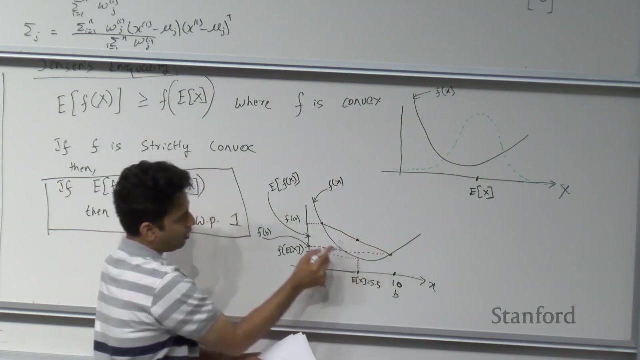 So the expectation, uh, of f of x is this one right? And this is expectation of f of x, right? And it- it so happens that this point will always be the midpoint of- it'll always be the midpoint of the chord connecting f of a and f of b. 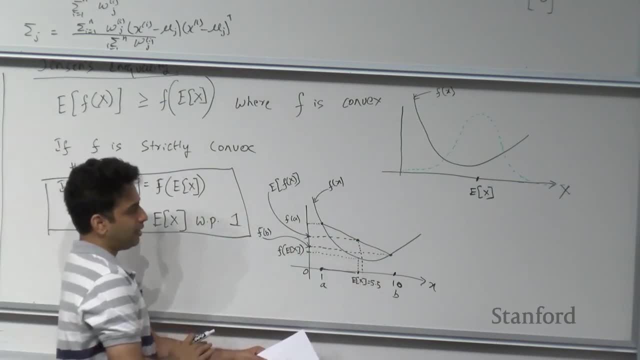 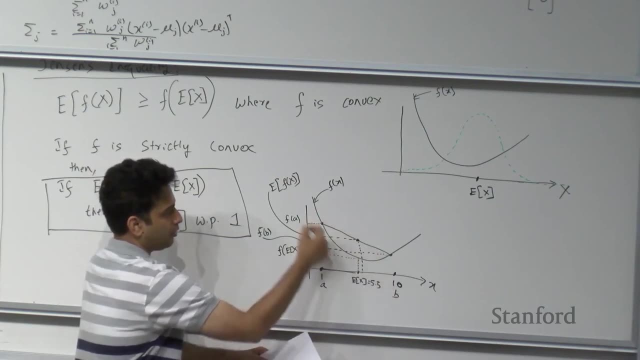 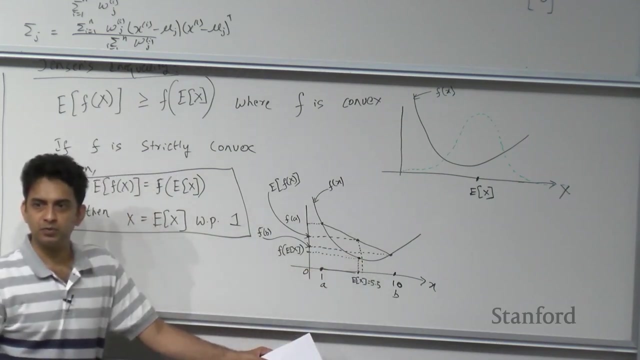 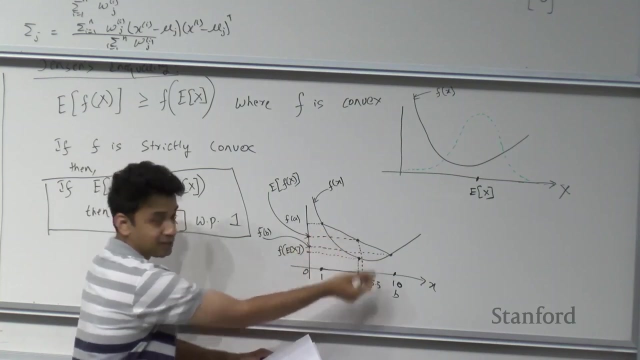 Right. And what Jensen's inequality is telling us is that this point, the point that that's the- the midpoint of the chord connecting two points on f, will always be higher than this point, right? So f of expectation of x is always less than the expectation of f of x, right? 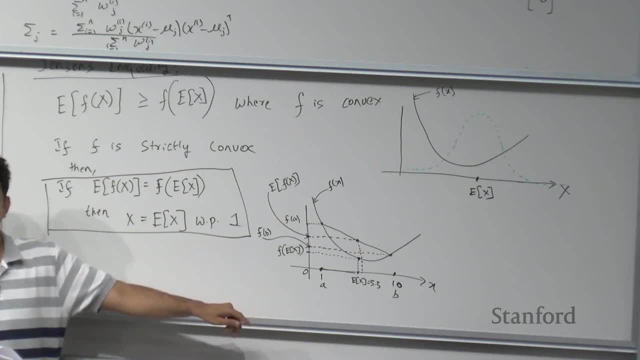 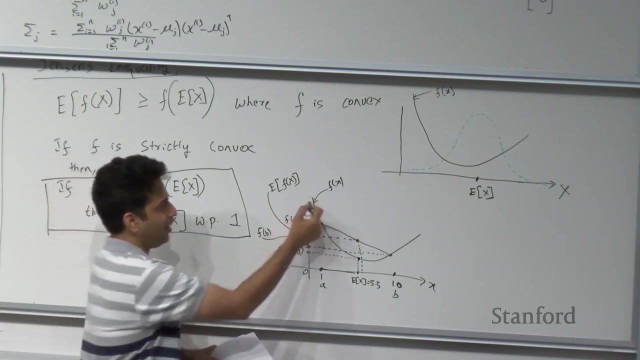 Is this clear? Can you raise your hand? if you understood this? Some of you have not. Okay, Can anybody tell me what- what's- what- what's- what's still confusing here? I can just go over it again. So f is a convex function which is kind of bending upwards right. 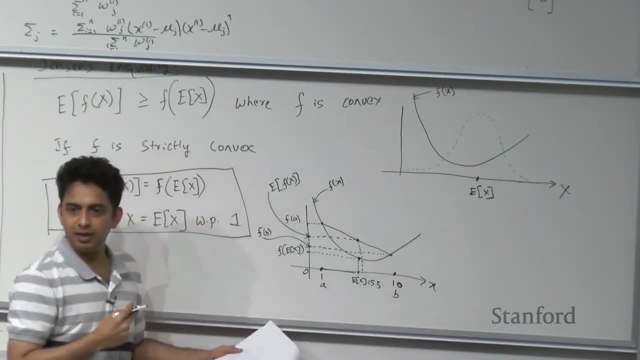 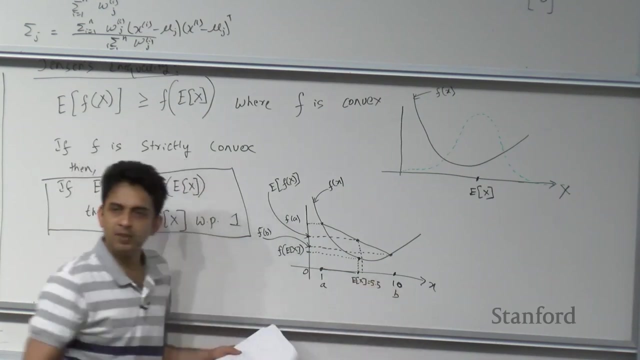 And the x-axis is-, is-, is- is- denotes some random variable right? And in this case, just for the purpose of understanding Jensen's inequality, let's assume x is-, is- is- takes on two values, one of two values, either 1 or 10,. 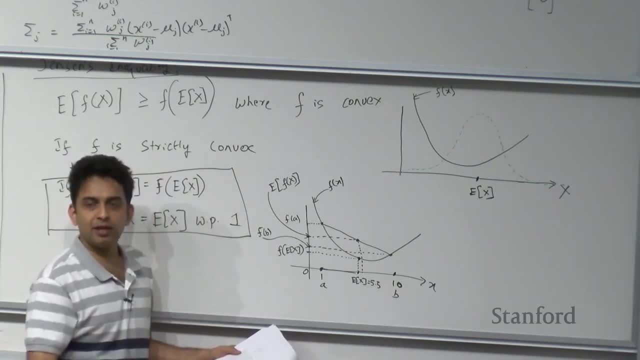 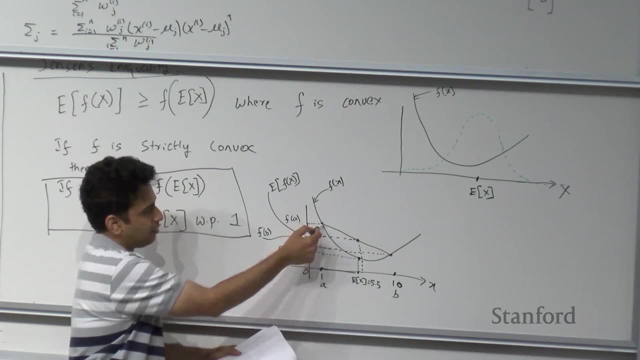 with equal probability. So the expectation of x is therefore 5.5, right, That's- that's over here. Now. f of 1, you know, let's call it a. you know, f of a is- is this point. 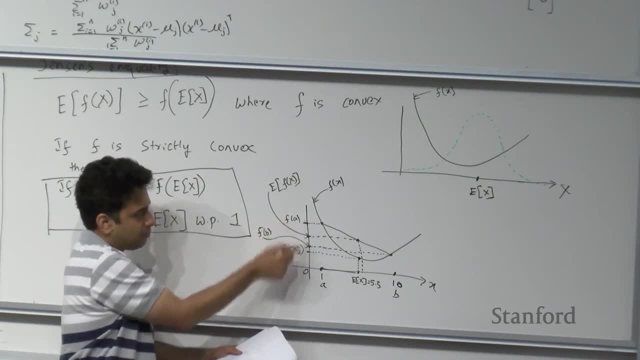 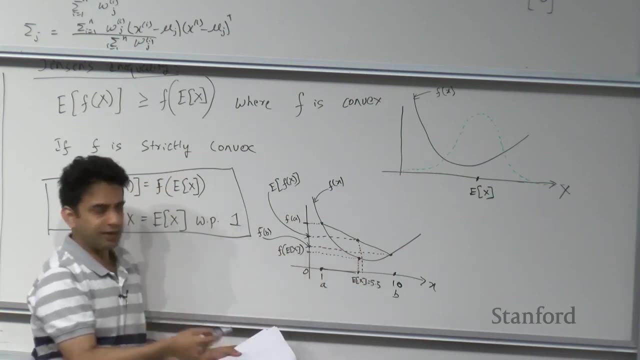 So this is f of a. So the height from the x-axis to this point, this is f of a And similarly, if this is b, this is f of b And the expectation of f of x is therefore the midpoint connecting these two points right. 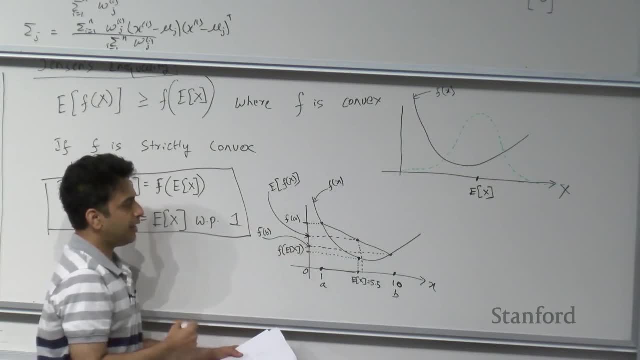 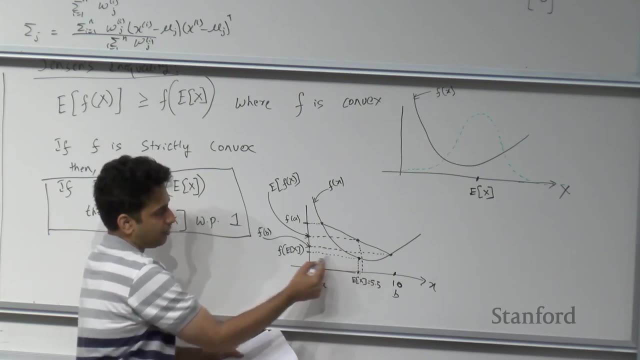 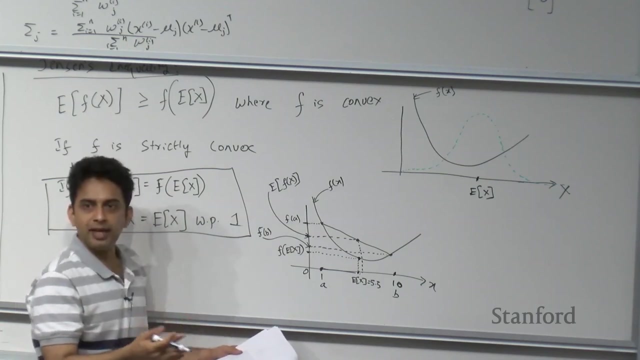 And that comes over here. And the ex- f of expectation of x, where expectation of x was- was 5.5, is this point that comes over here? And Jensen's inequality is- is therefore essentially saying that the chord connecting any two points of a convex function always lies above the chord itself, right? 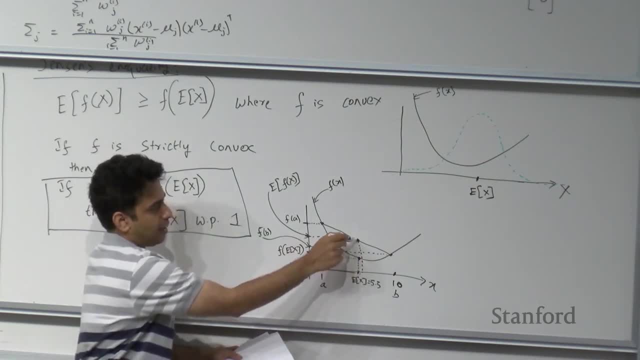 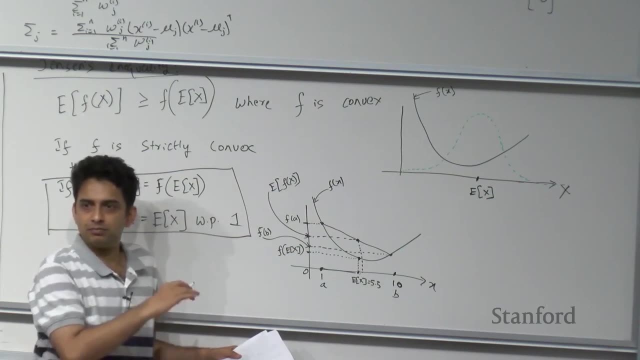 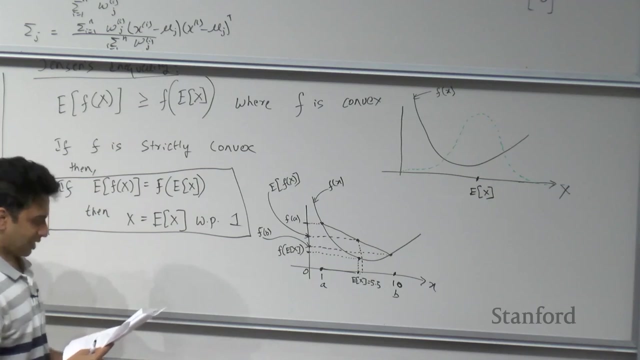 The expectation- expectation of f of x is- is higher than f of expectation of x. right, Kind of understood. All right, Okay, Let's- let's, uh, uh, move on. And it also tells us that if f is strictly convex, right. 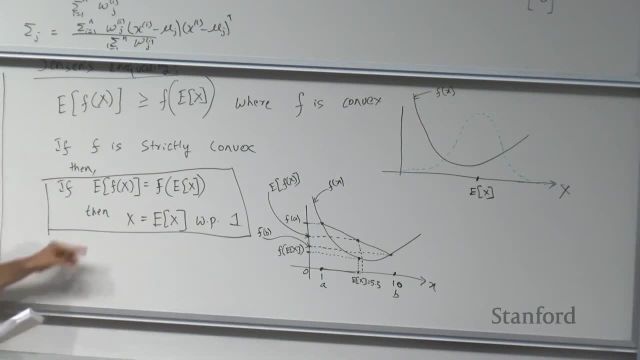 F is strictly convex, then um f of x equals- if it is, f is strictly convex, and if expectation of f of x equals f of expectation of x, then x equals the expectation of x, uh itself, which means x is essentially uh a constant. 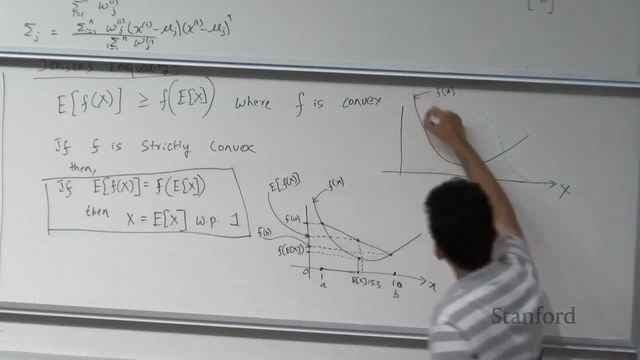 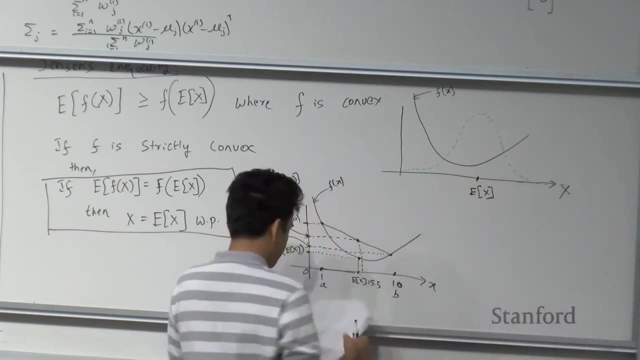 What does that mean? So here's an example of f of x that is strictly convex. right Now, um, if expectation of f of x equals f of expectation of x, when can that be possible? right Expectation of f of x equals. 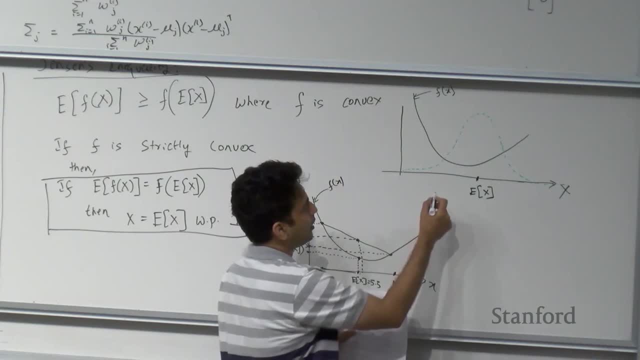 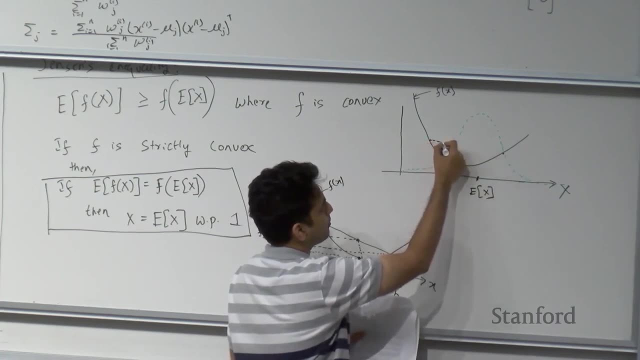 uh, uh. f of expectation of x. When can um- let's assume you know, a and b are here. This is expectation of f of x and let's say this is f of expectation of x, right, If f is strictly convex. 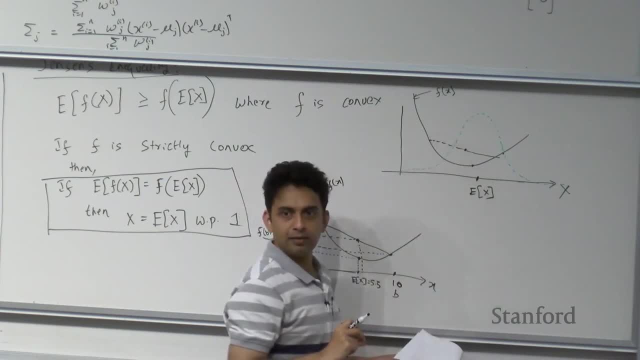 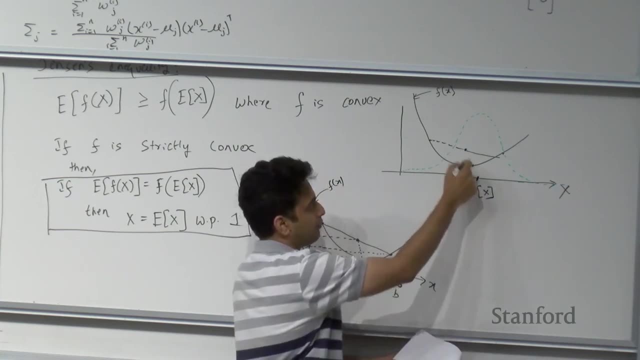 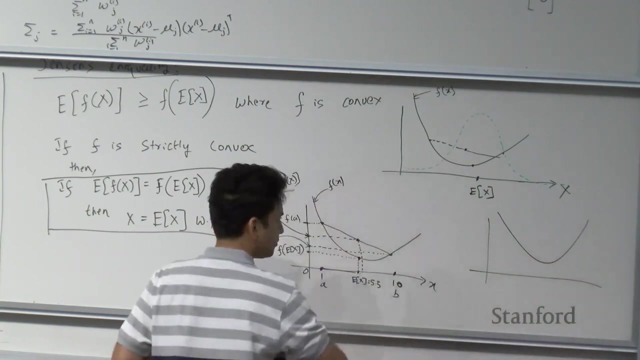 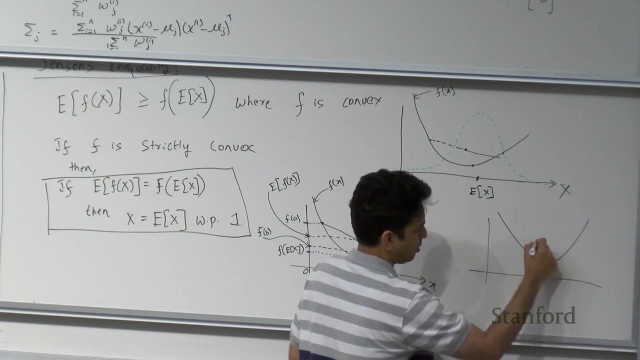 and if the two are equal- f of x equals expectation of x- then the only way that is possible that you know f of x equals expectation of f, uh, f of x is if x has a probability density right. 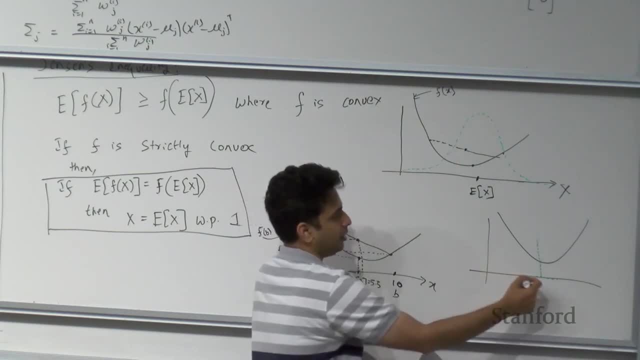 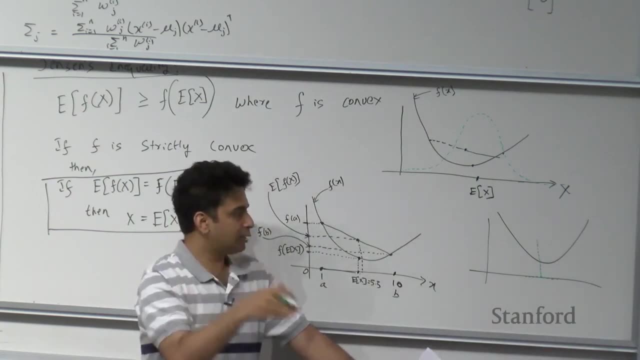 Now over here there's dotted line. Essentially, I'm drawing, uh uh, the probability density of x, which is like a Dirac delta function, where it has, uh, all its mass concentrated at just one point right. 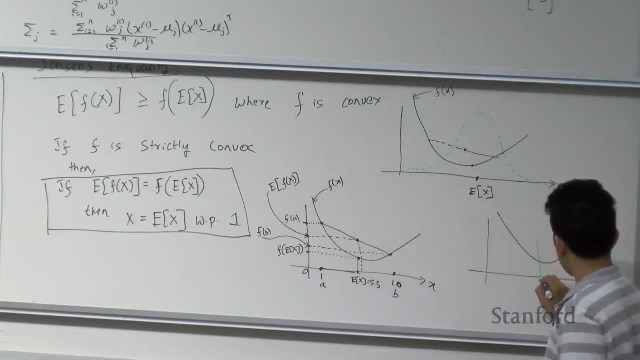 And in this case this is expectation of x, and f of expectation of x is here, And also because x always takes on this value with probability 1, f of x also always takes on this prob-, this value with- with probability 1.. 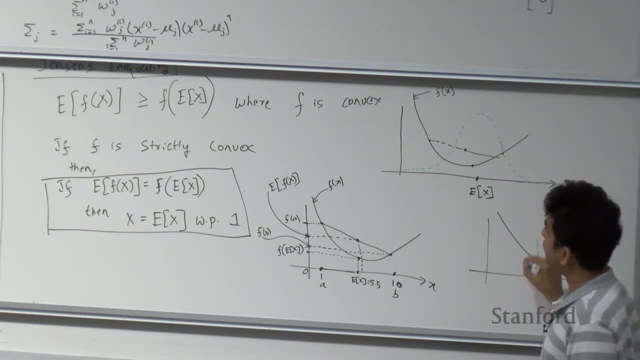 And therefore f of x equals f of expectation of x equals expectation of f of x, Because essentially, you know, the equivalent of the chord connecting two points has length 0 here. right, All the values of f of x are always here and x always evaluates to the same value. 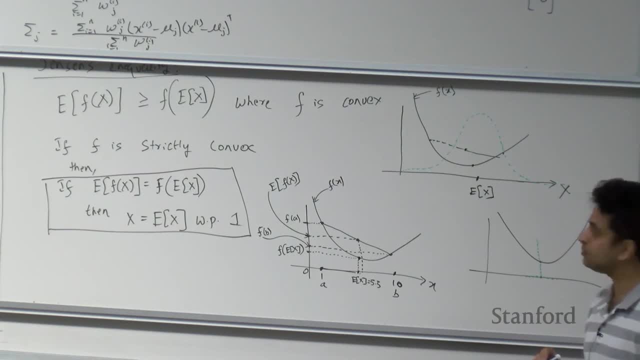 Next question. So what's the expectation of a- a continuous random variable? If x is a continuous random variable and it has a PDF, let's call it small p of x, right? Then expectation of x is equal to the integral of x times p of x px. 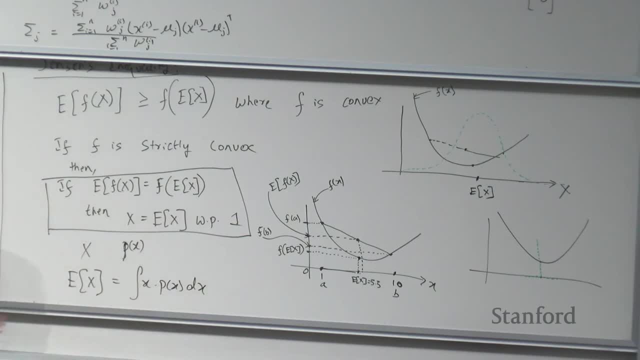 So here p of x will become f of x. So p in this case is some probability. So the green line, the green dotted line, is p of x here. So my question is: what is p of f of x? Yes, So-, oh, what's e of f of x? 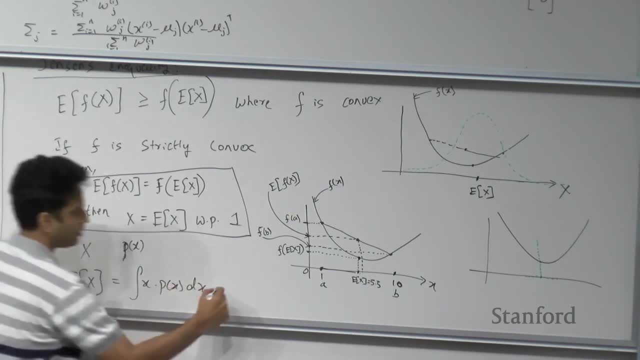 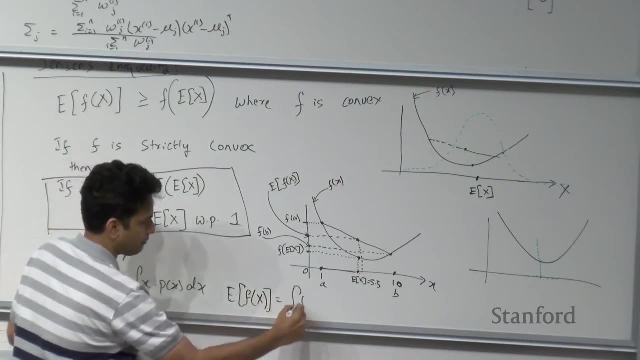 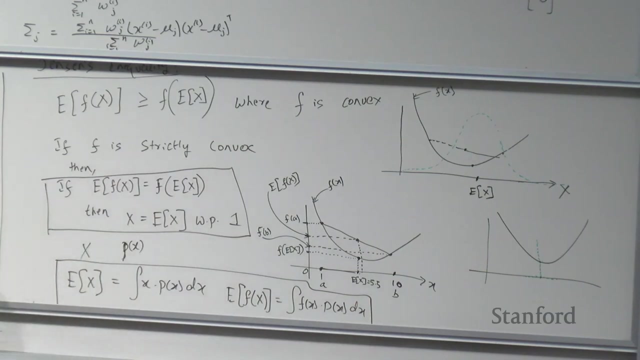 So e of f of x? uh, so if e of f of x is equal to the integral of f of x, p of x, dx, Good question, right. So this is-. this is Jensen's inequality. Um, and- and- and the reason. 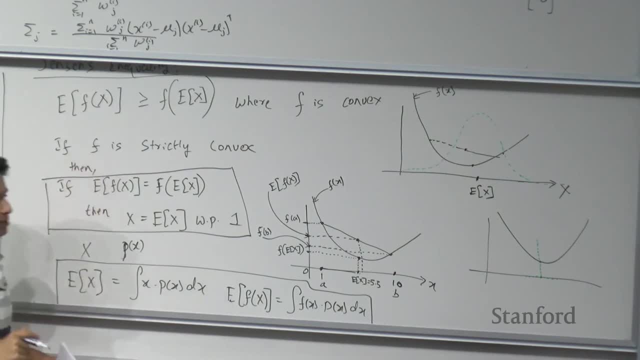 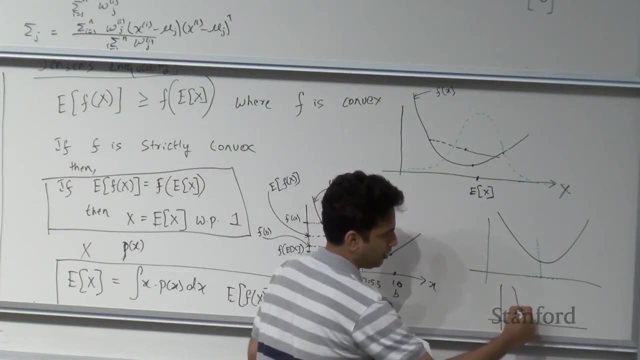 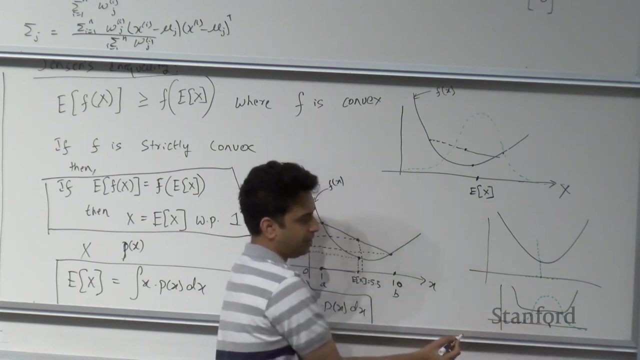 why we require f to be strictly convex is because um if f were not strictly convex, then you could have a case where x- x is- f of x is flat in some place and x has this uh density, And um expectation of f of x would be here. 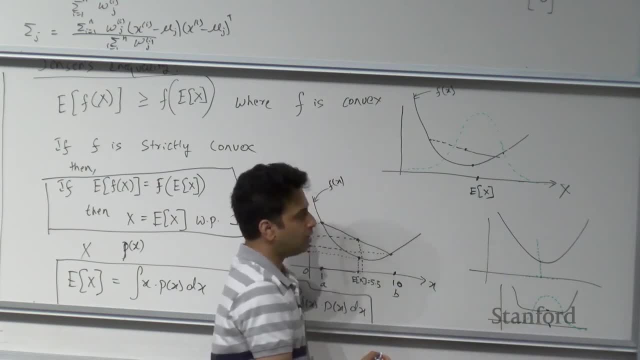 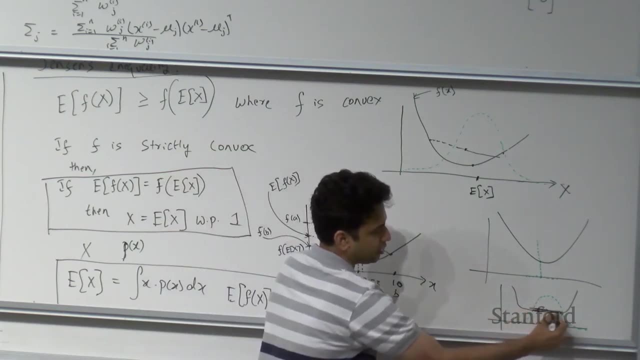 and f of expectation would be here, And also, uh, f- expectation of f of x would also be the average f of x in this region, which is also a constant. So expectation of f of x would be equal to f of expectation of. 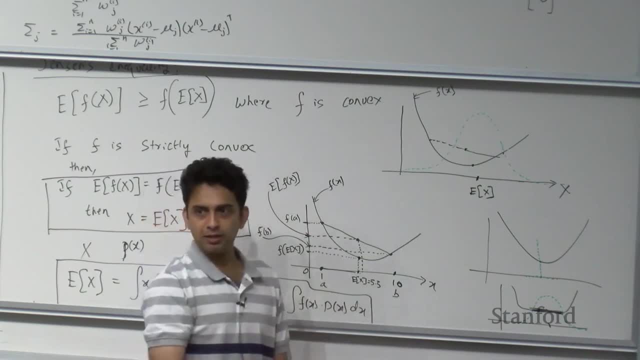 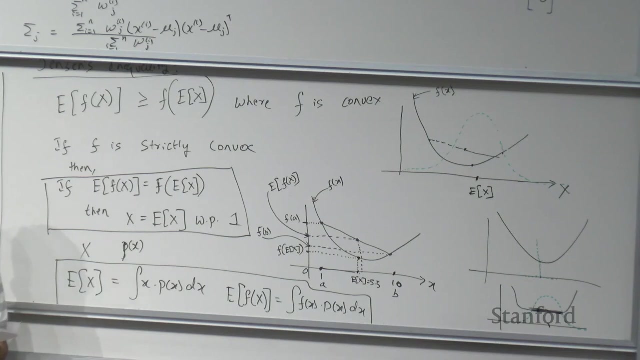 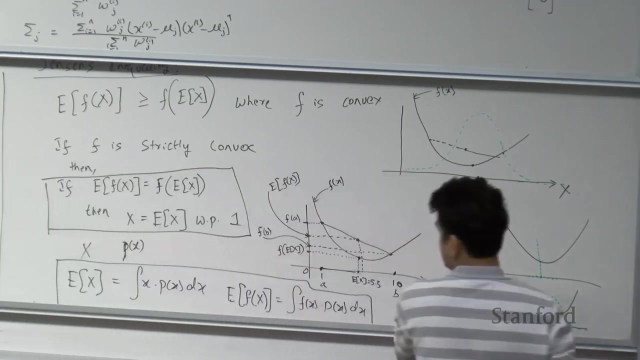 x, uh, even though x is not constant because f has a flat region somewhere. Next question: So the question is: uh, uh, uh, in- in the- in the convex case, can we assume that- So, for-, for-, for, um-, I mean. 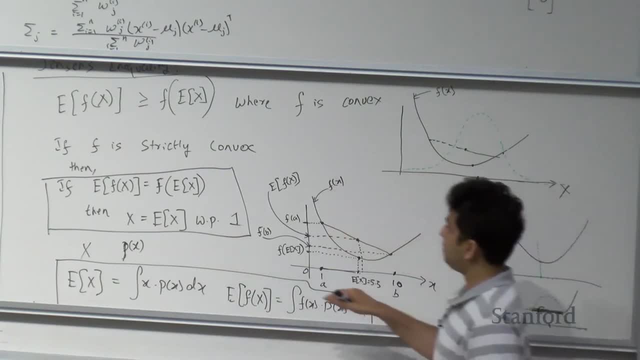 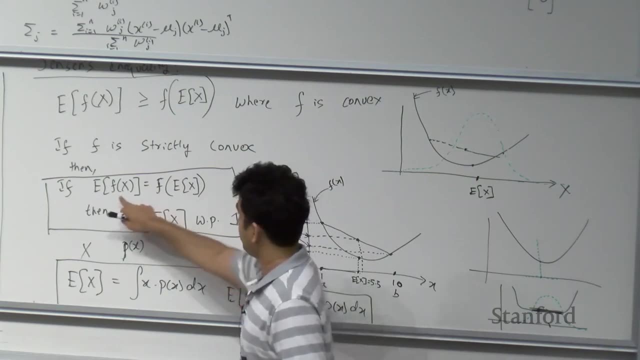 for this- for this case, Yeah. So if- if um for this to hold without uh, x being a constant, for x to- and f of x to be the same, then all of x should be distributed in a region where f is. 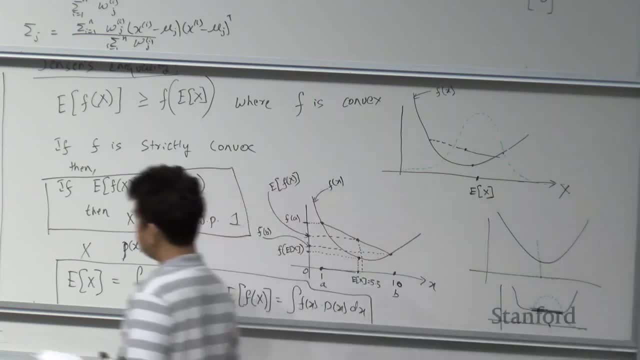 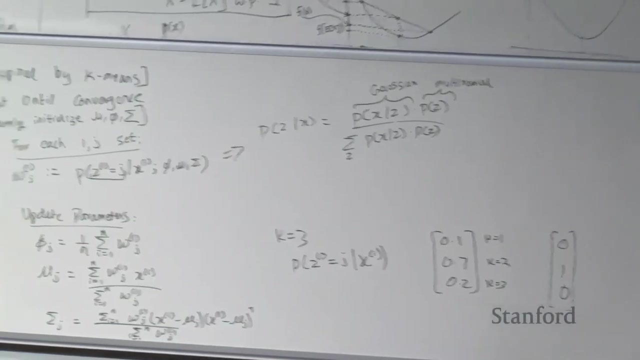 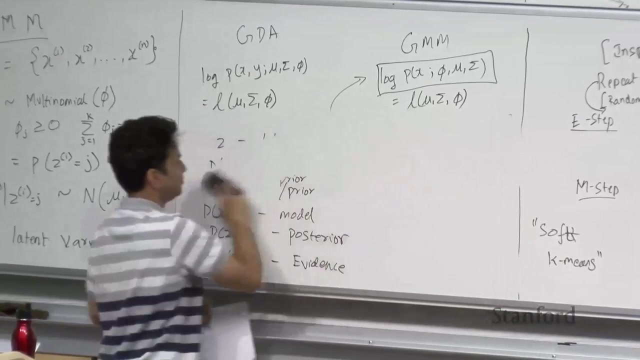 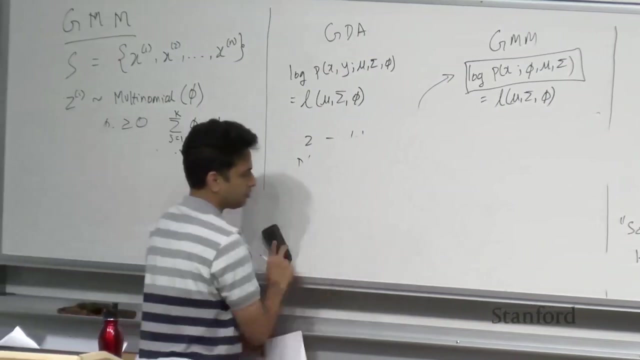 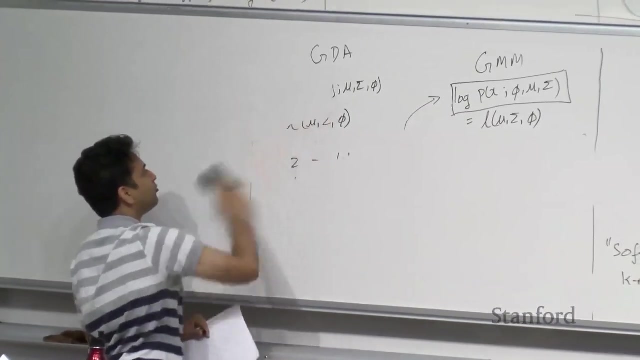 flat. Yeah, that's right. All right, So what are some examples of convex functions? Anybody have an example of a convex function? Y equals x squared. Y equals x squared. Example for concave function: Minus x squared. Y equals minus x squared. 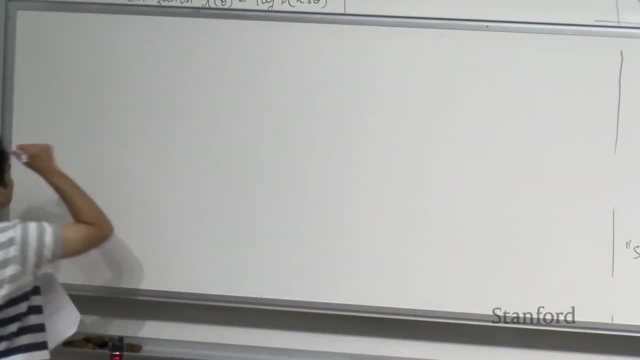 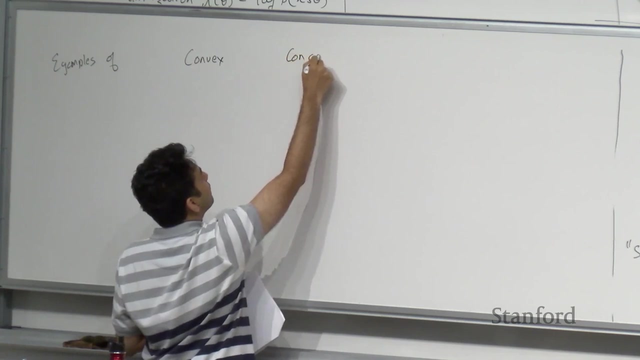 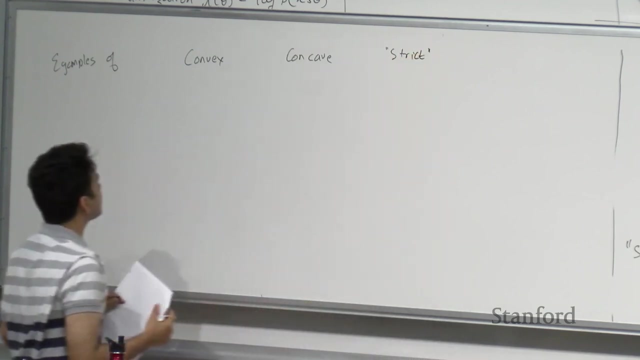 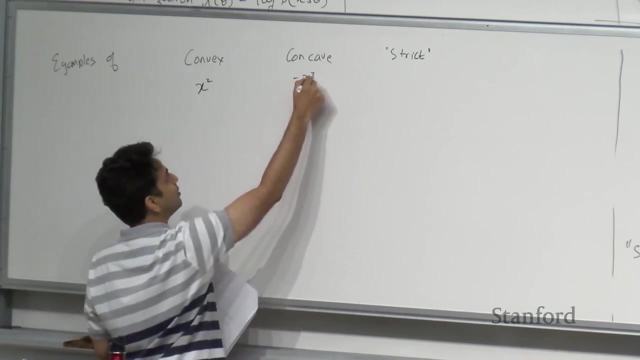 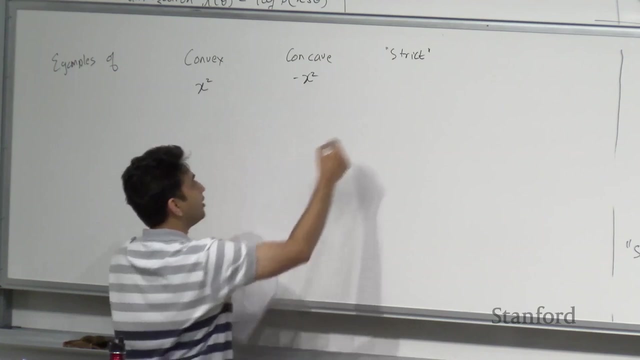 Yeah, Yeah, That's good. So um examples of convex, Concave and strict yes or no right. So convex function: we saw: x squared is convex, Minus x squared is therefore concave, right. And is this strictly convex and therefore also strictly concave right? 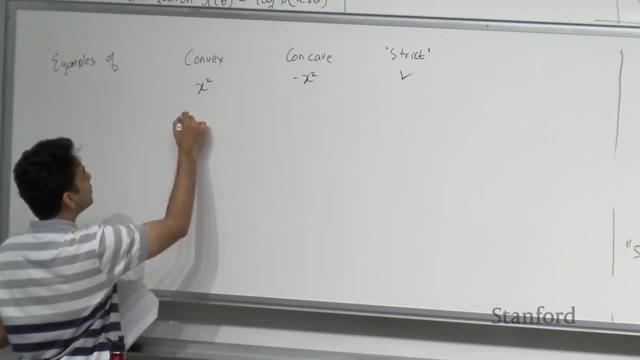 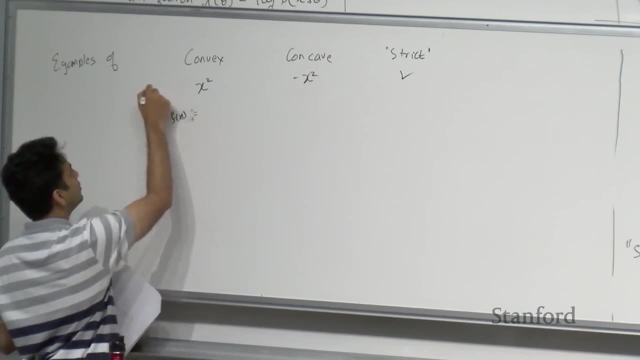 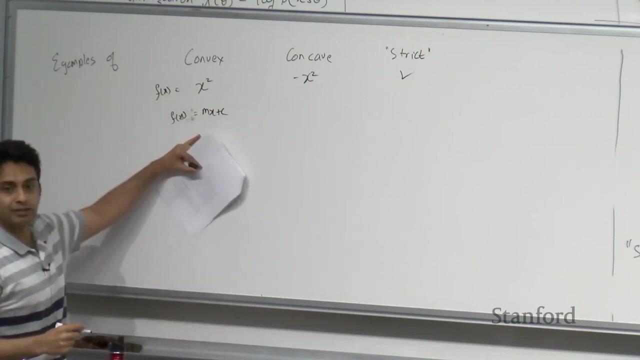 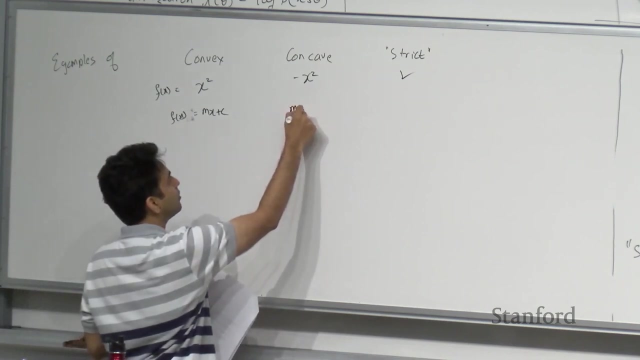 Now another function: um y equals or- or f of x equals equals, say mx plus c. straight line is convex. By definition it is convex. A straight line is convex and it is also concave. But is it strict? No right. 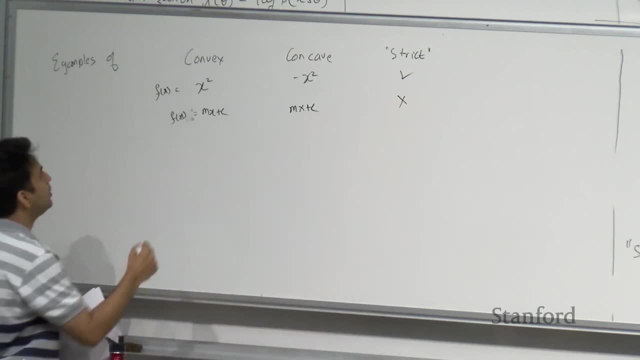 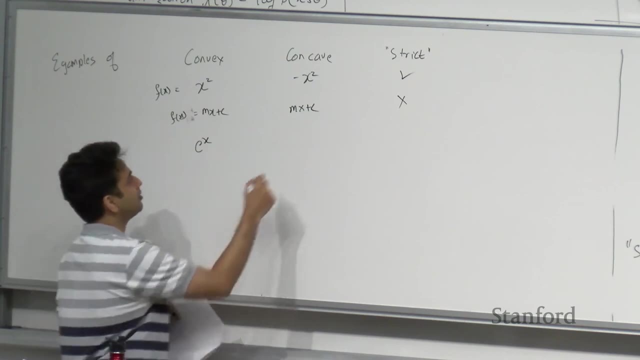 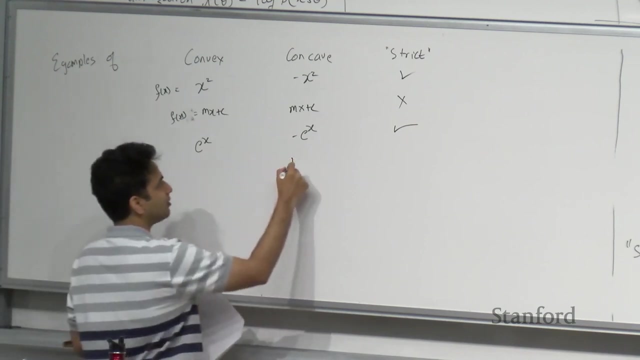 It's not Great. Now, um, what about? e to the x? Con- convex Minus e to the x is therefore concave. Is it strict? What about log x? No, yes, So log x is concave and therefore minus log x is convex, right. 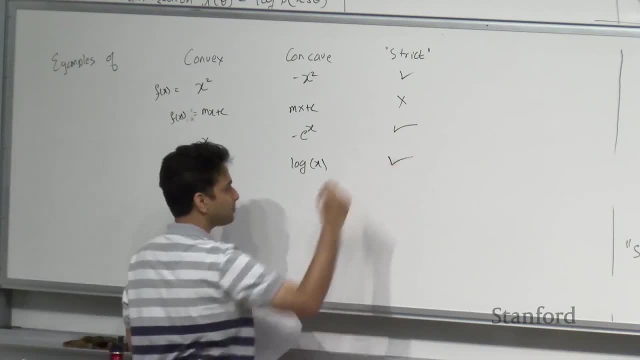 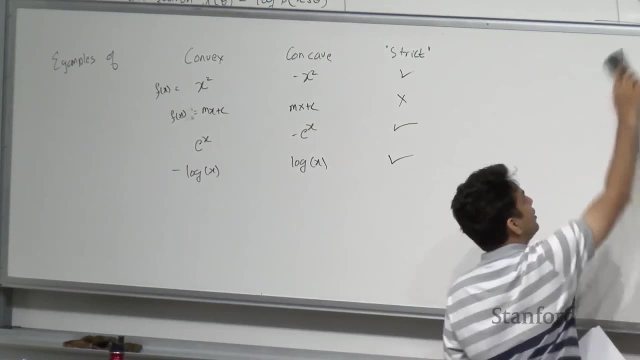 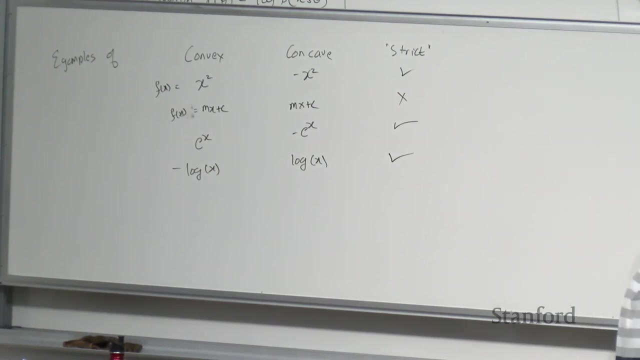 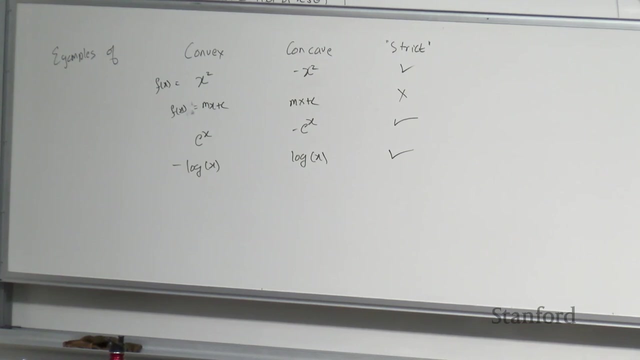 And it is strict. Okay, Cool. Now how does this- how is this useful for expectation maximization? Yes, question, Yeah. a straight line is always convex and concave, uh, because is-, is- is uh. 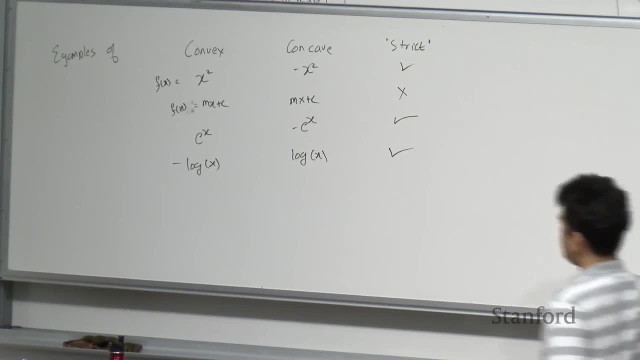 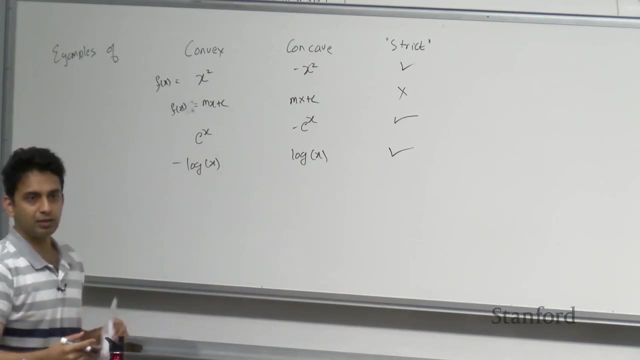 so f double prime is equal to 0, and the definition of convex is that f double prime should be greater than or equal to 0.. So- and it's equal to 0. So it satisfies greater than or equal to 0.. And similarly for concave. 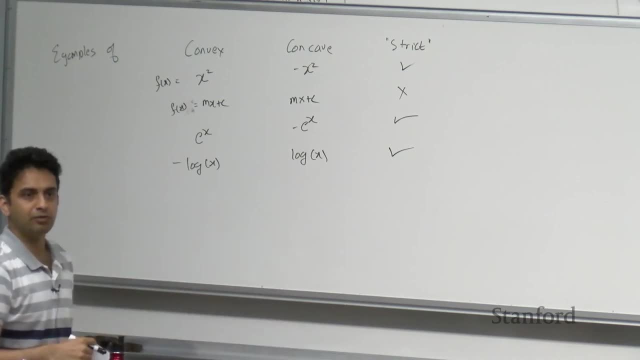 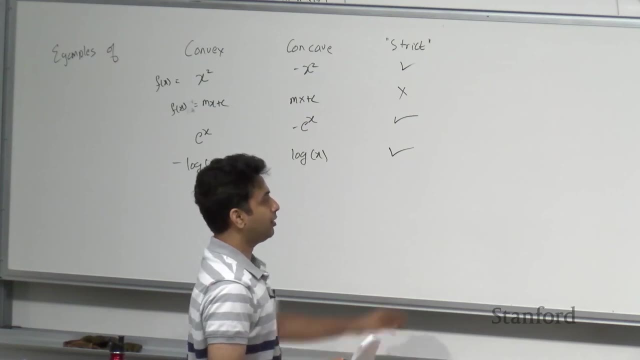 it is less than or equal to 0, and it's equal to 0.. So it satisfies: less than or equal to 0.. So now, um so, using Jensen's inequality and with these observations, that uh expectation of uh. 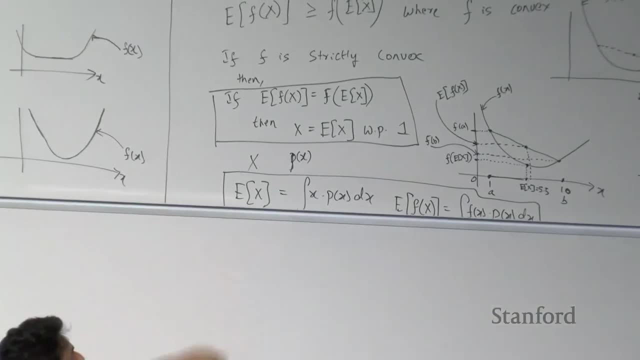 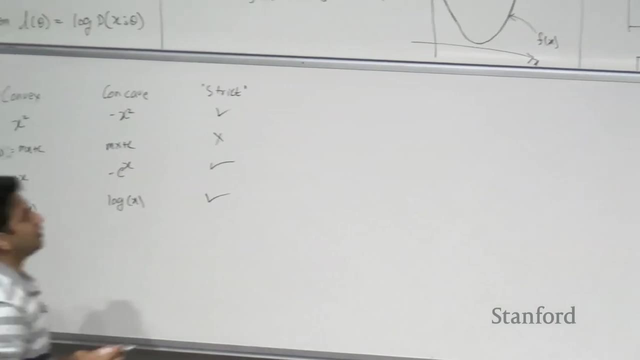 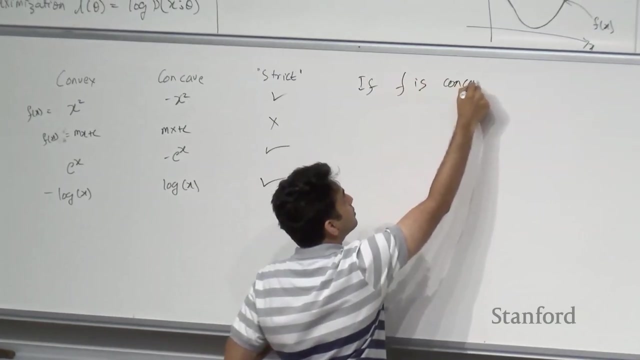 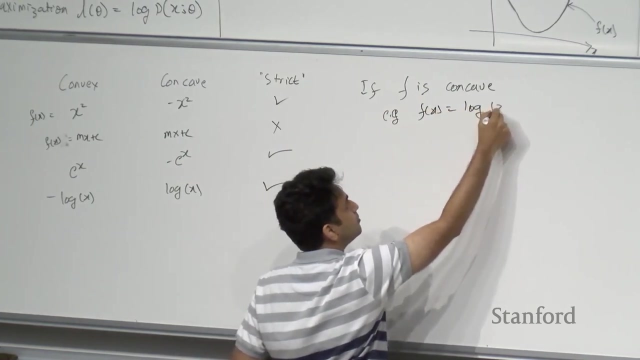 f of x is greater than equal to f of expectation of x and- and uh, so on. um we can adapt Jensen's inequality to the concave case, where basically it says: if f is concave right, Example f of x equals log x right. 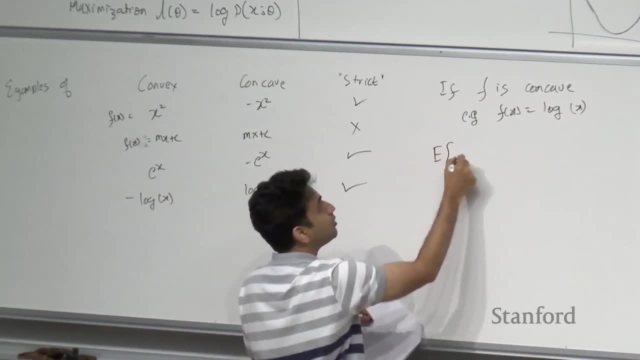 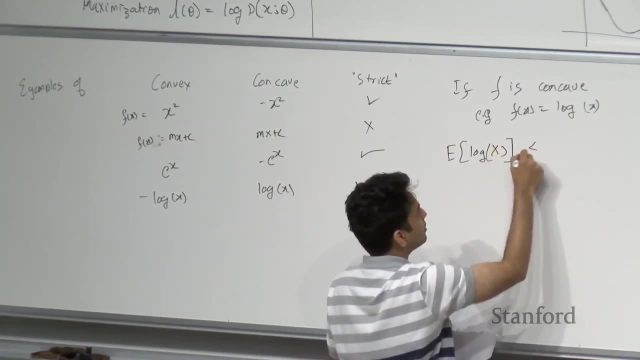 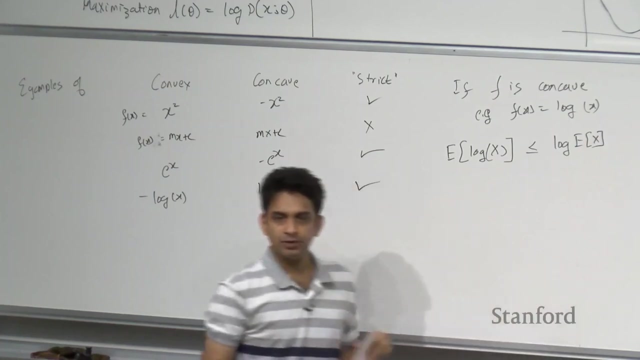 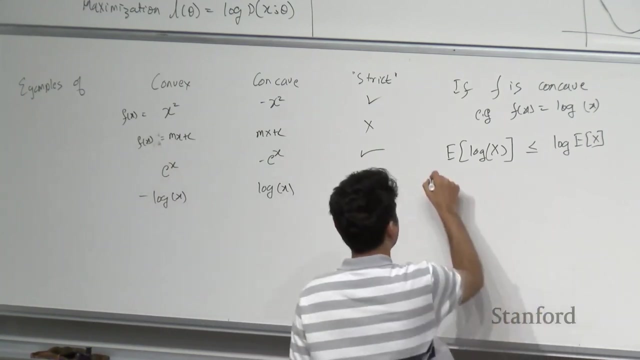 Then the inequality will switch. So the expectation of log x, instead of greater than or equal to, will be less than or equal to log expectation of x, right. This is also Jensen's inequality. So now let's derive the EM algorithm, right. 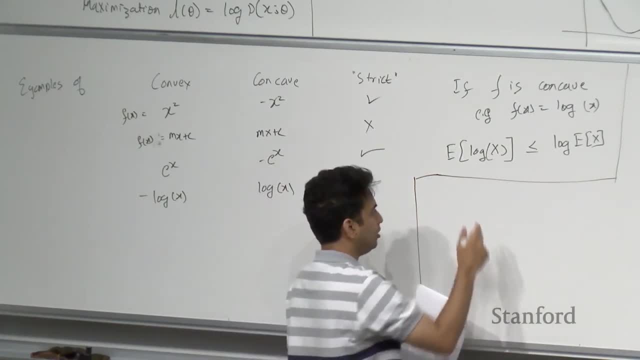 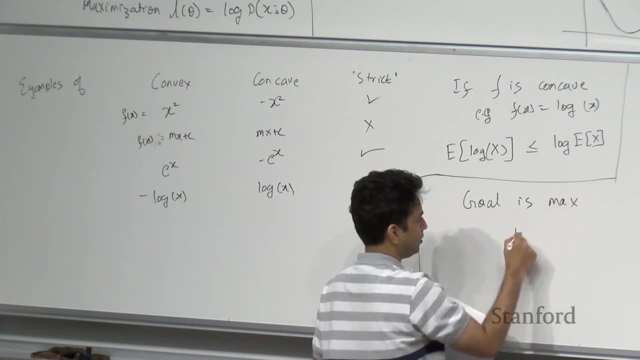 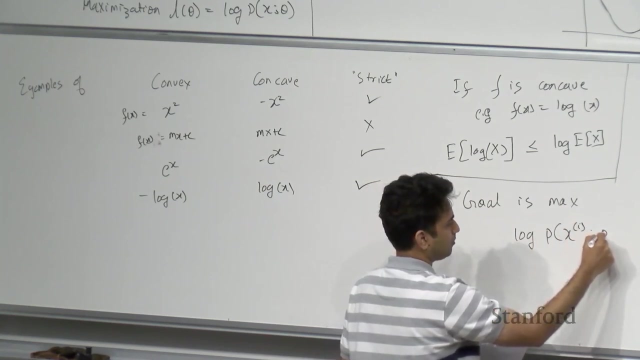 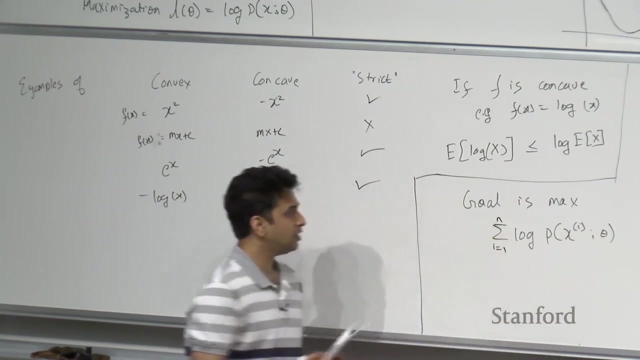 So in the EM algorithm, our goal is to maximize log p of x, i, comma, uh, theta, where by theta mean you know all the parameters- i equals 1 to n. right, We want to maximize this. That's the goal. what- what we are trying to achieve? 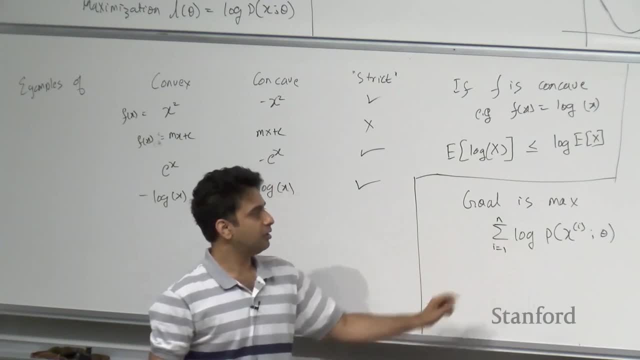 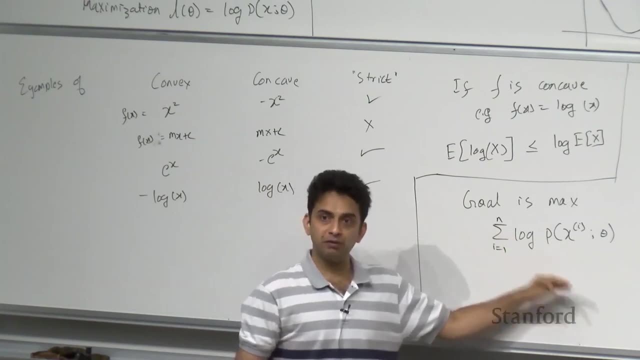 This is our end goal. We want to maximize log p of x. But, however, maximizing log p of x can be hard because the z's are unobserved. If z's were observed, this was very easy, but z's are unobserved, so it's hard. 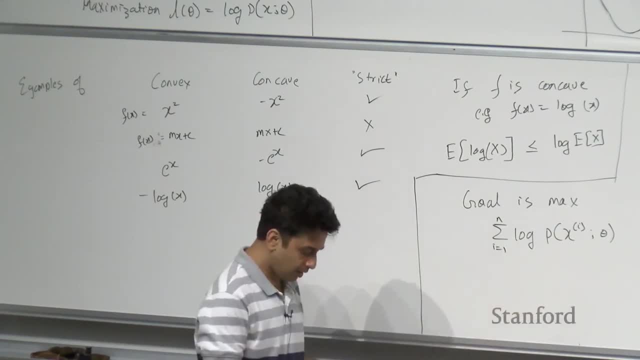 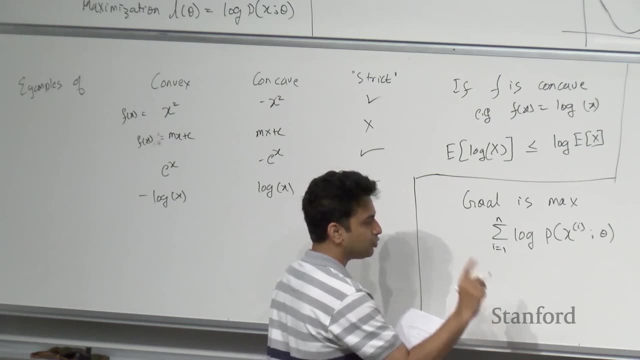 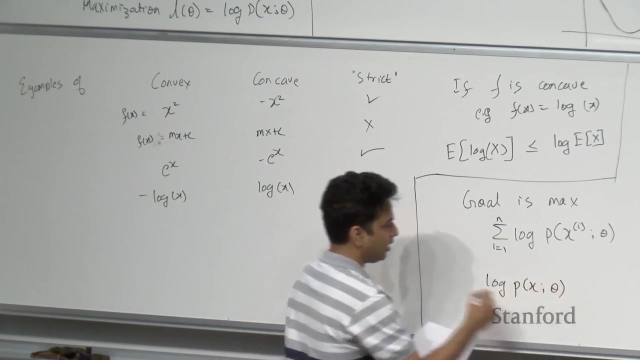 That's the case where- that's the setting we are in. And now for- for the derivation: um, I'm going to assume one example, So I'm just gonna write it as log p of x comma theta, And I'm going to leave the summation out. 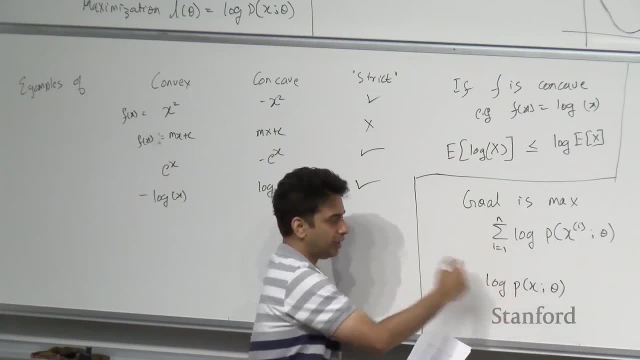 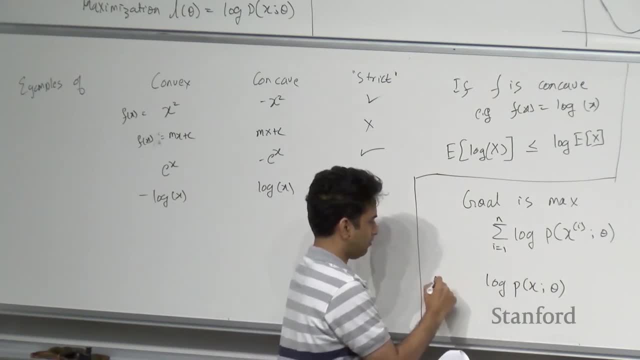 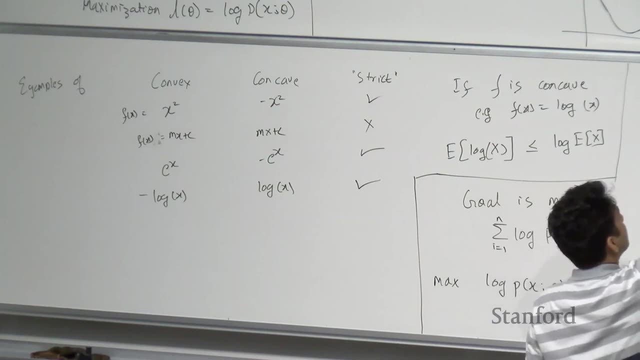 Right. So log P of x. we want to maximize this. That's our goal, Right? So the first thing we're gonna do is write log P of x comma theta is equal to log of the sum over z. P of x, z theta, right. 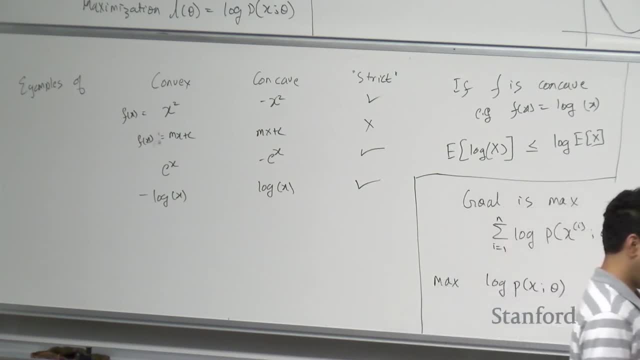 First we're going to marginalize out z right And then, once we do that, we will define an- you know some arbitrary probability distribution called Q over z's, and write this as log: sum over z: Q of z times P of-. 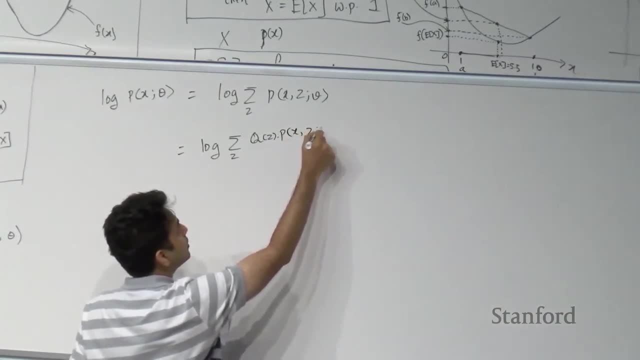 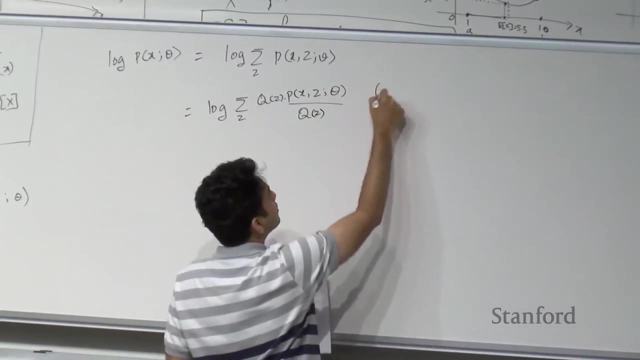 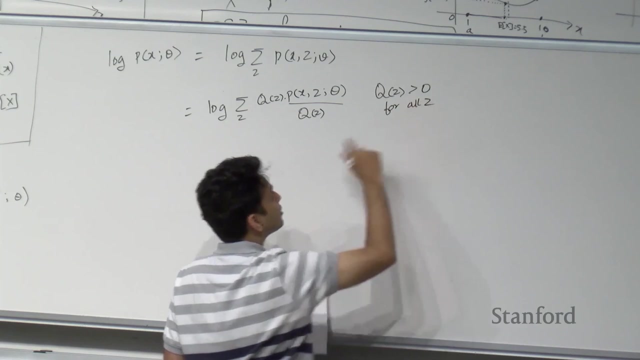 Okay, X comma, z, theta divided by Q of z, where Q of z is greater than 0 for all z. Some arbitrary probability distribution over z. It could be anything whatsoever. Any kind of probability distribution over z such that Q of z is greater than 0 everywhere. 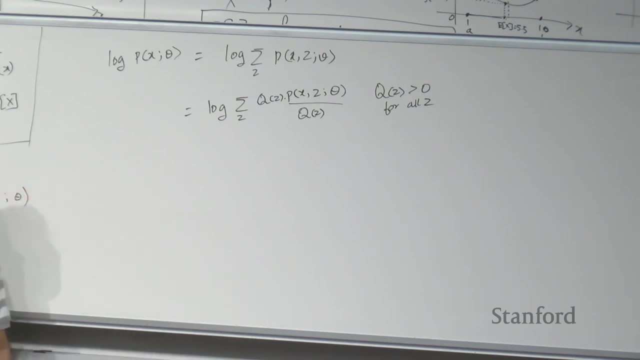 This question, So the- so the question is: ah, it's- ah, you know why is this a hard problem? So it- it is hard because- because you're having a summation over here, right, And in general, when- in- in the cases where z is continuous. 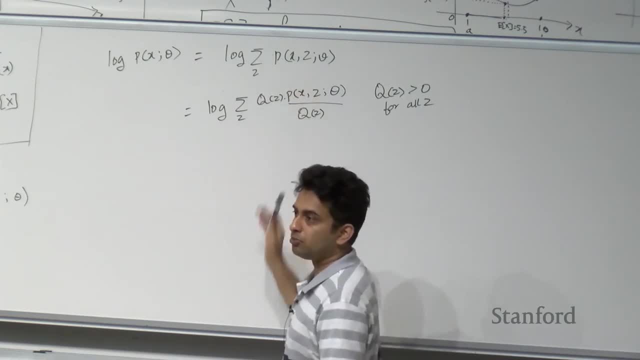 this would be an integral right And that integral can be, you know, arbitrarily co- complex. Sir you mean computationally expensive. It can be computationally expensive, It can be analytically not possible in cases when we want an analytical solution. 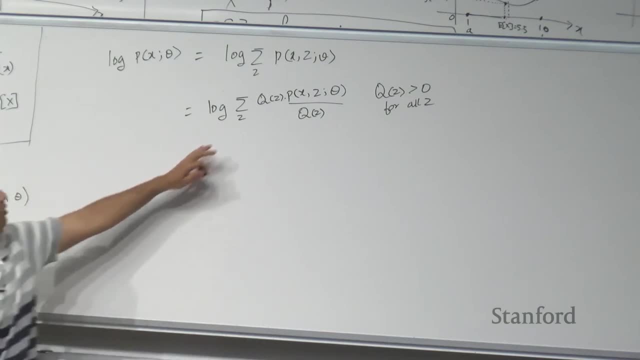 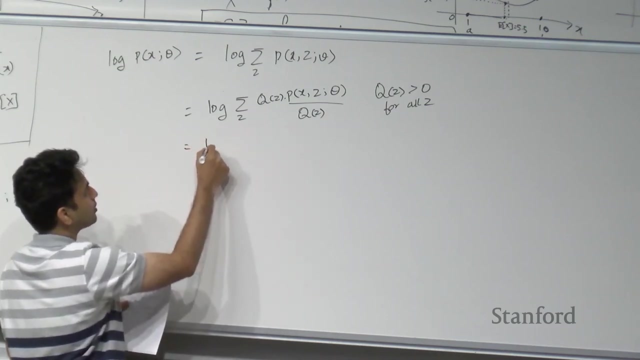 Good question. Uh, so we come up-. you know, q can be any distribution whatsoever as long as q of z is greater than 0 for all z And-. and now we can see that this can be written as log expect-. 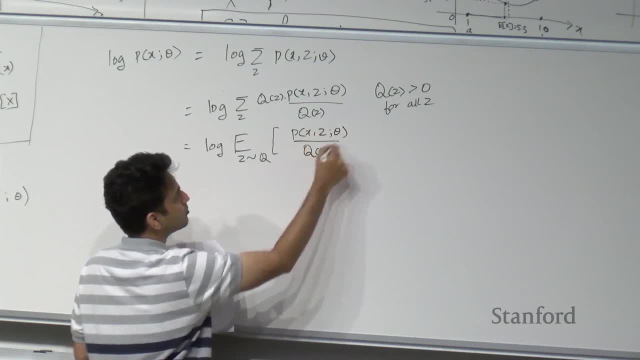 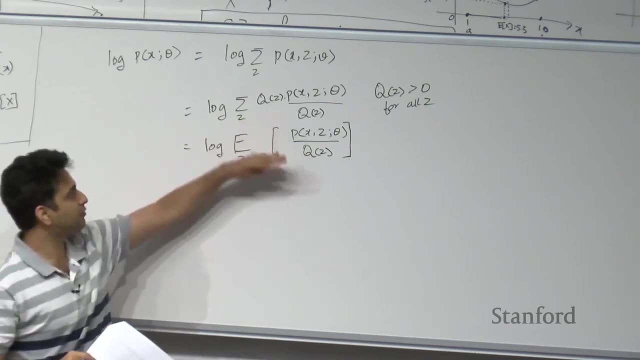 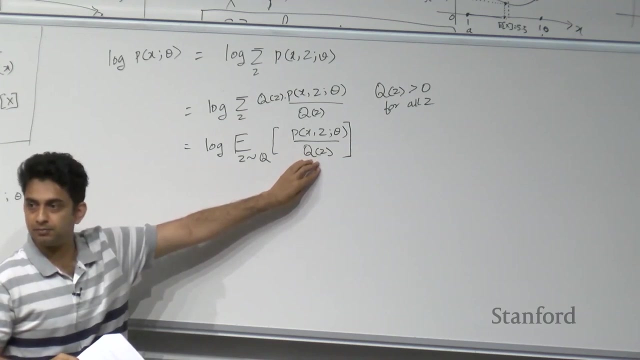 right? What did I do here? Nothing, basically. So this is the definition of expectation, right? So this is a function of s- you know z some function of z right? And uh, think of this as the probability, and this is some function. 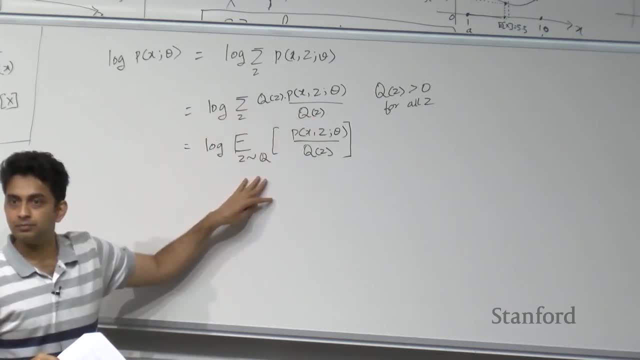 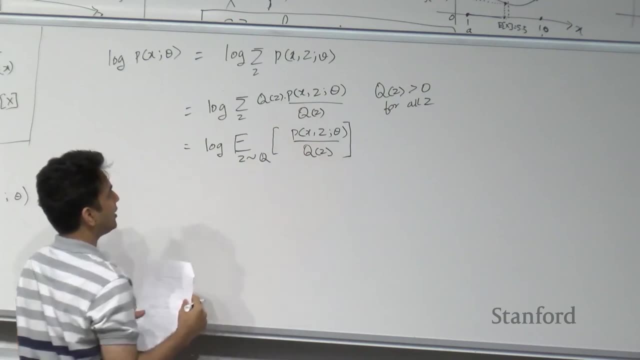 and therefore this is just the expectation. Is this clear? Yeah, Okay, So this is- this is just- uh, you know, um um- the expectation. And now we make use of Jensen's inequality and note that log of the expectation of something. 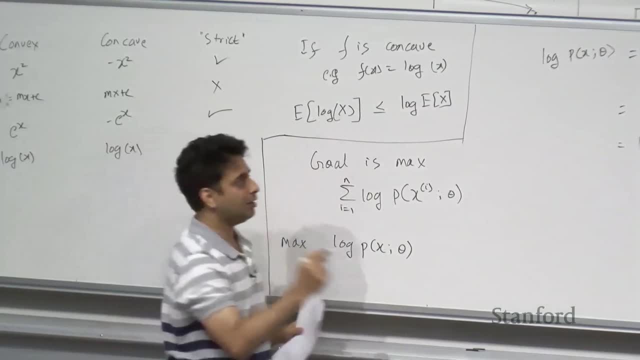 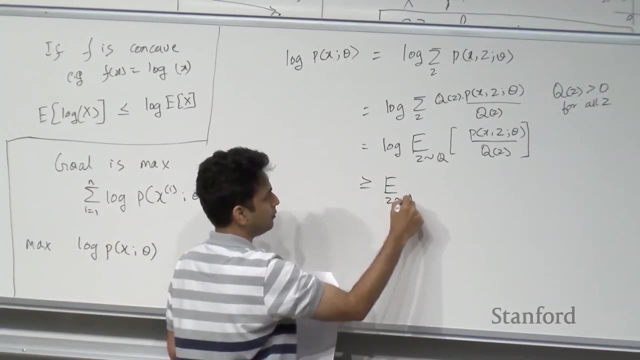 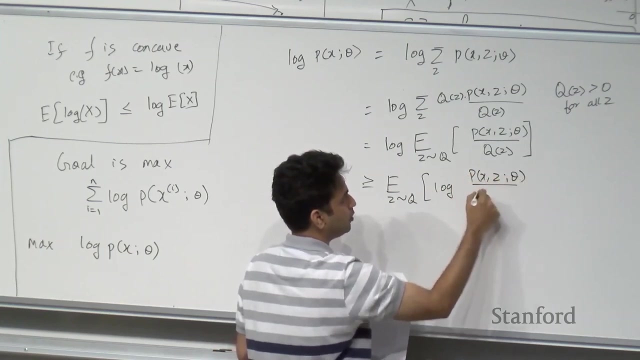 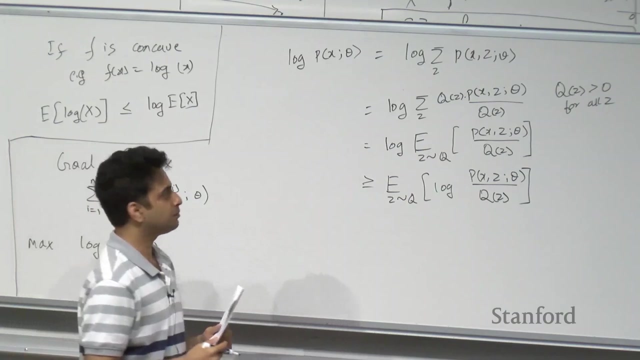 is greater than the expectation of the log of the same thing, right, And so this is gonna be greater than or equal to expectation of z of q log p of x z Theta over 0. Q of z. This question F is concave. 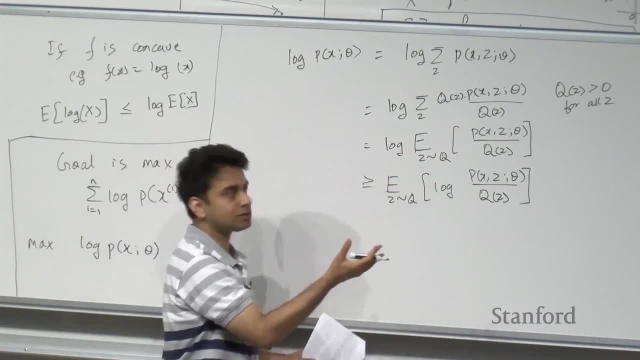 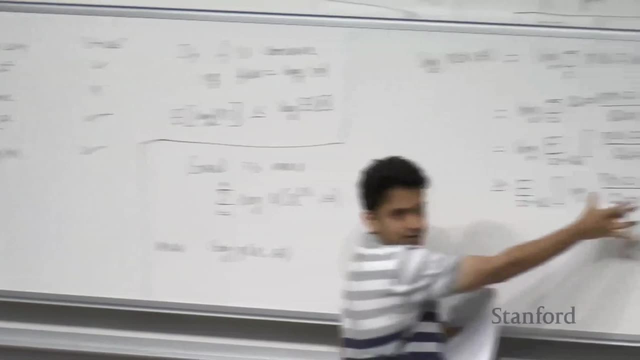 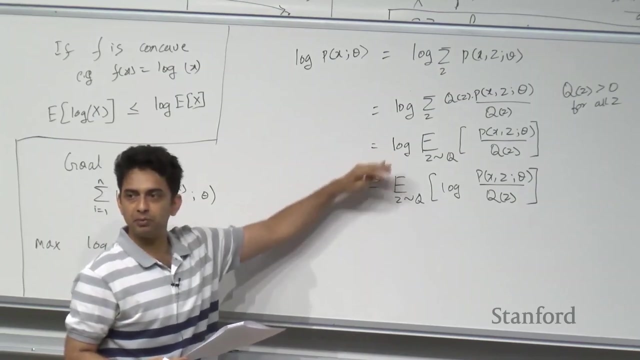 F, here is log and log is concave. Log is concave right And this is our random variable x right. Any- any- any- any. uh. questions on how we applied- how we went from here to here. 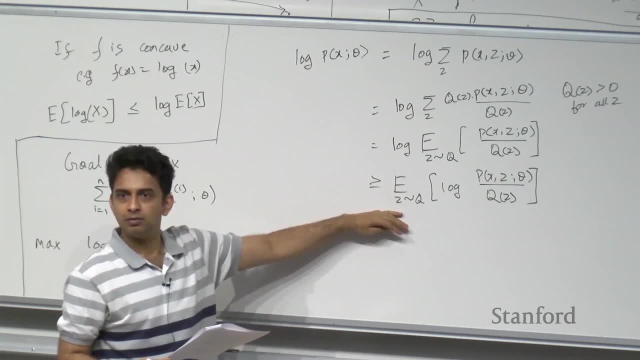 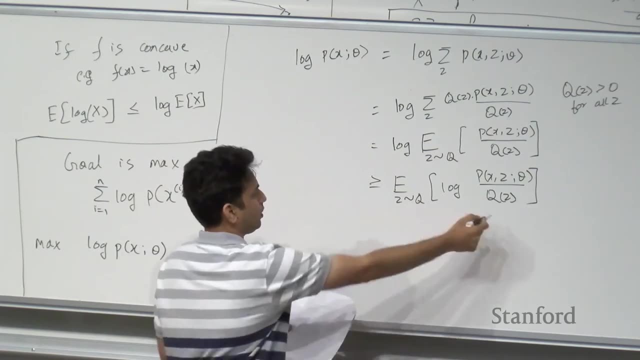 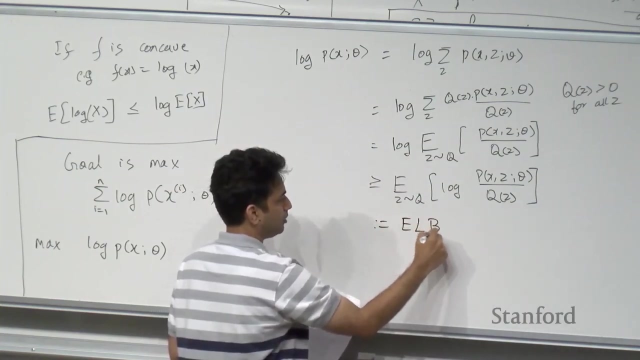 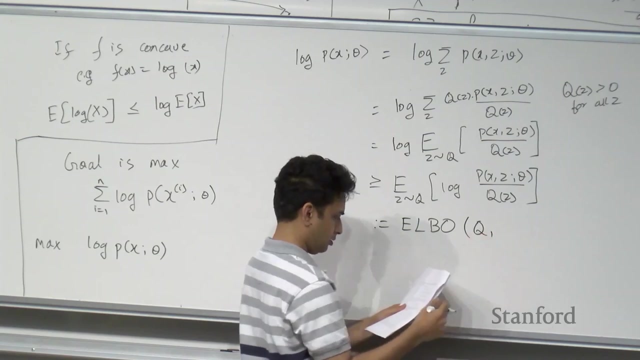 This is probably the most crucial step. All good, Okay, And this, what we see here, we will call this, you know, give it a name. we'll call it ELBO, Evidence, Lower Bound, right. So it's the ELBO of q and ELBO of x, q, Theta. 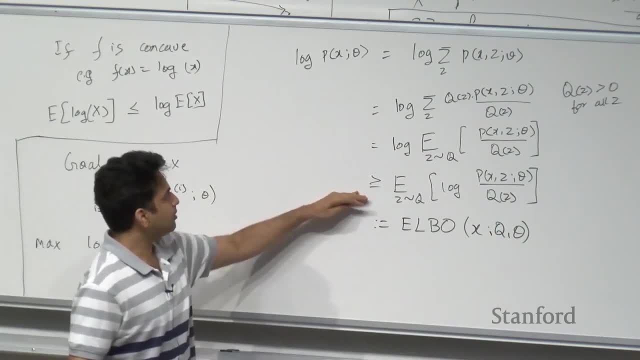 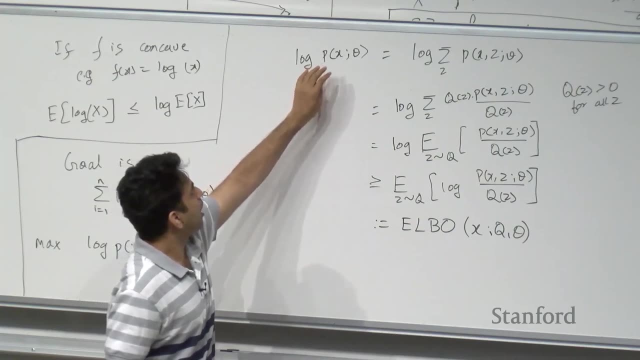 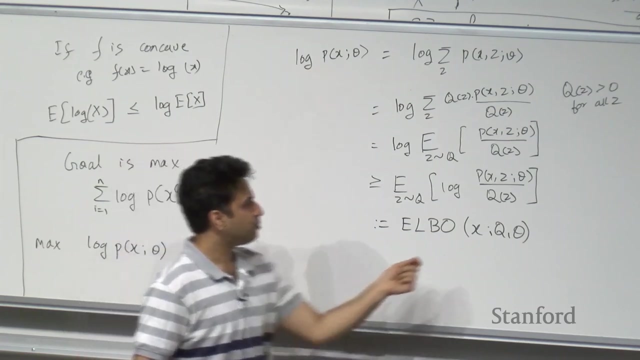 Right And Jensen's inequality tells us that the ELBO, you know, which is defined to be this term, is always less than or equal to our objective that we want to maximize Right, Which- which means now, if we find Thetas and q's such that we are maximizing the ELBO. 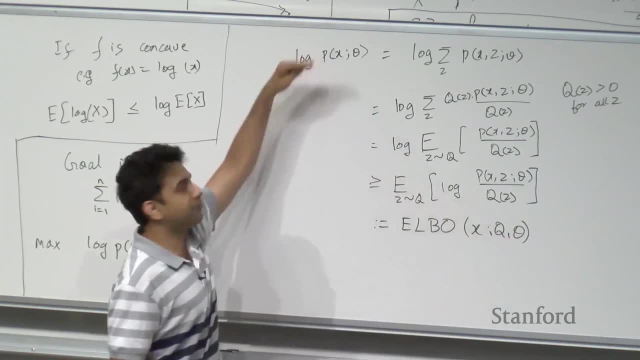 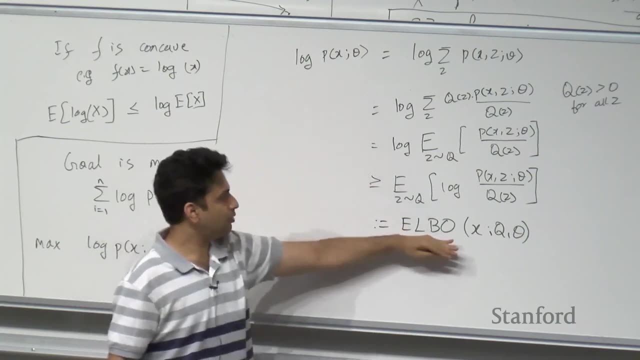 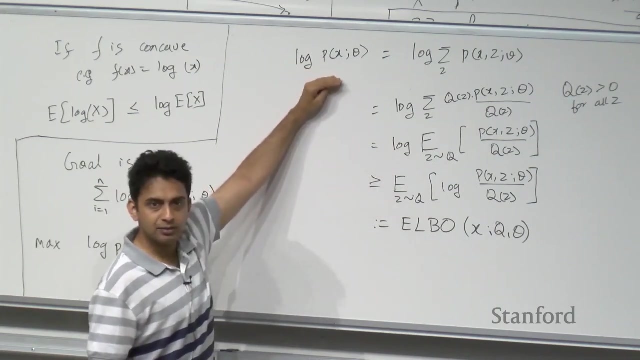 then implicitly, for the same values of Theta, log p of x is also going up. Does that make sense? Yeah, Does that make sense. ELBO is defined to be- is by Jensen's inequality. ELBO is always a lower bound for log p of x. our likelihood: 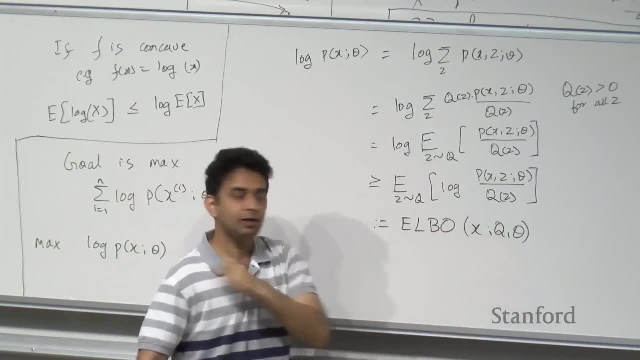 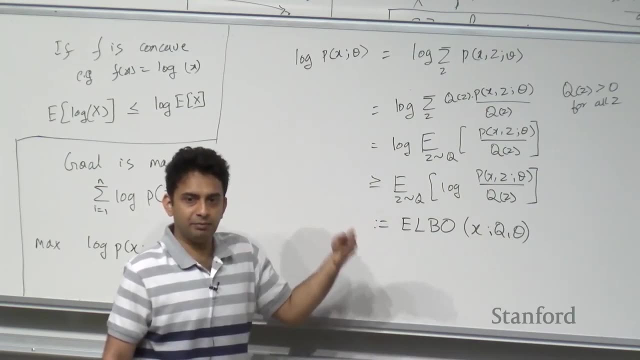 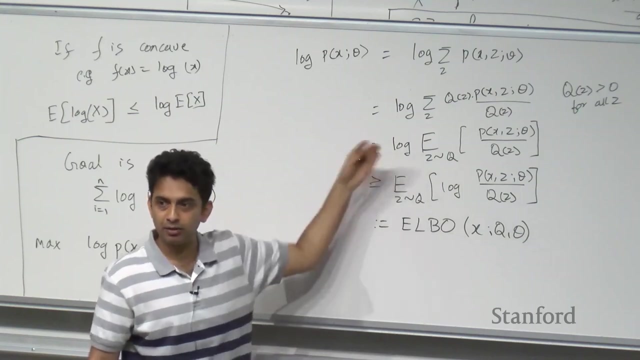 Both of them have Theta in them right Now. if we find values of Theta such that we are maximizing the ELBO, then it necessarily means that log p of x at that value of Theta is higher And Jensen's inequality gives us that inequality. 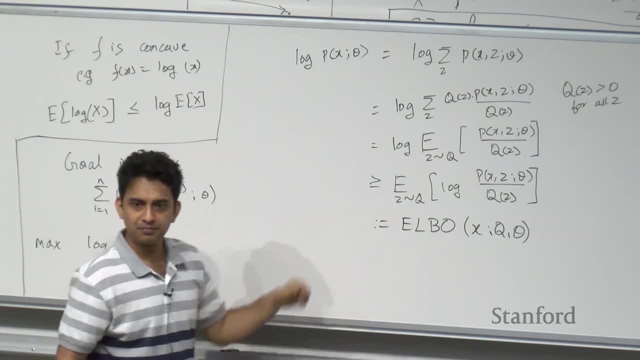 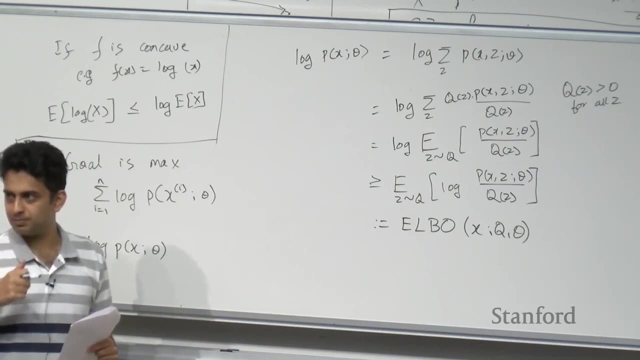 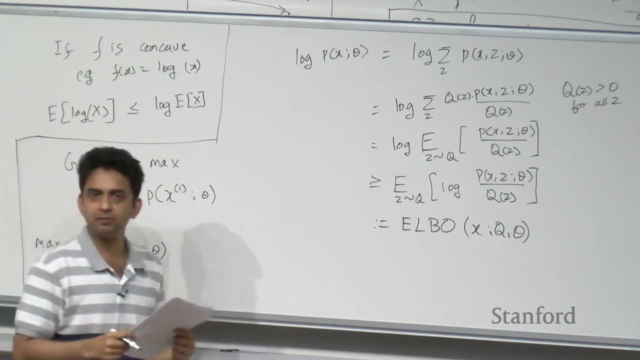 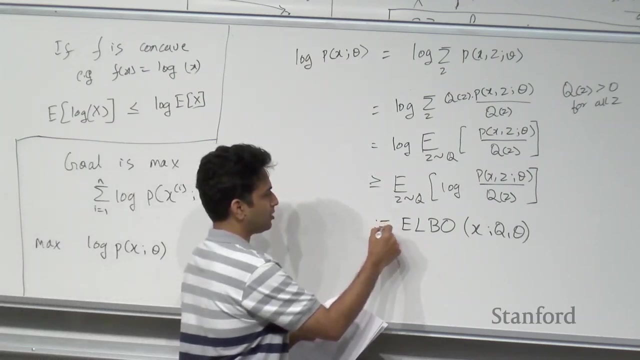 Yes, Question, We're going to- we're gonna come to that, Alright, So this is the. so this is the ELBO, And this term ELBO is, uh, something you will very commonly encounter if you are reading, reading research papers about, you know, a search engine. Yes, It's exactly the truth. yes, Right. So if we have high systematic for variable minimum value of S on the range value over this value, That would be, for example, you would be- that would be be- if you have veryofty low, you know. like, If you have very royalty in the range level, level B, it would mean that the我很 tall rival will be but訴診h very, very consistent over this condition. I, watching, will be able to get additional contract, will be will will be able to take it with maximum bench turn on the next scale life. 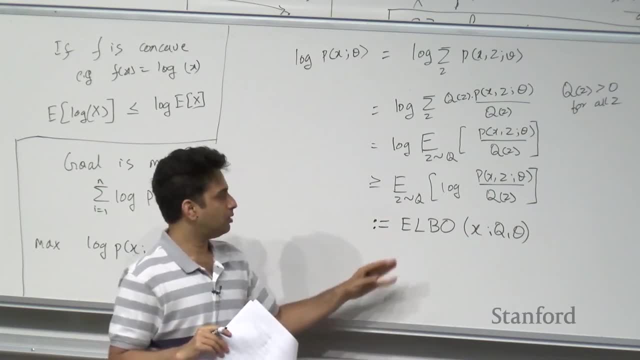 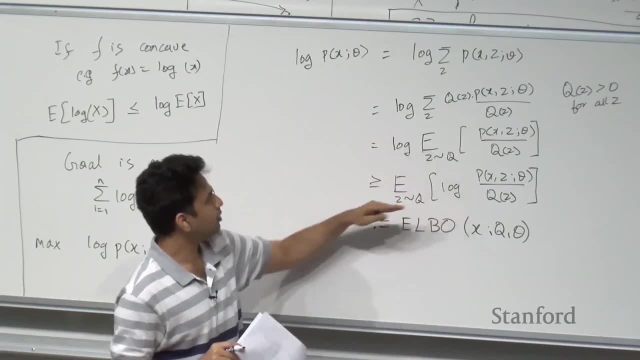 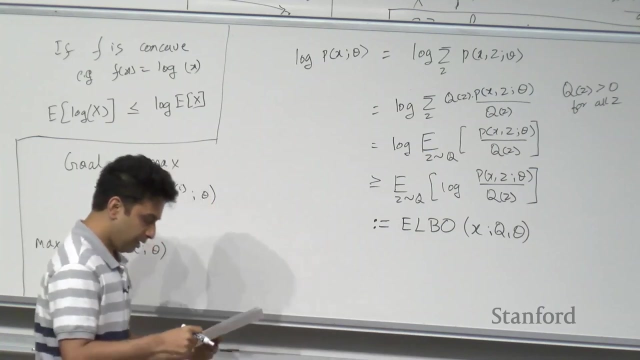 you know generative models or deep generative models. um, you know this- this is- this is a widely used term And ELBO means you know the- the- the lower-, the lesser side of the Jensen's inequality of log- log p of x right. 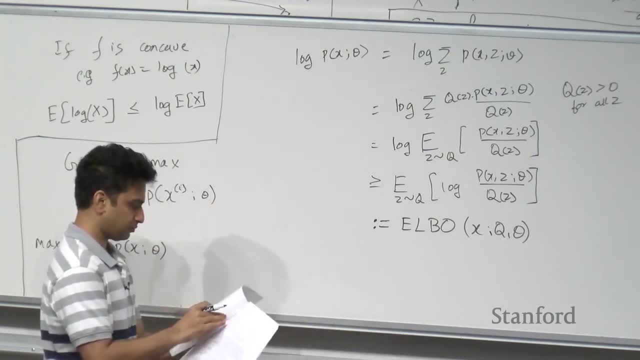 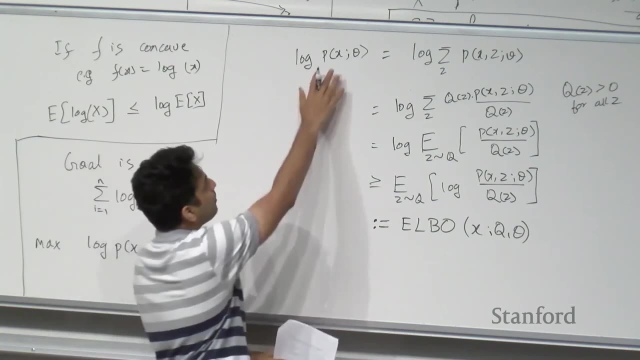 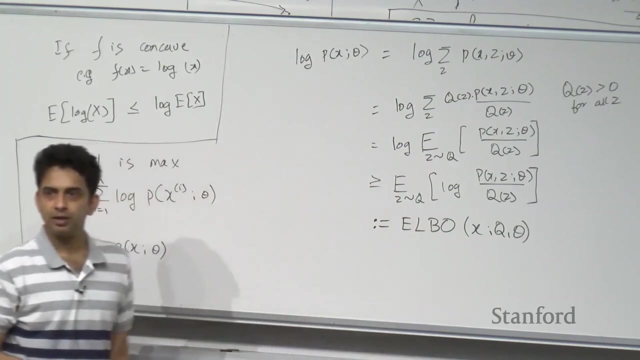 And our goal is to now-. before we go into our goal, let's- let's make a few more observations Now. log p of x is greater than equal to ELBO at all times. That's, uh, what Jensen's inequality says. 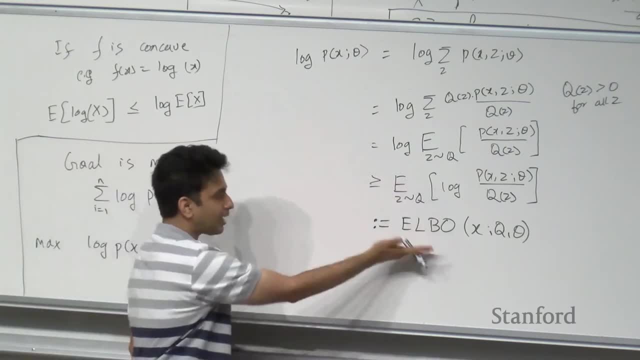 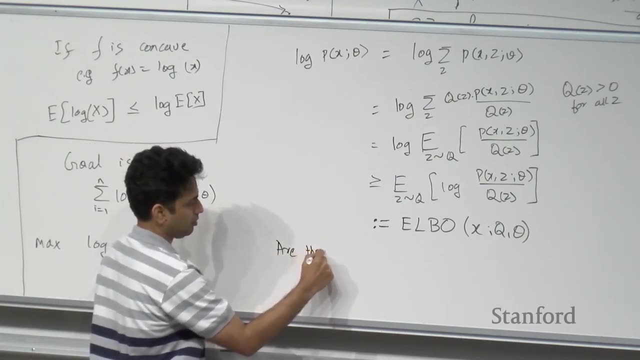 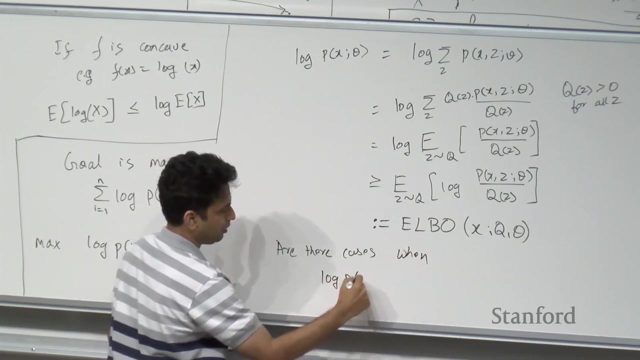 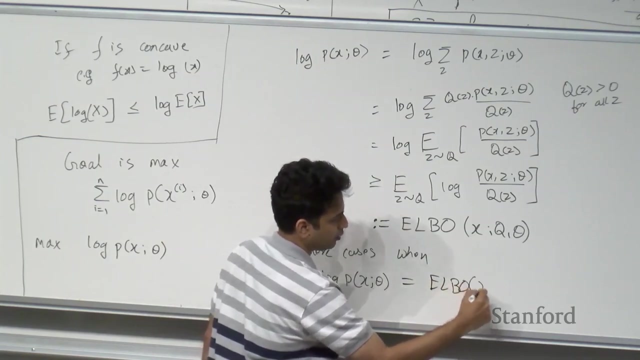 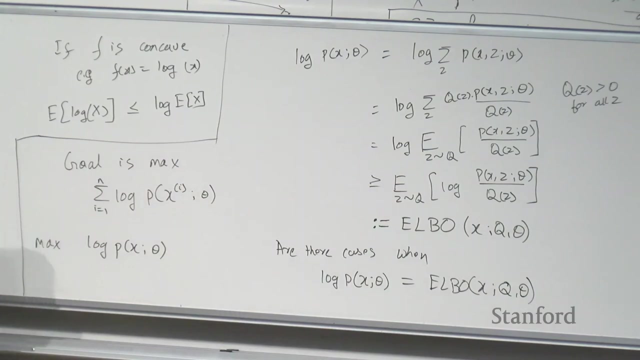 But are there cases when log p of x is exactly equal to the ELBO right? Are there cases- are there cases when log p of x- theta is equal to ELBO of x, q and theta? And the answer is yes. 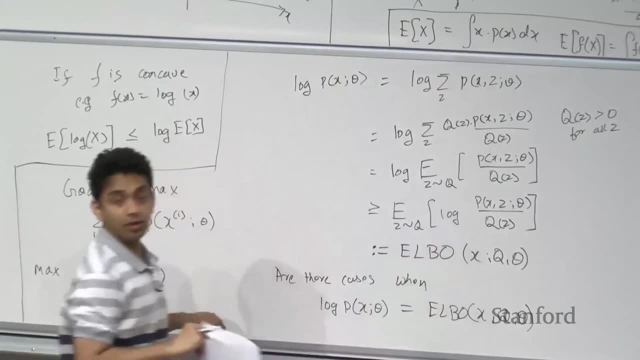 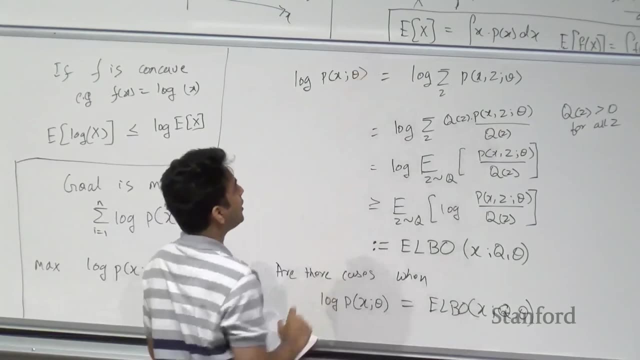 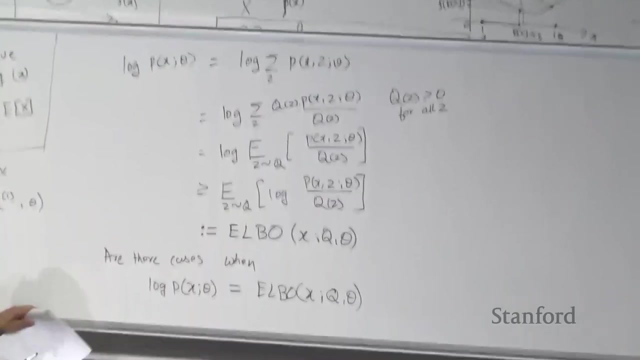 It is, yes, because of the second part of Jensen's inequality that we saw right. So, uh, Jensen's inequality, um, we also saw that if f is strictly convex, log x is strictly convex, right, If, uh, f is strictly convex. 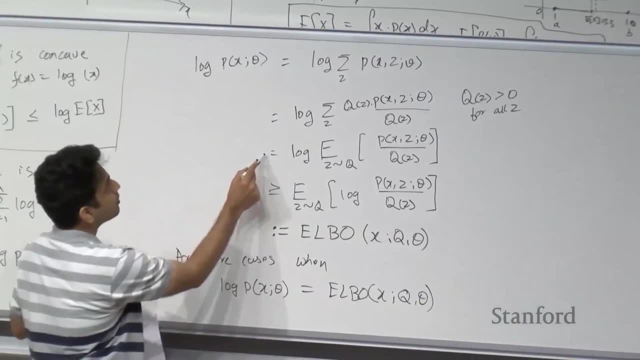 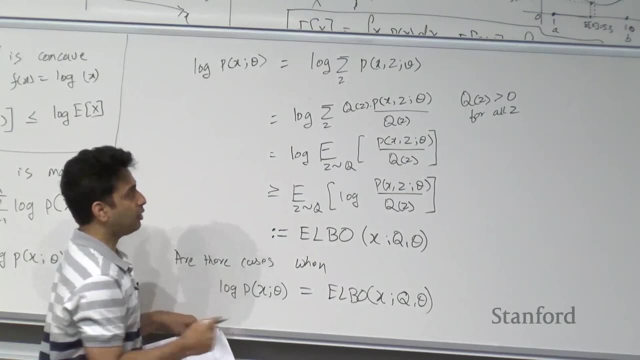 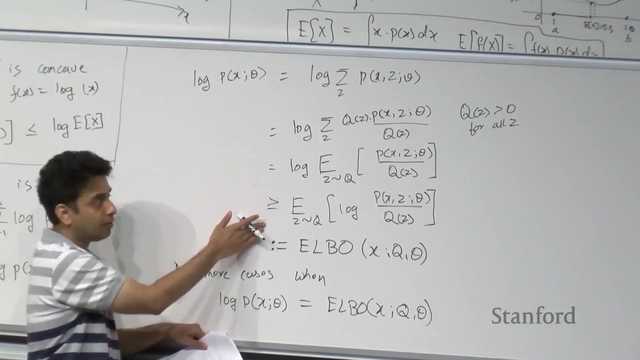 then expectation of f of x eq-, expectation of f of x equals, uh, uh, f of expectation of x if, and only if, x is a constant right. So this is one side of Jensen's inequality. this is the other side of Jensen's inequality, right. 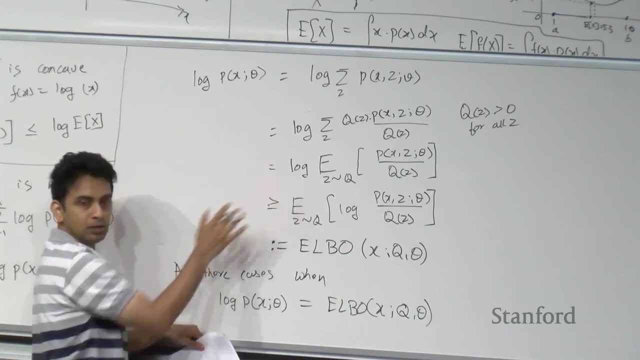 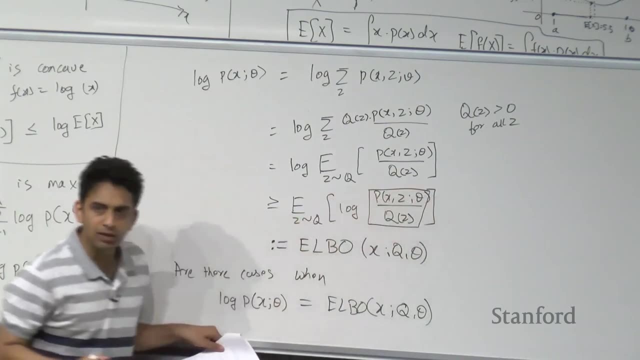 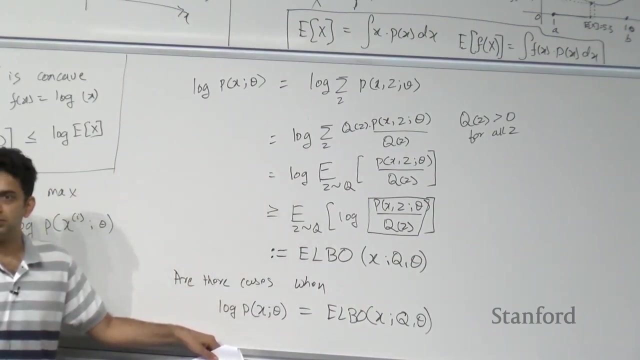 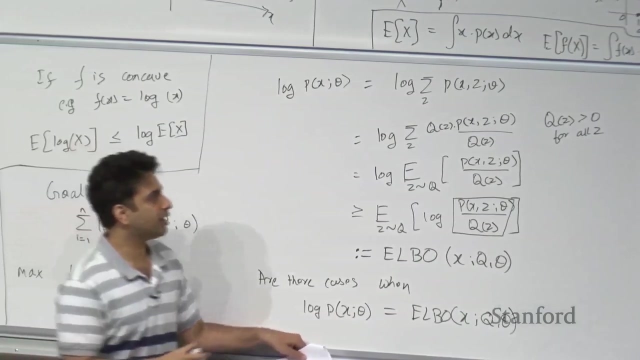 And the two will be equal if, and only if, the term inside is a constant. That's what uh, uh, Jensen's inequality, uh, told us. because log is strictly concave, Yes question. In this case, we want- we want this entire term over here to be a constant. 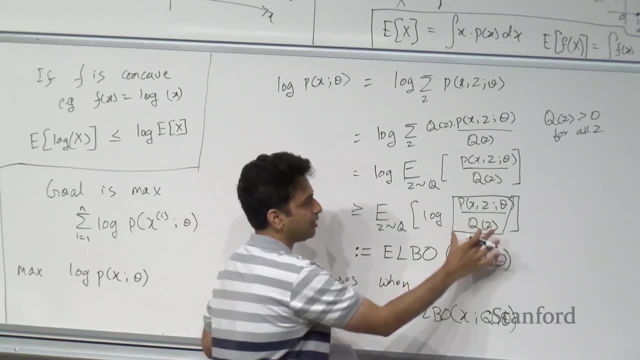 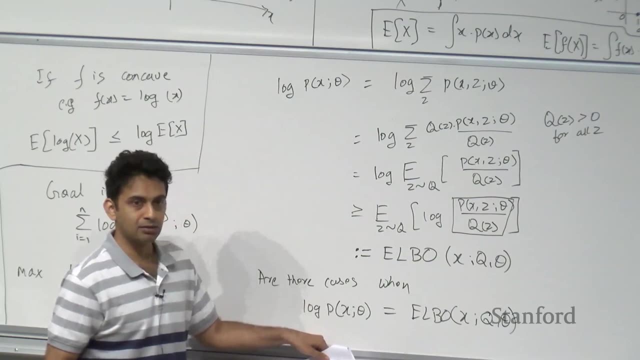 Now are there cases? so the next uh question is: are there? you know under what circumstances is this entire term over here always a constant That's- that's- that's what you're gonna answer next. It has to be- it has to be independent of z. 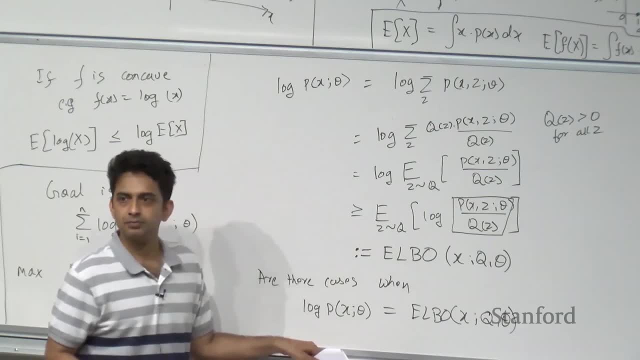 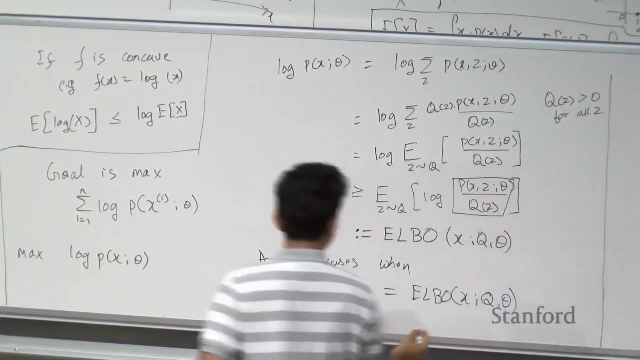 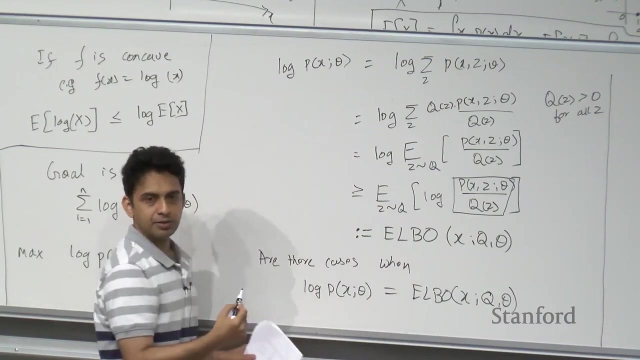 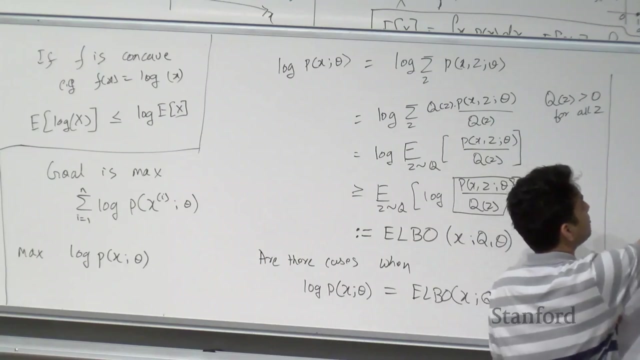 So it is constant with respect to z right. So the question now is: in order to make this inequality an equal, because- because log is- because log is strictly concave, the inequality becomes an equality if, and only if, p of x. 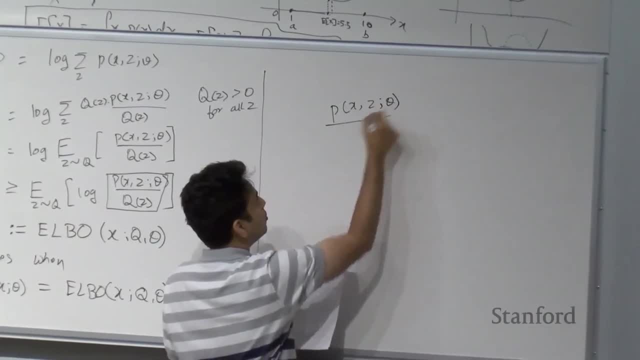 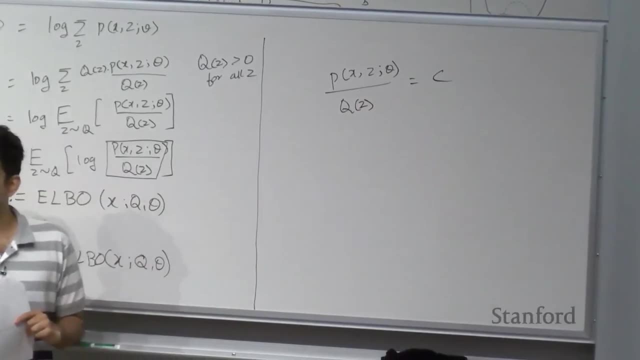 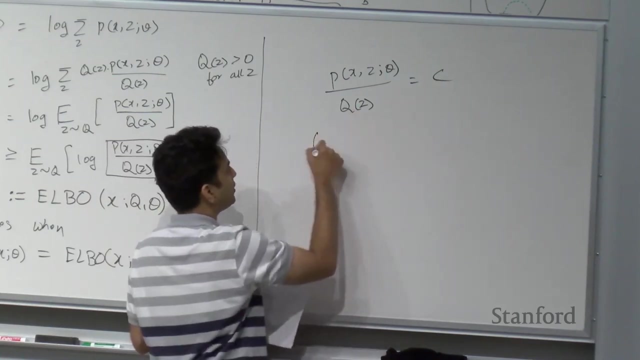 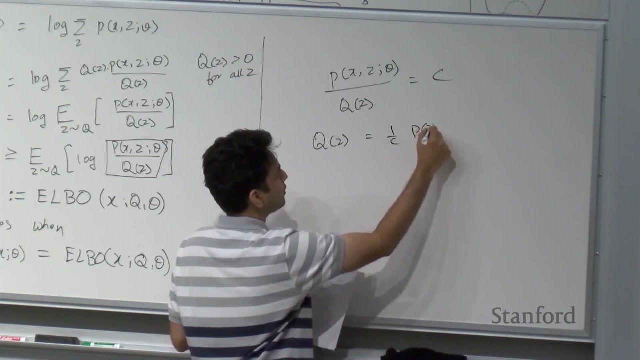 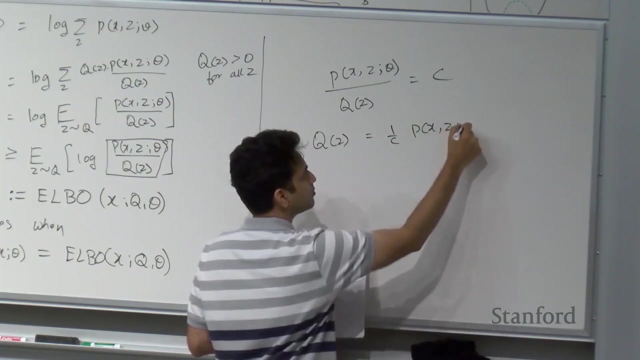 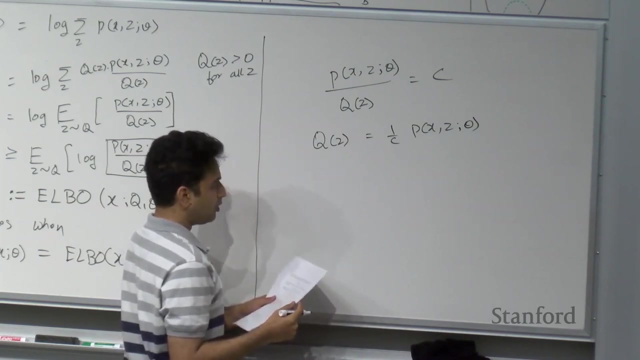 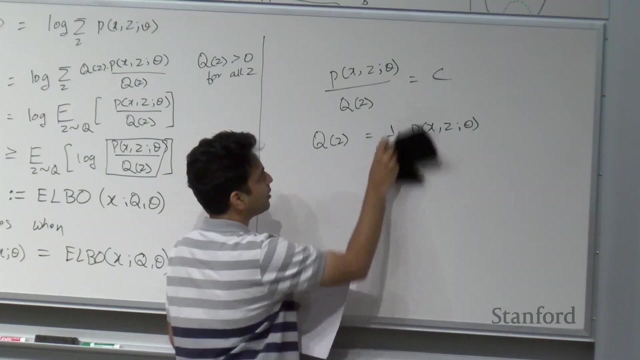 z Theta over q of z equals some constant c right. And now this implies that take q of z over there. q of z is equal to 1 over c times p of x comma z right. And we also know that because this is just a proportionality constant. 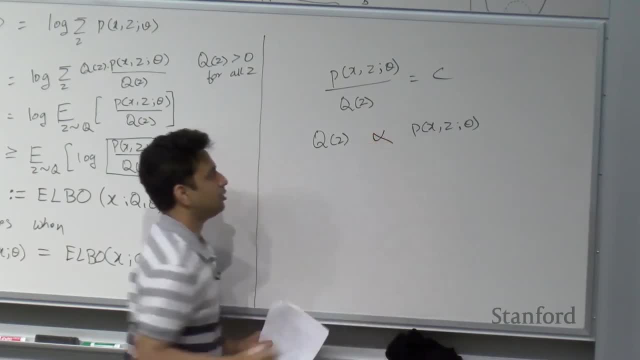 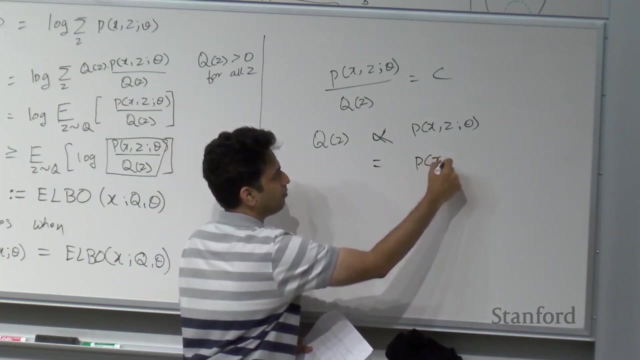 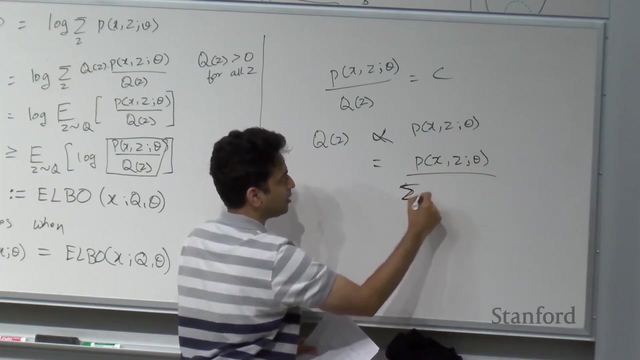 we can write this as q of z is proportional to p of x comma z. So q of z is just proportional to p of uh x comma z. And in order to make this equal to- we just use the uh. calculate the proportional normalizing constant. 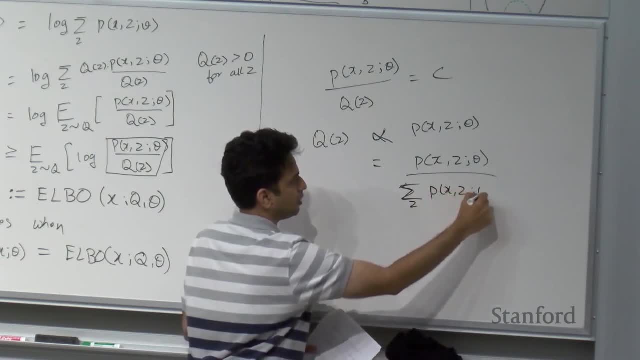 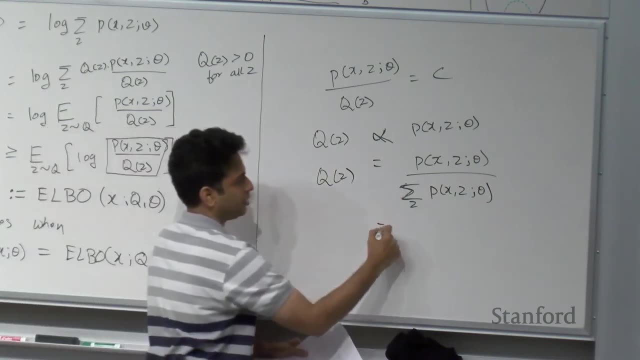 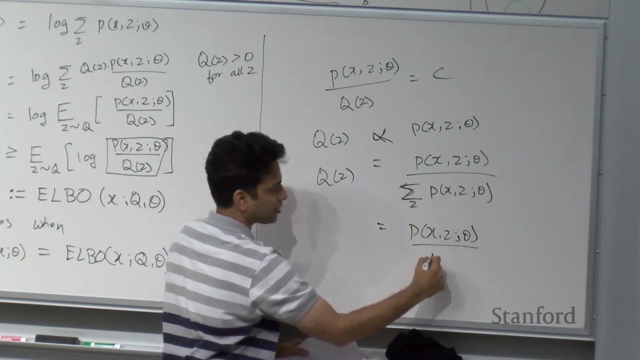 that you're summing over z, p of x comma z Theta, Right, And this is basically p of x comma z Theta divided by. when you marginalize out z, you just get p of x Theta and this is equal to p of z given x Theta. 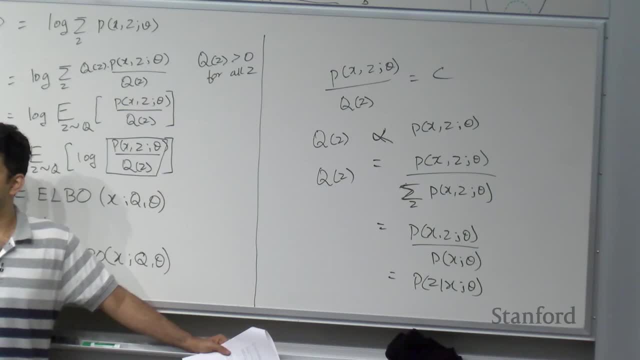 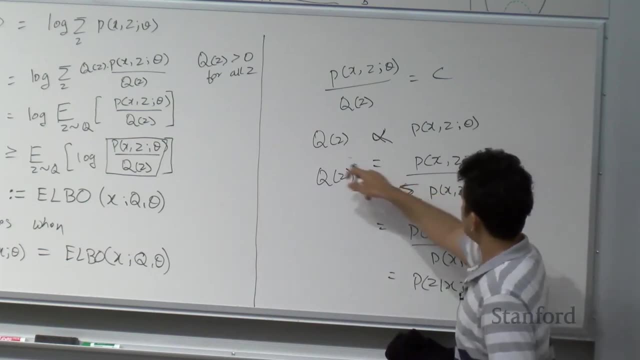 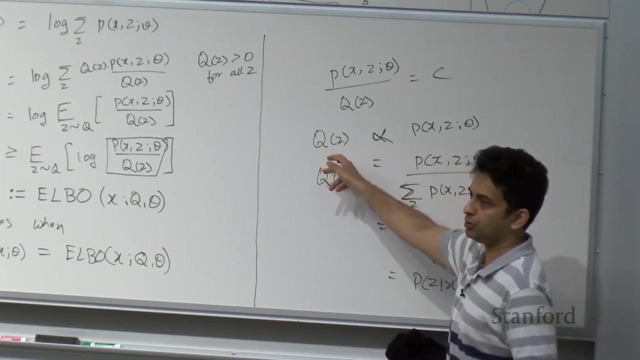 So the question is: why did we normalize it with p of x? Yeah, So, because q of z is proportional to this and in order to- and we know that this is a probability distribution, which means it has to sum up to 1.. 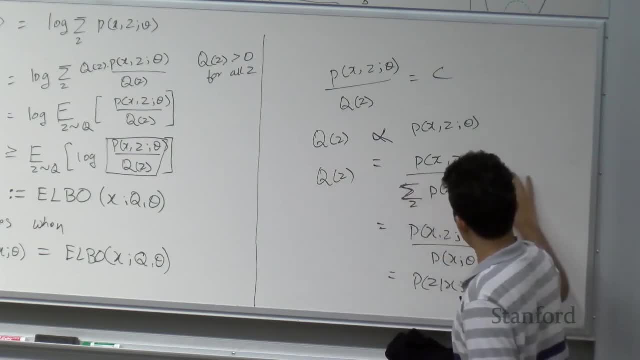 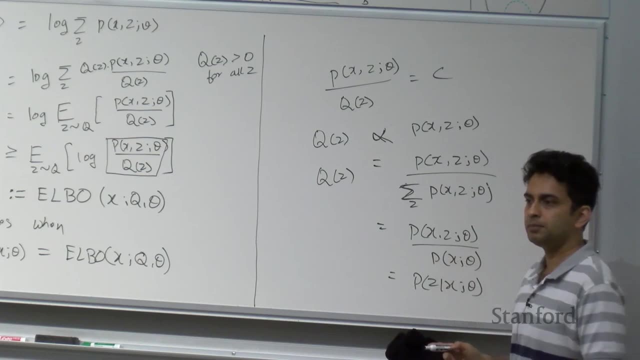 So this must ne- the normalizing constant- necessary- must necessarily be the uh um, sum of- sum of this. Is there another question? Yeah, So the denominator is this term, that is summed over all possible values of z. 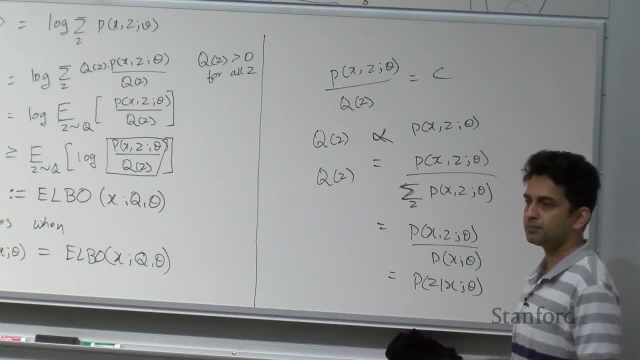 So this is a distribution over z. P of xz could be anything, x could be continuous. okay, Q of z is a distribution over z that must sum up to one right And that's proportional to uh. p of x, uh x, comma, z. 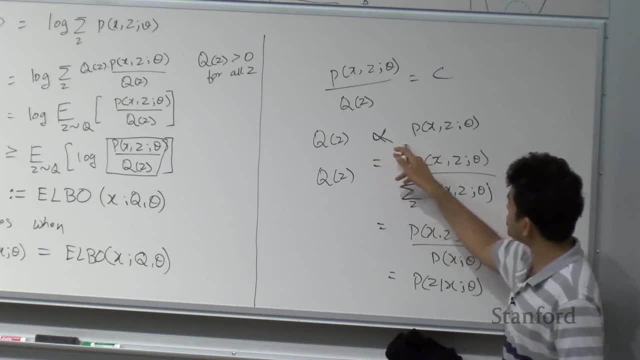 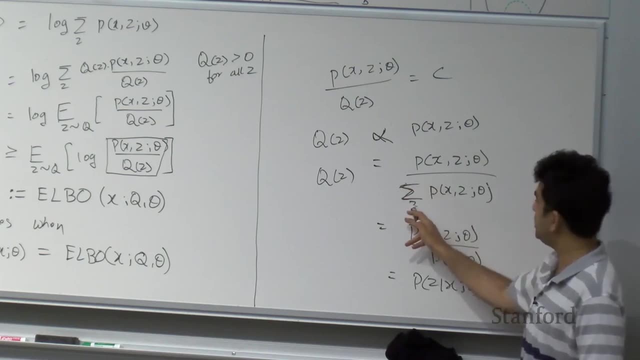 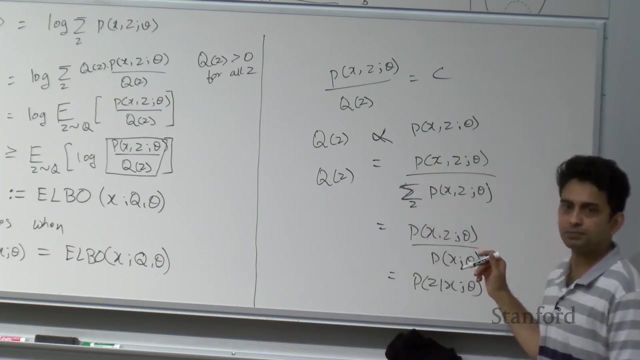 And uh the- the-. it is proportional and the corresponding normalizing constant must necessarily be the- the- the- the sum over the numerators for all possible values of z, because it must- it must sum up to 1, right. 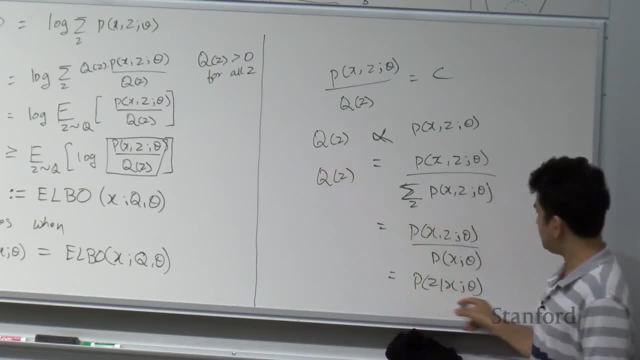 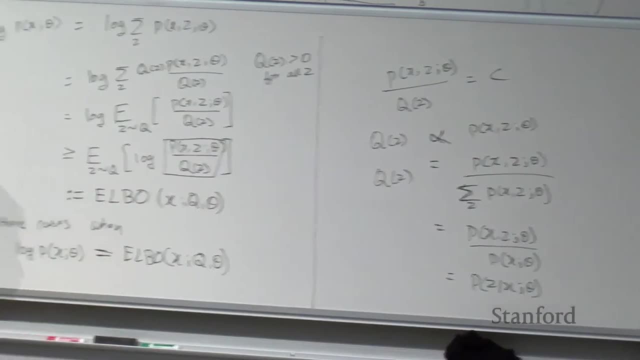 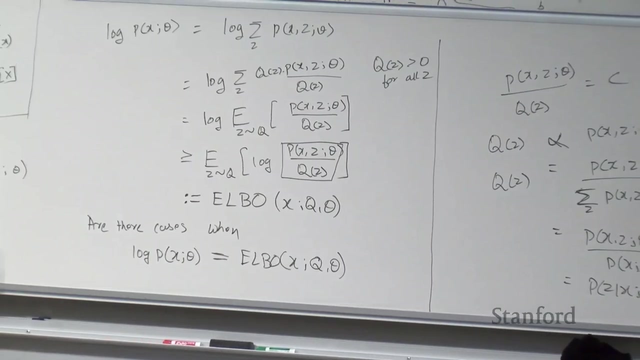 So when Q of z equals P of z given x, then Jensen's inequality will change into an equality right. Lots of moving parts. yes, So we started with- we started with log P of x, right, And wrote it out as- as. 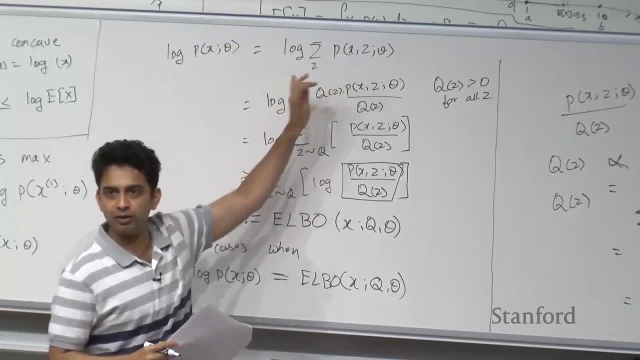 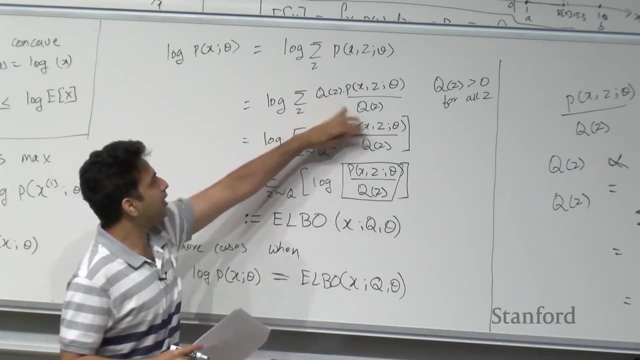 you know the sum over z of the joint. you know, and there's- there's nothing fancy going on here, right? We're just marginalizing out the um, um, um z, And then we multiply and divide it by some arbitrary distribution Q. 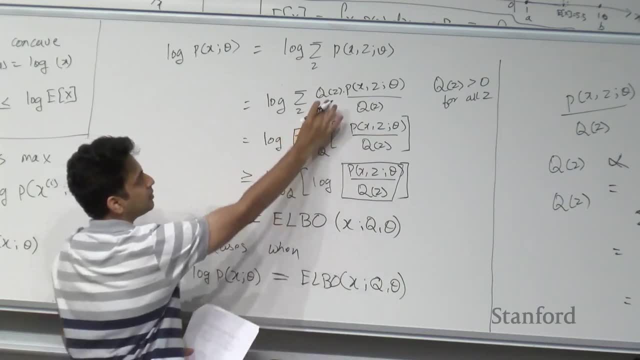 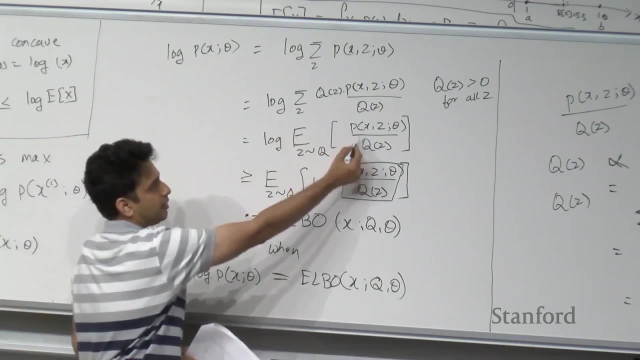 And by multiplying it and dividing it. this- the numerator allowed us to write it in the form of uh, an expectation right, And the uh and this stayed in the denominator, And once we wrote it as an expectation, we had log in the expectation right. 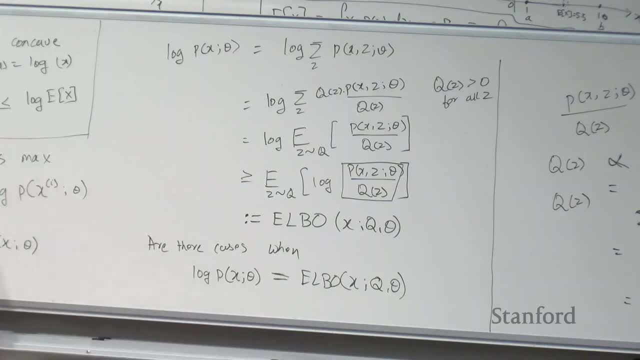 So initially we started with the log likelihood and therefore we use the concave version of Jensen's inequality. So this log and this expectation are then swapped right And we get a greater than equal to expectation of log right. And once we get this, you know. 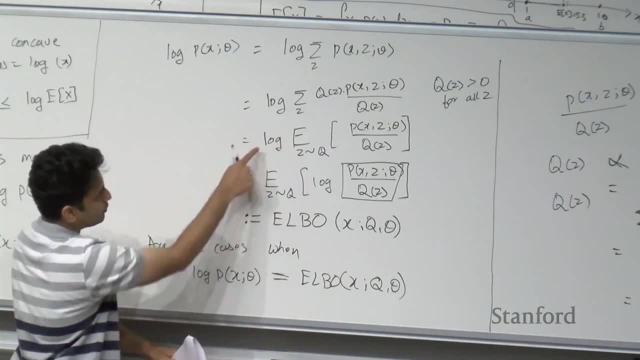 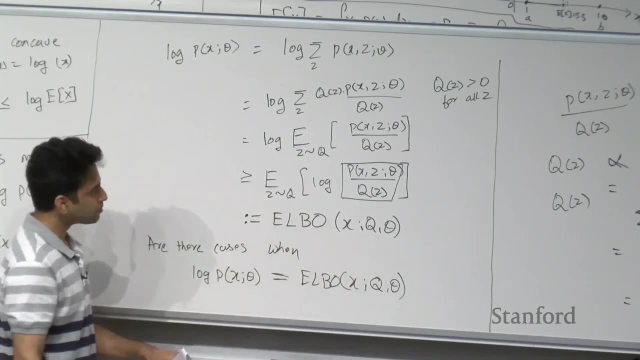 this is basically Jensen's inequality, The one side and the other side of Jensen's inequality. We call the lower- the lower end of the Jensen's inequality, we just call it ELBO, we just give it a name right, And then we use the- the uh. 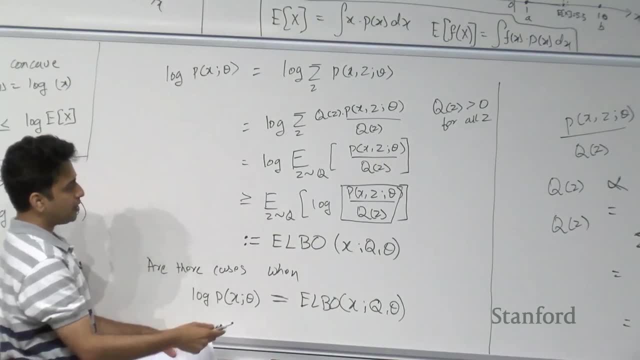 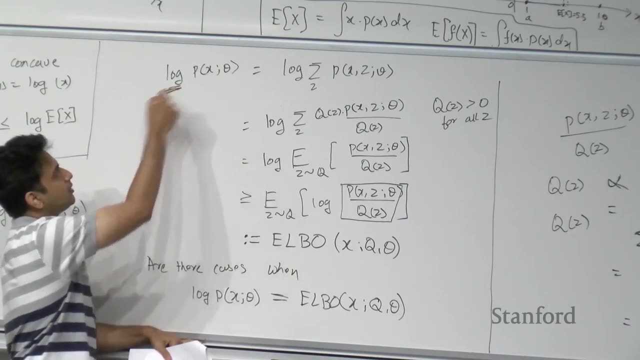 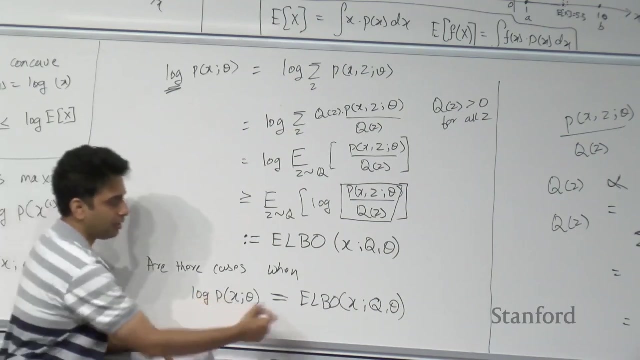 the corollary of Jensen's inequality, to look for conditions when this inequality will be exactly equal to right. And because log- because log is strictly convex- the corollary of Jensen's inequality gives us a condition when this inequality becomes an equality, and the condition is that this term must be a constant. 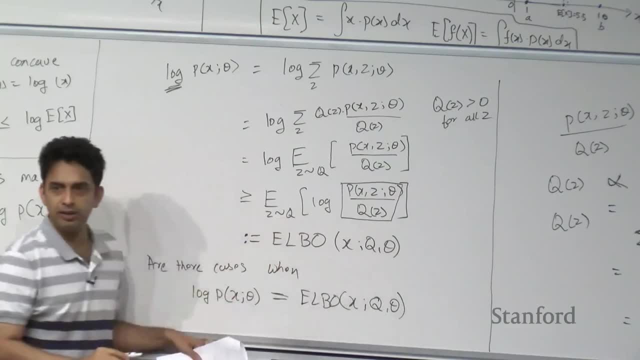 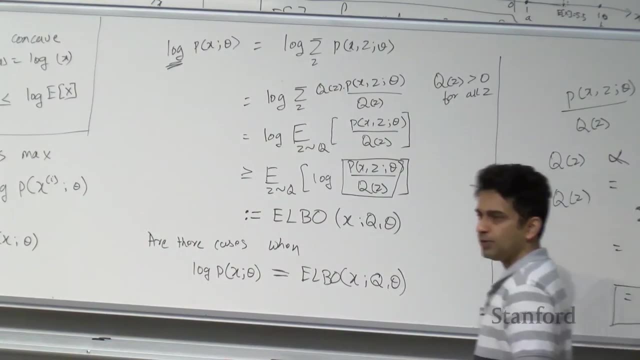 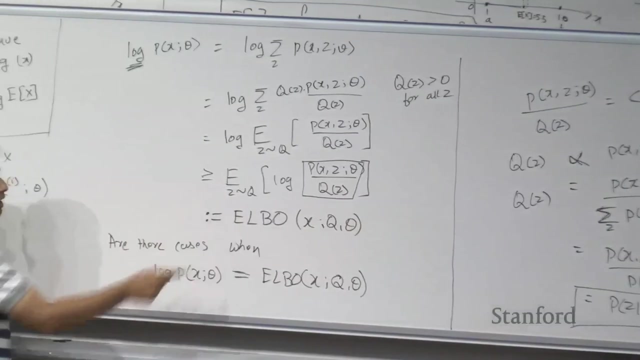 And then, in order for this to be a constant with respect to z, it is necessarily the case that q of z must be equal to the posterior distribution of z given x right. Whenever q equals z given x at that value of theta, then Jensen's inequality becomes a strict- becomes an equality right. 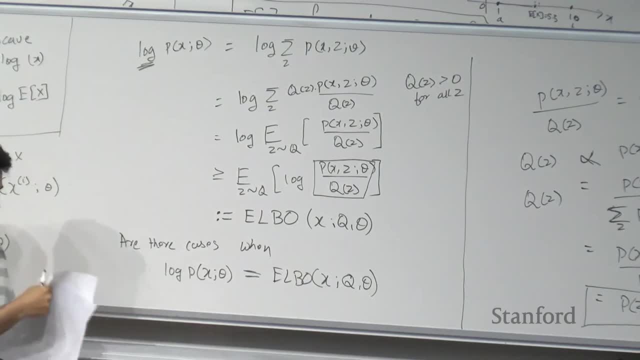 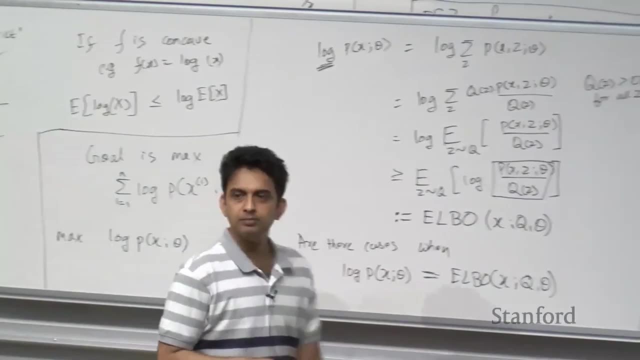 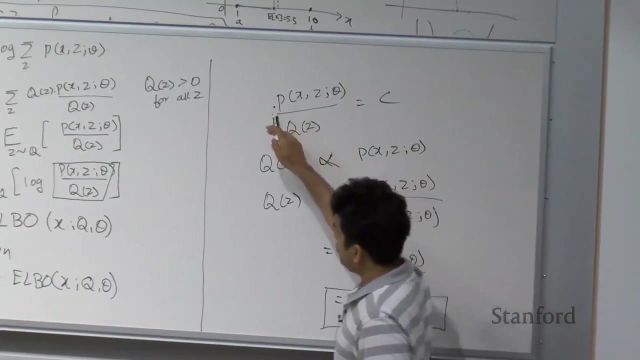 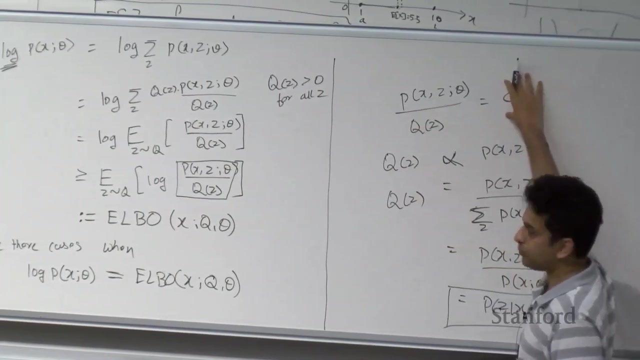 And now, given these two yes question, So y is uh, uh, uh, yeah, this All right. So we want to find the condition that p of x, z, divided by q, this is equal to some constant right. 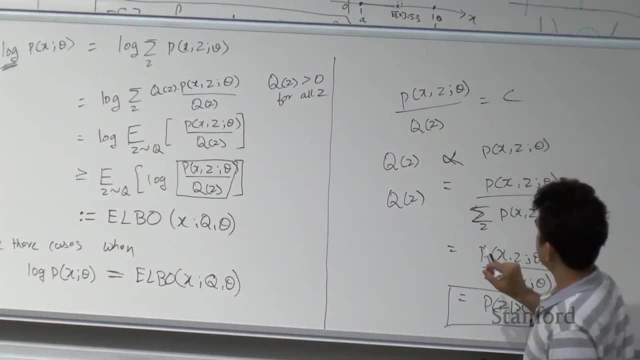 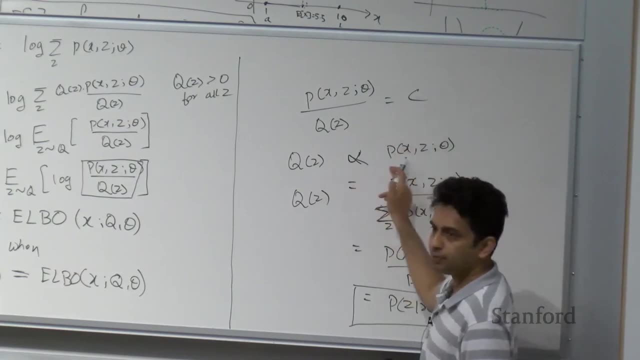 So now, let it be equal to some unknown constant c, right? So you can take q of z over here, right? And once you take it over here, this becomes proportional because of some constant times, right? So now what we- we also know that sum over q of z equals 1, right? 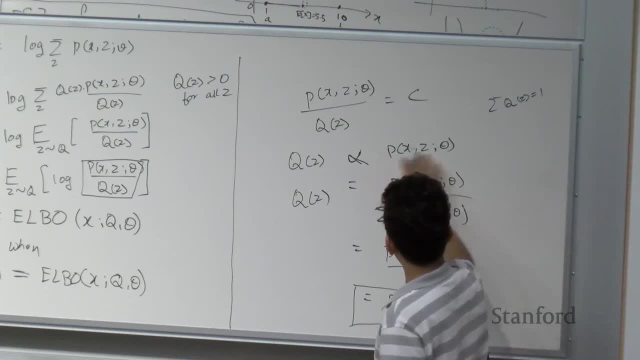 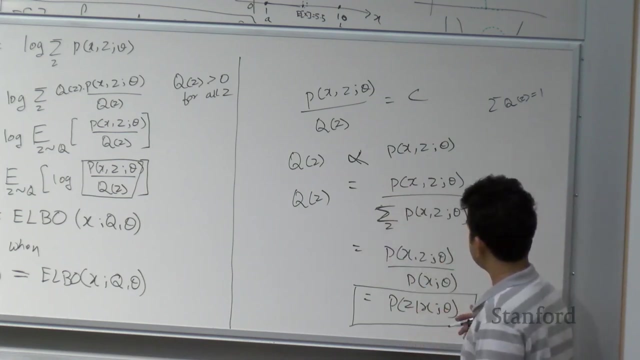 Which means, um, the sum over all of- all of the right-hand, uh, uh terms must be equal to c itself, right, And we divide it by c and we get exactly. So q of z is equal to the posterior of z, given x at that value of theta. 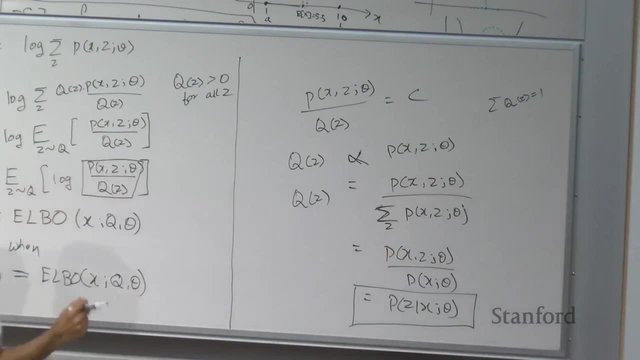 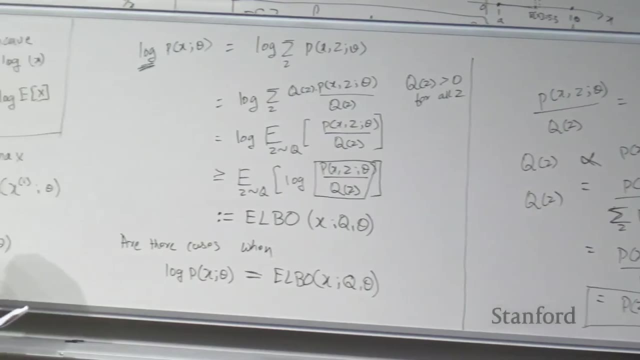 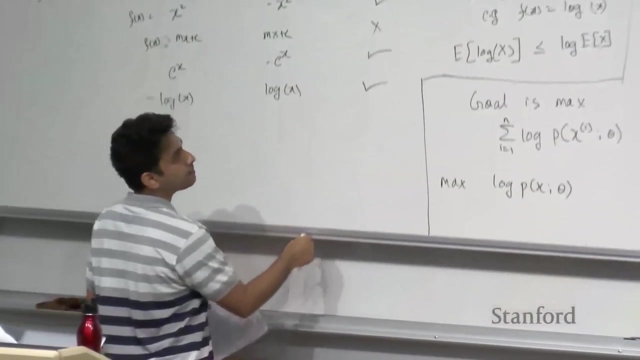 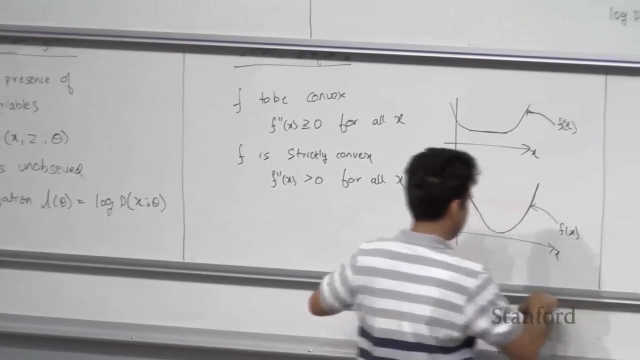 Thank you, Thanks for asking. Um, okay, So, based on this, we-, we com-. we write the: uh, the EM algorithm, or the more general form of the EM algorithm. right, Okay, of the EM algorithm. We call it the more general form because, throughout this- throughout this setting. 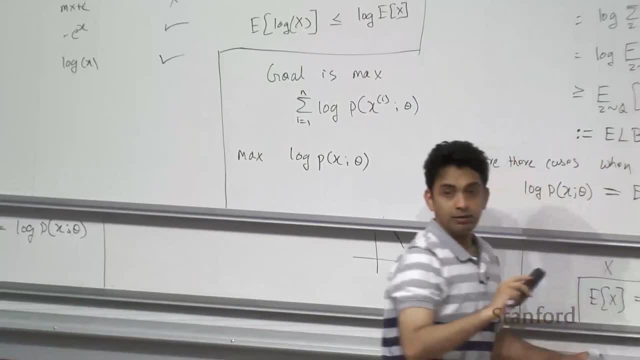 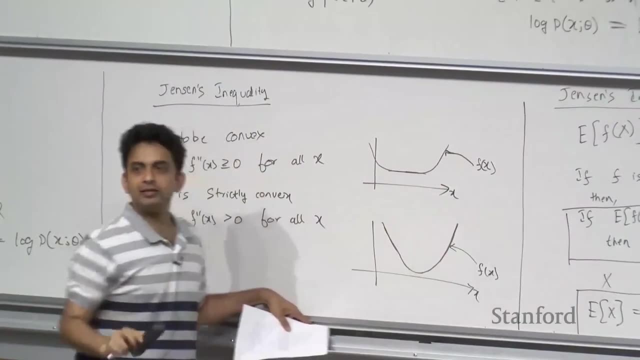 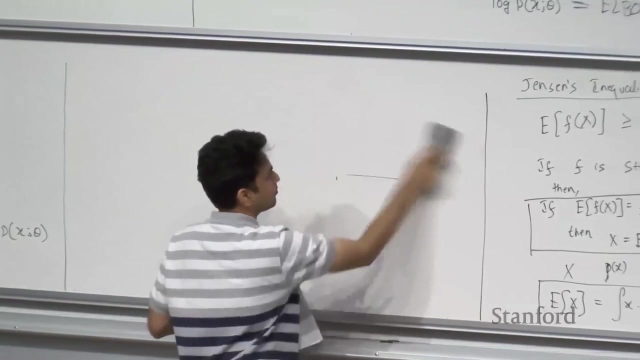 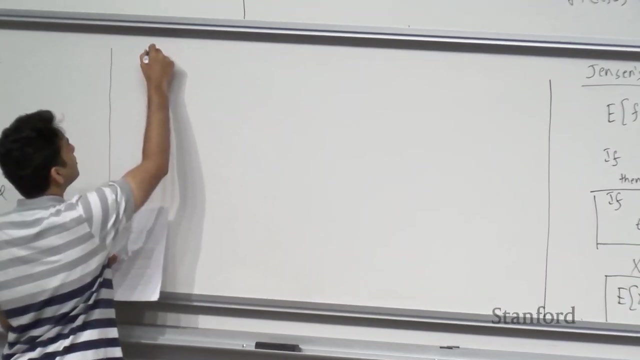 we have not assumed any specific form for P of x and z. right, It could be the mixture of Gaussians, it- it could be any algorithm. This derivation holds for any such latent variable model. all right, So that gives us the uh algorithm. 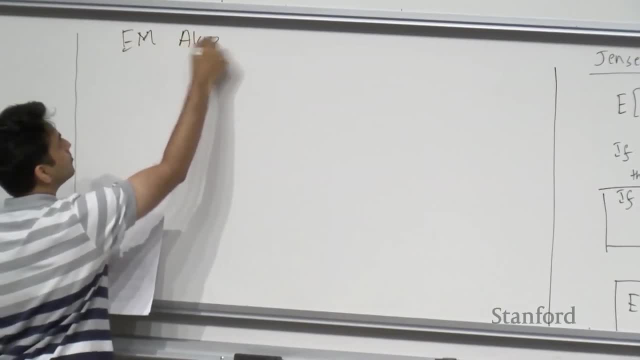 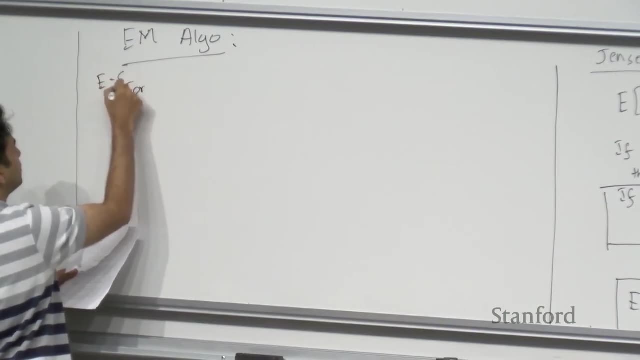 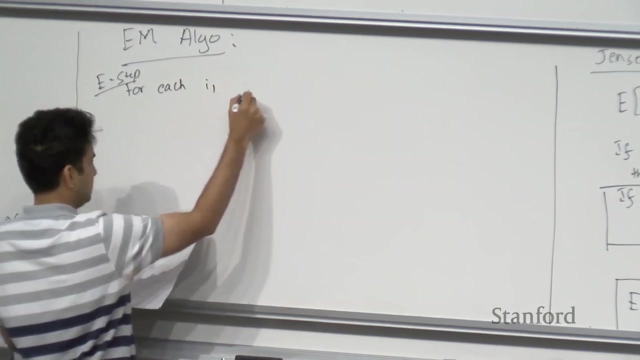 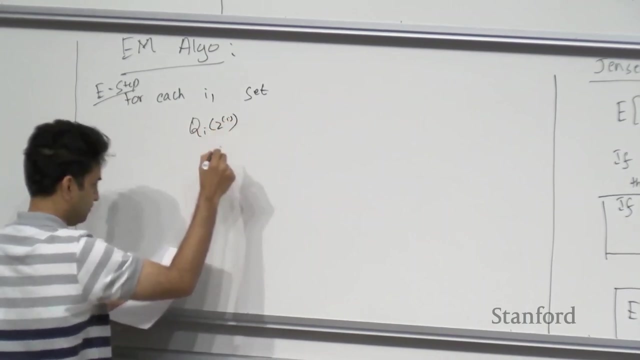 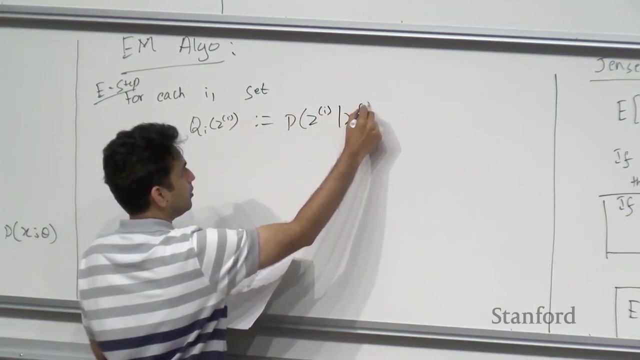 So the EM algorithm- the EM algorithm basically tells for- so we have the E-step For each i set. qi of zi is equal to p of. Forget the fucking setup. zi given xi, Theta and the M-step okay, 7,. 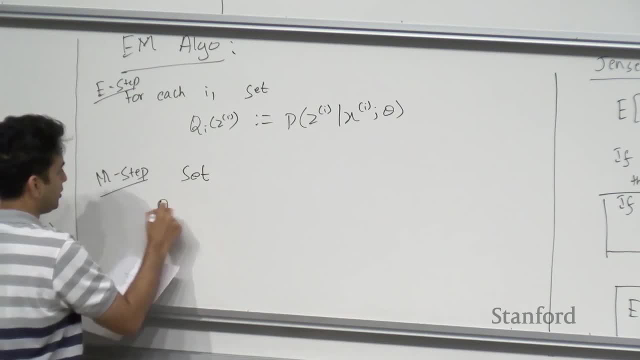 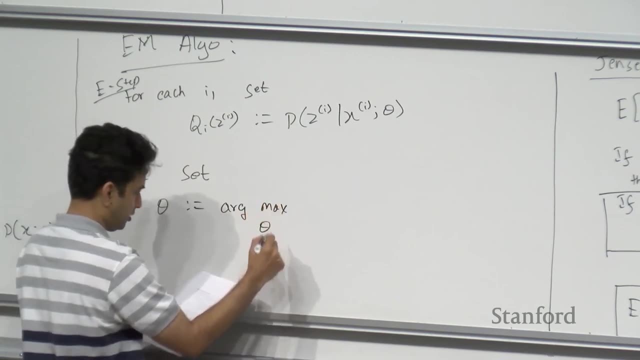 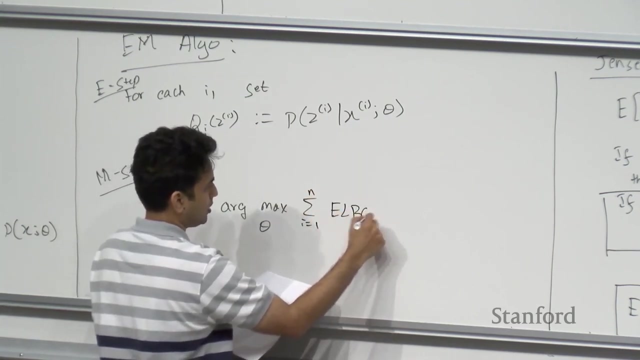 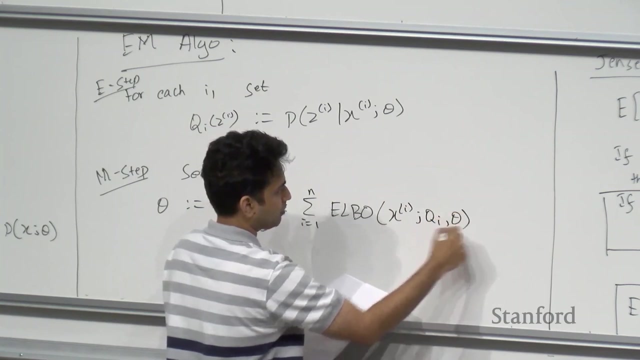 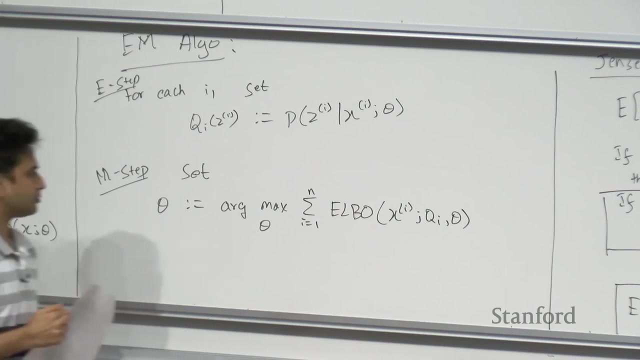 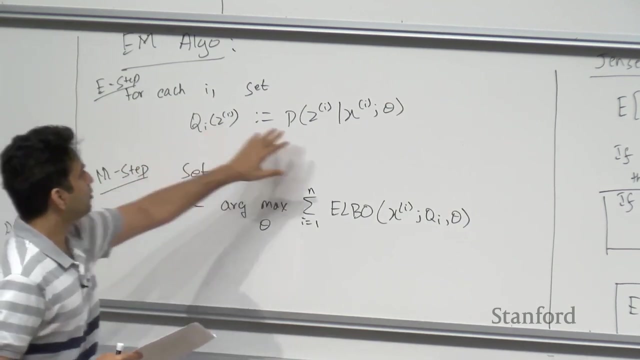 set Theta equal to R, max Theta of i equals to 1, equal to 1 to n, albo x, i, q, i, comma theta, right. So what did we do? We basically, um, we basically get this EM algorithm where the corresponding E-step is to set q to be the posterior distribution of P of z, given x. 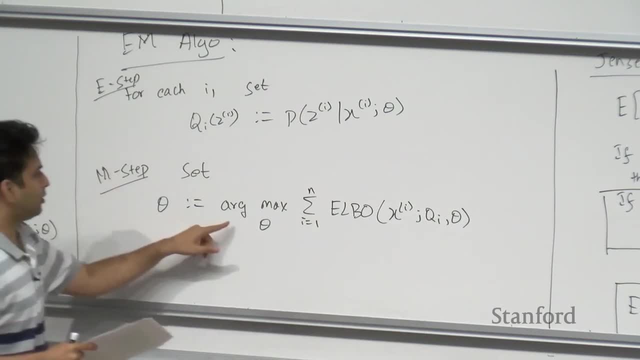 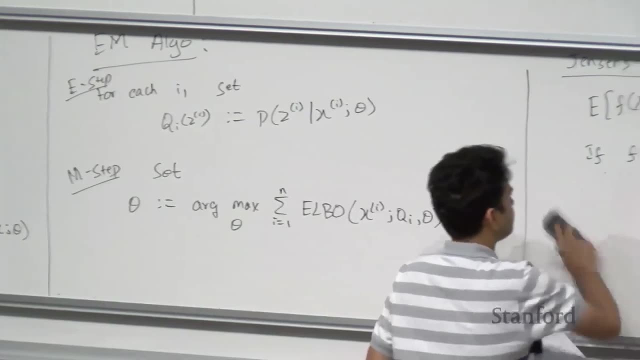 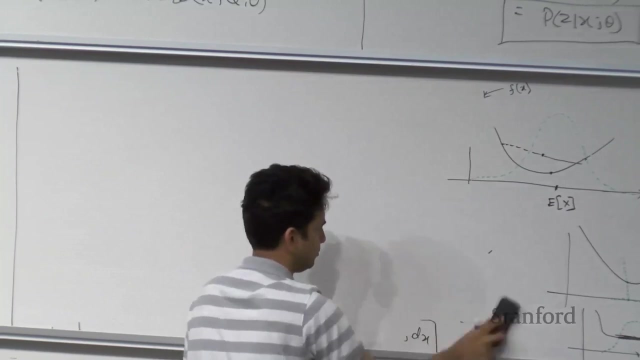 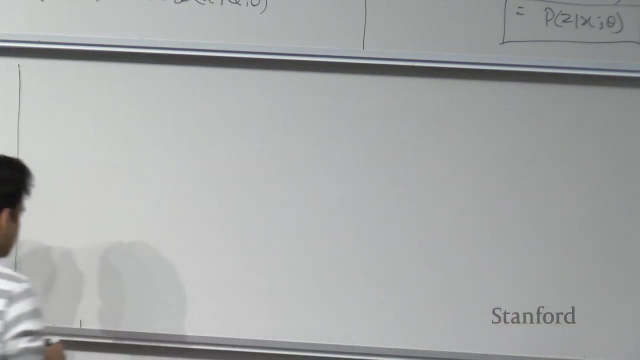 And in the M-step we set theta to be equal to the argmax of the albo. Now, why will this- why will this work? To see why this works, let's see this diagram. Now let's suppose this is theta. 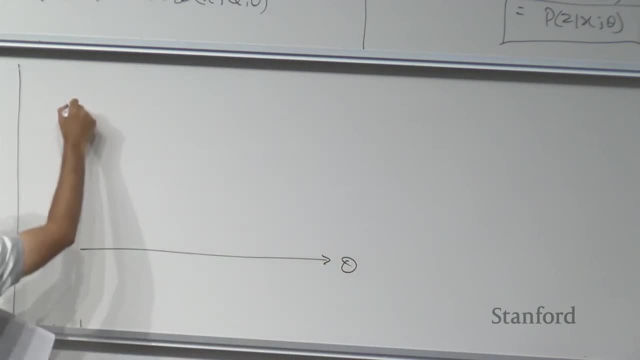 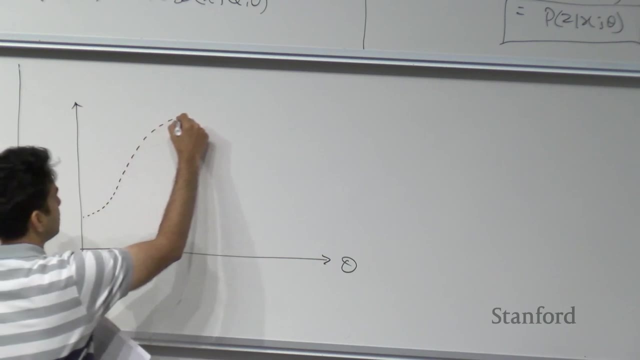 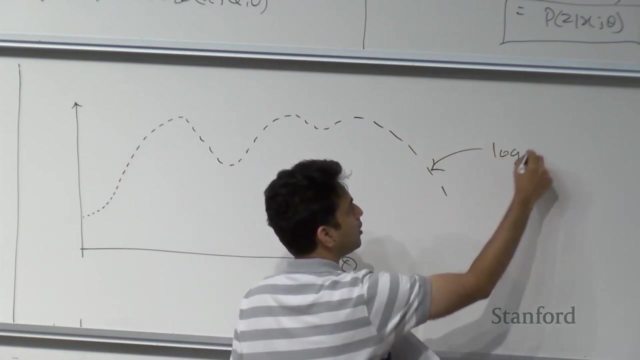 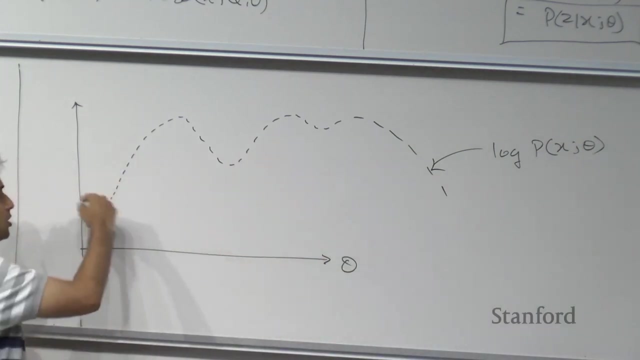 It's not x, this is theta right And this is- is- is arm. So let's assume this is our-. so this is log P of x, theta right. As we vary, theta log P of x gives us different values. This is not the density. 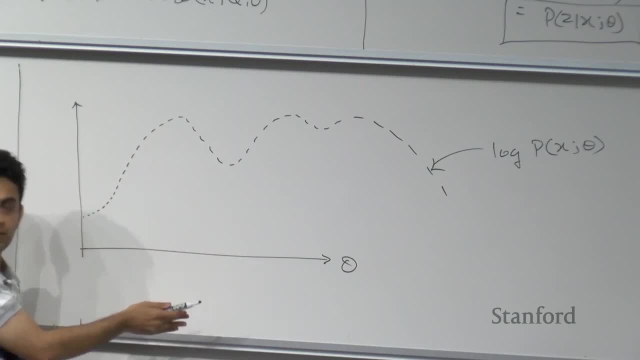 this is the likelihood, because the x-axis is theta and not x, right, And it's a dotted line. because we don't know it right, We- it- it is hard to calculate. We have to marginalize out x, which may be an integral. 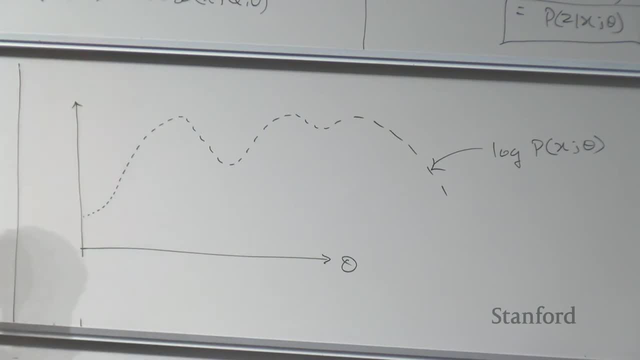 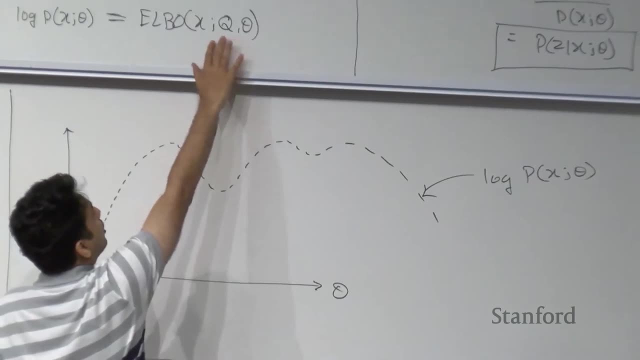 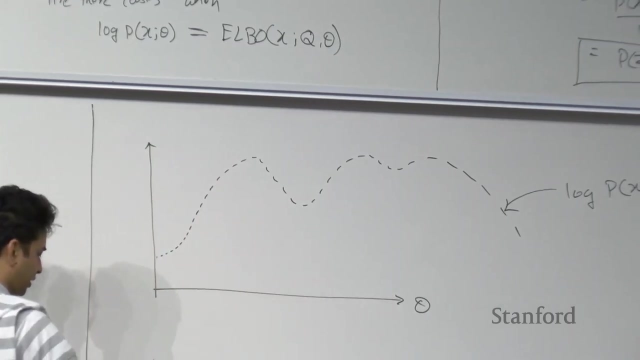 And what we got from this albo is that for any given value of q, the albo of-, albo of- of x for q and theta will always be less than or equal to log P of x. That's what Jensen's inequality uh, gave us. 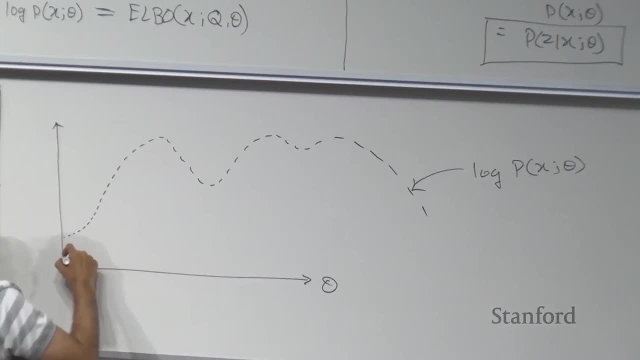 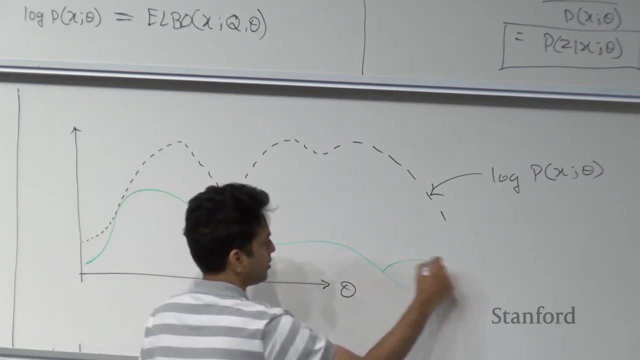 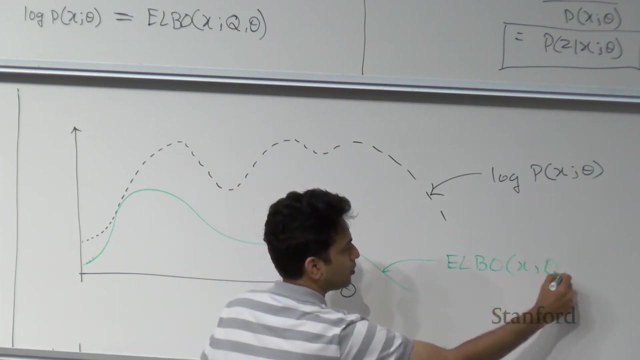 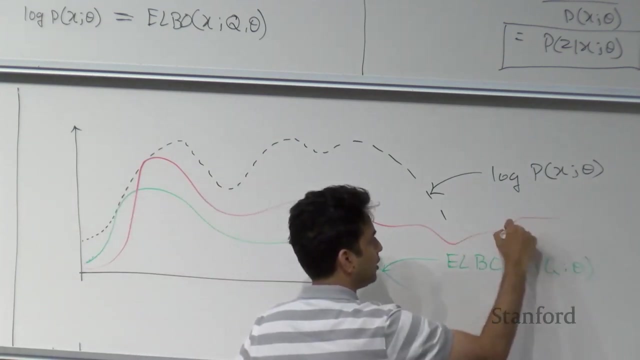 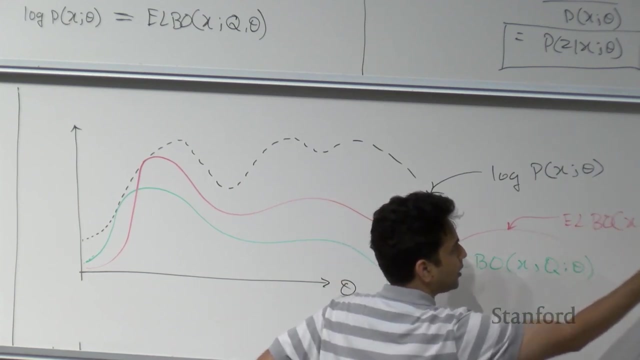 So Jensen's inequality tells us that. you know, this is- I'll write this as-. this is one possible albo x, q and theta. And let's consider another albo right. So, for example, this is another albo x, q, theta, right. 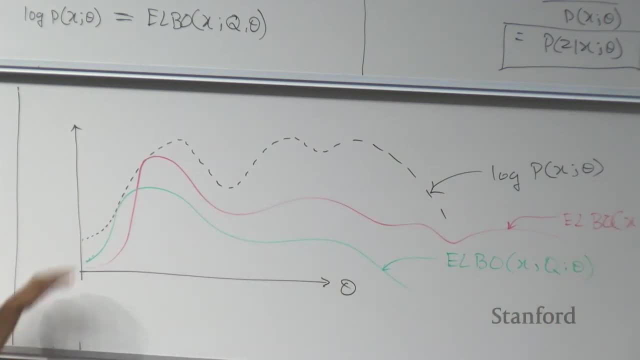 So for different choices of q we get different lower bounds of P, of x, right, And what Jensen's inequality tells us is that um or- or the corollary tells us is that for a given value of theta, let's- let's assume this is our randomly she-. 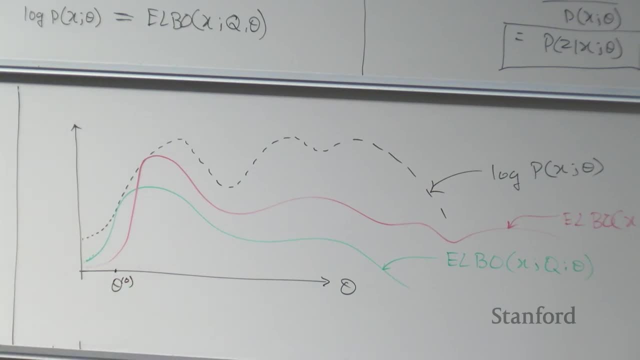 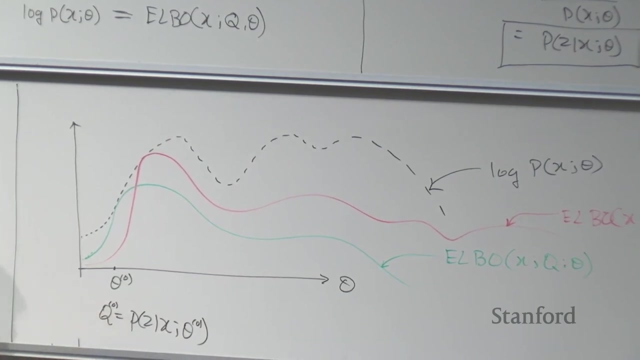 randomly initialized theta of 0, right. For this value of- of uh uh theta. if we choose q to be P of z, given x theta 0, for this choice of q, let's call it q: 0, right. 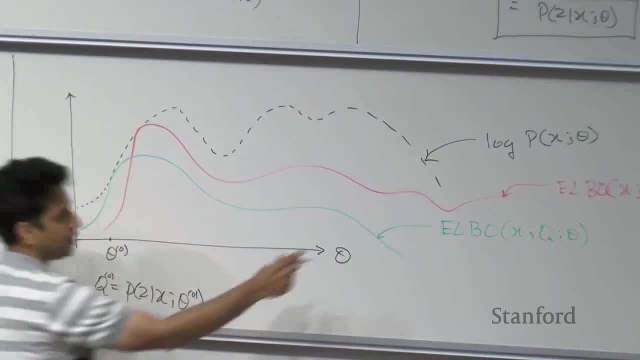 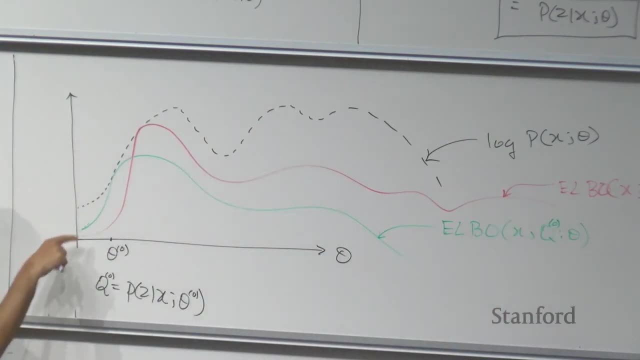 For this choice. if, supposing this is, uh, the albo for q 0,, then it basically tells us that the albo value equals log P of x at this value of- of theta, which means the albo touches log P of x at this value of- of- of theta 0, right. 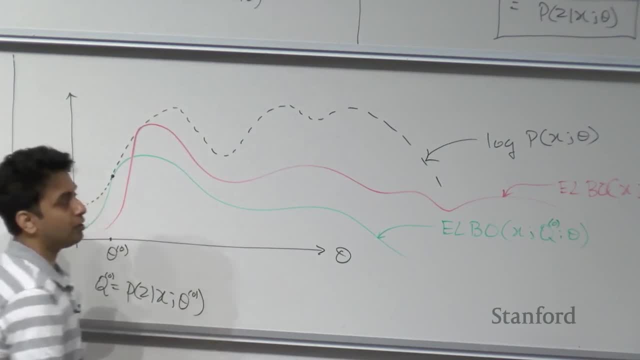 When we are at theta 0, if we choose the q for-, if we choose to construct an albo using q as the posterior distribution with that parameter value, then the albo will be tight, uh, with respect to the invisible goal that we are trying to maximize at that value of theta. 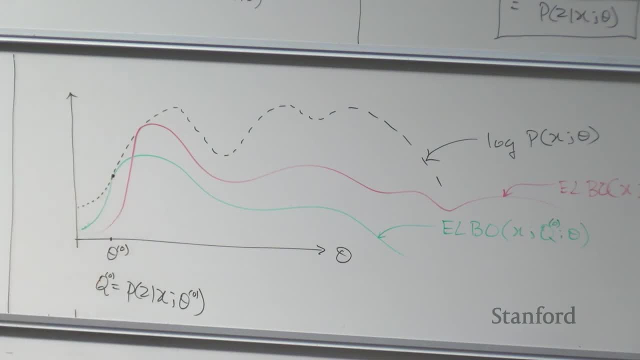 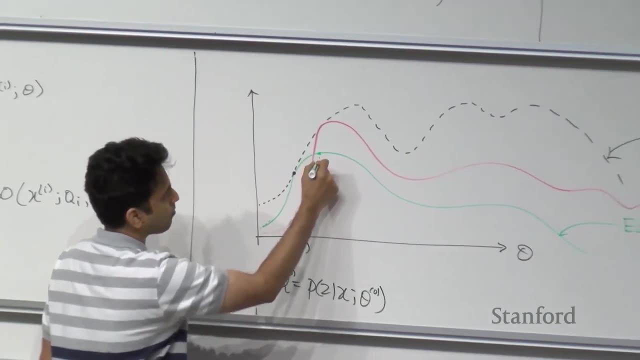 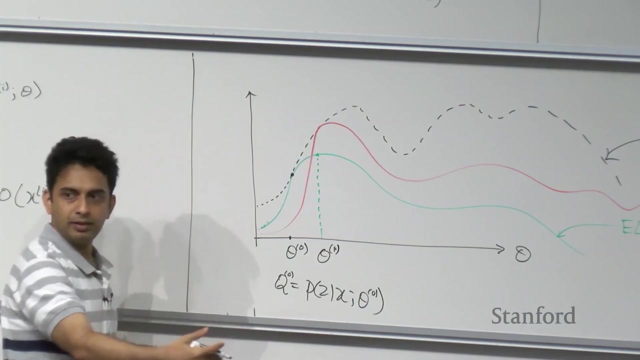 And now, if we maximize in the M-step, if we choose a new theta such that we maximize, okay, if this is theta 1, that is the- the- the- the theta for the next iteration. And now we can uh. 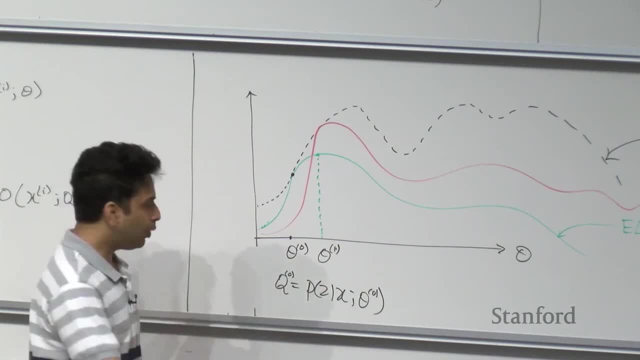 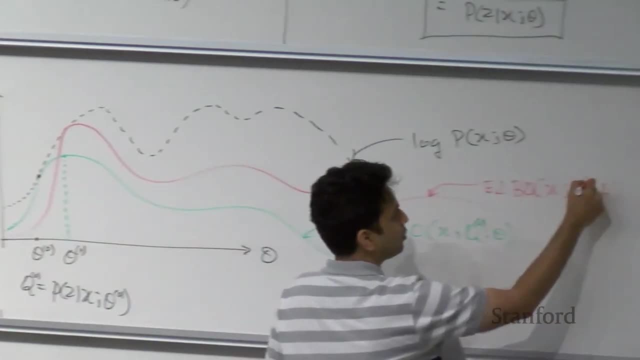 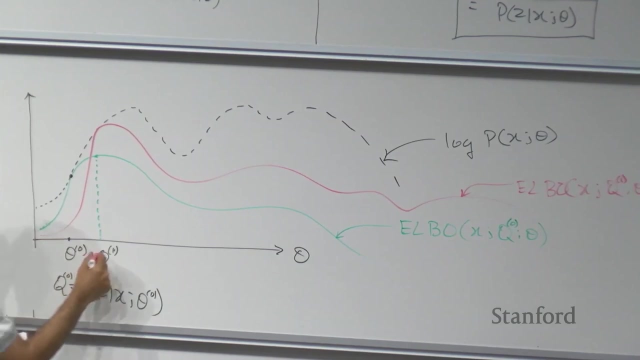 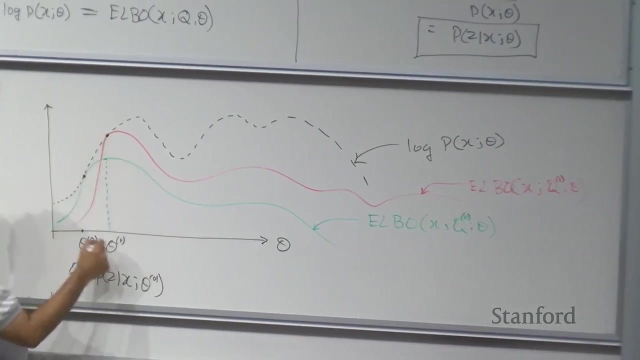 reconstruct yet another albo right Now. the new albo will be constructing- constructed using, you know, this q, q 1, which uses theta uh, uh, q 1, uh. um, then this albo will be- will be tight at log P of x, at theta 1, right. 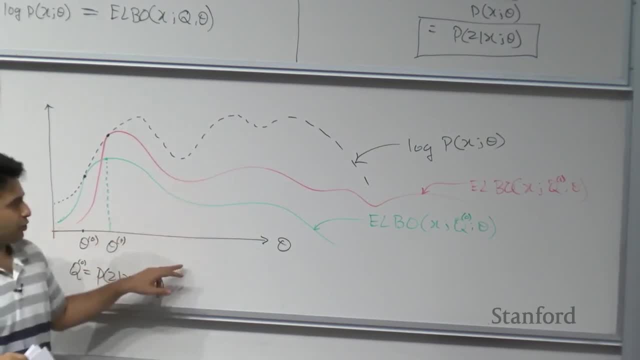 Depending on the uh uh, the choice of the Q to be equal to the posterior, using the corresponding theta value, the ELBO that we'll get will be tight at- at- will be touching the- the log P of x. 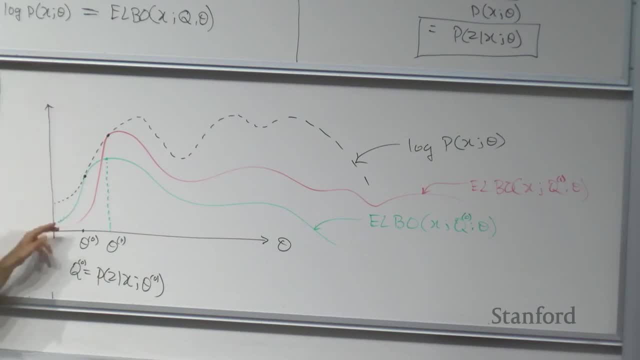 That's- that's what Jensen's inequalities, corollary- corollary, tells us. Now, if we start at theta naught, maximize the- the ELBO, that is the M-step. we get a new theta 1, construct a new ELBO.